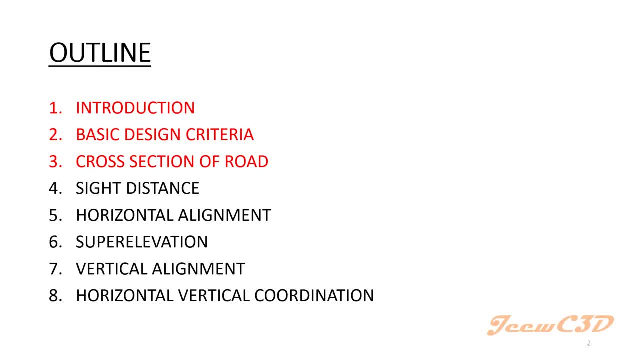 look into it a little as we consider this graph. So here we have a cross section of the road coordination, so this will be taught to you as a part of theories. after that I will be doing these things in a software called civil 3d- how to design roads. 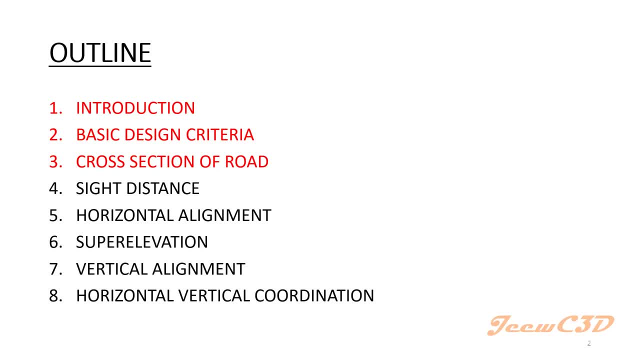 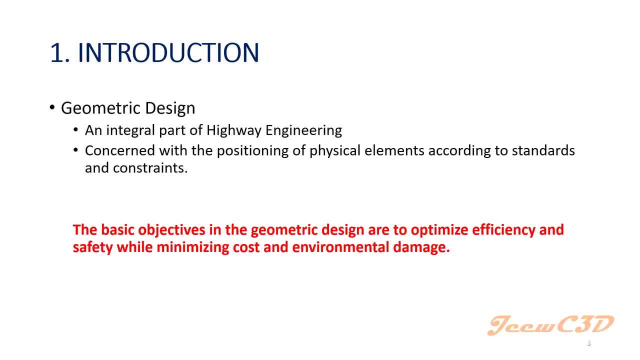 using that civil 3d software. so then I will move on to the introduction of my course. so geometric design is a critical part of idea engineering. you are doing idea engineering. geometric design is very important. you need to know how to do geometric design or otherwise, how to design roads. so it is concerned with the 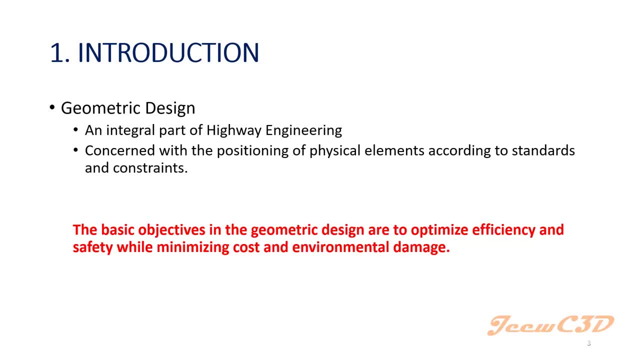 positioning of physical elements according to standards and constraints. so I will describe it in a little bit more in the next slide, but before that, the basic objective of geometric design is to optimize efficiency and safety while minimizing the cost and environmental damage. basically, in doing geometric designs you have to have 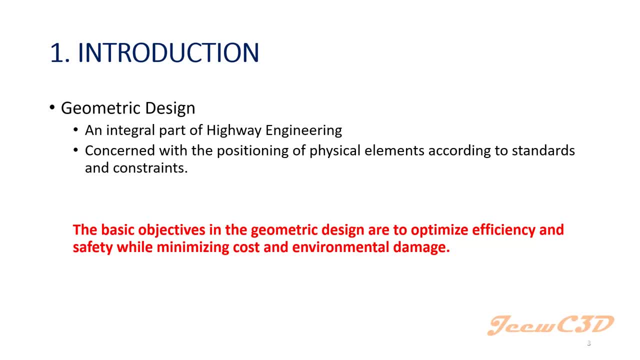 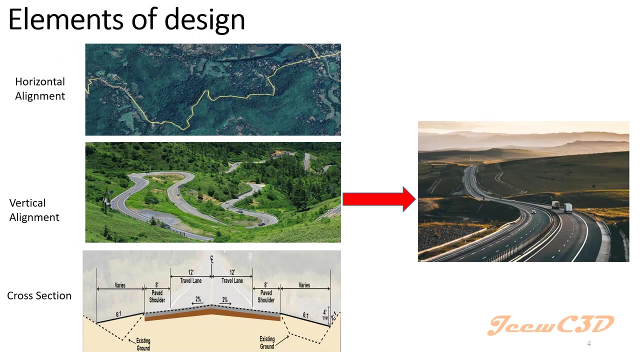 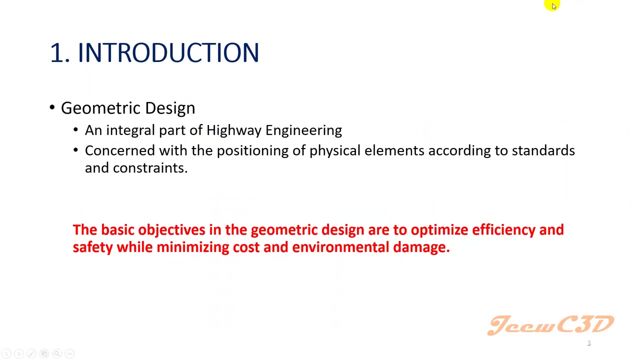 an optimized design so that it will give you efficient road or otherwise, a good, user friendly or driver friendly road, while maintaining safety aspects as well as minimized cost and minimum damage to the environment. so what are the elements? we talked in the previous slide. I told you we are concerned with positioning physical elements. so what are these? 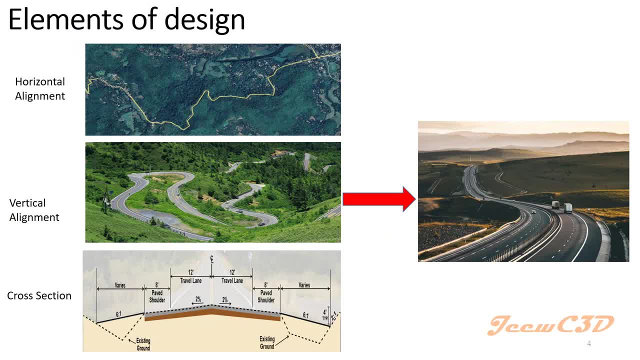 physical elements. there are three physical elements. that is, horizontal alignment, vertical alignment, horizontal alignment, cross-section. also, the alignment is the one we see from a plan view. that means if you see a road on a plan view, so if you think of a way, you see a road on a 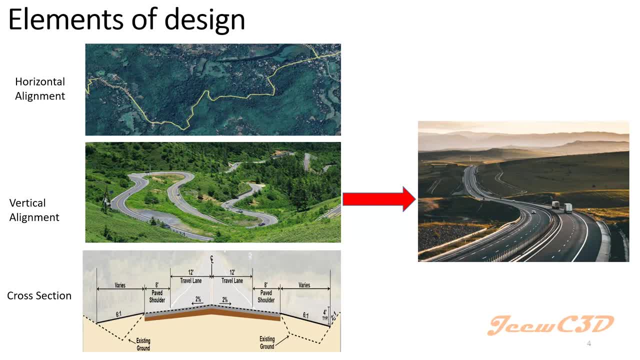 Google map or Google Earth, you will see the road, something like this. so you can't see any elevations here, just a plan. you can see the straight portion, then you can see the curved portion, so you only see the plan view of the road, no elevations. 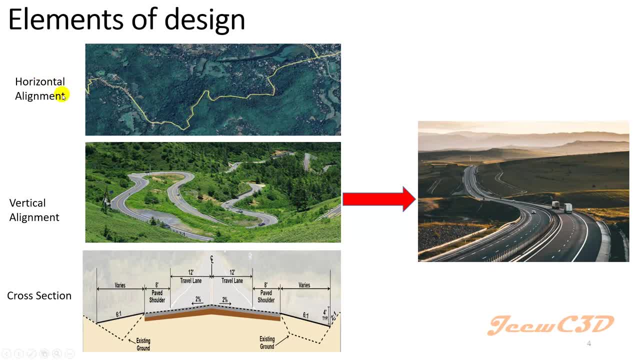 that is called horizontal alignment. then vertical alignment means the elevation view of a road. so if you consider this road, you can see this is coming to a top elevation from the bottom elevation, so we call it vertical alignment. then you have the cross-section. cross-section, as you know, is the width component of the road. here, if you consider, you have the 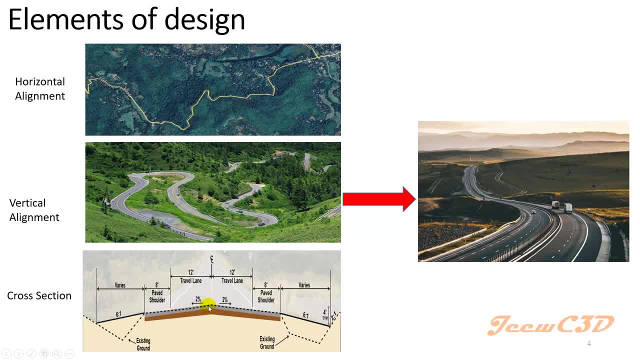 travel lane where your vehicles are expected to travel, and there are some other notations which I will be teaching you in later slides. so the combination of three will give you a nice looking road to you. so you have to arrange these physical elements in such a way that we get a good, efficient road, but we have to ensure that your 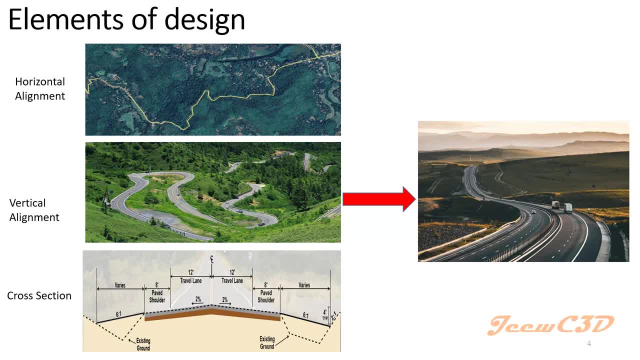 construction cost of that road is minimum. minimum is when I am saying minimum, you have to ensure that the quality is there. you can have a road with minimum cost but the quality may not be there. so when I say minimum cost, you'd have to ensure that it is a good quality road and you have to. 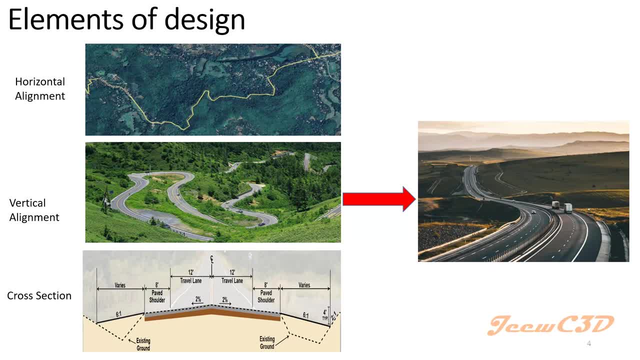 minimize the environmental impacts too, because if you have so many environments, even though you create or construct a good road, there will be some adverse effects to the environment. you will get negative impacts. there will be some adverse effects to the environment, you will get negative impacts- your road. so if you are a good designer, if you are a good design engineer, also constructing a road, 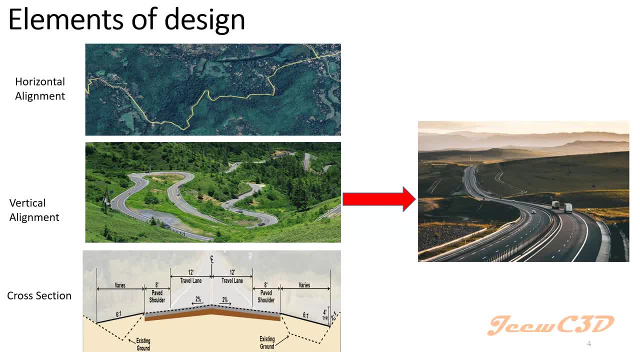 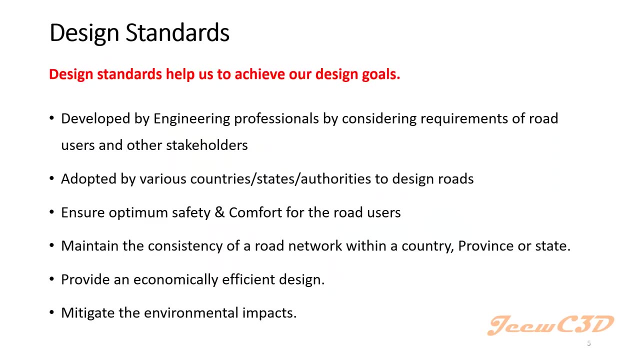 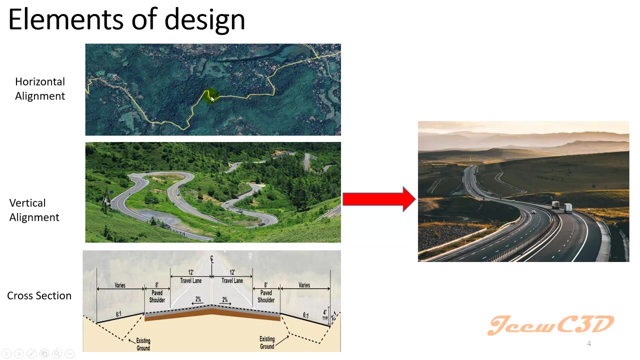 in a proper manner, you will be minimizing the damages to the road, minimizing damages to the environment. that is the best way to do good designs. then, to do a good design, you have to have design standards, because when i say horizontal alignment in the previous slide, when i say horizontal alignment, you need to know what are the curve radius you have to select for. 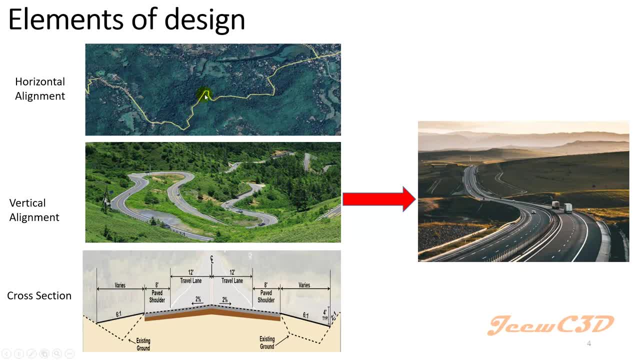 the curve, what kind of straight lens you can adopt, how much of length you have to select to design the road. then you have the vertical alignment constraint. that means what kind of gradient or what kind of slope you have to use for your role. so you can, if you see, here you have. 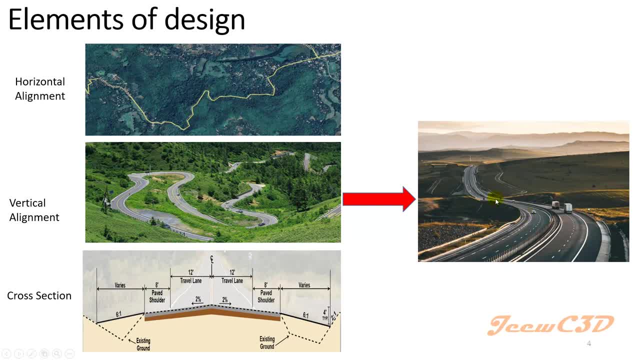 a slope here on the road. so what are the maximum slopes? what are the minimum slopes? what kind of slopes you have to ignore, what kind of slope you have to select? so they have to be decided by someone, otherwise you cannot design a role as you think. there are standards for that. 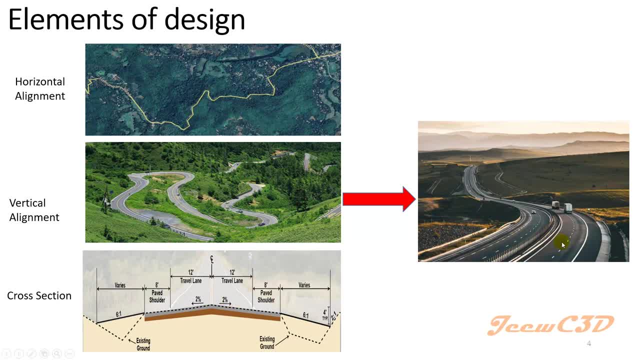 so when you come to the cross section, what are the lanes? what is this? we are calling this shoulder. we have a drain scheme, so what are this type of drains we have to use? what are the lane mix? what is the curve radius? all those things has to be known by someone to design a road. so 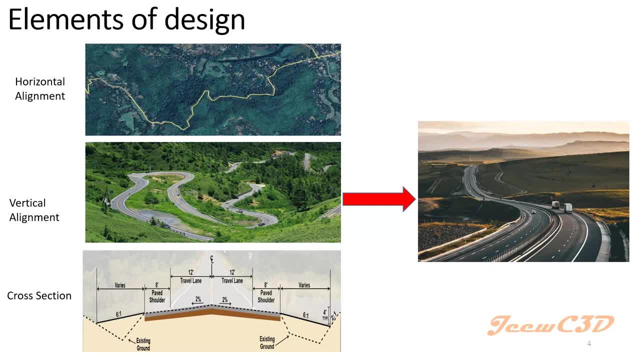 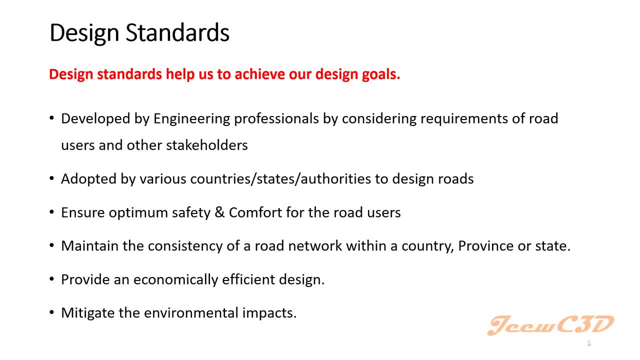 to get a good for the best practice, for best design roads. there are several guidelines in the world designed to create or design roads, so we call them design standards. if you do structural design or concrete design, you have bs standards, american standards. likewise for road design you have 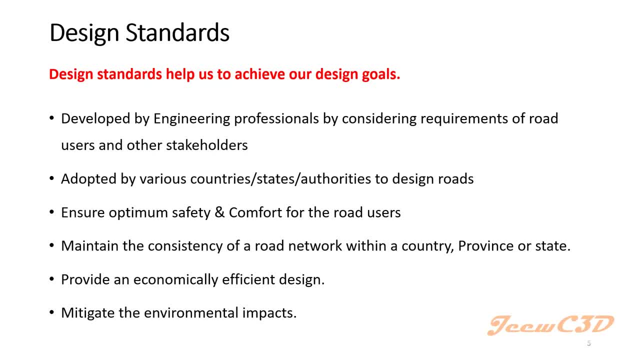 separate design standards. it will tell you what kind of road you have to design, what are the road mix, what are the curves, what are the slopes, what kind of roads you have to design, what are the road curve radiuses. then, the most important thing, when you are designing a role, you have to ensure you 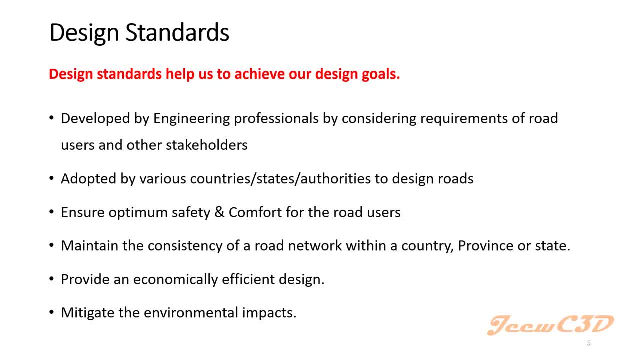 have to think of. what is the speed of the road, what is the maximum speed of the road? so, when you are using that maximum speed, what is the minimum radius you have to adopt for curves? those things are illustrated in design standards, so they are developed by engineering. 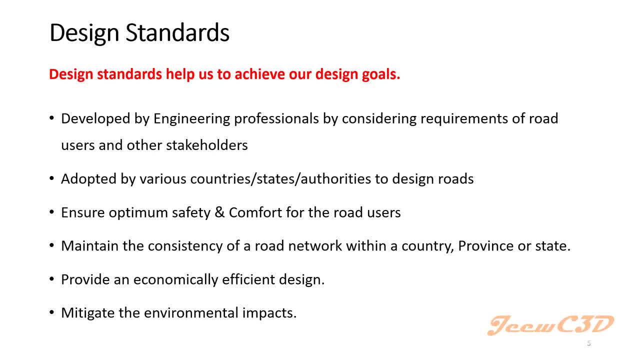 professionals. so it will. they are designed considering the requirement of toll users as well as other stakeholders. so adopt in these standards people can of the design, engineers can design roads in proper manner. so these standards will be changed or will be used in several ways. that means in one country they use one standard here, another country will. 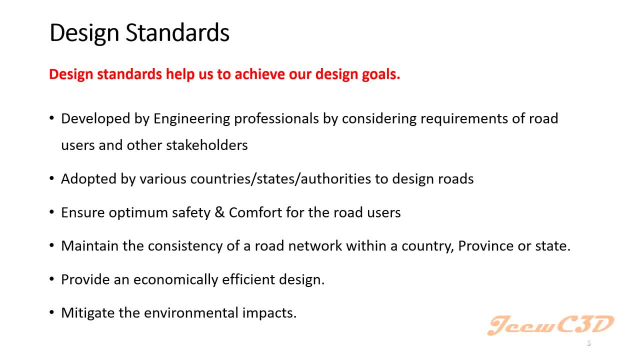 use another standard. so, for example, in sri lanka what we are using is rda road design guideline. if you go to usa or united states of america, they have astro design guidelines. but inside america there are several states- new york, uh, washington likewise- so those states have several. 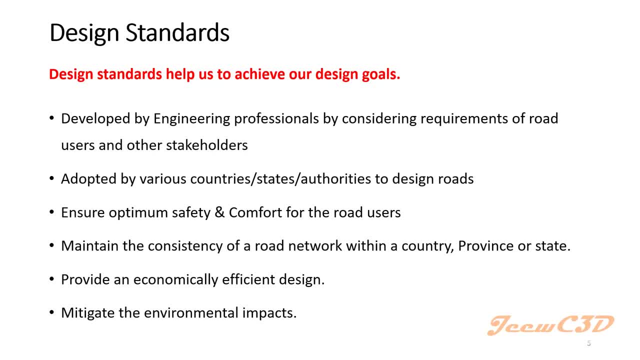 guidelines for road design. so, according to the situation, they have to use various guidelines, but all these guidelines do is what all these guidelines do is they ensure you have an efficient road while minimizing the cost as well as the other adverse effect to the environment or other road users or the other public. 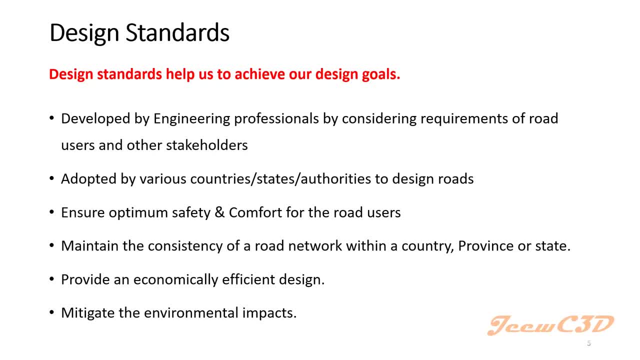 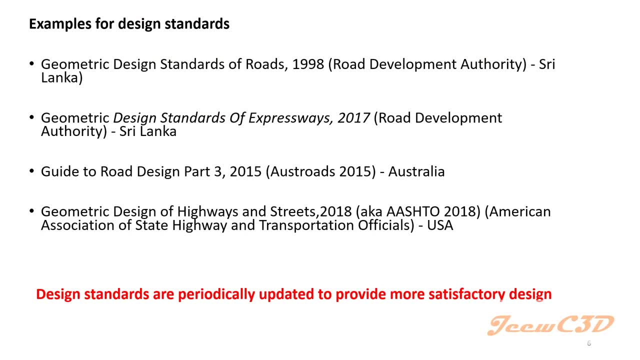 spaces over the people. then you have some examples: design standards. so in sri lanka we have geometric design standards. of course, it is published in 1998 by road development authority. then you have geometric design standards of extraspace, published in 2017 by road development authority. then you have guides. 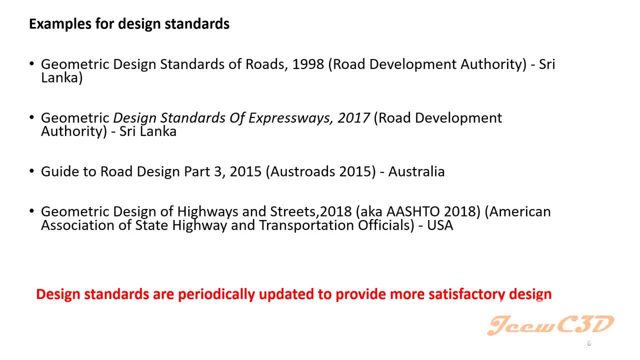 design part 3 for geometric design published in 2015. we call it as offshores 2015, so it is published by Australia. so in USA they have geometric design of IBS and street 2018. that is the latest publication, so it is also known as AKA means, also known as as to 2018, so that 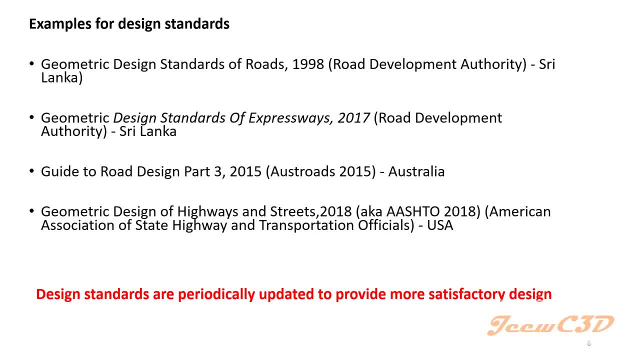 is published in USA. so these guidelines are periodically updated to provide more satisfactory design. because the world is changing every day. so we have to create more sustainable or more suitable design standard to the modern world. so these standards are changed periodically or modified periodically to get satisfactory design of roads. then we 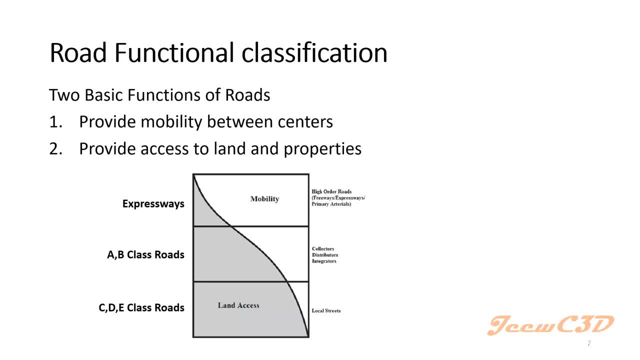 will be looking at the road functional classification. so before designing roads we have to know what are the functions of a road. we have two basic functions of roads, that is, provide mobility between centers and provide access to land and other properties. so provide mobility between center means it is giving a way to travel between two locations. so if you 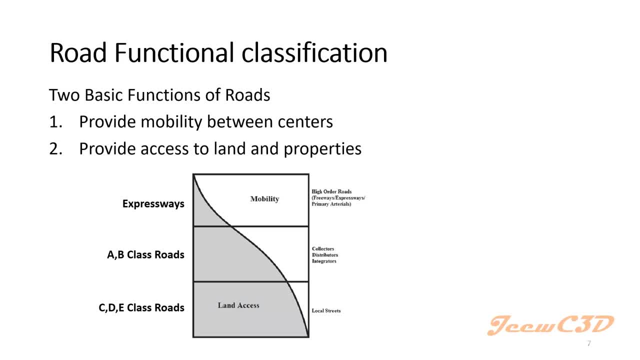 consider you are traveling from Colombo to Kandy, that there are several roads, so we call it. we have a mobility, we get the mobility from, let us say, can be colombo road. so you are getting the mobility from can be colombo road to travel from colombo to can be. so then, after that, 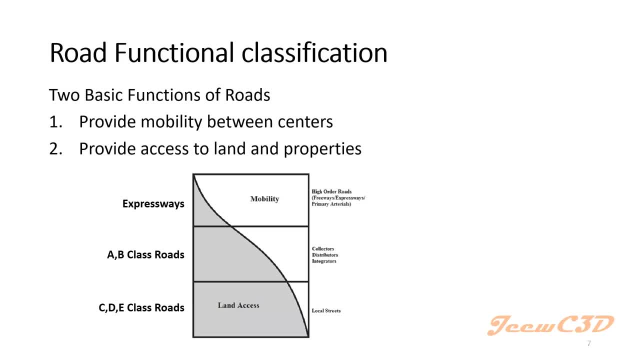 there are some other roads. that means, uh, if you want to go to some other minor location. so if you want to go to your home, it can be- you have to use another small route. a1 road or the colombo candy road is a main road, then you have to use some other small road to go to your property. 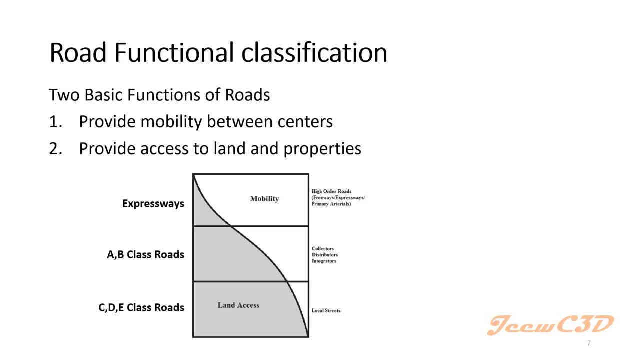 or your house. so you are that. that means you are going to access your property, you access your land to some other roads so that can provide more mobility. but the small road to your house provide more accessibility. it helps to access you. but the main road provides more chance to mobilize. that means it has more speed. so if you 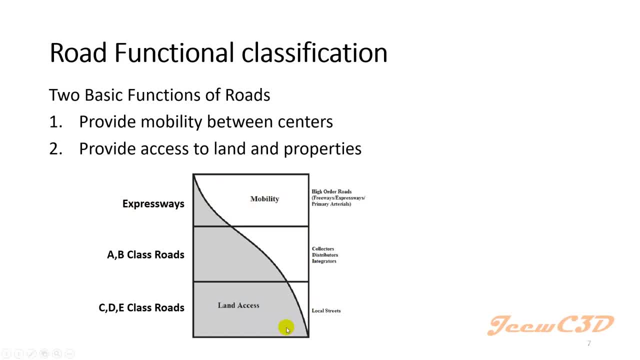 consider this chart you can see express case: have more mobility but less accessibility. that means you can't stop everywhere at the expressway, you can't stop only after going from an interchange. so you have less access. less access but more mobility. but when you come to a b class, 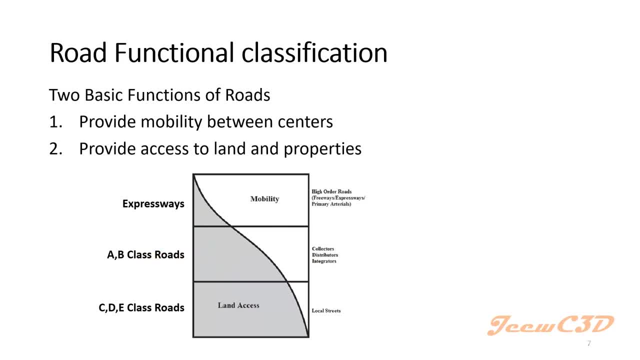 source. that means i will tell you what are the class source later in later next slide. but when the accessibility is coming high, your mobility will be getting lower. when there is more mobility, you have high speed. when there is low mobility, you have high access. so the cde class. 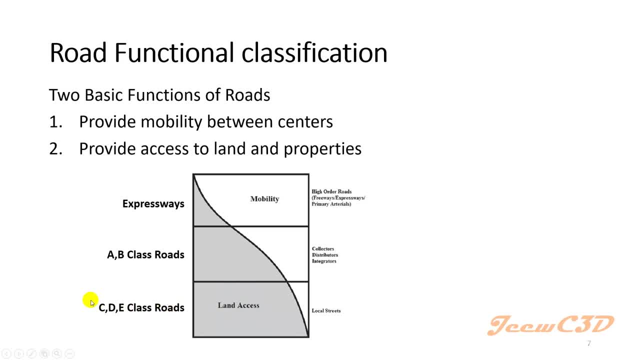 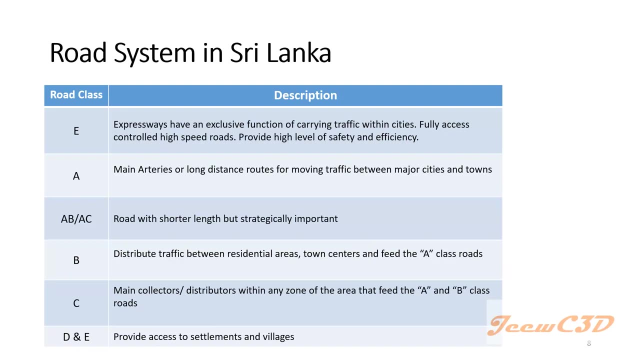 of roads, or in other words, other words, the roads we are using to access our houses have more access, but low mobility, we have less speed. so these are the road system in sri lanka which i talked earlier in the video slide. so class e roads means the expressways, you know. as you go to google map, you will see e1, e2, e3. 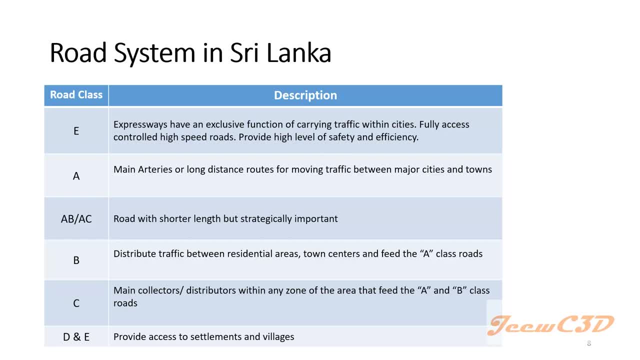 likewise for expressways. so e class road means expressways which we have high uh mobility and fully access controlled roads. so you cannot access the expressway from everywhere. you can access the expressway from a particular location called interchange, so we call it full in access control. 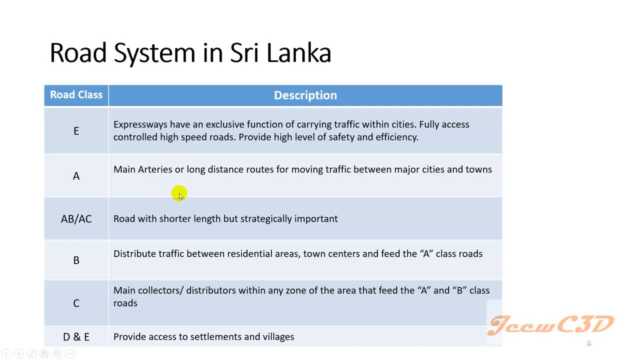 when you go to a class source. still, there is high mobility most of the time, but there are less. it is less compared to expressways. mobility is less compared to expressways but accessibility is high. so going down, you will see, uh, the mobility increases but the accessibility increases. so, a class road, they are mainly the roads, uh. 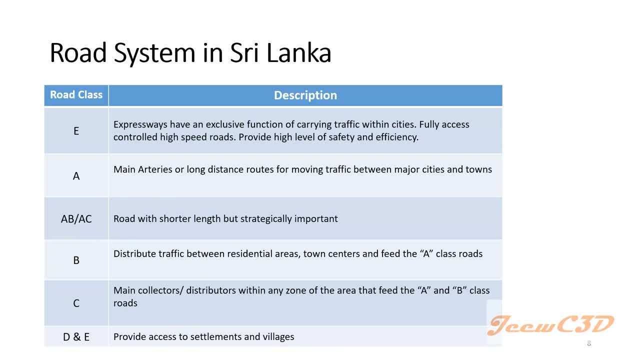 within two provinces. a class stores are the roads within two provinces, then b class rules are the roads within a province, major roads within a province, and a, b and a c cars are major roads. but the road development authority has 13 third south county deed towardsза, so these are from b class. 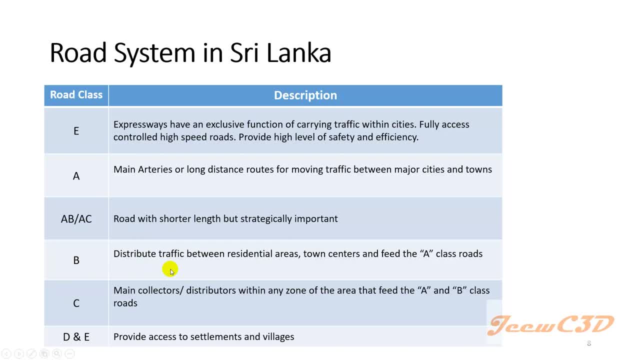 so they are within the province, but they have high importance. so that is why called them abo ac. so let's, because they are within the province. uh, especially this: e, a, a, b, ac and b class stores are governed or maintained by the road development authority, and then the c class stores. 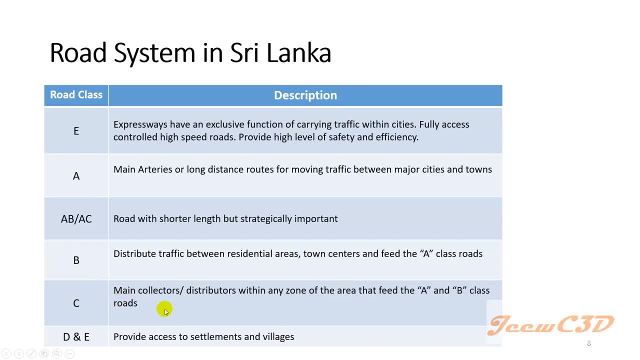 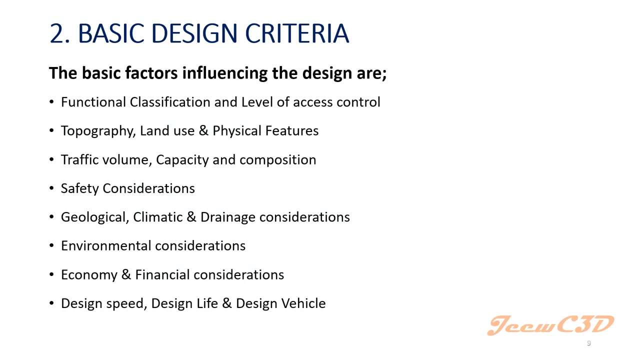 the provincial road development authority, or we call them ERDA. then D and E class roads are the small roads where we used to access our homes or villages. so the accessibility will be increasing downwards but mobility will also decrease downwards. going upwards, you will see mobility increases and the accessibility decreases. then we will look at the basic design criteria. what is the design? 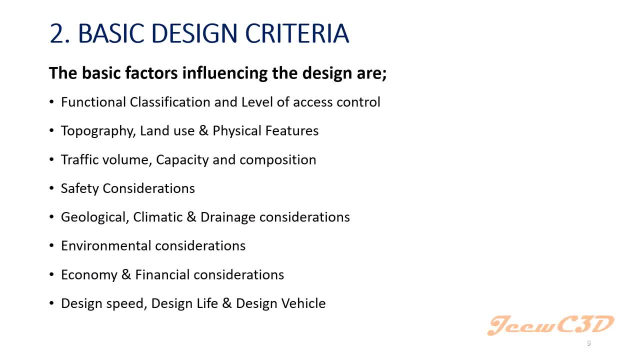 criteria we have to adopt when we are designing a road. so there are several criteria we have to adopt, so i have list out some of these. i will explain this one by one in here. so functional classification. i told you what type of road we are designing, what is the mobility, what is the 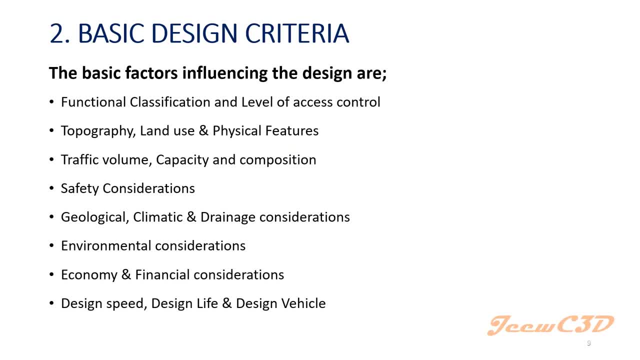 accessibility, whether we are giving more mobility or more accessibility. that is called the functional classification and the level of access control: how much you are allowing to access that road, how much you are allowing to some, how much you will limit. so, if you consider a expressway, we are not allowing the bicycles or three-wheelers to access that road. so 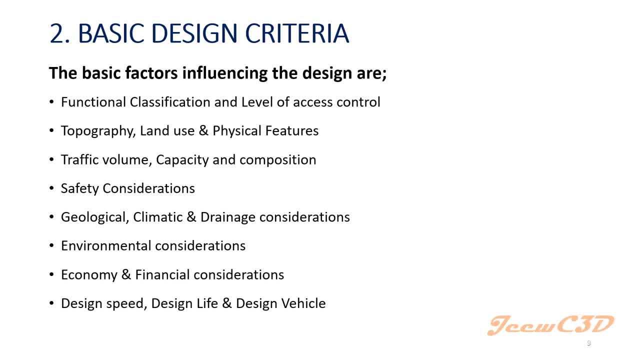 we are keeping some kind of access control for smaller vehicles in an expressway. so that is what what you meant by functional classification and level of access control. then you have the topography, land use and physical features. so these criteria also should be considered when designing roads. so topography means what kind of land, what kind of area you have. i 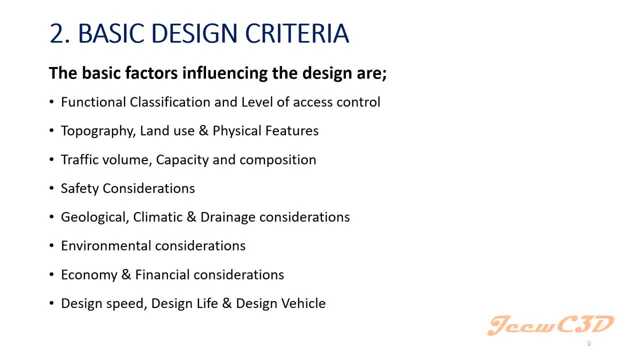 will be discussing in detail in a later slide under vertical alignment, but in general i can tell you, topography means whether you have a flat land or mountainous land, so kind of a mountainous and cut combination land in that area where you design the road. that is mean by the topography then. 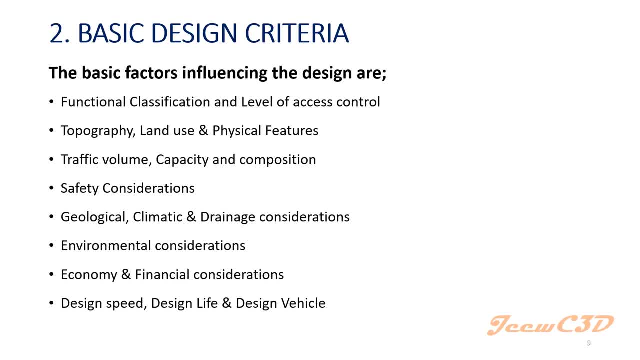 land use means what kind of use in the land in that area. so if it is an urban area, you have high land use. you have buildings, schools, pieces, industrial zones. likewise, you have high land use. if it is a rural area, the land use is very low. you have small houses here and they are 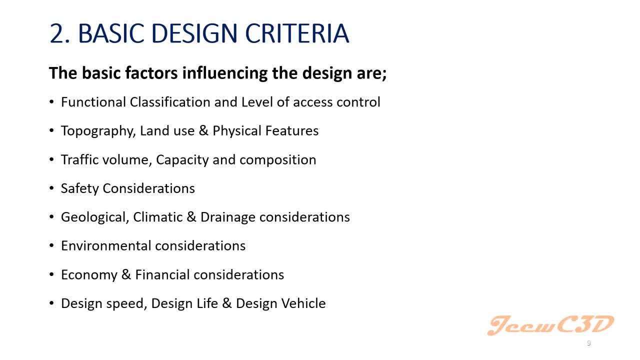 the congestion is very small. so the land use means whether it is urban area or rural area or some urban area. likewise, the other hand, the physical features are. there may be reverse historical locations, buildings, trees, so you have. they will affect the design of your road. so also we call them constraints, which will affect your design if there is a. 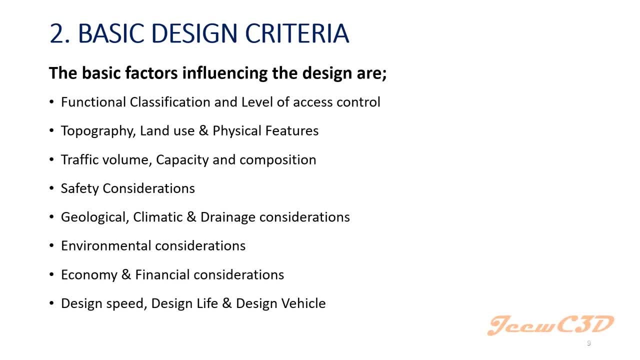 so let's you assume that you are constructing one, so you are designing a road in a new area. if you are supposed to design a road in a new area, if there is a temple in that road trace when you are designing, if you have a temple in the protest road trace, you cannot demolish the temple. 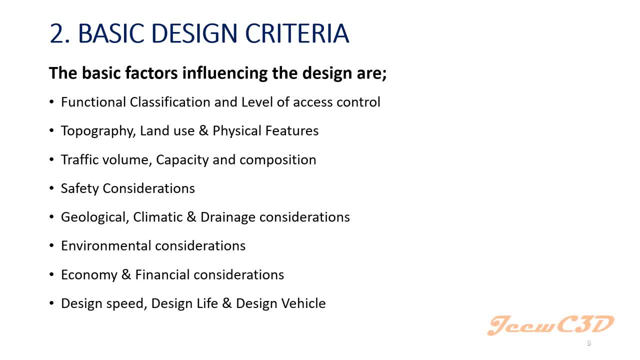 you have to redesign the road so that the temple is not affected- so we call them constraints when you are designing. so you have to address those constraints while you are designing. so those are the topography, land use and physical features we encounter in for design. then you have traffic. 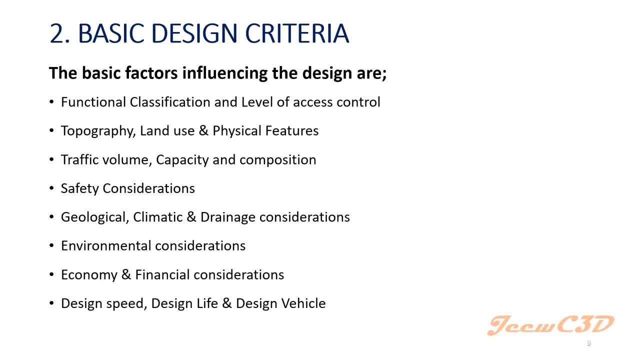 volume, capacity and composition. so traffic volume is how much of traffic you have. that may be traffic volume per hour, traffic volume per day, traffic for some period of time, so you can measure much of traffic in the toll. when you are designing the road you have to measure that volume and then 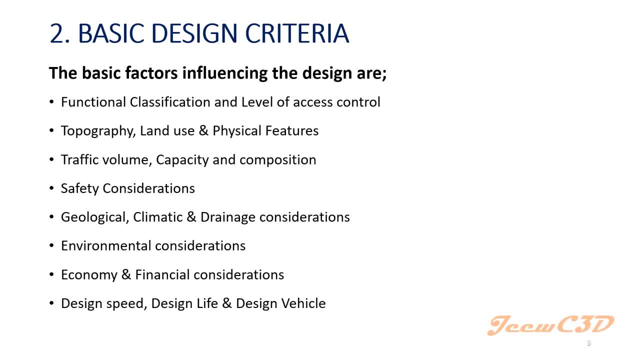 you have to forecast the traffic for a future period. that means from the date you from the, from today to 20 years ahead, or 15 years ahead, what kind of traffic might be there? likewise, you have to design the traffic volume when you are designing the road. so then, what is the capacity? 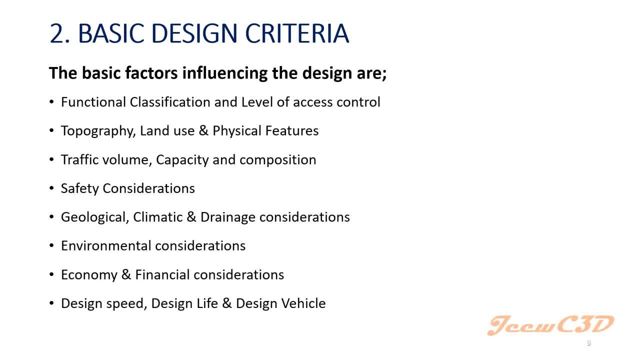 of that road. so how much vehicles that can be accommodated in that road section? so if it is a smaller road, if there are so many vehicles coming, the capacities of the road is smaller, so your road will be getting congested. so likewise, you have to think of the. 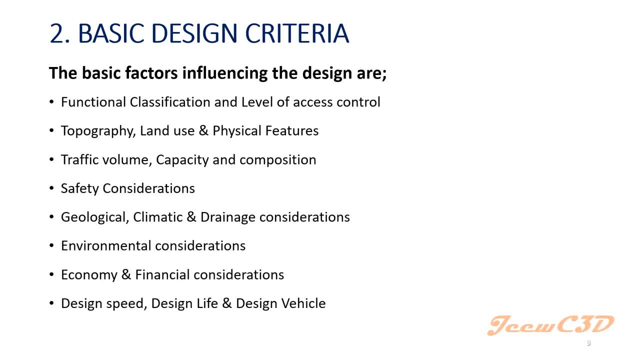 capacity of your road. so, depending on the capacity of your road, you have to accommodate one lane, two lane, three lane, four lane. likewise how many lanes you have to use then the composition of your traffic. composition means what kind of vehicles you have in your road, if you have so many. 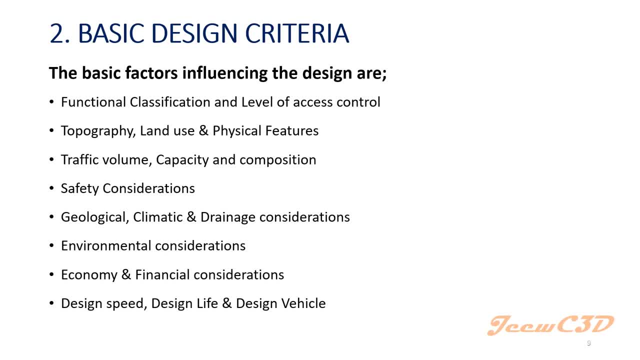 cars, or if you have so many lorries, of course you have so many trucks, you have your so many uh three dealers or bicycles you have to design for you to consider that fact in the design. so what kind of vehicles? what is the composition of the vehicle? how many percentage of trucks? how many percentage? 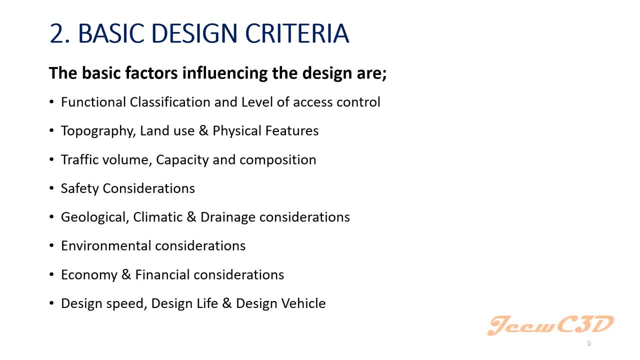 of cars will be going in this road. depending on that, your road cross section may be varied, vary, your design of the road may be varied. so these things you have to consider, then, more important, with the safety considerations. so it is an integral or essential part of road. 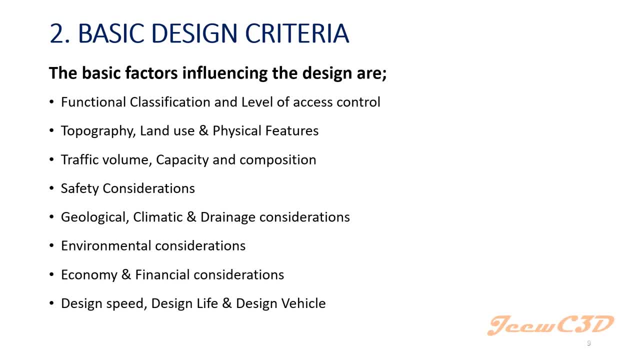 design. you have to ensure that you provide enough concert to consideration while designing the roads. so when you are designing a road, you have to use proper radius for curves. it it depends on the design speed of the robot, so we will be discussing them. then you have to provide guard rails if you have sharp curves and steep slopes. so you 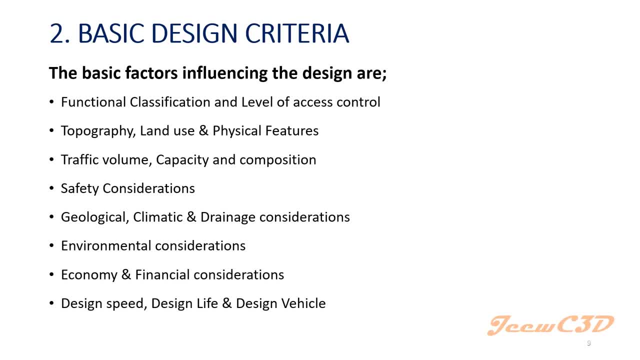 have to provide guard rails which will prevent the vehicles from falling down to the steep slopes. then you have to use proper sign boards on doors. you have to use proper lane marking and if there are so many bicycles on the road, you can have a separate bicycle lane. 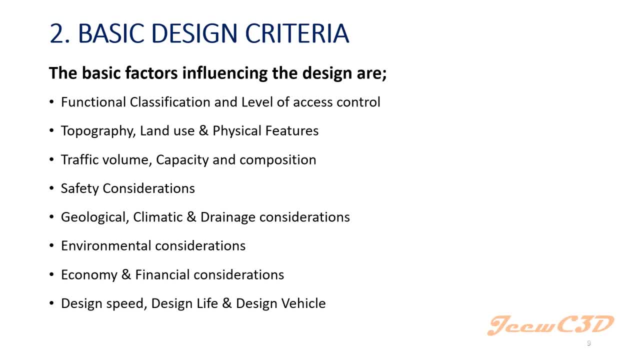 so the bicycle users are getting more safe driving. then the geological, climatic and pernage consideration. so in that area of where you design the road, there are many different landslides. there may be slope stability issues, there may be flooding, there may be marsh. 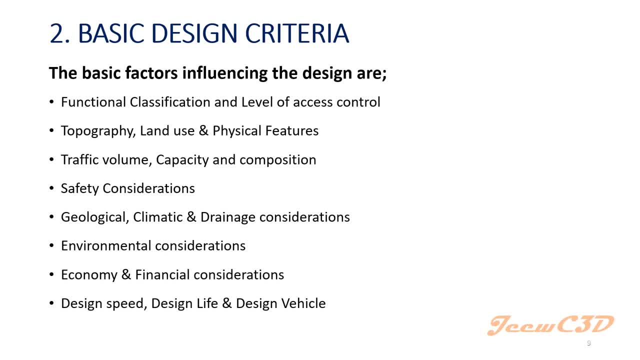 lands there may be settlements on the ground. so we have to consider these things when we are designing the road and we have to address those issues or address those constraints before these will be more hazardous problem to the road. So we have to consider those. 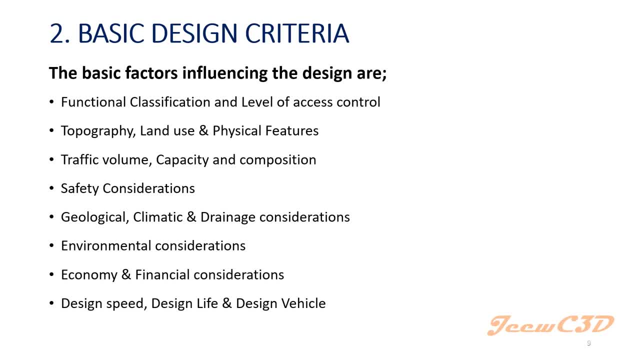 issues also, we are designing the road and the other one, environmental consideration. so we have to minimize the damage to the environment when we are designing a road. So let's, for example, to design a road. So let's, for example, to design a road, for example, to design a road, for example, to: 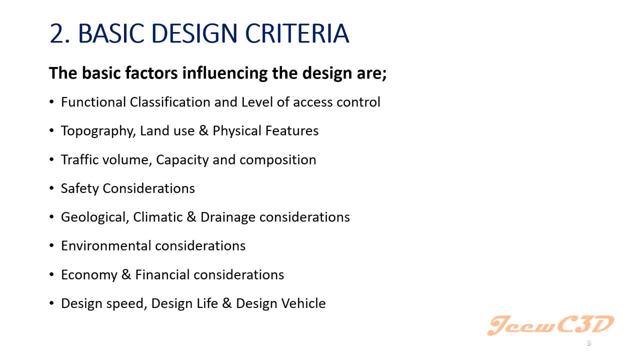 to construct a road. once you design the road, when you are constructing it, after designing when you are constructing it, if you are cutting a mountain, it will be a huge environmental impact. cutting mountains means it will affect the trees or the fauna floor or the animals or natural. 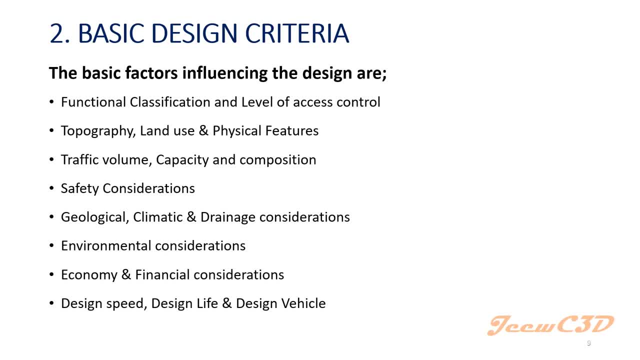 habitats in that area it will affect, then it will have affected the ground water table, if you can remember this. uh, there was a certain issue on the over promise you can do regarding a tunnel, so there was water issues for the people, so you have to consider these things. so 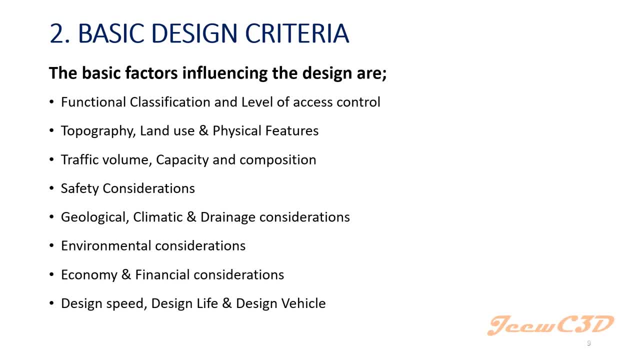 if you have some many mountains and you have so many rope cuttings, so many cut sections in the mountains, sometimes you can accommodate paths in that area to minimize the cuttings of the mountains, but in the meantime you have to ensure that the people will be less affected by the 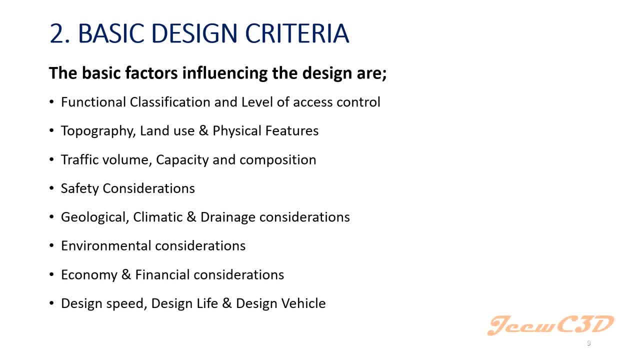 channels, and also you have to consider about the wildlife or the animals or the species in that area, so you have to minimize the damages for them also. then, one of the most important things: economy and financial considerations. so, whatever you do, you have to do it economically and you have to do it within the, within the minimum cost, as well as within the best. 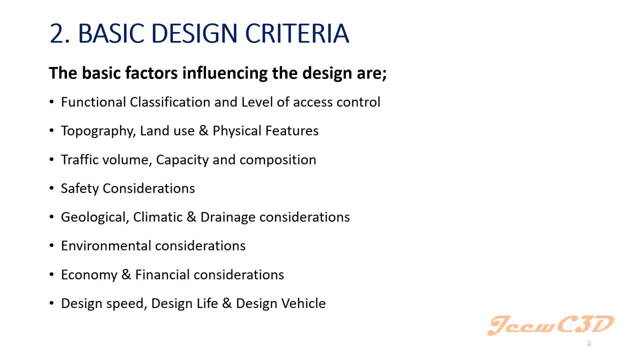 standards, so you have to. you can design a robot with best standards, the best possible way, but if it is taking so much of money, that is not a good design. you can design a road with minimum cost, you can construct the road with minimum cost, but the quality is not there, so that is not a good. 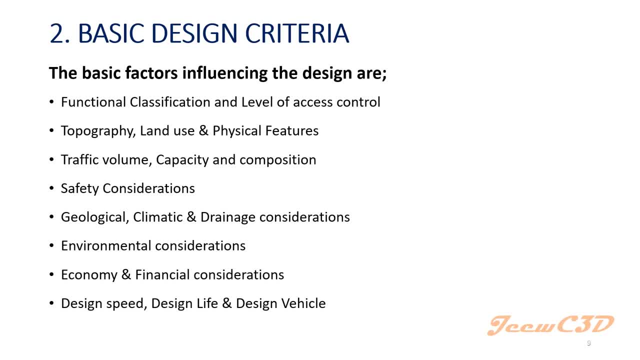 design. so you have to balance the economy and the safety and the comfort of the road within the firm's budget and financial consideration. finally, but even though it is final, that is one of the most important things: design speed, design life and design vehicle. so design speed is what is the. 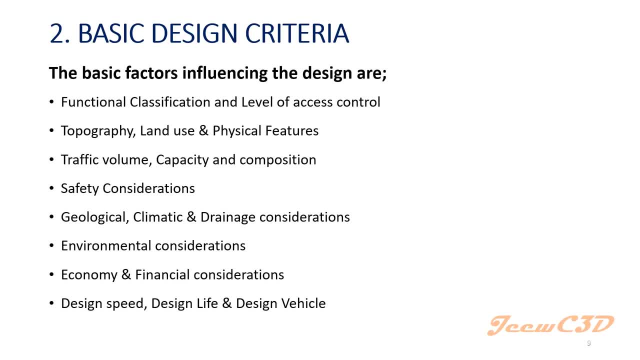 speed we are allowing in that road. actually, there are two things we have to consider. sometimes we we are allowing the road, allowing the road users to use the designs speed, or we are not allowing the road users to use the design speed. that is something like this: let us say we are designing a road with a speed of 80 kilometers per hour. that means 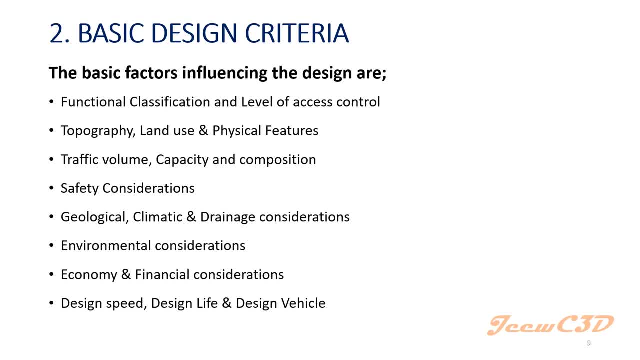 in that road the drivers can go at 80 kilometers per hour without any problem. but when you are doing the sign boards or by government regulations, we will tell you can't go beyond seven kilometers per hour. that is for the safety that we are designing the road for 80 kilometers per hour, but we are allowing only seven kilometers per hour. the 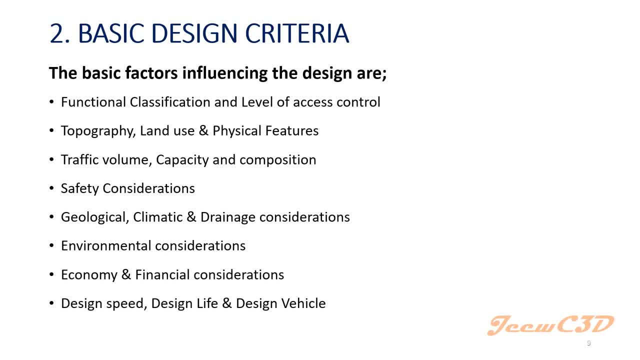 additional 10 kilometers per hour is for the speed. so that is for the design speed of the road. what is the speed? what is the maximum speed? you are designing the road, so this design speed affects the radius of the road: horizontal, equal to horizontal alignment, which we will be, we will be learning later. so it affects the horizontal. 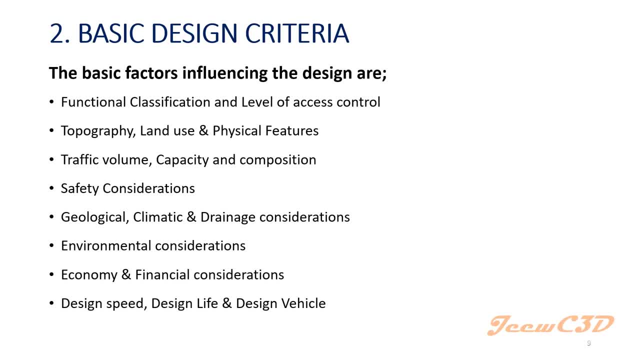 alignment as well as the vertical alignment. so design speed is what is the maximum speed you are allowing in the road, in that road? design life, that means how much of the road, how much is the life of the road before doing any rehabilitation or before doing a modification to the road? what is the 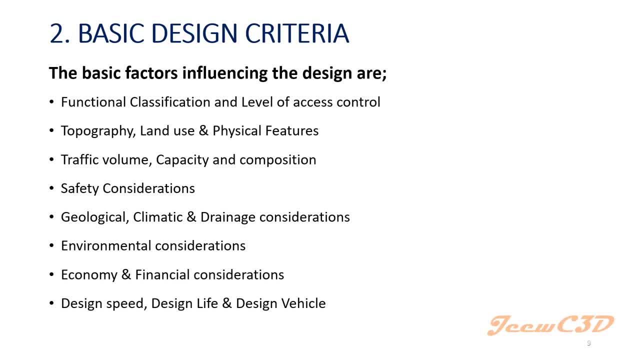 design life. that means after the design life, you have to remodify your road. that means you have to. you may have to increase the road width, you may have to do a new layer on the road, what we call it overlaying. that kind of thing may be there, but within the design. 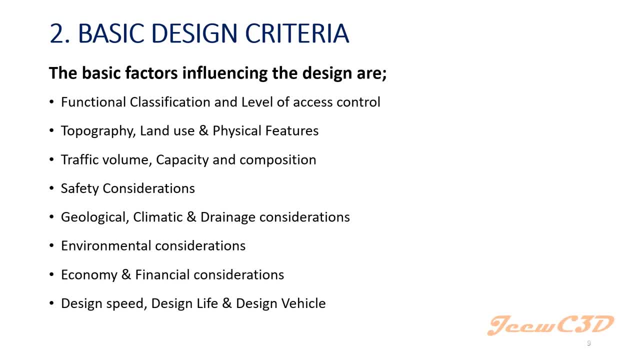 life you have, your road should be provide it should. the road should provide its safety and comfort driving to the road users. within that time period When one of the most important thing- design vehicle, design vehicle- is the vehicle that is supposed to, that. the design vehicle is the vehicle, the largest vehicle that is frequently. 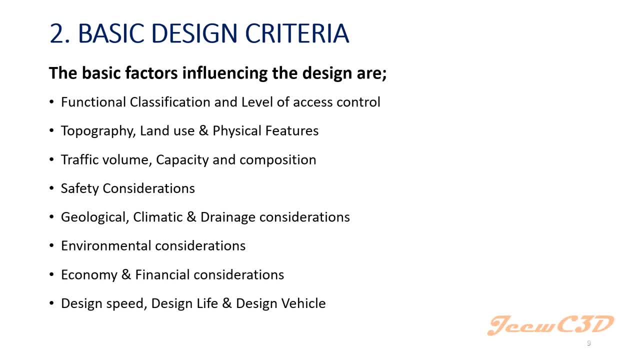 running on that road. so this design vehicle affects the curve radius of the road. so if you have very large vehicle you should have- car parliament주 co- Search Portędipol- larger curves, otherwise these vehicles cannot be turned in that story. so but when you are selecting the design vehicle, you have to select a vehicle that is. 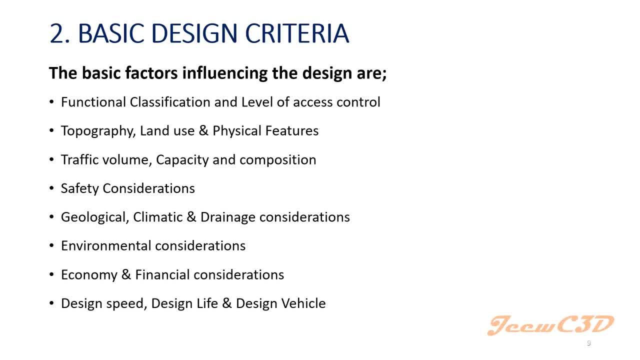 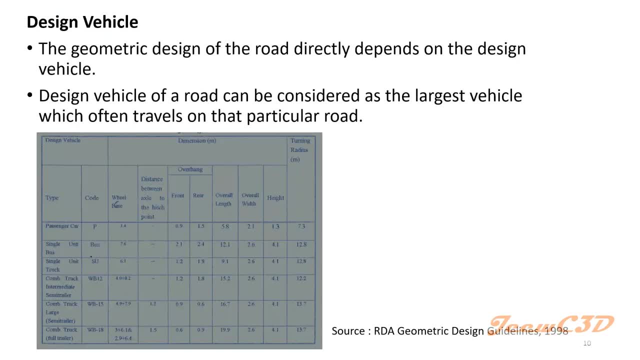 frequently running on that road. let us say you have. I will move on to the next slide to show you the design vehicles. these are the design vehicles that we use for RDA. so you have this single unit truck. you have. you have the dimensions here. signal unit truck. we call it a SEO, so it's overall it is 2.6 meters and it. 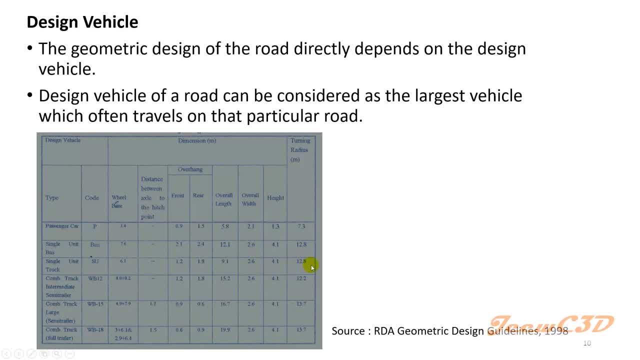 has a turning radius of 12.8 meters. so again, this truck is very often running on a road. so you have that. if, if there needs that, if that this truck is the maximum vehicle in that road, you have to design the road using two-heighter single-unit truck. 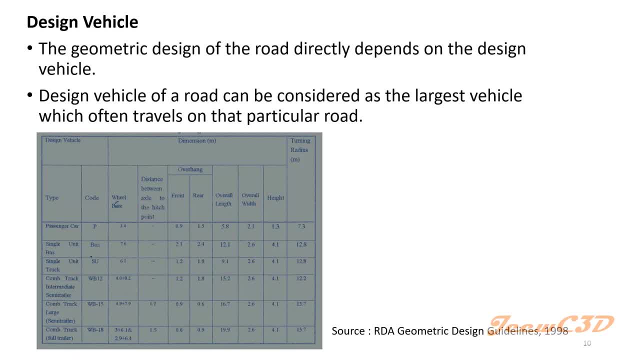 or you have to assume that this truck is frequently going on that road. But if you are going to design the same road for this combo truck, which is rarely going in that road, let us see only once a year this truck is going on that road, so you don't. 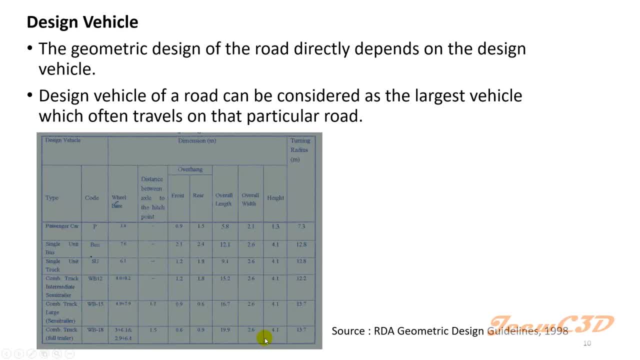 have to design a road for combo truck which rarely runs on that road. you have to design the road for a design vehicle that is frequently running on that road. but that frequently running vehicle should be a larger vehicle, otherwise there is no point. so if you say: 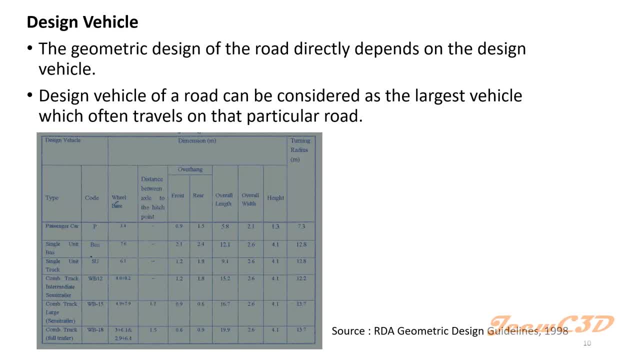 if there are so many cars in that road, you cannot design for cars but you have to design a larger vehicle, such as single-unit truck, SU truck or combo truck, intermediate semi-trailer, WD-12, likewise. so these are the dimensions of design vehicles. so the design speed, design. 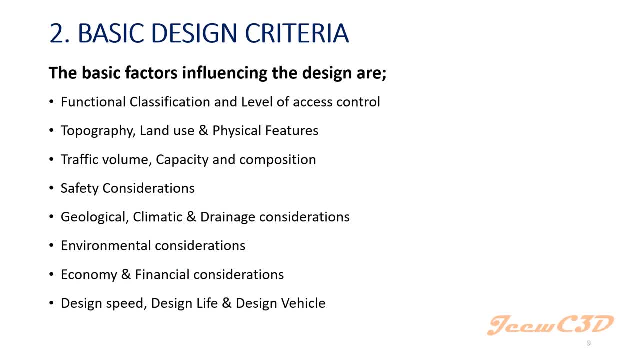 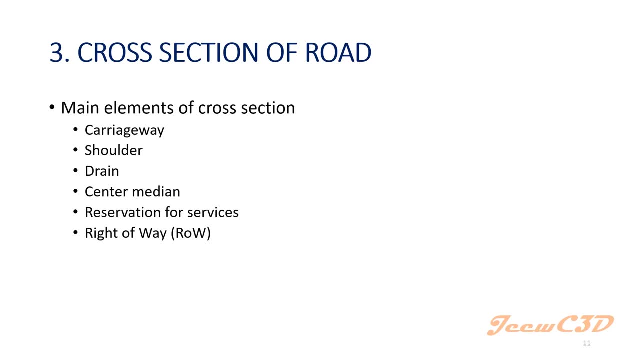 life and design vehicle are very important in basic design criteria. So these are the main things we have to consider when you are doing geometric design. Then I will move on to the cross-section of the road. that is the last part we are discussing. 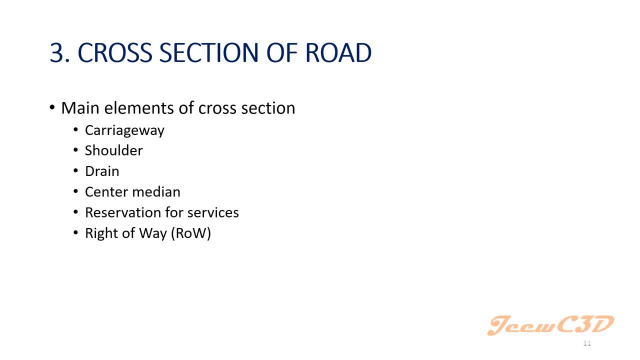 in this session. So what is the cross-section of the road? These main elements of cross-section of the road is extracted from the RDA design guidelines. since we have discussed it- We are living in Sri Lanka, we are considering, we have to consider both the local roads. 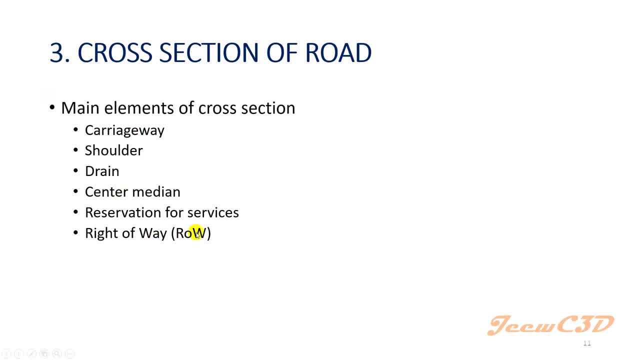 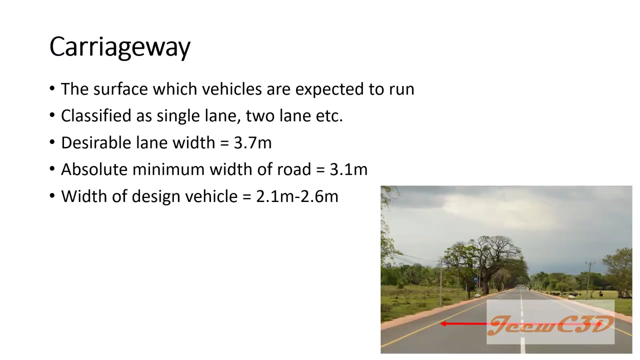 so these definitions are extracted from the RDA design guidelines which I told you earlier, the guidelines we used for local road design. so these definitions are taken from this. so the values given in these topics in the later slides are extracted from this. First, the term carriageway: it is the area where vehicles are expected to run. so if 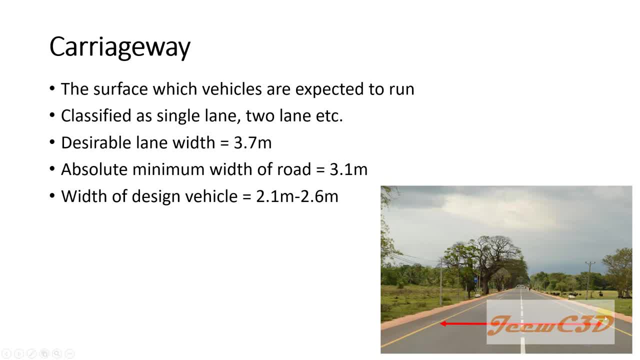 you see this image. you have two yellow marks. the width between these two yellow marks, or the lane edges, are called the carriageway, so this is where your vehicles are expected to run. So in Sri Lanka we are calling the desirable lane width is 3.7 meters, but it is kind of 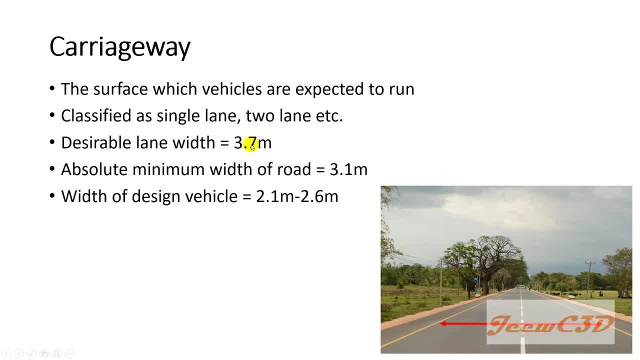 a larger value, we have to. normally we are using plus than that, maybe 3.5, 3.6,. likewise, And if you are using a minimum value for the road width, the absolute minimum should be 3.1 meters. 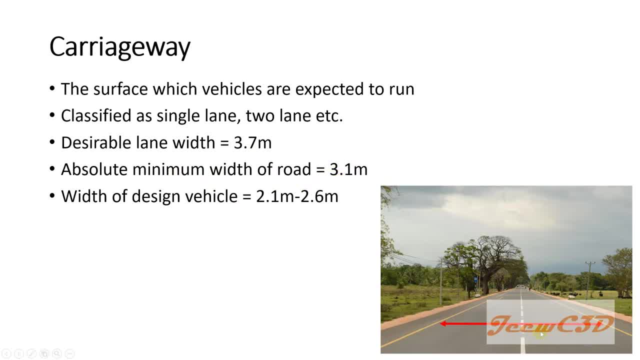 To use lane marking at least your road should be 3.1 meters. So your design vehicle width would be 2.1 to 2.6 meters. So that means if you have 3.1 meters width of the road, your design vehicle may be enough. 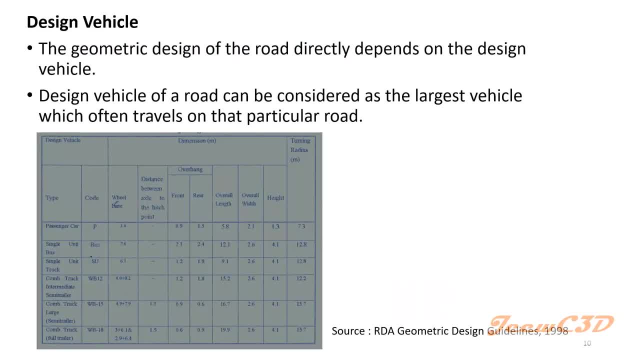 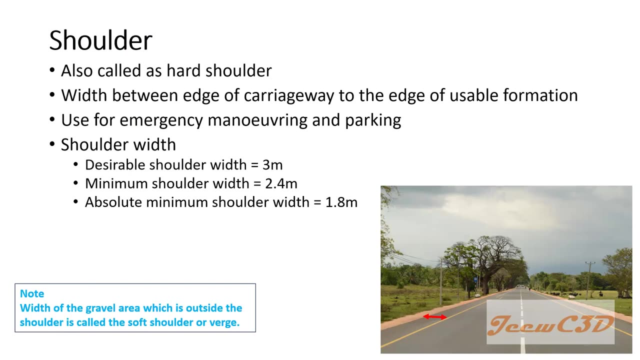 to travel in that road. So in Sri Lanka if you have 3.1 meters width of the road, you have overall width of the vehicle 2.1 to 2.6.. Then we will move on to shoulder. 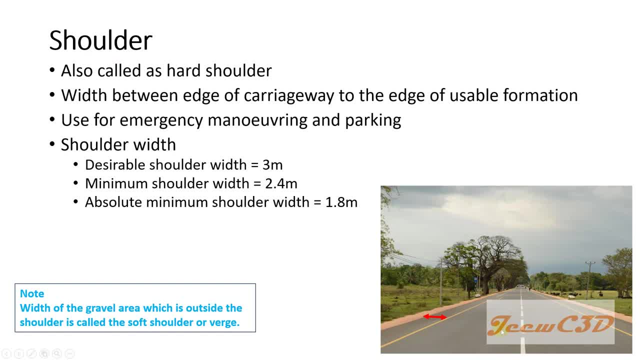 Shoulder is the paved area. Paved means you have as cold here this black color material. we hold it as cold. so after the lane you have some extra width of this road. So after the lane you will have some extra width of this road. 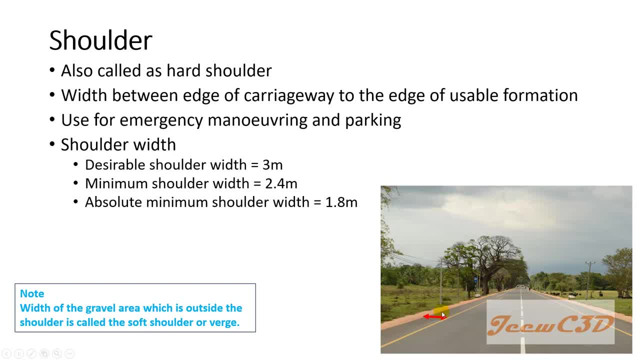 So after the lane you have some extra width of this road And then you can see, you can see these main various interlaces here, because you can see extra with as fold here, equally shoulder, it will use, it will be used to, will be. 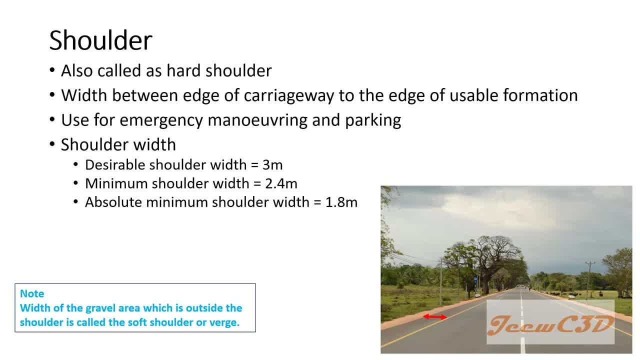 used as to give the lateral support to the payment this will give. this will part will give you a lateral support without going out. so one function is to do lateral support. the other function is to use as an emergency memory for parties a vehicle break down in this area. the vehicle can be parked in this. 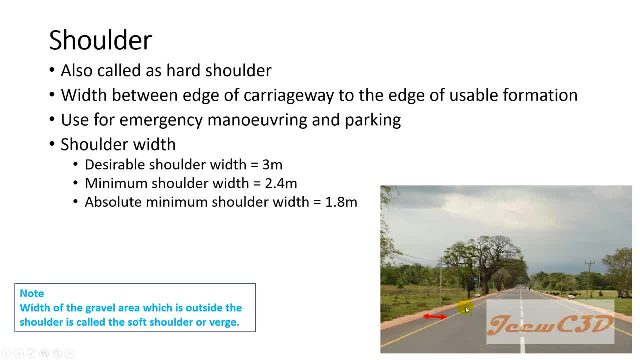 area. so that is why we are using a shoulder, so the designable shoulder with this three meter, and minimum shoulder with this 2.4, and that, so your minimum shoulder with this 1.8. but locally we are not practicing these values, since these are too high values. so 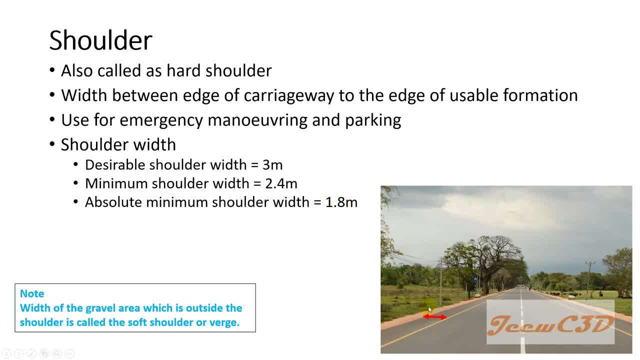 if you adopt these values, your road mix will be very high, so the adjacent lag have to be acquired to construct that kind of road. usually, if they are not express based, if they are not express based, we are not using these kind of values. usually we are using 1.5. 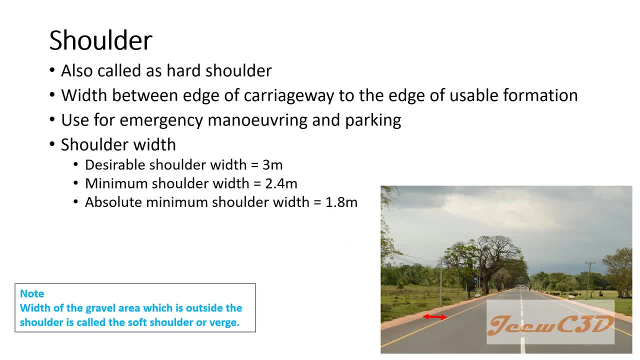 or 1 meter point 5, like I spoke, so really you can see there are other soil area or gravel area. after the usual, this is the day of shoulder. then after you have some gravel area, that is called soft shoulder or words. so this one we usually call your shoulder, or in Sri Lanka we call it on shoulder, this gravel. 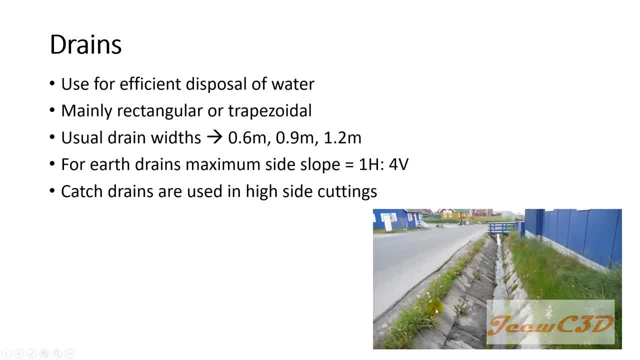 part- you call it soft shoulder- then we will be moving on to the drains. so adjacent to the road you will have drains to drain off the water collected into the road or when, in a rainy situation, we have to use drain to collect the water and drain them away from the road so you can have earth drains. otherwise you can have 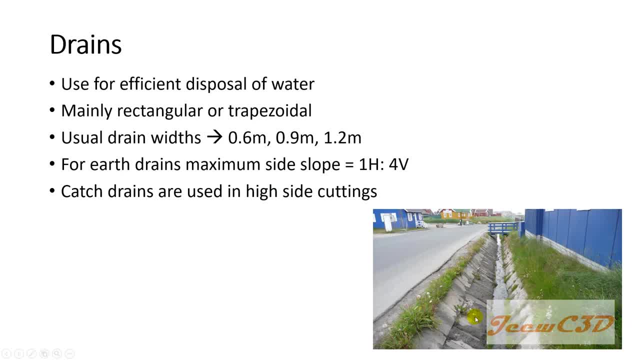 there may be this kind of v-shape drain or sometimes there may be rectangular drains. so usual drain needs are 0.6 meters, 0.9 meters, 1.2 meters. that means that is for this rectangular drains. so if you have an earth drain, that is drain is formed using the existing ground. 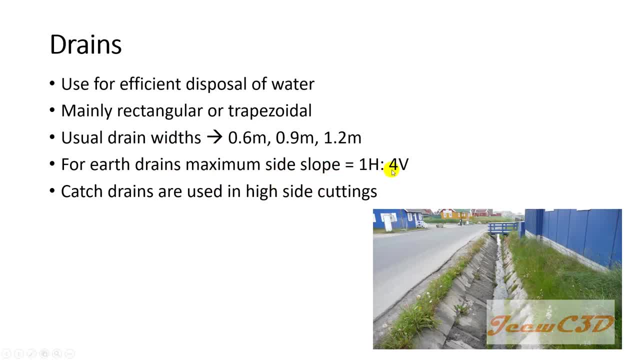 so this slope would be 1 horizontal to 4 vertical. that is the earth drain. if you have earth drain in the floor section, then you have catch drains which are used in high cutting sections. that is the drains which we used in high cut areas. so you can google this thing or search in internet what are called catch drains. 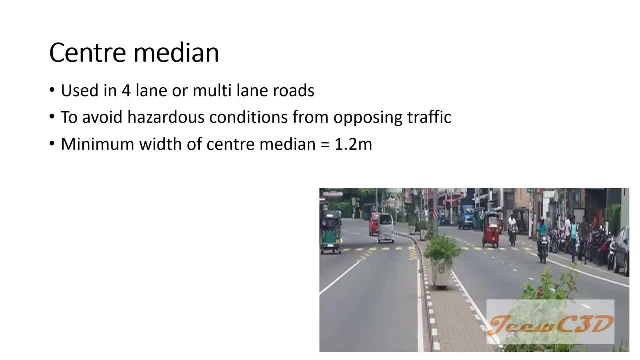 you will see what are catch drains. then you have the centre medians. when you have more than 2 lane load site wise, such as 4 lane roads or 6 lane, like multi lane roads, so the road is divided into two parts by having a centre median. 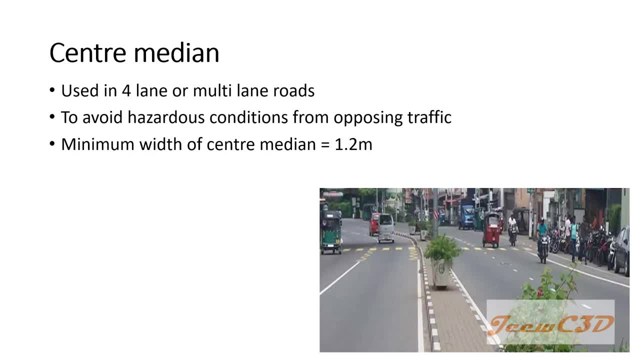 so it will avoid hazardous conditions from the opposing traffic. so if you are adopting this kind of centre medians, usually minimum width would be 1.2 meters. that means this total centre median width would be 1.2 meters. that means 0.6 meters to one side and 0.6 meters to the other side. 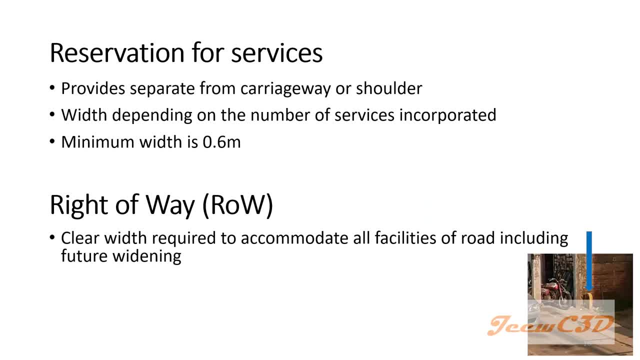 then you have reservation for services in your road, because in the roads you have after the road you have water board lines, electricity lines. sometimes nowadays you have telephone lines, fiber optical cables. so you have to have some free space just away from the road for these services. 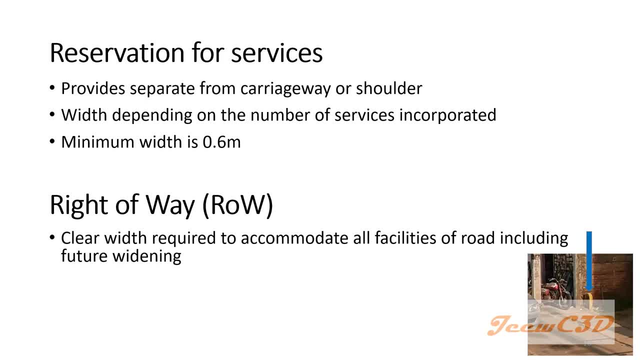 so we have to have reservation area for services, so we call it reservation for services. so if you are providing that kind of service area, the minimum width should be 0.6 meters. then you have something called right of way, that is, the area which belongs to the road. 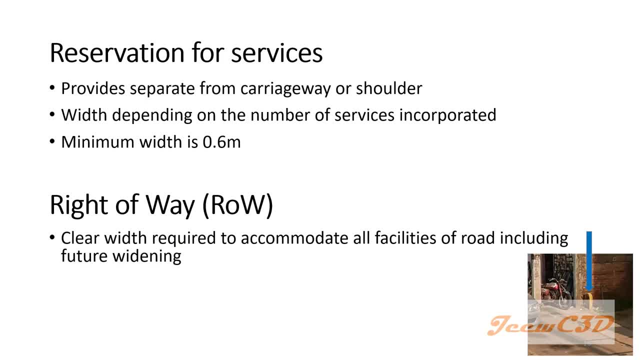 not the road edge but some area away from the road. we call them the right of way, so in the roads you might see this kind of boundary in the after some distance from the edge of the road. that is, these are called, after some distance, RDA boundaries. 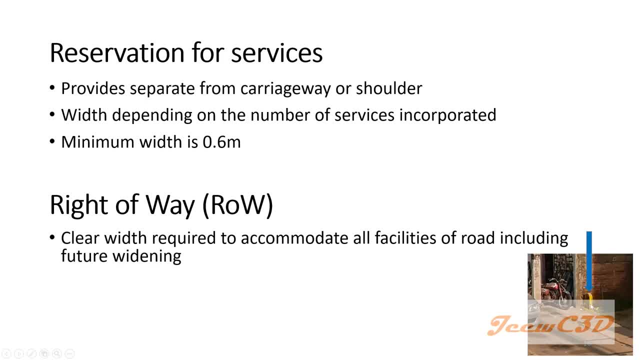 in this image. you can see here, these are RDA boundaries. that means up to this point, from the centre line of the road, up to this point, the area is owned by the road development authority. so the people can't do any construction. people can't do anything. 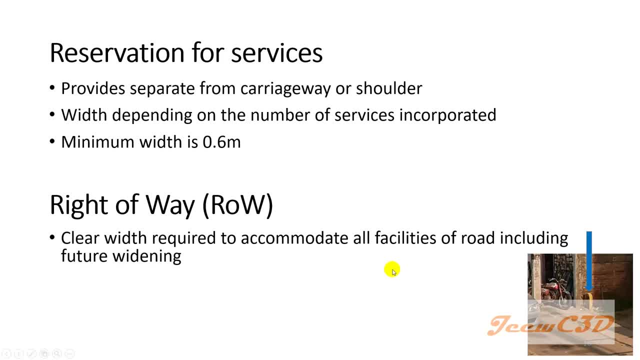 people can't build any permanent structure beyond, towards the road side of the RDA boundary. you see this building. this is inside the RDA boundary, so someday this person have to demolish this area so that it will be acquired by the road development authority. so this boundary will be marked on the road. 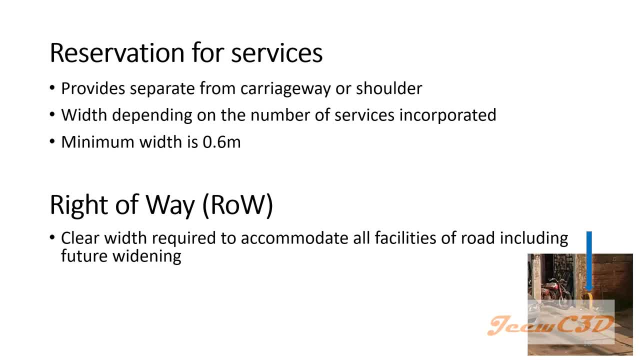 just after, just some distance from the road. so it will ensure that if there is a future widening of the road it can be done without problems to the neighboring houses or industrial people or business community anything. they will not be affected if you are constructing their houses or business or commercial buildings. 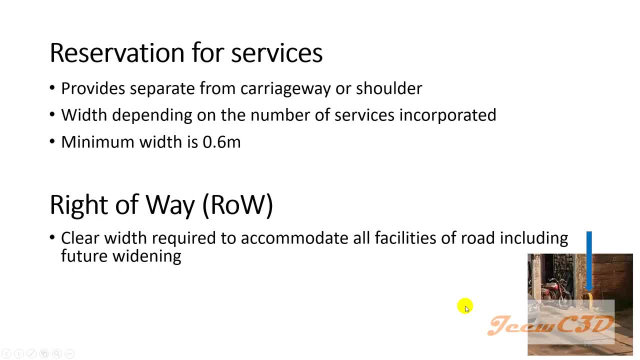 away from this RDA boundary, you can be called in the right of way. so that is about the cross section of the road. so in this series we have learnt what is highway geometric design and introduction about that. then we learnt about the function of the road. then we learnt about the basic design criteria. 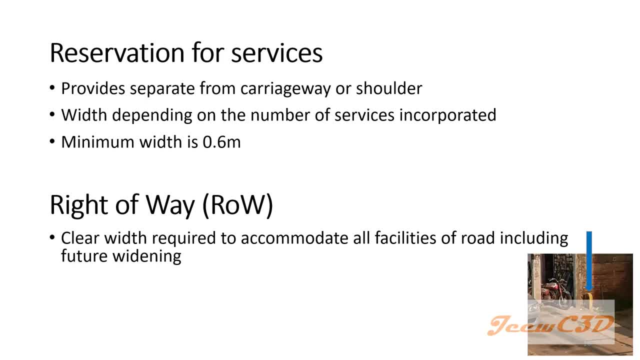 what are the factors affecting, what are the considerations for geometric design of roads? and finally, we talked about the cross section of the road. so under the cross section of the road, we learnt what are the components of a road. so what are the minimum values and what are the governing values? 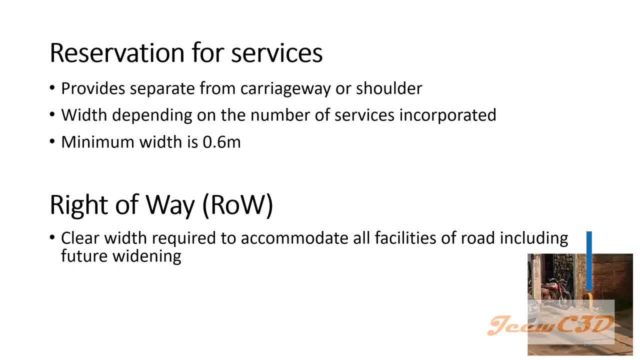 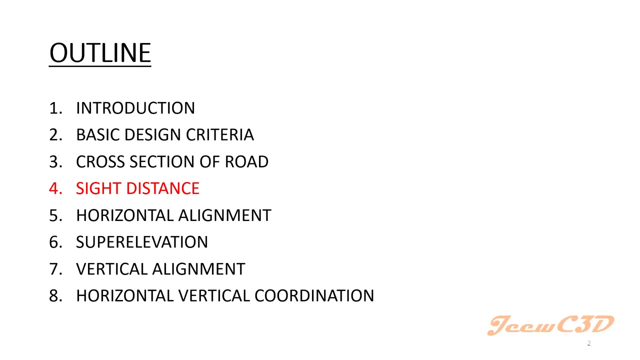 those things we learnt under the cross section of the road. so in this lecture what we have covered is those three parts. so in the next lecture we will be looking at the side distance, another important factor in designing roads. in this video we are going to look at 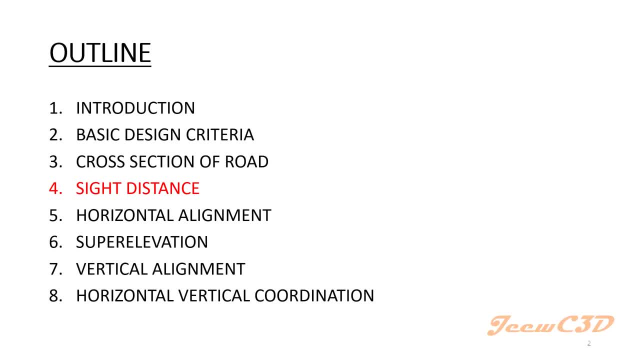 the side distance of roads. in the previous video we have got an introduction and we learnt about the basic design criteria and the cross section of the road. in this video, what we will be looking at is the side distance of the road. so what is side distance? side distance is. 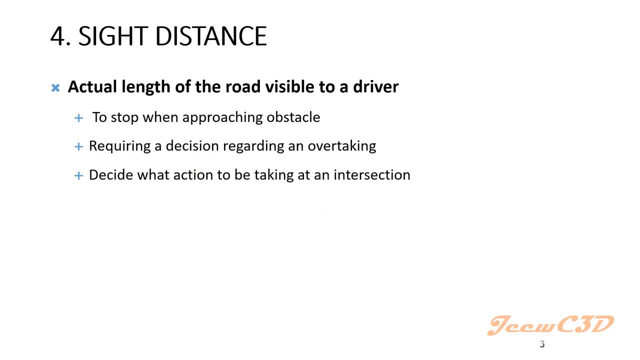 the actual length of the road visible to a driver. so if you are driving a vehicle on a road, you can see a head. so the length of the road, a head which you can see- is called side distance. but when I say the length of the road it should be along the road. 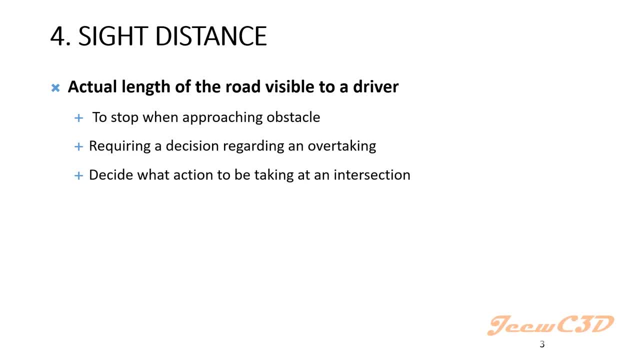 if it is a straight section of that road, the side distance is along that straight section. if it is a curved portion, the length should be measured along that curve. so the side distance is the actual length of the road visible to a driver. so why do we need side distance? 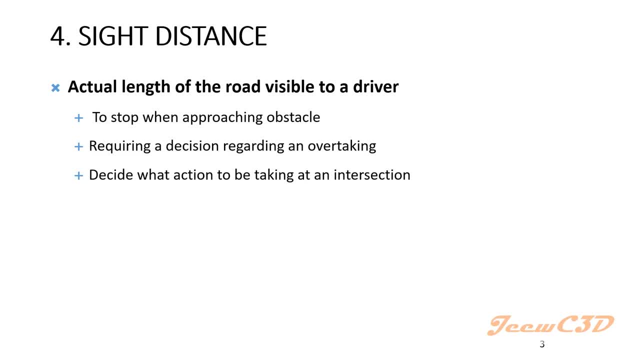 there are three locations, but there are many locations. mainly I have listed out three locations. so we need side distance to stop a vehicle when approaching an obstacle. so if you are driving, if you see some objectives on the road, so you have to stop the vehicle before hitting that object. 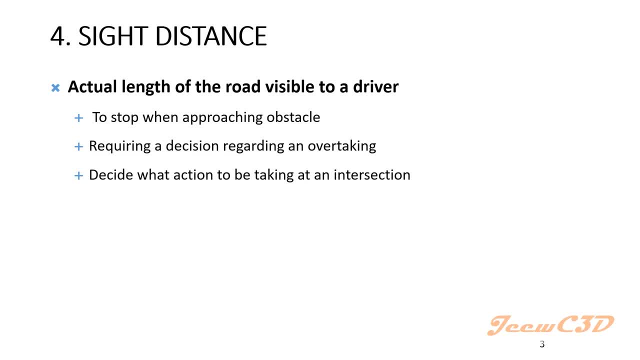 so we call it stopping a vehicle when approaching an obstacle. likewise, at an overtaking scenario, if you are going to overtake a vehicle, you need to see the road ahead so that it is clear to overtake safely. and again, we need side distance when we are coming to an intersection. 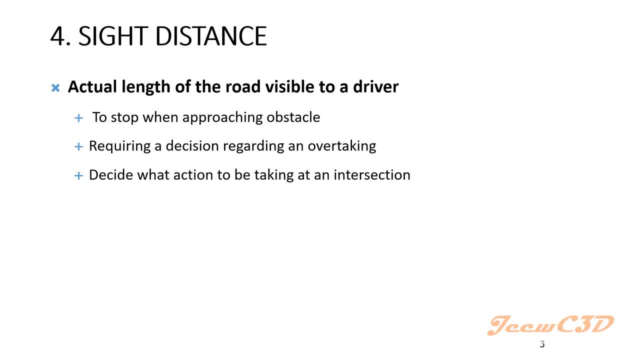 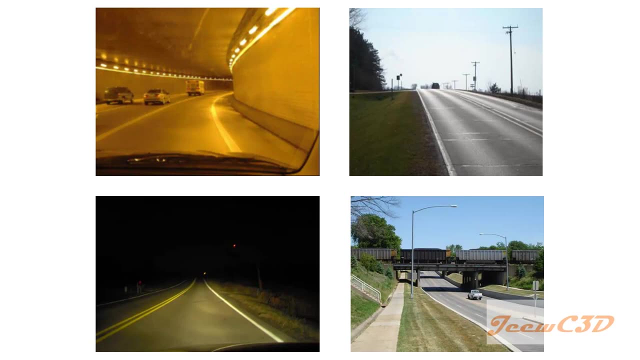 or a junction- whether to put your vehicle into the junction or stay until the junction is clear. so these are some scenarios. we need side distance. so here we have some images where side distance is important or constrained. so in the top left image you can see the side distance is somewhat blocked by this. 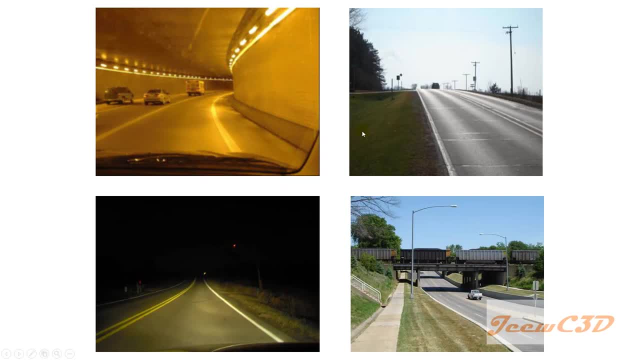 wall. in the second image you can see the side distance can be blocked by the gradient of this road if this vehicle is going further forward. this vehicle cannot be seen to this place. so the grade of the road affects the side distance here. this is a night time situation. 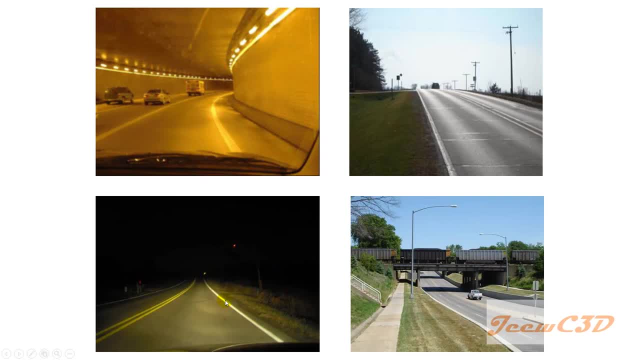 where, if the road is, even though this road is straight, you can see the road until the headlight goes up to some distance. we call it the headlight distance. you can see the road ahead up to the headlight. this can happen if there is no road light. 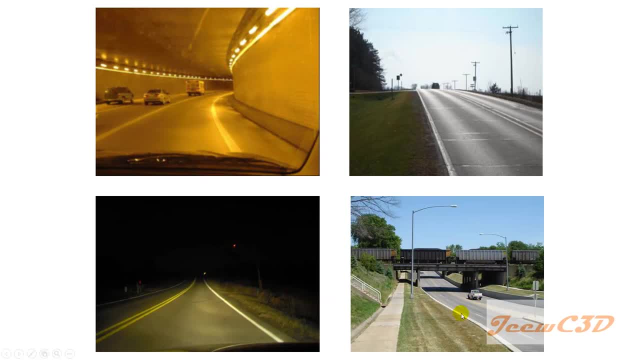 then in this fourth image you can see, the side distance is blocked by this wall bridge, this overhead bridge. so you can see the vehicle here, but if it is too far from this bridge, you cannot see it because of the bridge. so these are the things where you 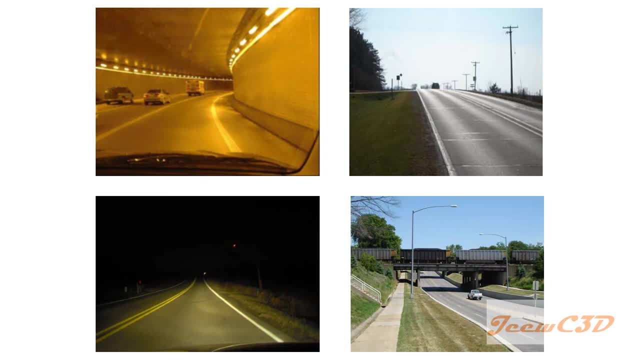 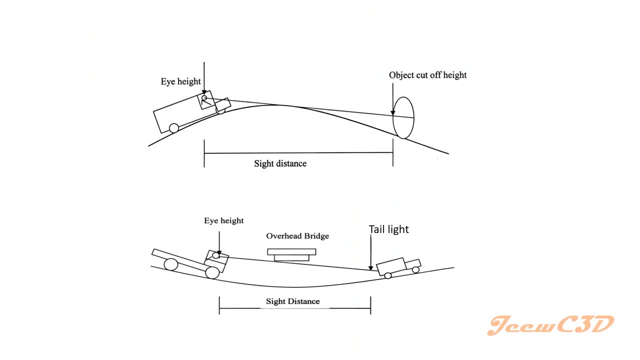 come across the side distance criteria. so in this image you can see how side distance is important. so you can see this is a curve. you call this a pressed curve. on a road the curve is like this. you call it a pressed curve so a driver is coming from this side. 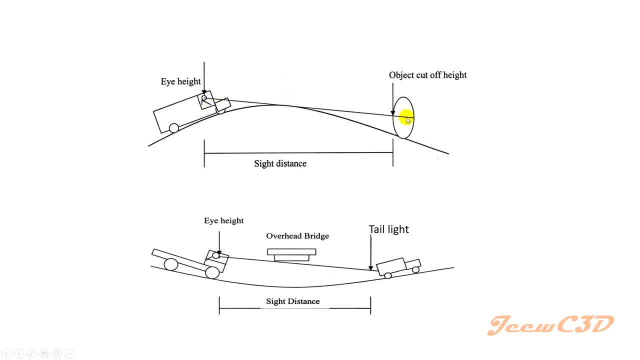 then he has a some object here on the other side of the road. so this is the line of sight you can see. so along the road we call the distance side distance. so to measure this line of sight you can see, so to measure this side distance, you have to calculate. 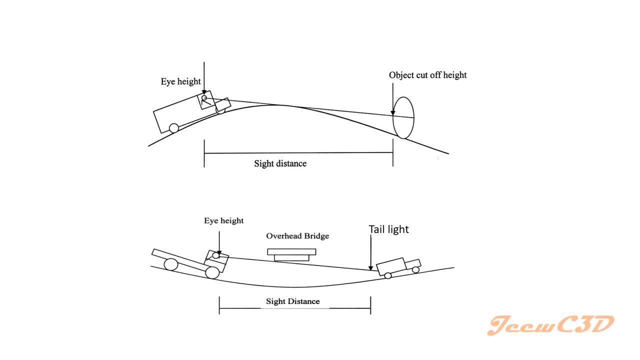 the side distance. so what are the factors affecting the side distance? by seeing this, this top image, you can see the driver height. eye height affect the side distance because if this is a car, the car driver sees less area because he is at a fairly lower elevation in the car. 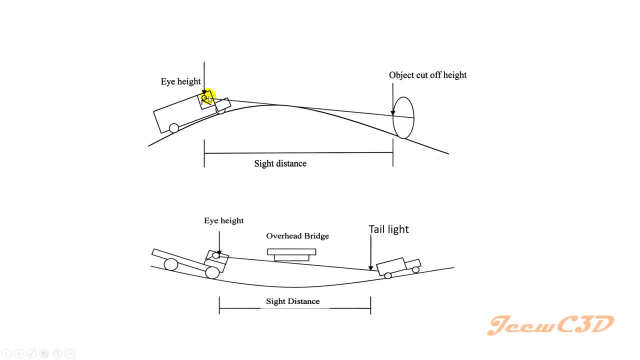 if this is a lorry or a bus or a a truck or a container, the driver is at a high position. he can see much of the length ahead because his eye is at a high position on the other side, this object, if it is a high object, 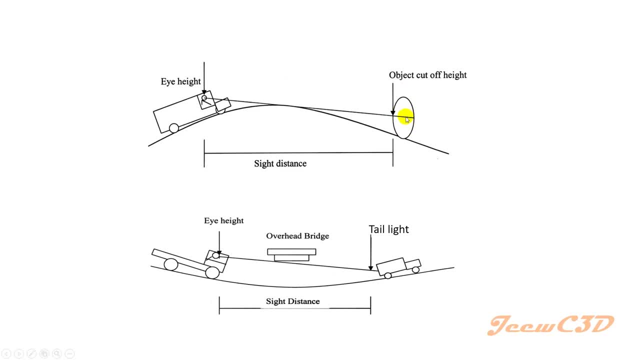 the driver will see it early. if it is a very small object, the driver will see it lately because this object is high, so the object cannot be seen within this line of sight. in the bottom image, same thing happens here. you have an overhead bridge, so the line of sight. 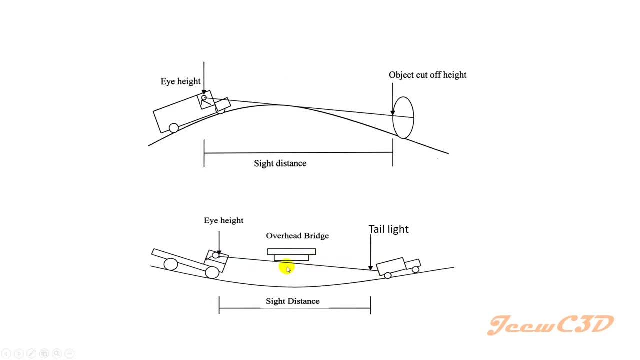 will be blocked by this bridge. so this overhead bridge height would affect the side distance. so if it is at a high elevation than this, the driver will imagine this. if this is a night time situation, the driver will see the tail light of the preceding vehicle. this driver is coming. 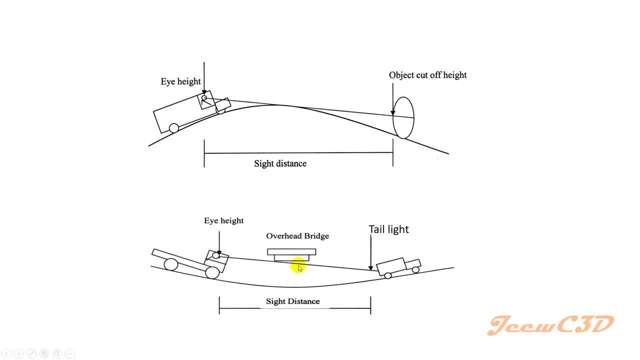 from here and another vehicle is going here, so this driver will see the tail light, the that side head light of the preceding vehicle. so the height of the tail light will affect the side distance. so if this is at a high position this driver will see it early. 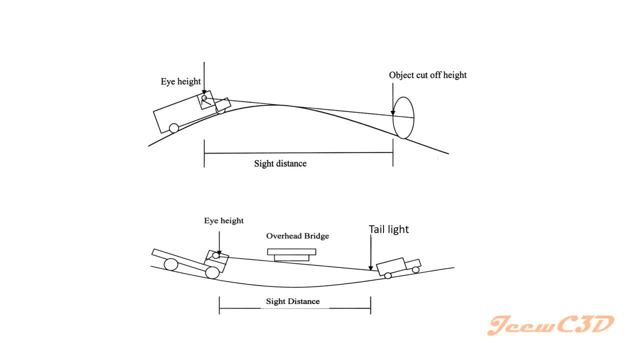 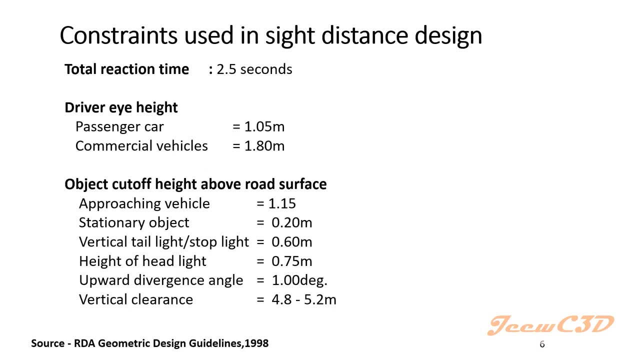 but if it is at a lower position sometimes he may not see. so that is the factors affecting the side distance. so here i have listed factors which affect the side distance design. that means the sri lankan standards. but if you consider other countries like usa or australia, 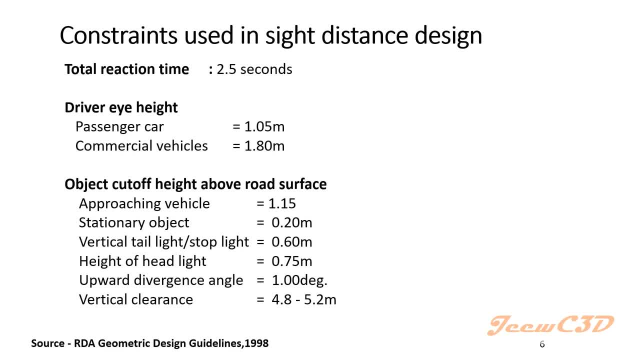 or england. they have their own values. some values are similar to these ones, some values are different from this one. so, according to the sri lankan standards, we have to set out these values, because we are mostly working in sri lanka. so here one. 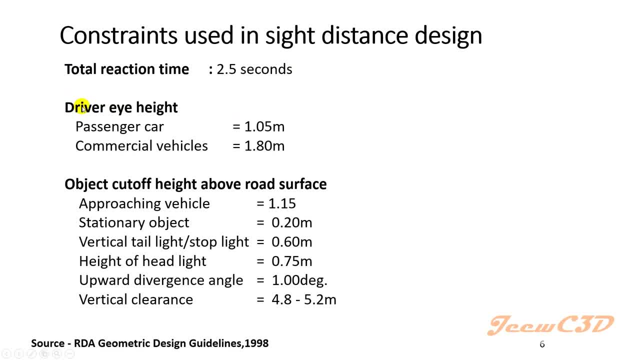 important thing. it is the total reaction time. i will tell you about this later. if the driver is in a passenger car, we will take the driver height as 1.05. if it is a commercial vehicle, like a lorry or a truck, we select the side. 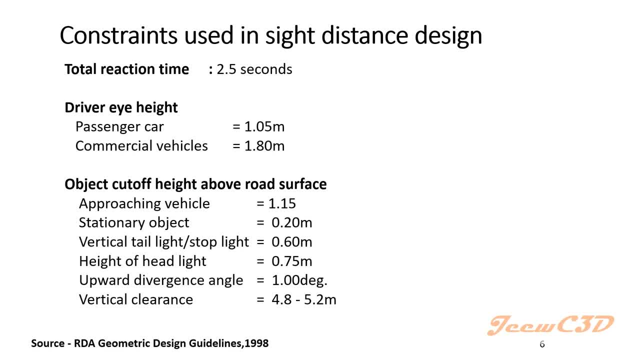 distance. it is not the driver, it is the other vehicle or the object. so if it is a approaching vehicle, it is approaching from the other side. we select the height as 1.15 meters. if it is a stationary object, that means that the vehicle is moving. 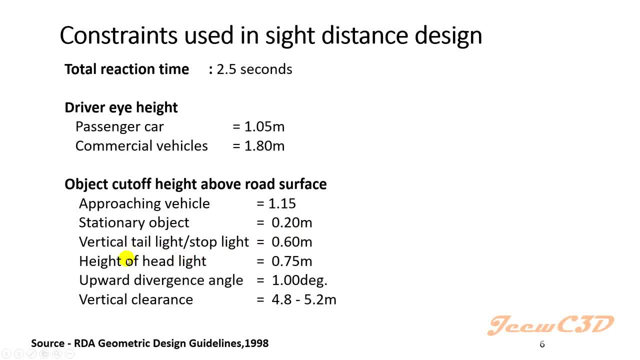 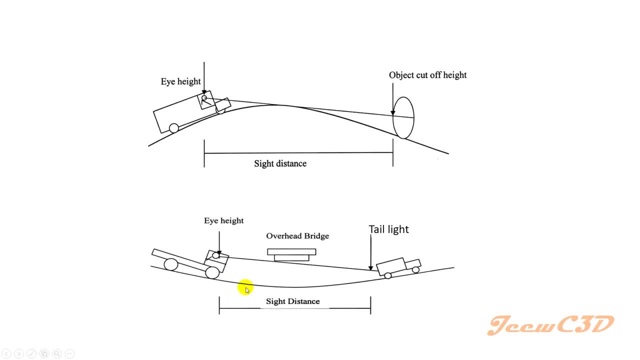 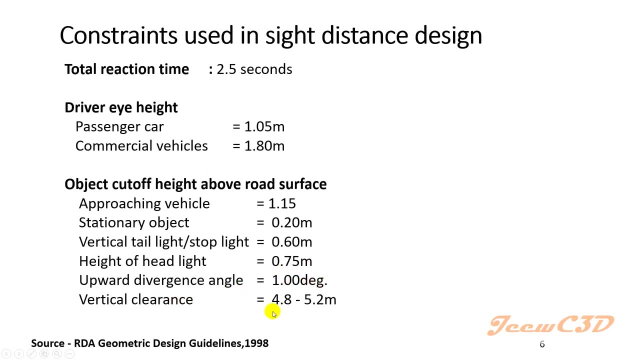 in the right direction. so if the vehicle is moving in the right direction, then the vehicle is moving in the right direction. so if the vehicle is moving for a certain angle, then you might choose the right direction. so as we looked at the road, that one has a 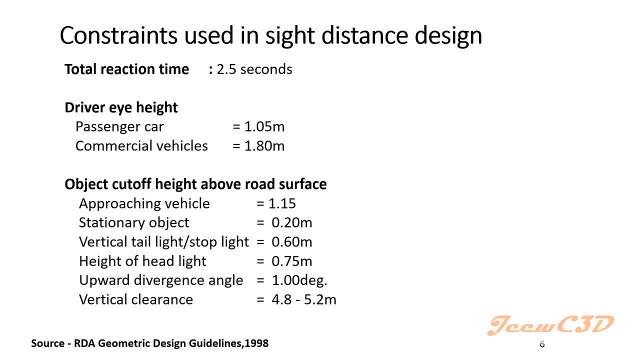 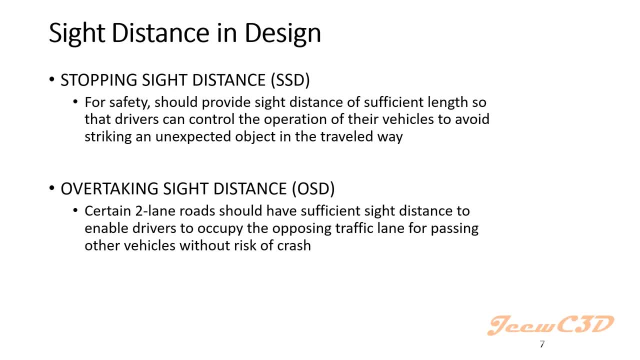 monthly distance from the. Then we will look at what are the types of sight distances we come across in sight distance design. There are four types. one is stopping sight distance. So, as the name implies, you know, stopping sight distance means when you are driving. 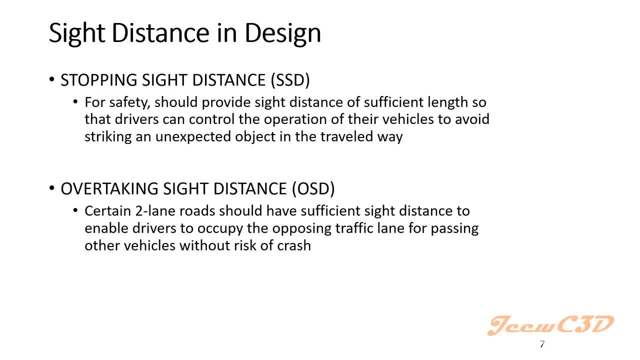 you come across an object or obstacle when you are driving, So you apply brakes in your vehicle, then the vehicle will be going to decelerate and stop just before hitting the object. So the distance travelled at that time we call it stopping sight distance. 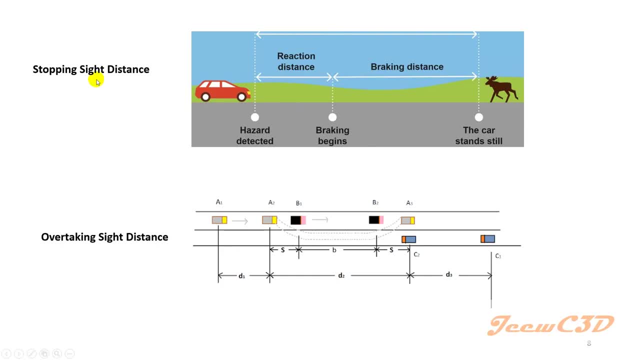 So in this example, a car is driving and an animal is here. So in this example, a car is driving and an animal is here. So this car driver detects that there is an animal in the road. So he decides. he detects that there is an animal, then he decides that he should brake and stop the vehicle. 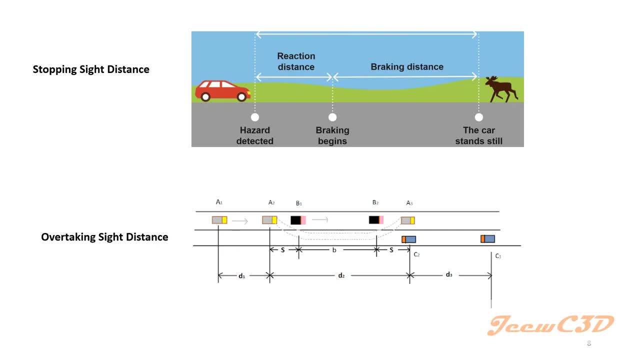 So once he is going to decide that thing, he will get some distance travelling until he is deciding. This reaction time is that Until he is deciding that he is going to brake, the vehicle travels some distance, Then he applies brake. So once he applies brake, the vehicle decelerates and stops just before hitting the animal. 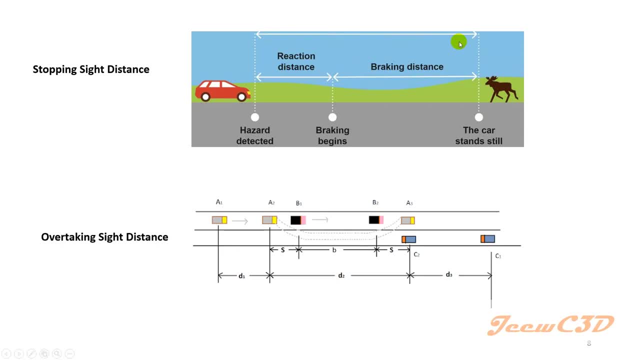 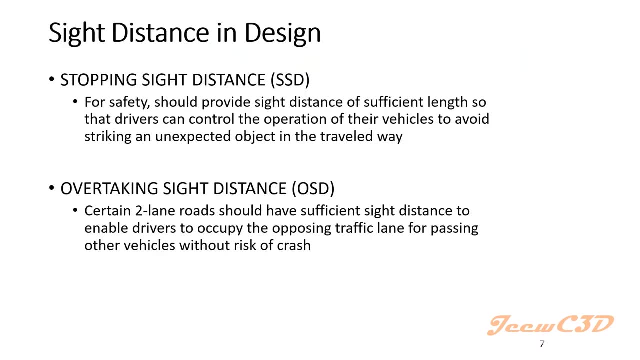 So this total distance, this total distance is called stopping sight distance. Then you have the overtaking sight distance. So if it is a two-lane road, if you have a vehicle going in front of you and the other side of the road, you will see there are no vehicles and there are dash lines on the centre line. 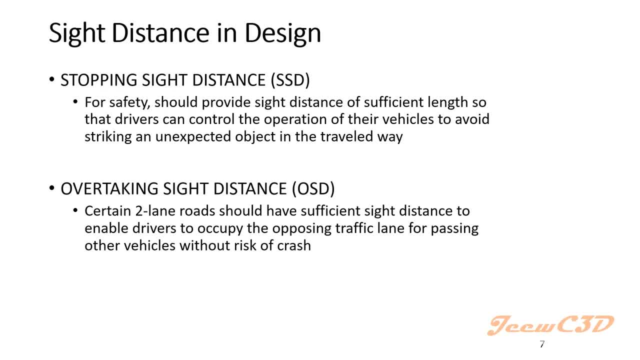 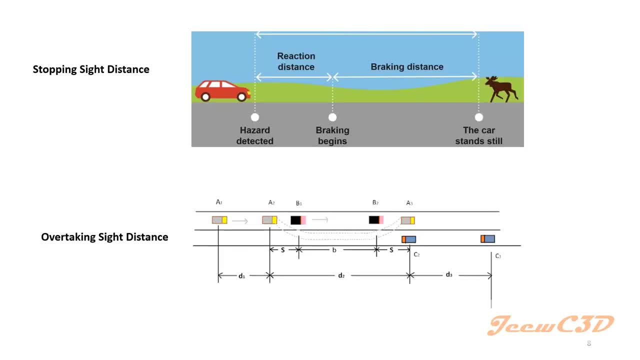 So you can overtake, So you decide to overtake that vehicle, Then we will see what happens there. Then we will see what happens there. Here you can see, you are on this vehicle and the other vehicle is travelling. So you see there is a vehicle coming from here, but you assume that you have enough distance to overtake. 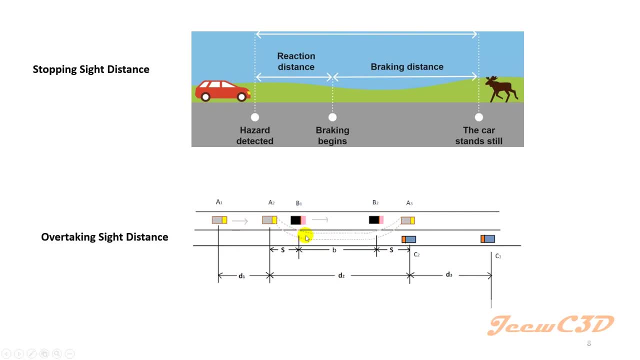 So you come here, you overtake and you come into the lane. So total distance travelled in this, this D1 plus D2 is called the overtaking. So total distance travelled in this, this D2 plus D2 is called the overtaking sight distance. 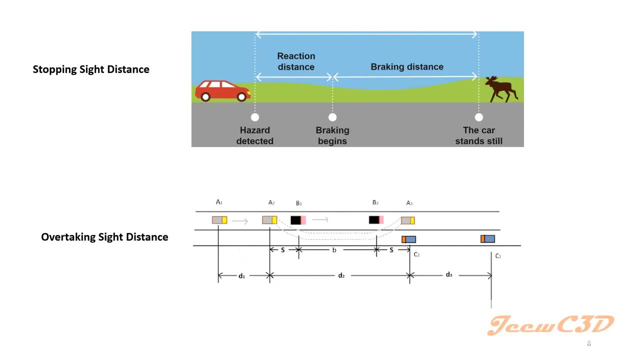 So in overtaking sight distance you will be travelling on one lane and you put your vehicle to the other lane and overtake the vehicle in front of you and you come back to your original lane. So distance travelled at that time is called the overtaking sight distance. 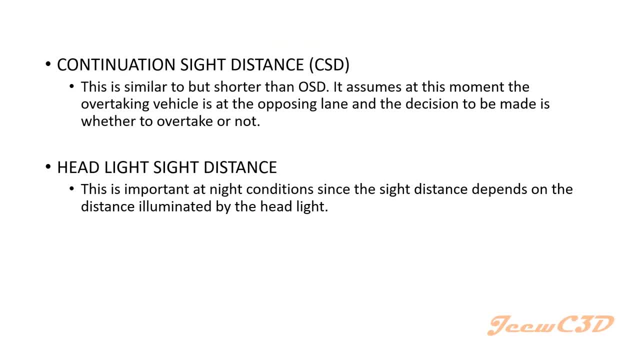 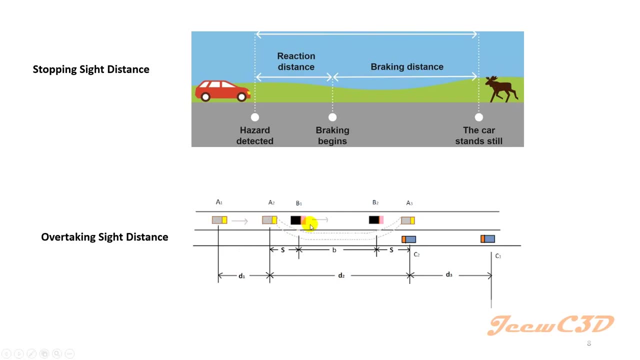 Then you have something called continuation, Then you have something called continuation, Continuation, sight distance. It is a part of overtaking sight distance. So if you see this example, sometimes when you are going to overtake this vehicle, you put your vehicle into this position, just parallel to this position. 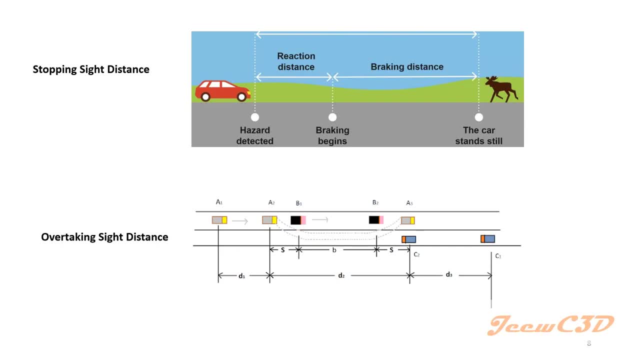 Then you see ahead of the other lane and you decide whether to overtake or not to overtake because, depending on the situation of the other lane- Let us say you are in this position, then this vehicle is somewhere here. You think before hitting this vehicle or before facing an accident with this vehicle you can overtake. 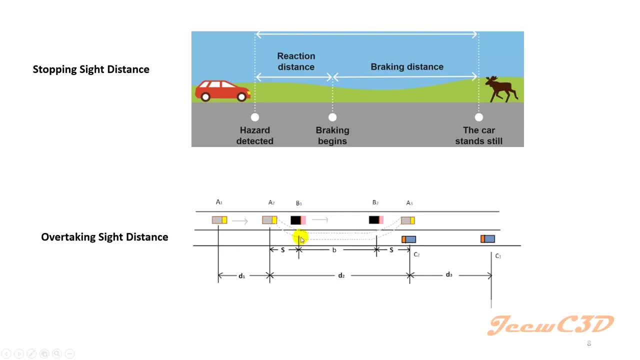 So you overtake. So the distance travelled in this time period is called the continuation sight distance. So in continuation sight distance, what the difference is? you are at this position, you are at the other lane and you put your vehicle to the other lane and decide whether to overtake or not. 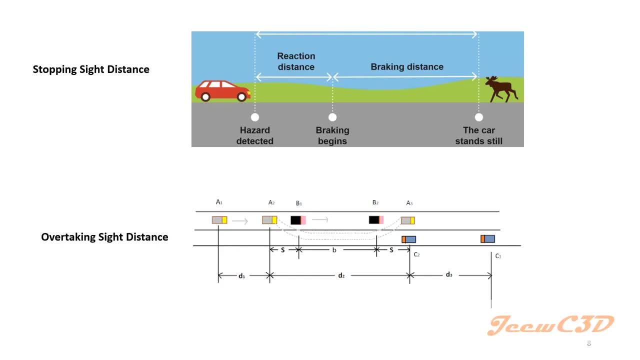 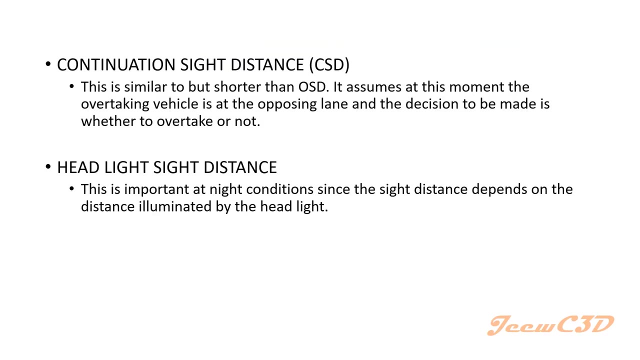 If you are going, if you overtake that vehicle, the distance is called the continuation sight distance. If you think that the sight distance is not enough, so you will come back to your normal lane again without overtaking, Then the headlight sight distance means the length of the headlight which can be seen at the night time condition. 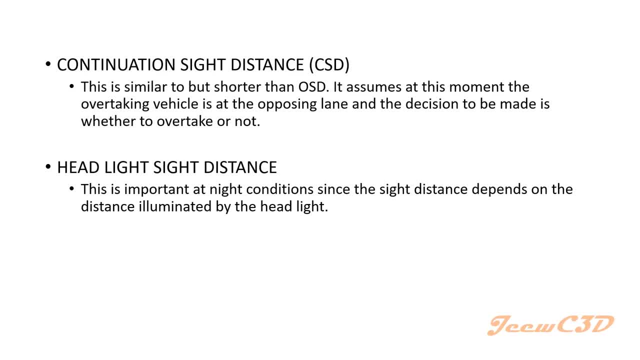 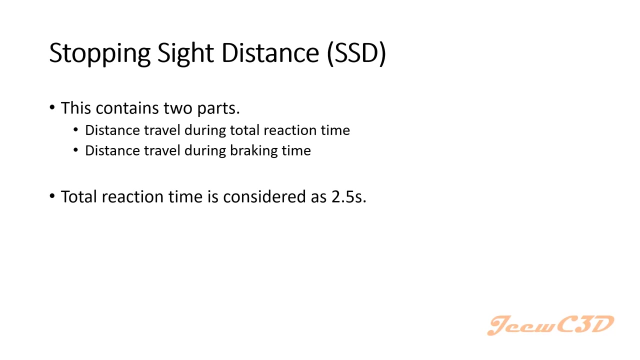 Usually we take this headlight sight distance as similar to the stopping sight distance. So as you take the stopping sight distance- Stopping sight distance equal to the headlight sight distance after headlight sight distance criteria situation- Then we are going to talk about stopping sight distance. 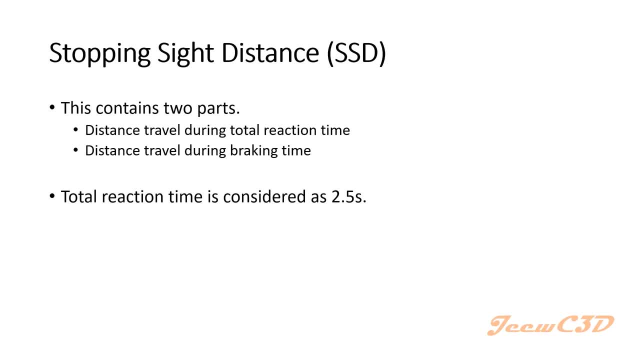 This stopping sight distance has two parts. I told you before, when the driver sees an object Before he is going to brake he will think whether what is going to happen. So if he thinks he is going to hitting the object, he started to brake. 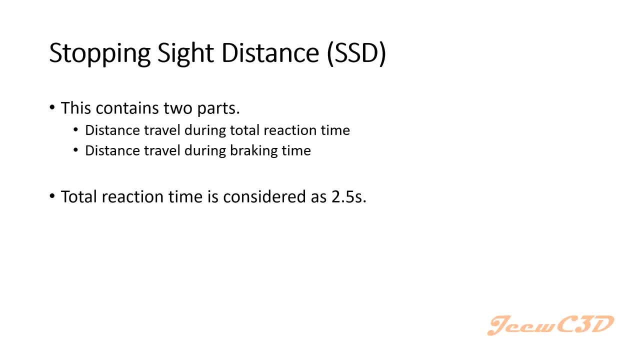 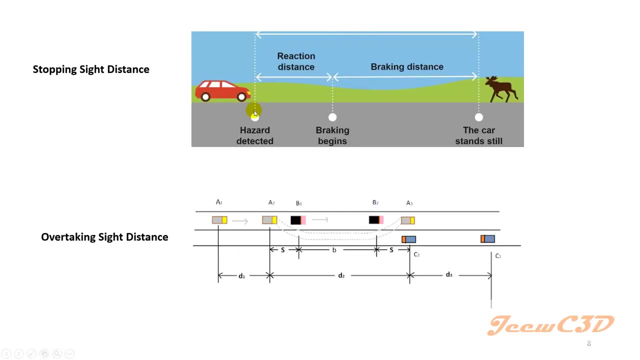 So when he is thinking he is travelling some distance in his speed, So we call it the reaction time. If I move back to this slide, In this location the driver thinks he has to apply brake. So before pressing the brakes he will cover some distance. 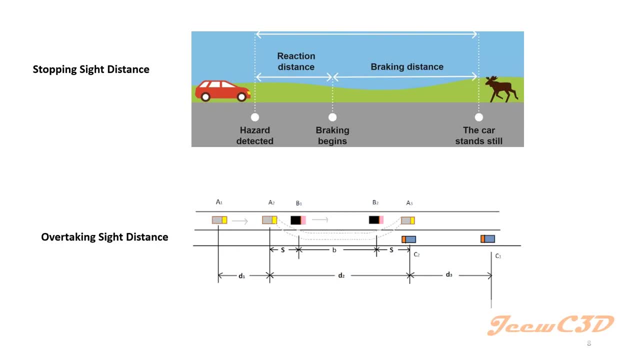 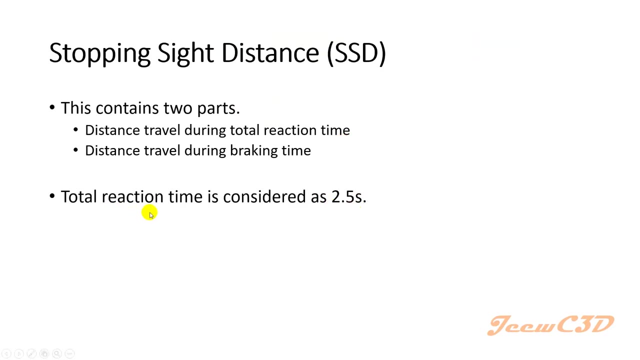 So the time interval between detection of the hazard and applied braking is considered as 2.5 seconds. So we call it the reaction time. So it is taken as 2.5 seconds. But this 2.5 seconds is not for all drivers. 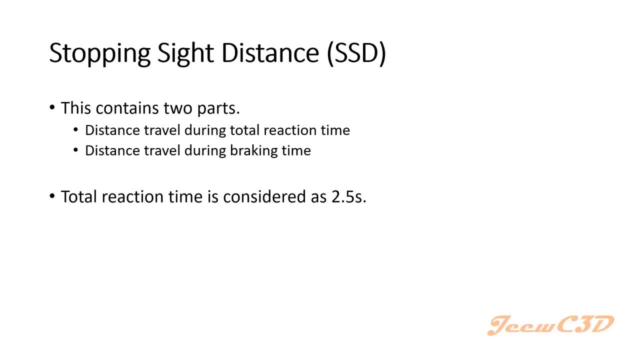 If you are a very quick driver, it will be less than 1 second. So if you are a very old driver or a non-experienced driver, you may take some time. So by research, the people have identified a general value which is 2.5 seconds. 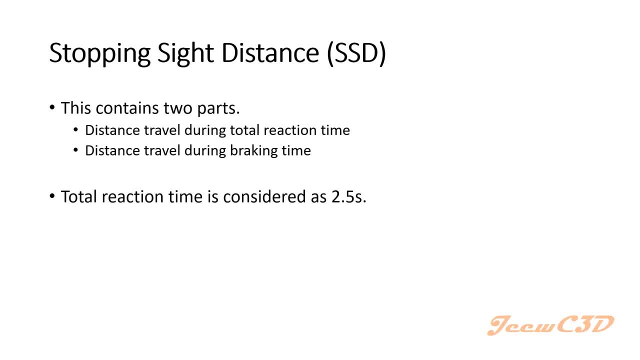 So it is 2.5 seconds for reaction time to cover up all the situations. Then after braking, the vehicle will be stopped. So after braking the vehicle will cover some time, some distance and stops. So there are two parts, as I told you earlier. 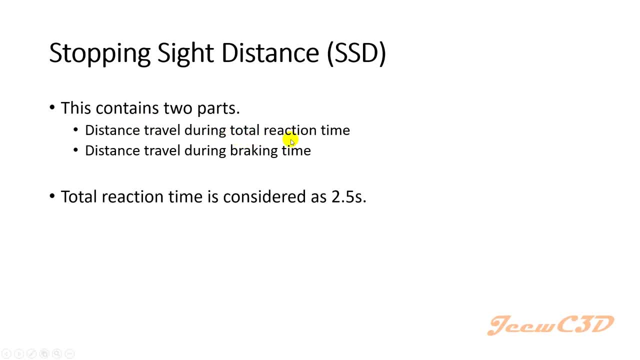 The distance covered during the reaction time before applying the brake. After applying the brake, the distance is 2.5 seconds. the vehicle will cover some more distance and stop the collection of the planes in these situations are for the stopping side distance. so this is the equation for stopping side distance. 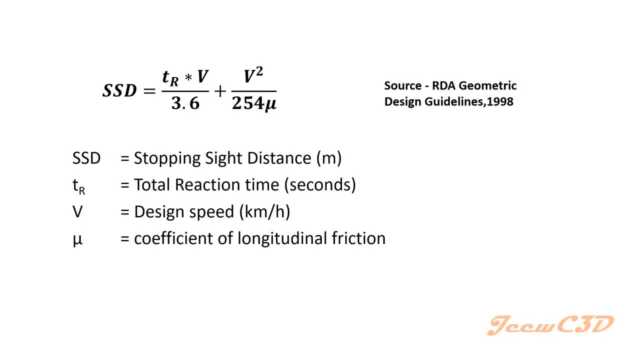 which is listed in rba unit design guidelines. this equation is same for most of the other guidelines, also astro and also they have the same equation. actually, what rba has done is look at the equation from those guidelines. the stopping side distance, ossb, is equal to. 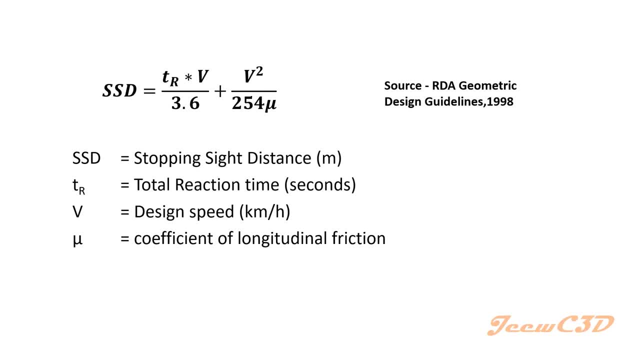 into v over 3.6 plus p, square over two hundred and fifty four new. so v, tr is the part of reaction time, which is 2.5 seconds, as i told you earlier. v is the design speed, which is the design speed of road, and now is the provision of longitudinal friction. Longitudinal friction means friction. 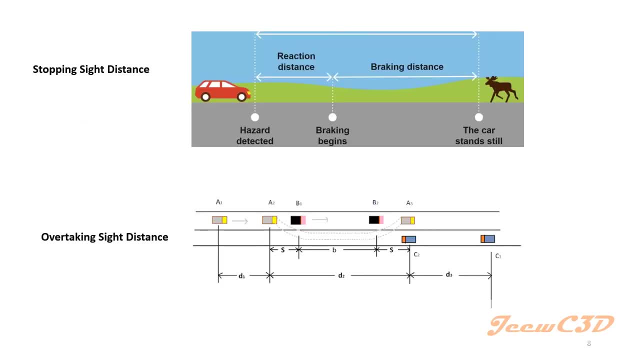 along the road. Once you apply the brake, the friction will act. the friction on this surface will act on this vehicle along this line. So longitudinal friction means the friction along this road surface, The friction along the road surface which another vehicle is travelling, because there is another friction part which we will be learning under horizontally. 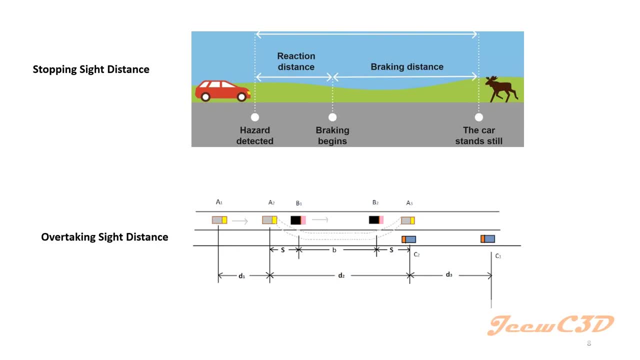 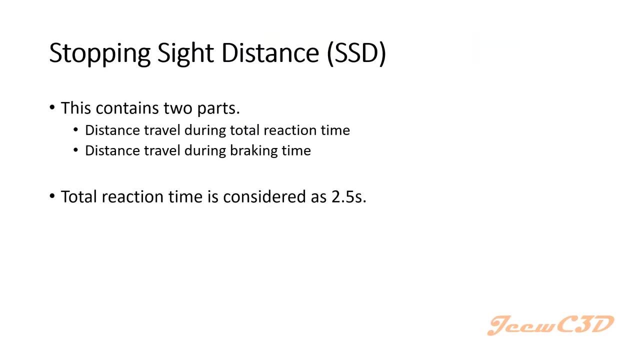 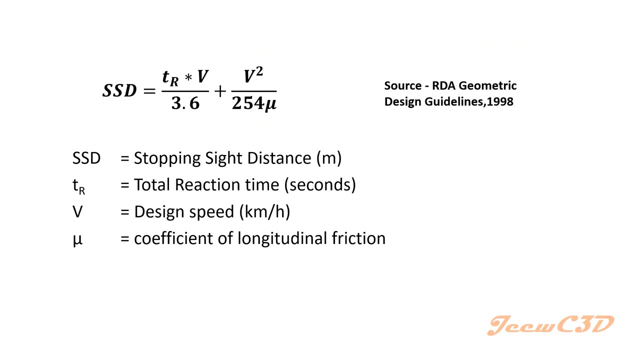 alignment. So this friction component is applying on the vehicle along the travelling direction, So we call it longitudinal friction in a section. So AR, we know that is 2.5. usual V is the design speed. we will be knowing that also when we are designing a road. MV is the one we don't know, So it is given. 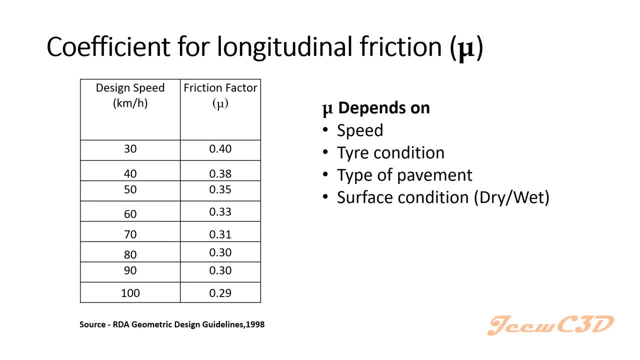 in all the design guidelines according to the design speed. According to design speed, LF-C will be change from higher value to lower value. If the design speed is lower, friction factor is high. If the design speed is higher, friction factor is low And the 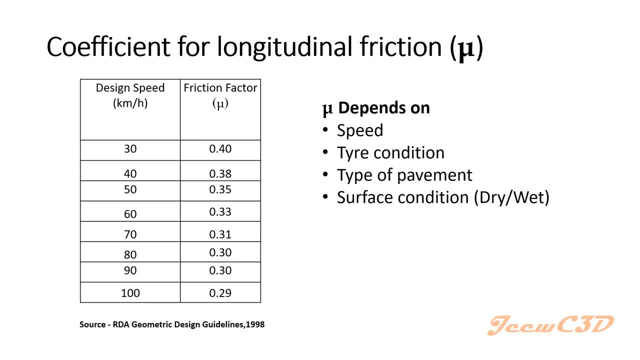 friction factor, or mu, depends on several conditions, that is, the speed of the road, as we see in this table, and tyre condition, type of pavement and the surface condition. if it is, if the tyres are new, you will be having a good friction with the pavement over the road surface. this 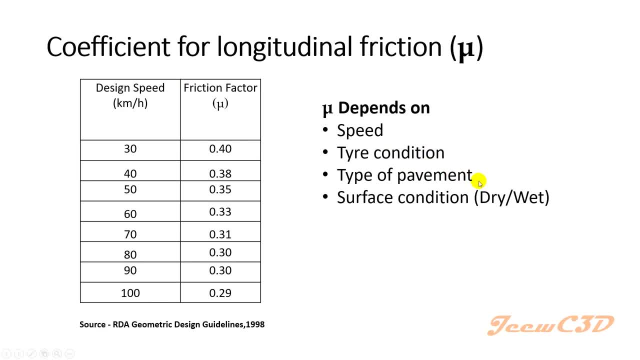 pavement means the road surface. if the road surface is a good road, good new road surface, the friction will be higher. so actually not only good, but it should be a good quality pavement. so you will be learning these things in highway construction management. so if the pavement material and the material mixture is better, it will provide, it will give you better friction. so 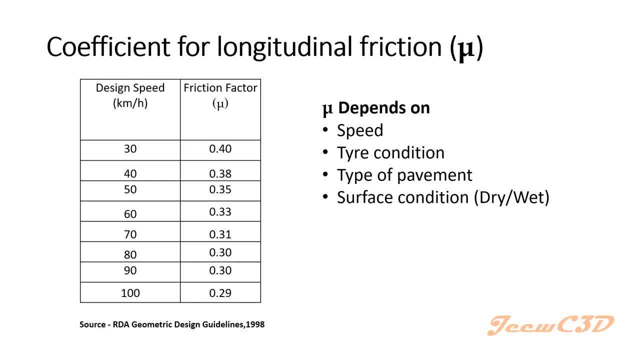 it. then factor will be depending on type of the payment, then the surface condition, whether it is by over. if the surface condition is over, the whole surface is good. you will have some kind of lesser friction value. but these values are taken to address all the factors to some extent and so these values have some kind of safety margin also. 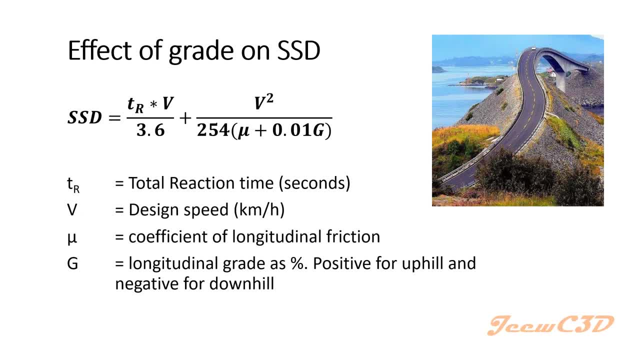 throughout the use, such as drink, which is also one of the key values they discuss there. then the previous situation for stopping site distance is for a flat ground. that means the road is flat for that equation, but generally we find, of course, a broad ground. that means the road have slopes, like here. this road is coming along a 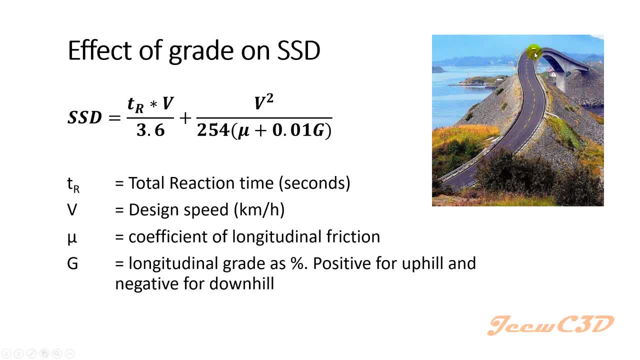 vehicle is going this way. it is going upward, it is coming to the this coming to this direction. it will be coming downward, so we can modify the equation according to the grade of the road. so what will happen is you have the same equation here and this is the. 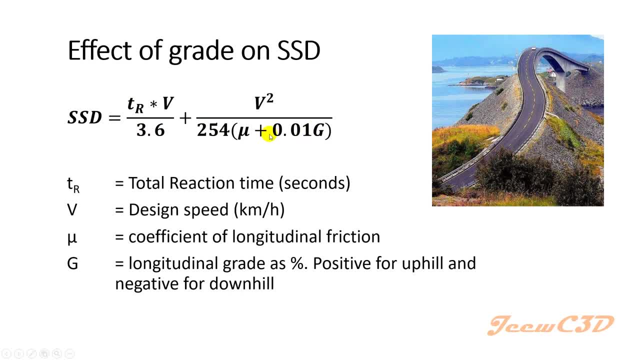 uh modification part. so instead of mu you will be having mu plus c. 0.01 g. g is uh given as a percentage. so if the road has a 10 slope you call it 0.1. 10 into 0.01, that is. 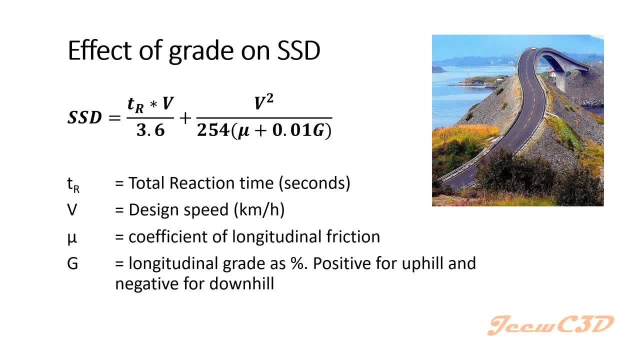 so 10 into 0.01, that means 1 here. so likewise you have to calculate the grade and check the stopping side distance. so if this g value is a positive one, you call it uphill. so if the vehicle is traveling in this direction, so you have a. 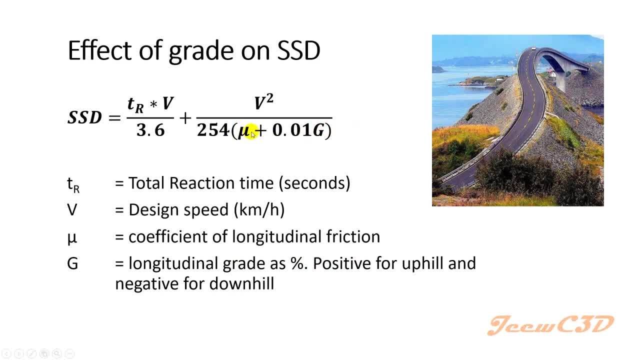 positive grade. so if this is positive preface- and this is already possible- this bottom one will be higher. so this part will be lower. so you will be having a lower stop inside. if it is coming downwards, this have become a minus 1 because it is negative for downhill. so 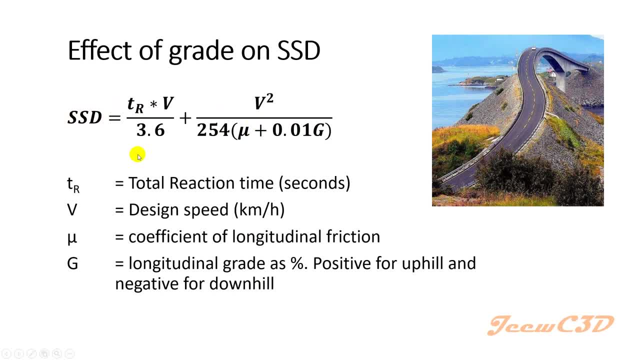 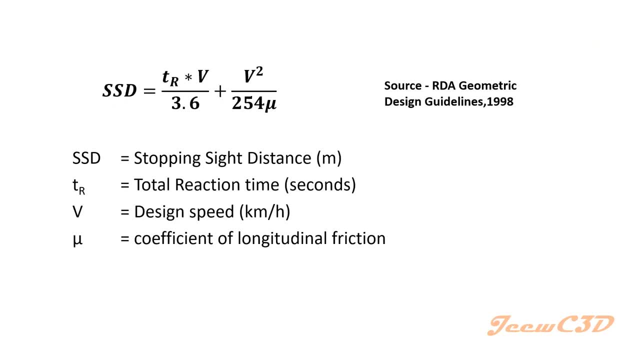 in high side, stepping side distance. then one more thing i have to tell you: in this equation, this part represent the breaking this. this part represent the length you traveled until you get the decision. that means the length you travel and at the total reaction time, and this is the length you travel at the breaking distance. so this is the collection of distance to get the. 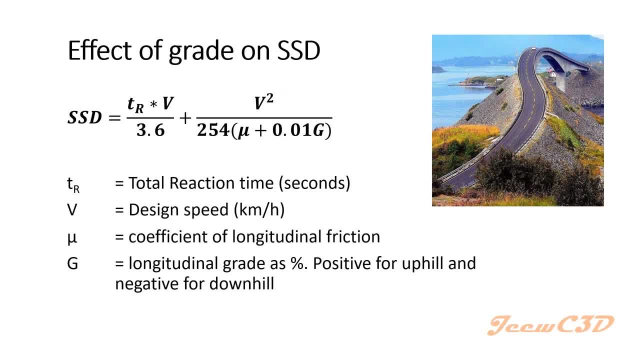 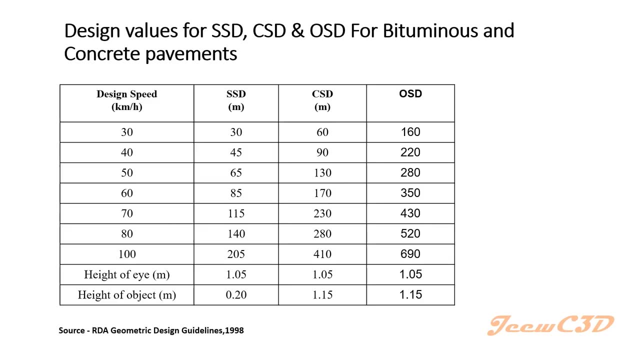 stepping side distance. so here also you have the same. this is the length of the road until you get the decision. once you apply break, you will get this length. so that is about the stepping side distance. then these are some general values for stopping side distance listed in RDA geometry design guidelines. if the stopping side this the 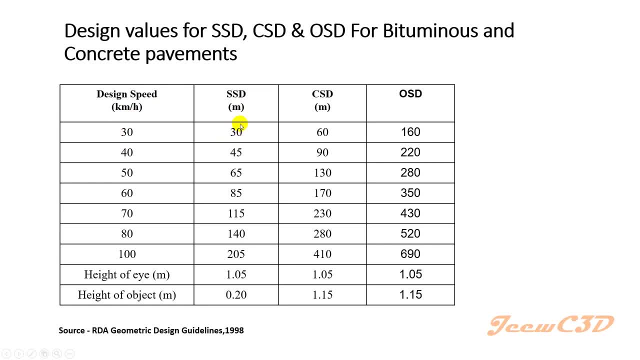 design is to be 30. you can see the stopping side distance is around 30 and continuation side distance is 60 and overtaking side distance is 160. you can see this overtaking side distance is very than these two. so here also, if you put the this design, speed value and new value into that equation, 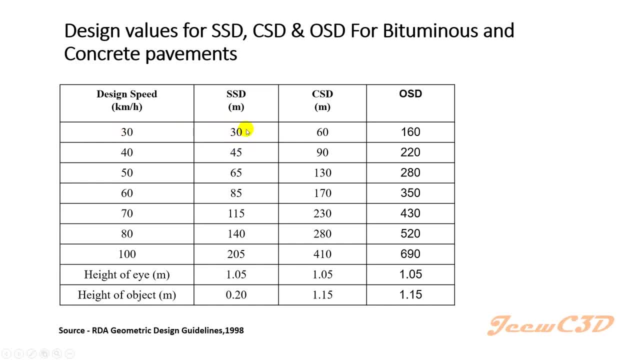 you will get this well, so you will get something like 29 point something. so you have rounded up to 30. that is what. that is what we are getting. that is why we are getting 30 as stopping side distance. then you can see this design speed of 40 you have, stcd is stopping side distance is 45 and 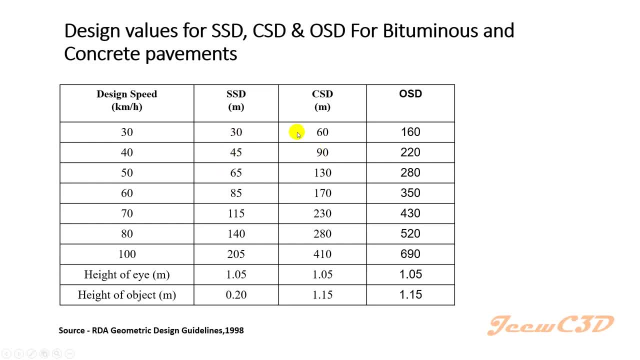 continuation side distance is 90.. if you see these two, you can see stopping side distance is half of the continuation side distance. otherwise, in other words, continuation side distance is equal to twice of stopping side distance. so these are the uh object values we have selected to calculate the stopping side distance and other side distance. 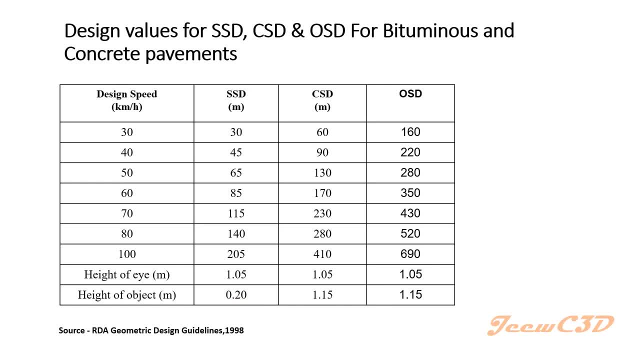 actually we are not designing for overtaking side distance. we are not considering overtaking side distance. if we are going to consider overtaking side distance, we have to put the values to these design values over speed values and put these parameters into a module and calculate the overtaking side. 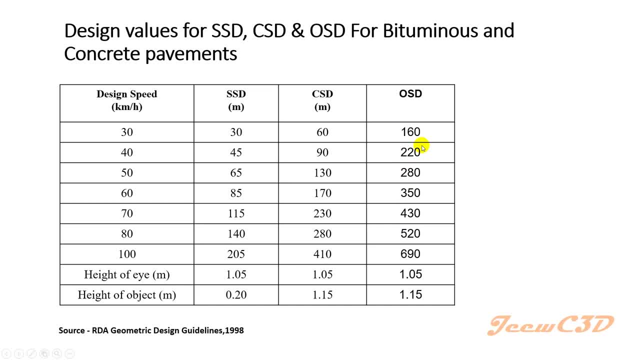 distances. but since these values are very high, we are not going to adopt these values in our design. it will make our design very uneconomical. instead, what we do is we are doing designs for SSB or stopping side distance or, if the conditions prevail, if you can have. 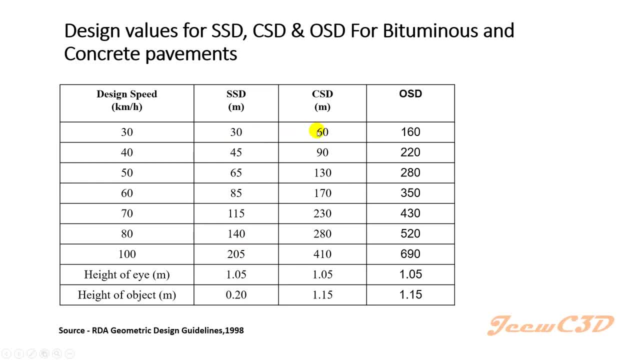 more side distance than 30, so we will be giving the continuation side distance. so in this stage sometimes you may not understand what we discuss as stopping side distance and appearing like this into a road, because still you don't know where you apply the stopping side distance in the 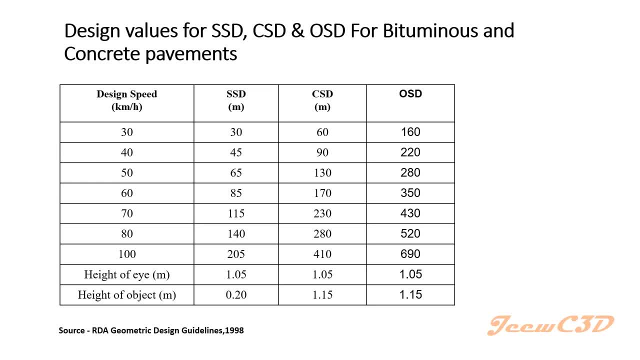 road. So you will be learning it under vertical alignment. You will understand this thing very clearly at the vertical alignment section. But in this section what we are discussing is what is the length of stopping side distance, So continuation side distance at each design speed, and what are the parameters affecting? 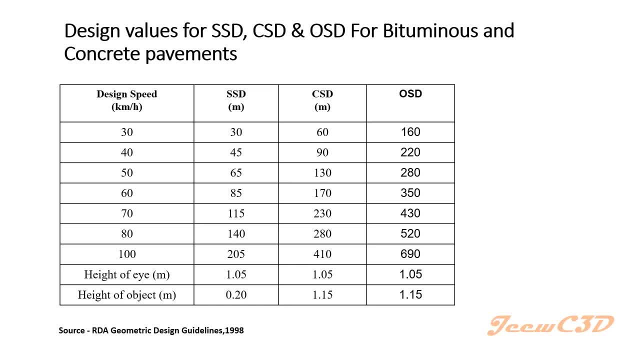 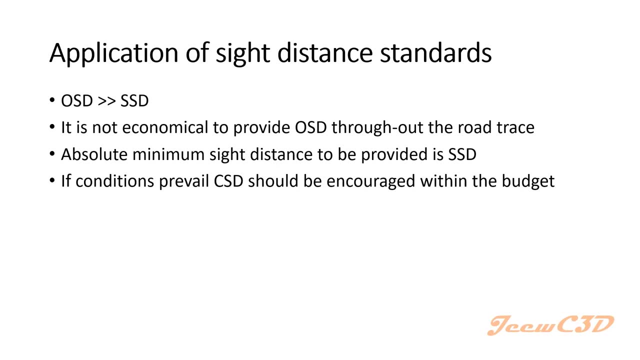 the design speed. So, as I told you earlier, we are not taking overtaking side distance into account when designing roads. So the application of side distance standards- as I told you earlier, overtaking side distance is very much clear. So it is not economically to provide overtaking side distance throughout the road place. 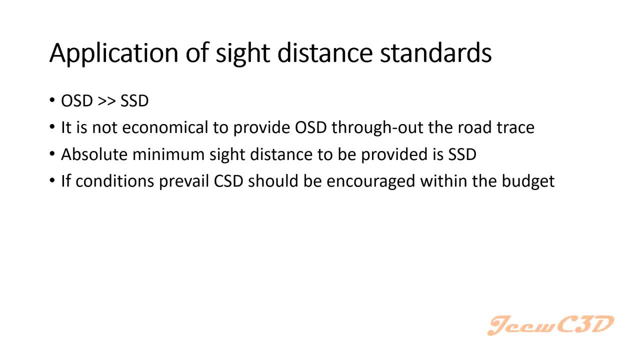 If you can provide it easily, you will. you can provide it, but you are not required to adhere to overtaking side distance everywhere. So instead of that, you can use absolute minimum side distance, which is a minimum stopping side distance. 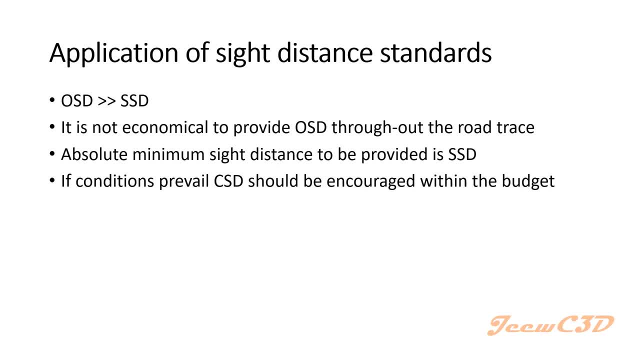 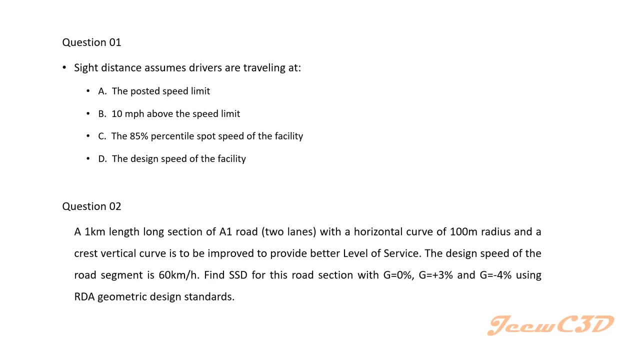 If you have a chance to adopt continuation side distance, you have to use that continuation side distance in the design instead of stopping side distance, without going too much into the budget. Here you have two questions. First one: the side distance assumes drivers are travelling at proposed total speed limit. 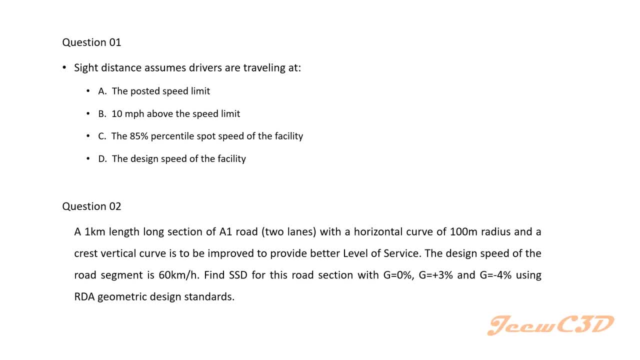 10 miles about speed limit or 10 kilometers about speed limit, then the 85th percentile spot speed of the facility and the final answer is the design speed of the facility. So if you discuss these four answers, you can, you can see very clearly that all the 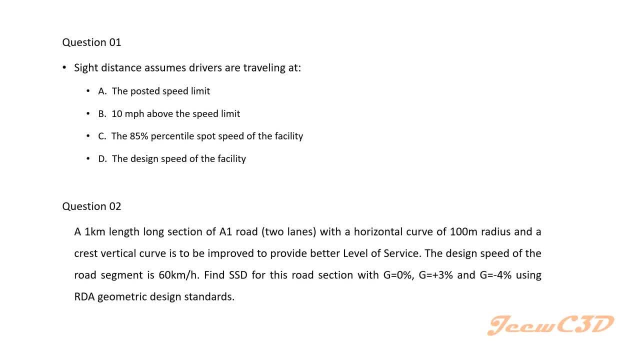 questions are related to design speed of the facility. So the answer would be design speed of the facility. Then we have a second question. In that question we have to calculate stopping side distance under three grade in the road. So your road grade will be flat grade. OG equals zero and three percent upward gradient. 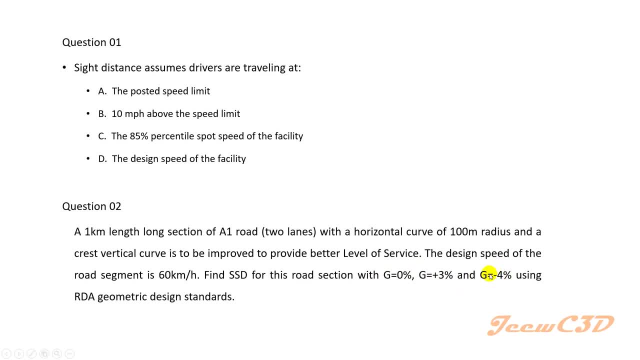 and four percent forward gradient, For minus four percent or four percent downward gradient. you have to do this calculation by yourself. I will be discussing it in a later time. So that is about stopping side distance and side distance. So in this video we have learned that is stopping side distance and side distance. 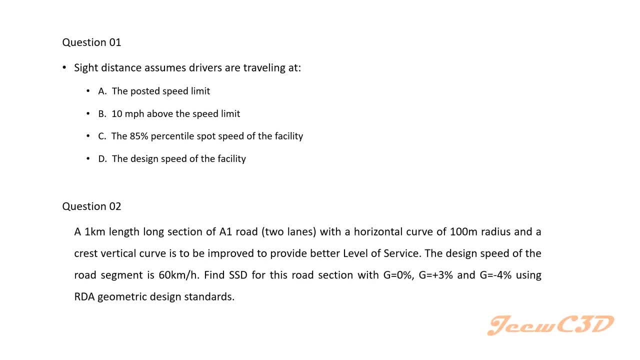 What are the constraints, What are the parameters we consider in side distance, What type of side distance we have And what are the equations? What is the equation to calculate side distance? And finally, we talked about the application of side distance in road design. 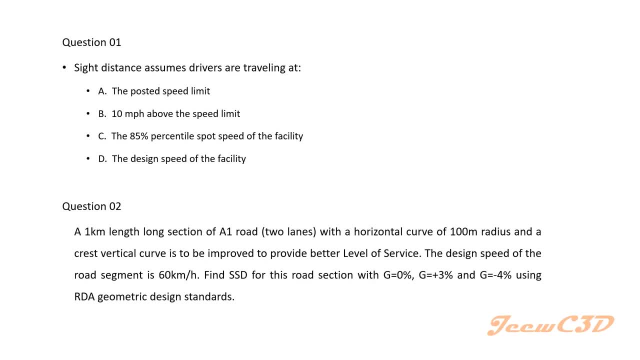 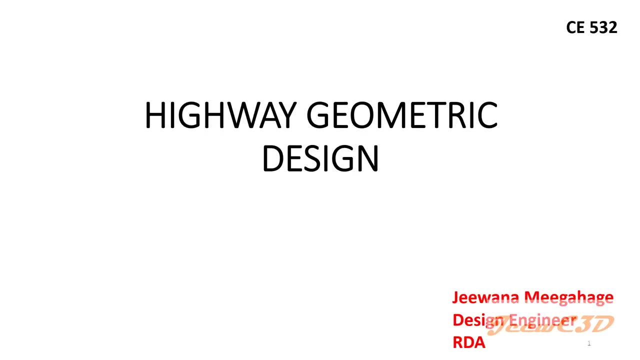 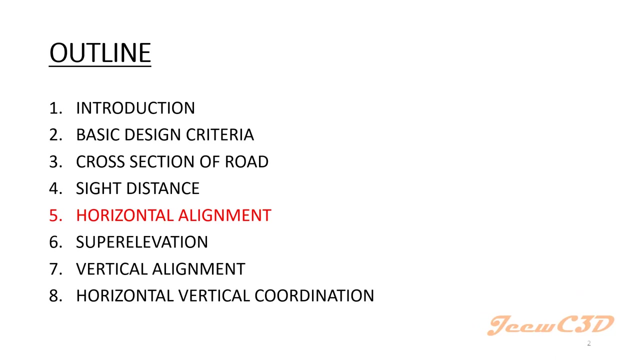 So that is about side distance. In the next section we will be looking at horizontal alignment. horizontal alignment, vertical alignment And this is called the side-line relationship of the road. so far we have learned up to site distance section. we got an. 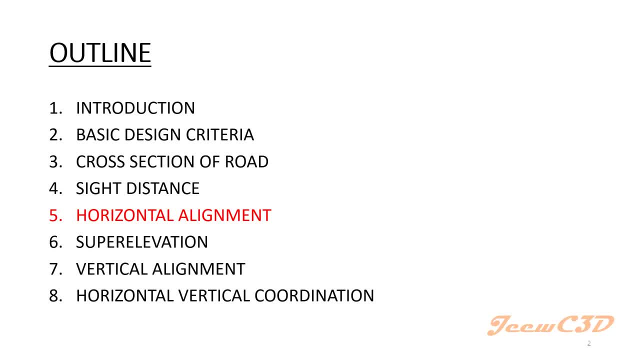 introduction to road design. then we learned about the basic design criteria and then the perception of the road and finally the site distance criteria when designing roads. in this section, what we are going to do is look at the horizontal alignment of the road. so what is horizontal alignment? horizontal- 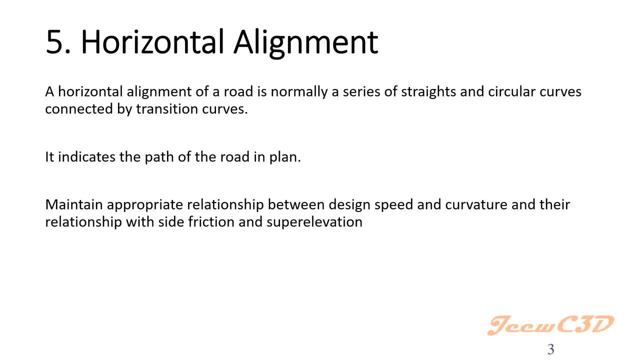 alignment means the plan beam of the road. so if you go to the sky and see the roads below, you can see only straights and curves on the road, so you cannot see any elevation of these roads. you'll only see this: straight sections and curves section. 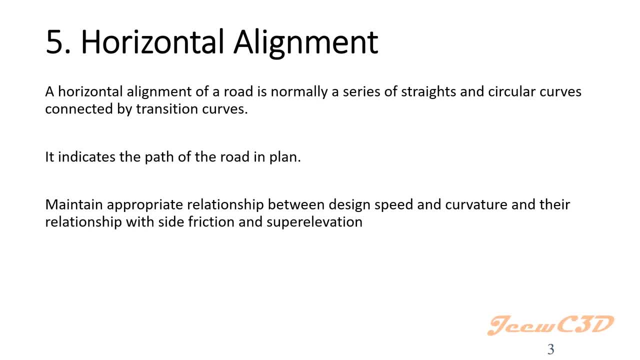 so the horizontal alignment means the plan view of the road. it consists of straights and curves. so horizontal alignment, design, means we are maintaining the appropriate relationships between design, speed, curvature and another relationship between the site distance, friction and super elevation. so we will be learning these things in the coming. 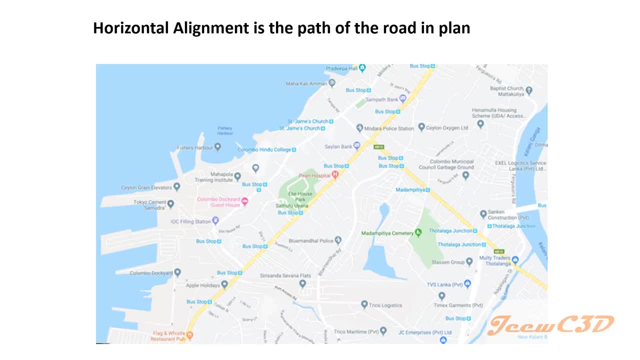 slides. so this is what happens. when you go to Google map, you can see the plan view of a road. this is a collection of roads. only you can see is the straight sections and curved section of the road. so this is the horizontal alignment of the road. this is what we call horizontal alignment. then, as I told you earlier, 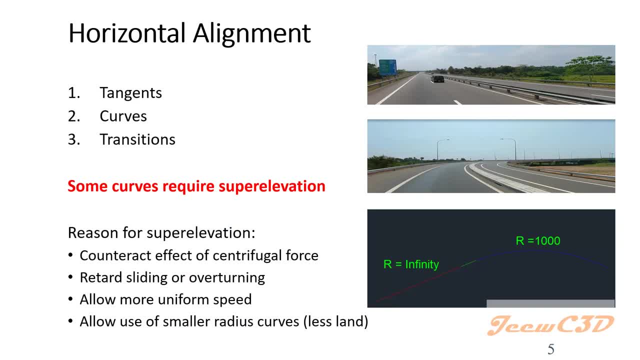 horizontal alignment consists of straights and curves, but we have some additional thing here. these tangents are called the straights, then the curves are the curves and finally we have something called transitions. so in this image you can see this is a straight road. in the middle image you can see the 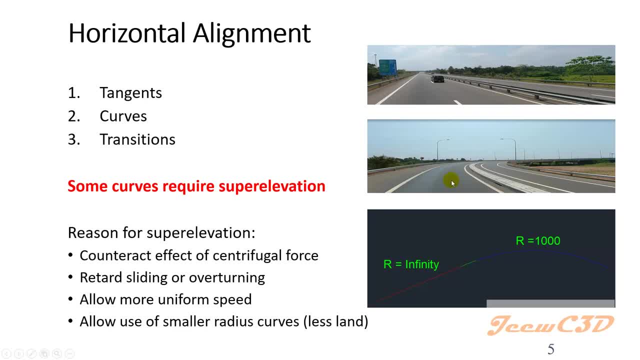 curved road, so we call it a curved section of the road. this is a straight section of a road, so if you consider about the radius of a straight section- that is infinity, then something like this, a curve, it might have a radius something like thousand or hundred or fifty, whatever. so it has some value for. 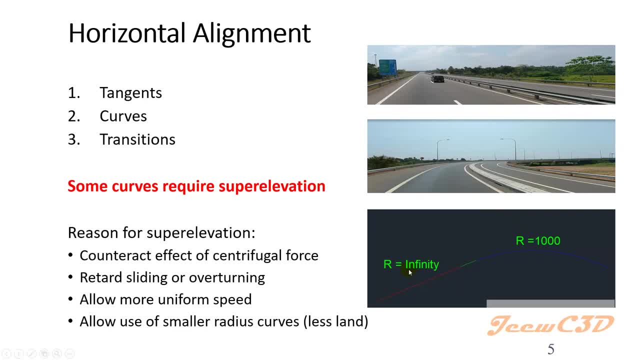 radius. so when you are going to change the radius from infinity to thousand, we can introduce a small curve which changes the radius from infinity to thousand. in this section the radius of the road changes from infinity to thousand, so we call it transition curve. so we are using this transition curve in 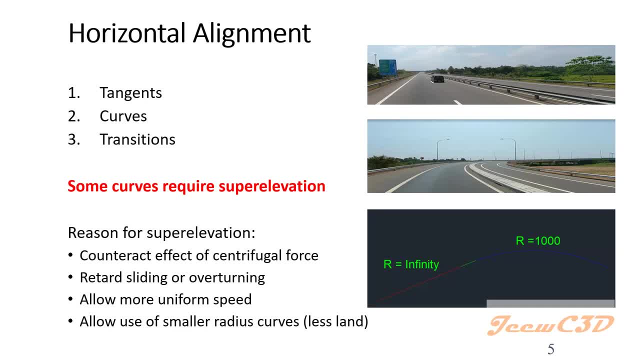 horizontal alignment design at lower speed actually as well as higher speed. we are using that, but the major criteria is the radius of the road. if you have less radius for a road curve such as this, so if you are designing for a design speed of 100 kilometers per hour, if you have a thousand radius curve, you 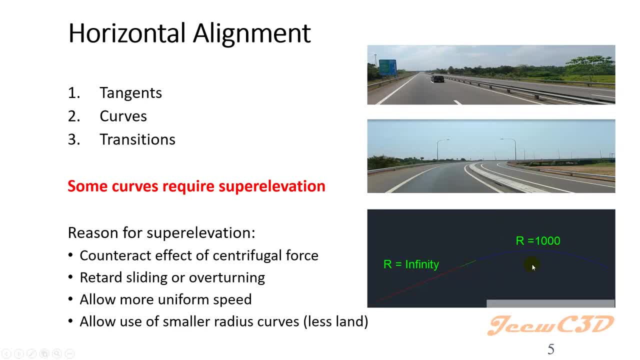 might use the transition curve. sometimes we don't need to use transition curve if this radius is high value. so that is about transition curves. then we have some important thing. some curves require super elevation. so I will talk about super elevations in a later slide, but as for the sake of the completeness, I will 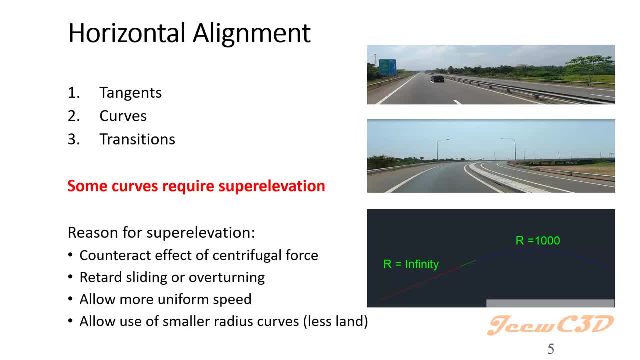 tell what is super elevation here? super elevation is the slope of the road. if you see in this image, the middle image, the slope of the road is completely to this side. so you call it the super elevation because the road is fully rotated to one side. usually you see the roads as usually you see the roads rotated to two. 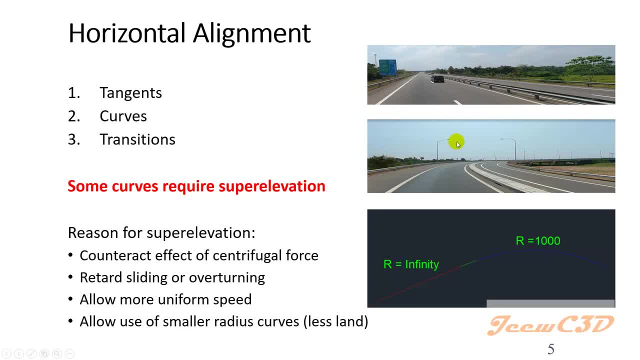 directions. that means some at center line. it comes like this and goes like these two directions, but at a curve you have a one direction slope. we call it super elevation. so the super elevation is used to counteract the effect of centrifugal force and to retard sliding and 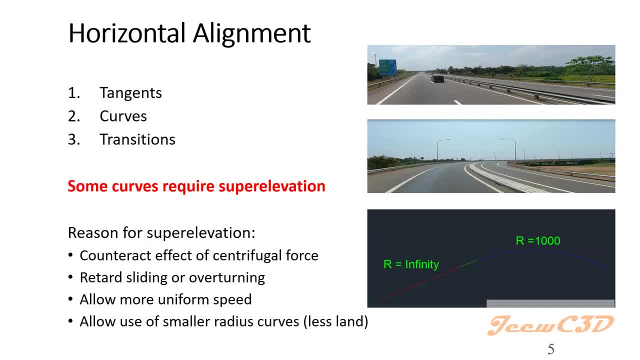 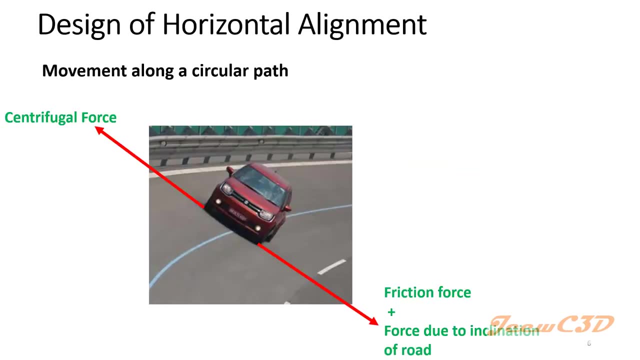 overturning and allow more uniform speed, as well as for use of lesser land for road design. so we will be learning these things in later slides, so here I will describe what is meant by super elevation and what is happening when your car or a vehicle is driving on a circular road, so you may have learned this in your 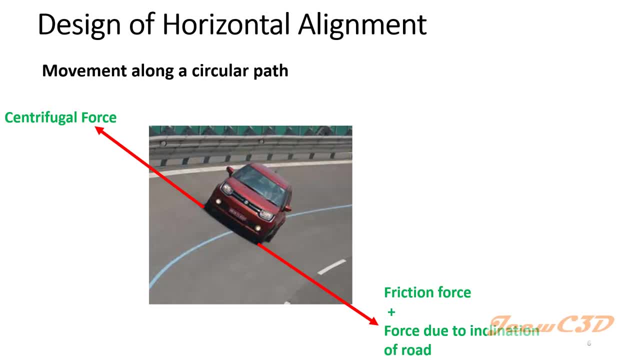 A levels in physics, movement along a circular path. so if you consider this car, it is coming inside this curve so it will have a centrifugal force which is acting outside the which drags the vehicle outside of the curve. so that centrifugal force will drag this vehicle towards the outside edge of the curve. but you have 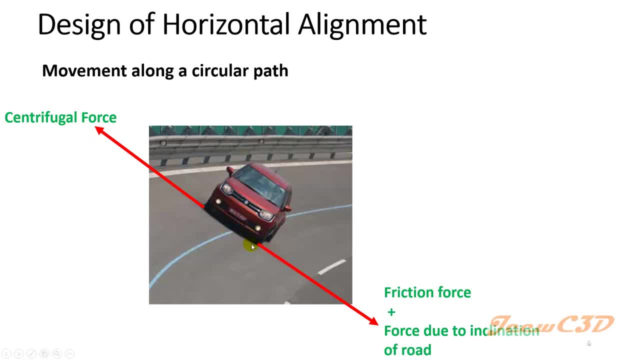 the friction force acting inside direction to the curve, because if the vehicle is going to slide to this way or drag to this way, the super friction force will counteract that and it will act towards this side or the inside of the curve because of the inclination of 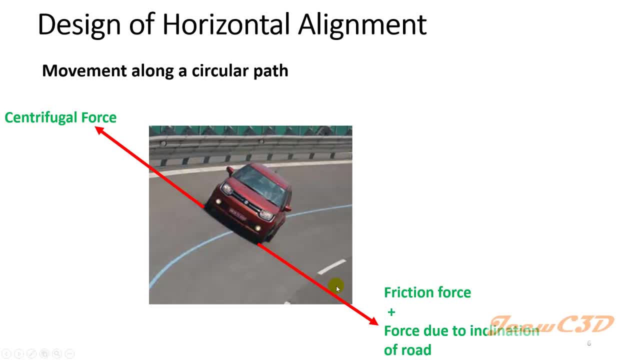 this road. that means this super elevation, this inclination means super elevation. because of this inclination you have a component from the weight to inside of the curve curve. the vehicle weight is coming down, straight down, but some component will act in to the inside section of the road. so the collection of this friction force and force due to inclination of 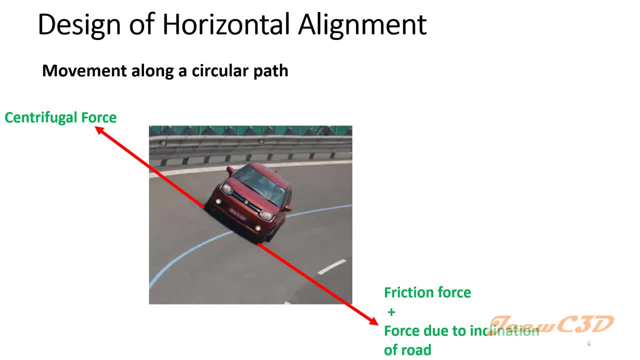 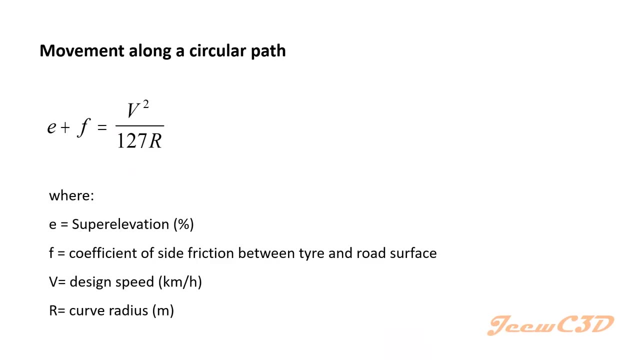 road. these two will counteract this centrifugal force. so using the equation f equals half mv square, you can derive the equation something like this: e plus f equals v square 127 r. so e means the super elevation. as i told you, it is this inclination of the road. then f is the coefficient of side. 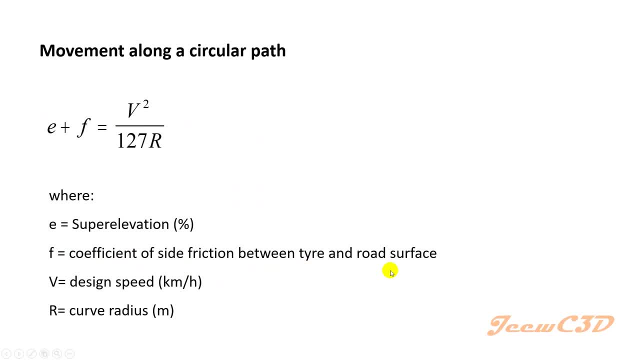 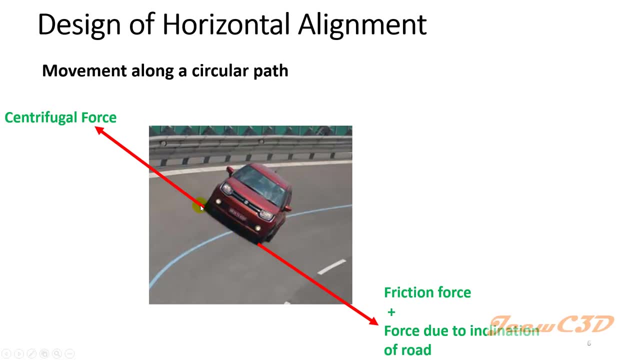 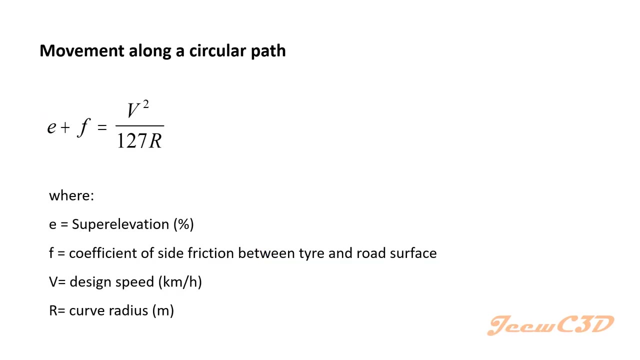 friction between tire and road surface. that means when the vehicle is going to drag this way, the friction of the tire and road surface act along this way, so that friction is called the side friction. if you can remember, we learned about another friction factor called longitudinal friction factor. that is acting along the road. this one is acting across the road. so 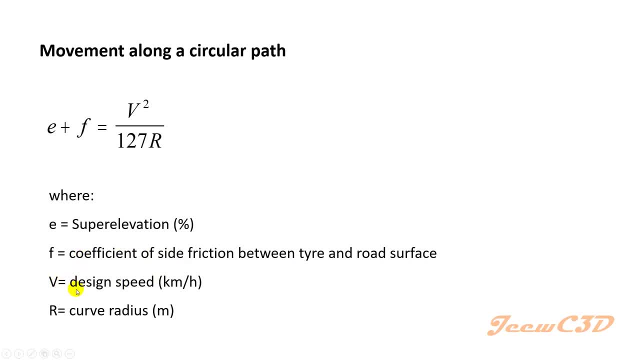 then we have the design speed of the road and finally we have the radius of the curve. so we can see. the moment of along a circular path depends on these factors, especially v and r. if v is increasing, r should be decreased, so r should also be increased. so from this equation, 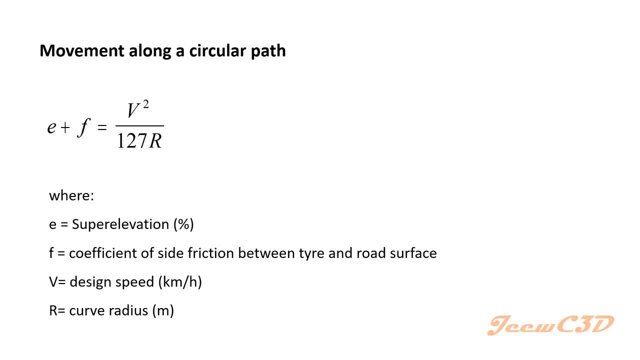 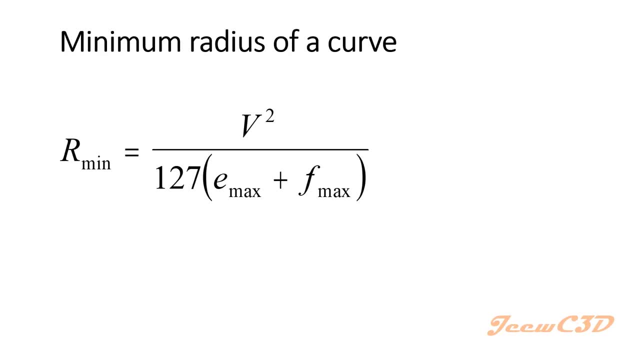 e plus f equals v squared over 127 r. we can get r as the subject and we can put all the things to the other side. so we have r at the left and all the things other side. so we can derive a minimum radius for a curve. so you do take the minimum radius design speed for a code section. 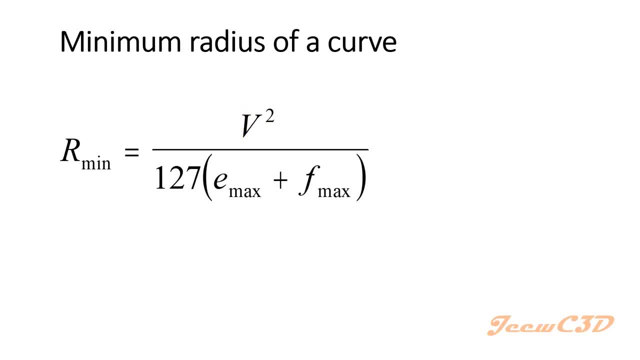 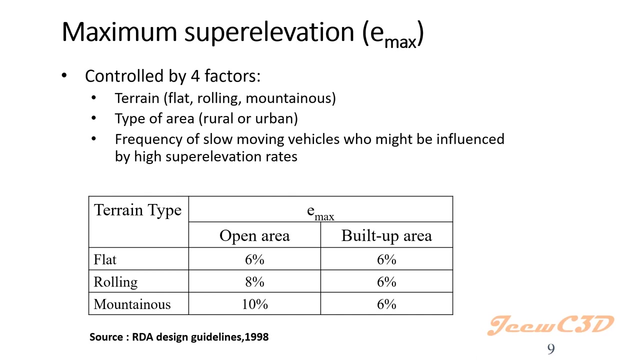 is a constant value, so it depends on e and f, super elevation and side friction. so this r would be minimum when e is maximum and f is maximum. so we get the minimum radius when you have lowest super maximum super elevation as well as maximum side friction. so now we will look at what is the maximum super elevation. 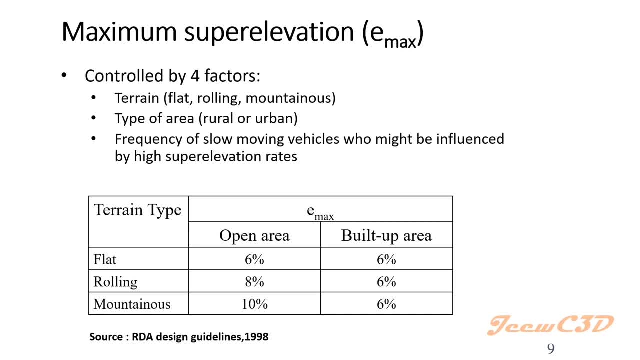 so you cannot have as much as super elevation you like, because inclination of the road depends on several factors or superelevation depends on several factors. what are these factors? one thing is terrain. terrain means what kind of natural ground behavior you have in this area. if it is a flat terrain, that means you have a flat area. you don't have high variation of the. 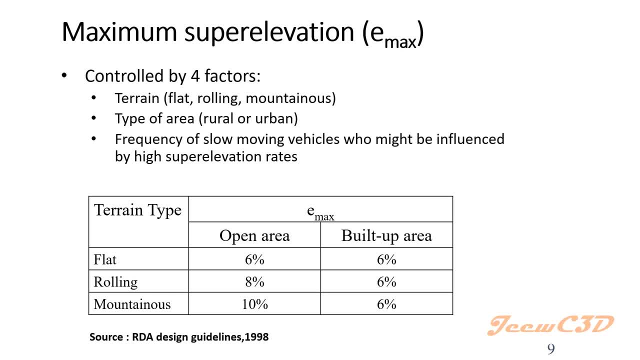 road, so you call it a flat terrain. if it is a rolling terrain, you have flat as well as some mountainous type high sections in the road. if it is a mountainous terrain, you have a mountain to climb in that road section. you have a high steep slope in the road. 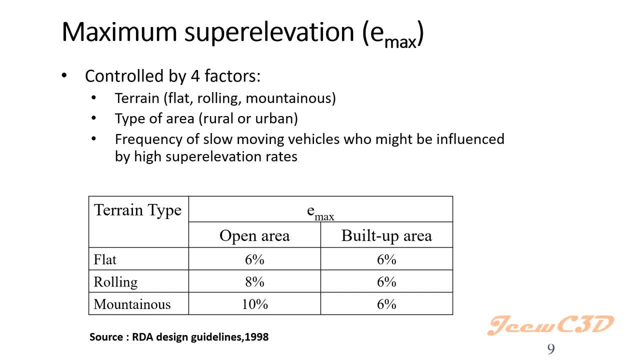 so you call it mountainous terrain. so your super elevation depends on terrain type: flat, rolling terrain or mountain. then type of area, that means whether it is a rural area or a urban area. for rural area we call them open areas, and urban areas we call them built up areas, like here. so then frequency of 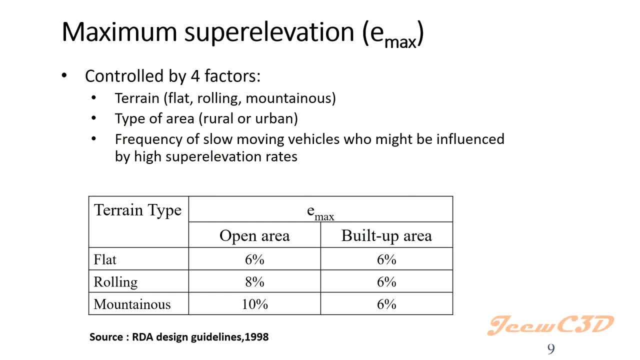 slow moving vehicles who might be influenced by high super elevation rates. so what is this mean? this means slow moving vehicles. that implies for trucks or heavy vehicles, they are moving slowly. so if you have high super elevation rates and if you have so many slow moving vehicles, if you can remember. 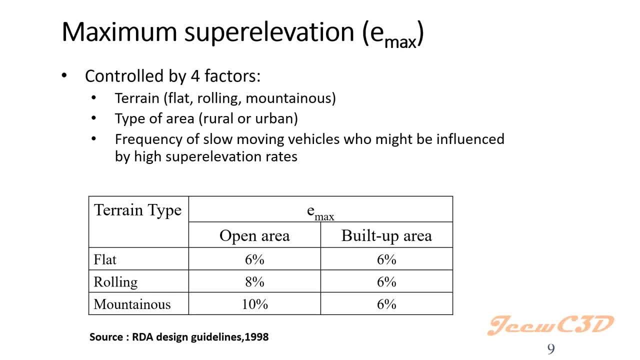 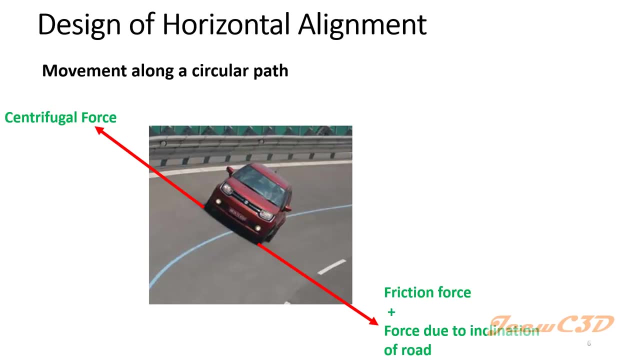 that a component of the vehicle load acts in side direction or the uh towards the center of the curve. so if you, if i go back to this image, so if you have a heavy vehicle here, so this load will act on the ground and one component will act along the road. so if you have a high inclination, 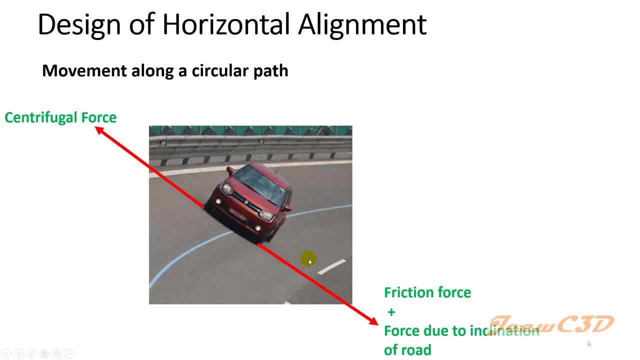 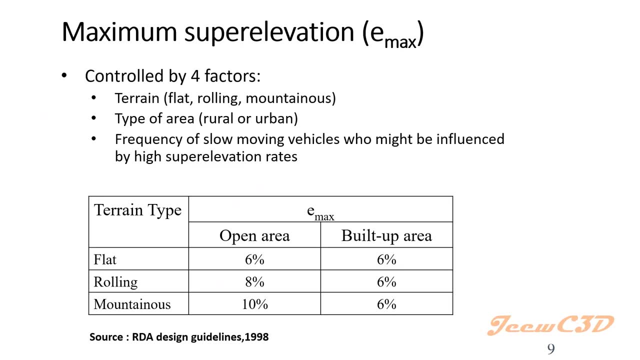 this load component will be high and it might tend to. it might cause the heavy vehicles to fall or topple on the road. you may have seen this in roads. sometimes the heavy vehicles are fallen apart or they are toppled on the road because of this super elevation effect. so 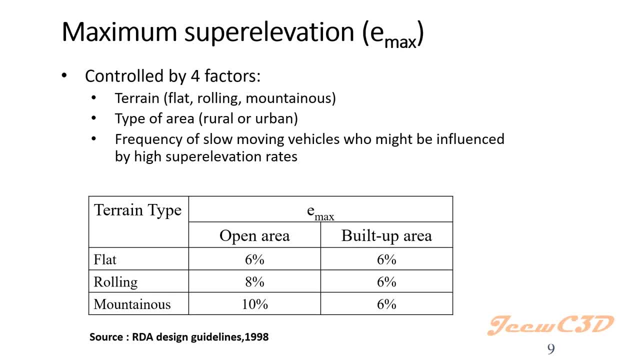 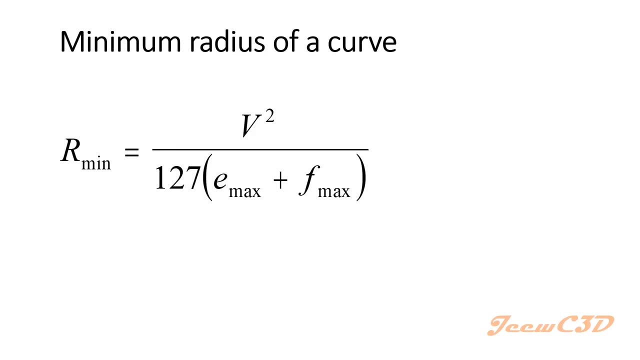 in this table. this table is taken from RDA design guidelines. it will tell you if your road is, if your road is in a flat terrain and if it is open area. that means if it is a rural area, you have to use maximum super elevation of 6%. so if you are trying to get the radius you have to use for a. 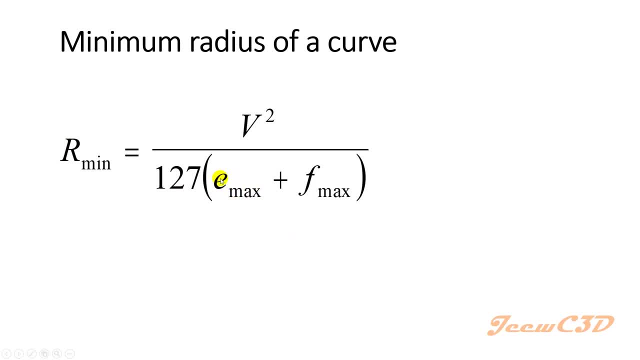 flat terrain you have to use a max of 6%. that does not mean you have to always select 6%, but the maximum is 6%. you can use less than that value, 6% or less than that value. then for a rolling terrain you can go. 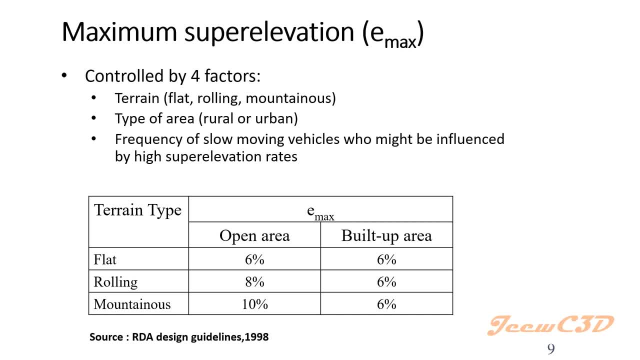 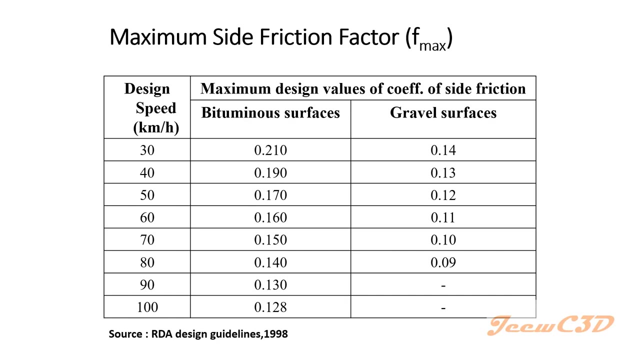 up to 8% and mountainous terrain you can go up to 10%. so in the data areas we always think that the highest super elevation is 6%, not more than that. then the other factor, maximum side friction factor. the equation equals e max plus f max. so the maximum side friction factors are given in: 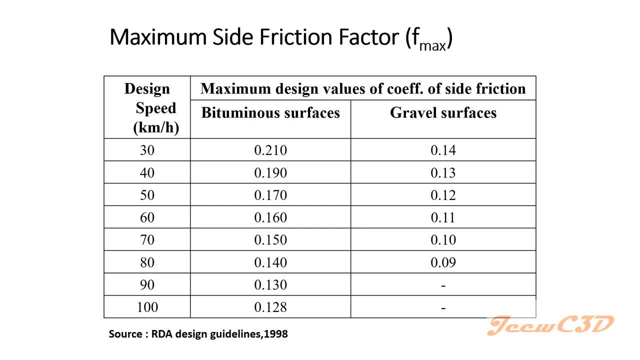 RDA design guidelines. so it depends on the design speed of the vehicle. so you can see these values depends on the design speed of the vehicle. the f max values, the bituminous surfaces are the surfaces, the asphalt surface or the tar roads. so that is the surface surface for the tar roads. so the 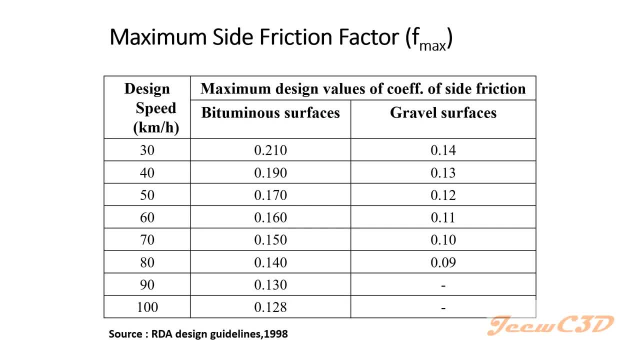 those are the friction values for tar roads and this is for gravel roads, which is which we are using in village roads. so these are factors you have to use when calculating the minimum radius for a horizontal curve. so in these two parameters we can define the recommended minimum curve radius. 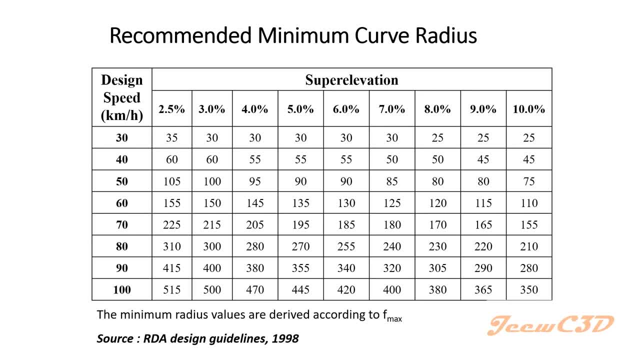 for a road curve. that means something like this: if I consider this row, if I consider this row, assume that you are assigned to design a road, so the design speed of the road is 30 kilometers per hour, then you have to have- let us say you have to. 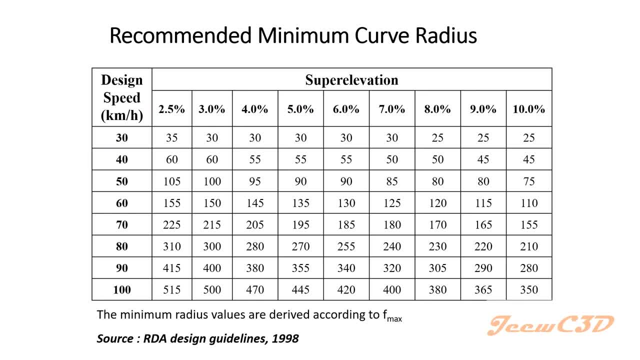 have a road curve, you have to design a road curve. so now you are in a program where you are in a position to select the road curve. so when you draw the curve, you can you. when you draw the curve, you want to have an idea. you need to have an idea what kind of radius I have to use for this design speed. 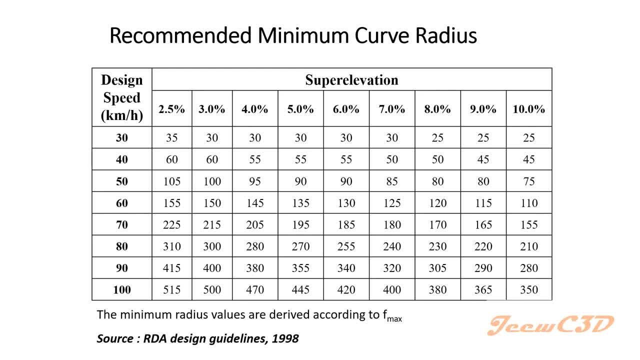 so if you design the road for 30 kilometers per hour and if we assume that road is in an urban area, so if you design the road for 30 kilometers per hour and if we assume that road is in an urban area, so if you design the road for 30 kilometers per hour and if we assume that road is in an urban area, 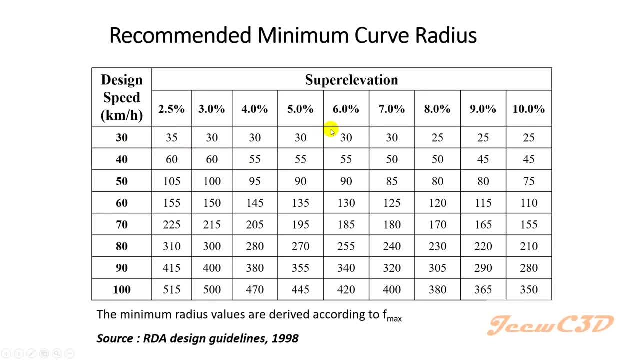 so maximum super elevation you can go is six percent for maximum super elevation, six percent for design speed of 30. the lowest radius you can go is 30 meters for the road curve, so the horizontal alignment. you cannot use curves where your radius is less than 30 meters. 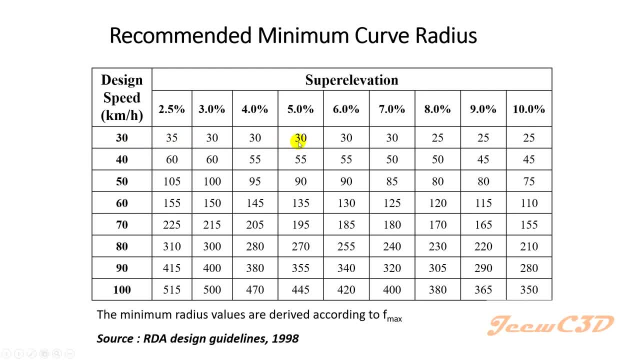 for design speed of 30 in an urban area. so if you have a 25 meter radius- that can't be so- you have to increase the radius to 30 meters or more. it is okay to have radius, let us say 35 meters, then it is okay because it is greater than 30. 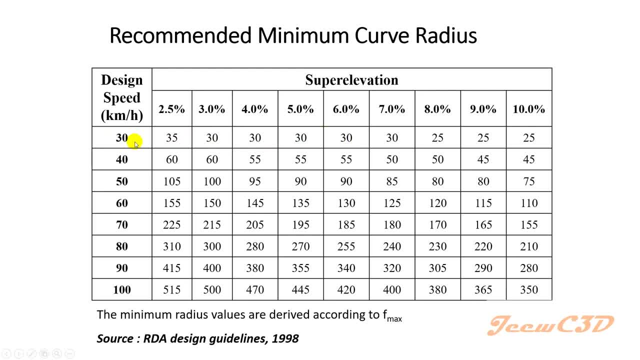 so that is the basis: how to select road curves. one more example if I use: if we assume that we are going to design a road with 50 kilometers per hour here, 50 kilometers per hour, let us say that is an urban area as well, so you can have maximum super elevation of six percent. 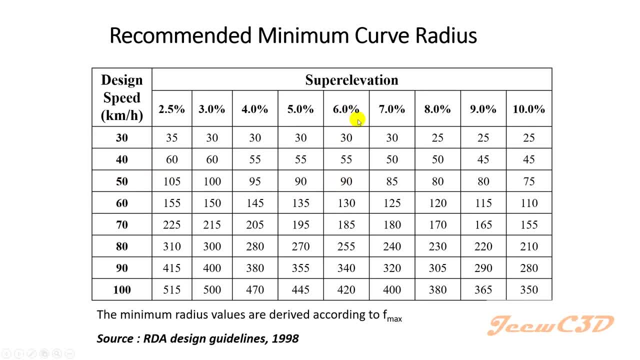 so you have this row and this row, so the lowest radius you can take is 90 meters. so, whatever, the radius you apply to a curve in your road should be 90 or greater than that. so if there is a situation you can't adopt 90 meter radius at some location, there are some certain precautions we can get. 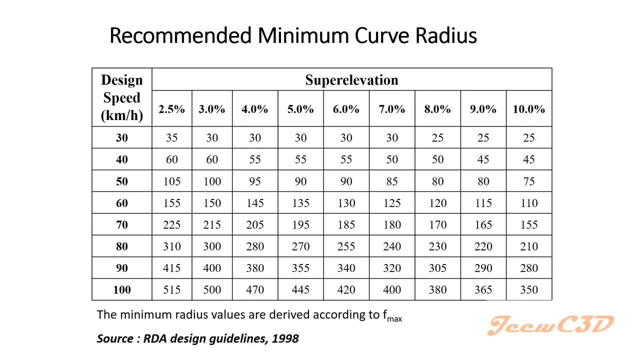 but generally you have to use the radius which is greater than 90 meter in your design. so the design speed of 50 kilometers per hour. so that is about minimum radius of curves. you have to select the minimum radius and depending on the design speed and depending on other scenarios, 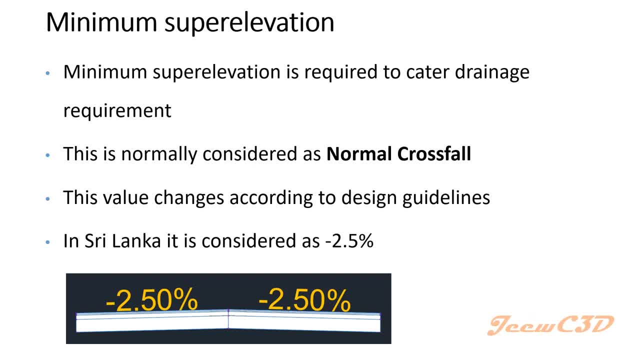 we learned about the maximum super elevation, so what is the minimum super elevation you can have? we learned about maximum super elevation. what is the minimum super elevation we can have? so what are the criteria we need to consider when you think of the minimum super elevation? the minimum super elevation is used to cater the drainage requirement. 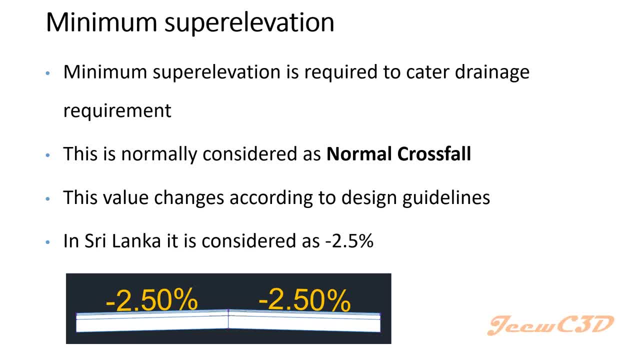 so when you are constructing a road, you need to ensure that no water is retained inside the road. when it is raining, or when it is a wet season or a wet condition, the water which comes on top of the road should have to be drained out from the road. 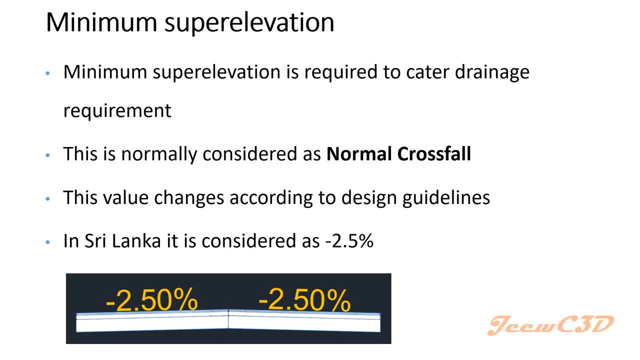 it cannot be retained or it cannot be stored. or it cannot be stored on the road until it is dried out. so we need to make sure that there is no water retained on the road when it is raining or when the road is at a wet condition. so the minimum super elevation is selected to cater the drainage requirement. 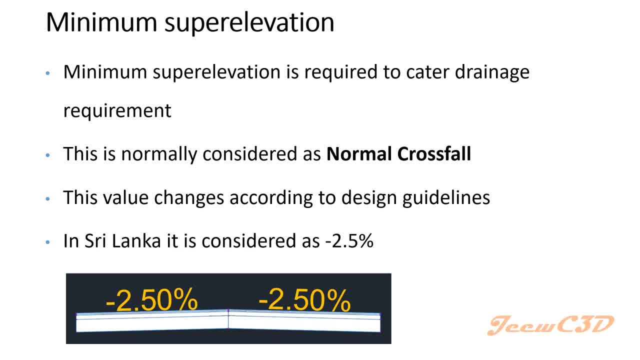 in Sri Lanka the minimum super elevation is minus 2.5. minimum super elevation means you might have, you can actually when, when you are, when the vehicle is driving on a curve, we learned that to counteract the centrifugal force we need super elevation. but on a straight section we don't need super elevation. 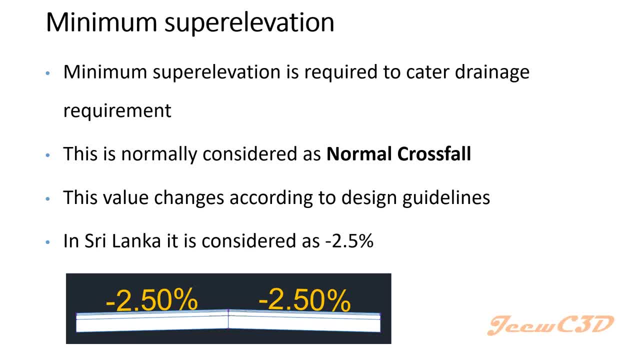 so that means we can have a flat road. but if you have a flat road it will not drain out the water from road. so in straight section, specially to drain out the water from the road surface, we use a inclination to the road, so we call it the normal cross fall. 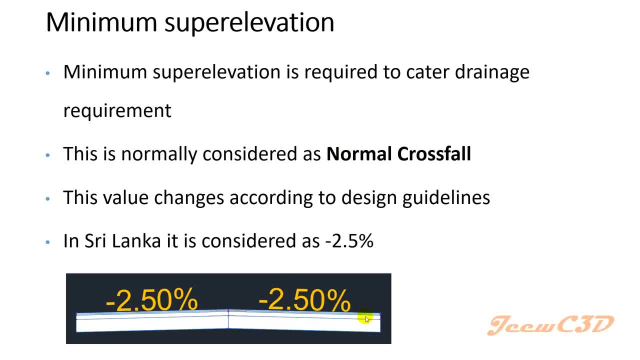 it is minus 2.5 for each direction of the road. if this is the center line of the road, it will slope down minus 2.5 slope. so that is the general practice in Sri Lanka, but this might not be the case in Sri Lanka. 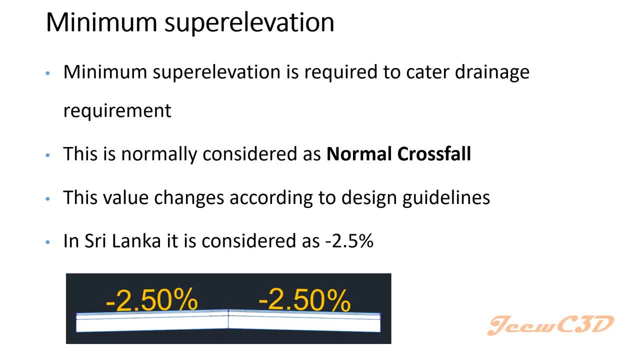 so the normal cross fall is minus 2.5 value or this normal cross fall is changed from country to country depending on their design guideline. in USA they might usually use minus 2, in Australia they use minus 3, so in Sri Lanka what we use is minus 2.5. 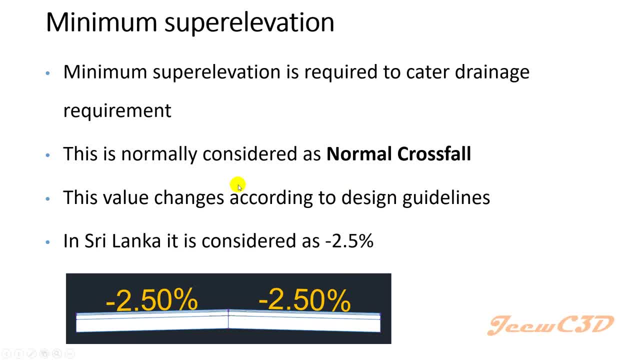 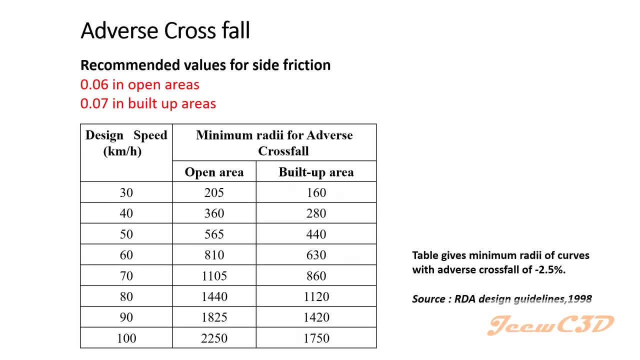 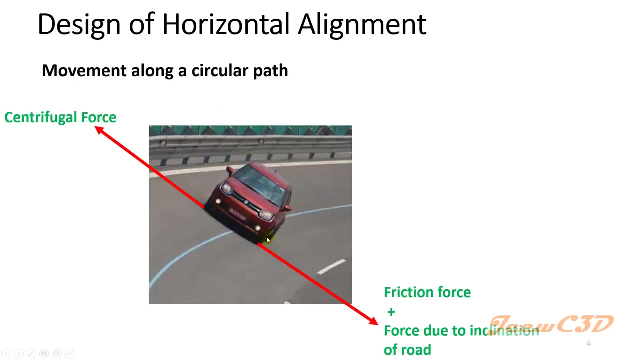 then we are looking at the concept called adverse cross fall. so what is adverse cross fall? to describe this, I will go back to the slide where we learned about motion along a circular path. so in this slide we see the inclination of the road and the friction force will counteract the centrifugal force. 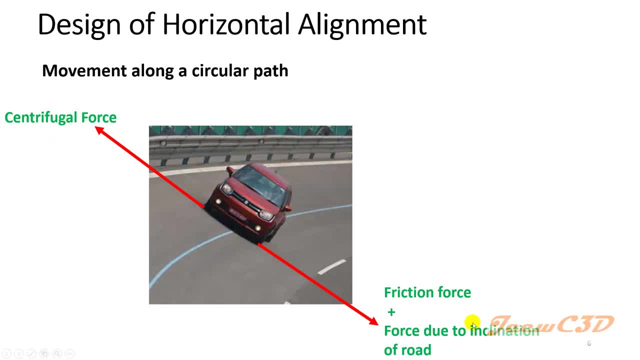 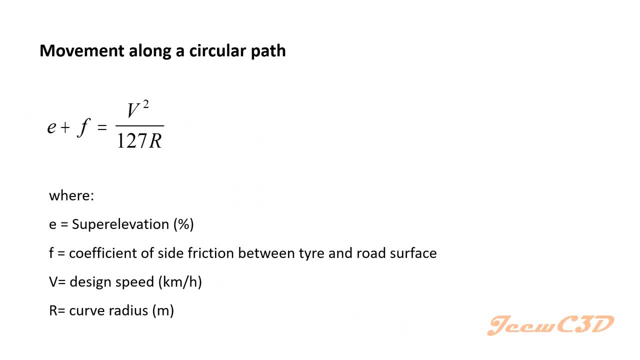 so the inclination of the road or otherwise the superelevation of the road will depend on the radius of that curve. if the curve radius is high, you might not have higher superelevation. if the curve radius is lower, you should have higher superelevation. so if this radius is high, 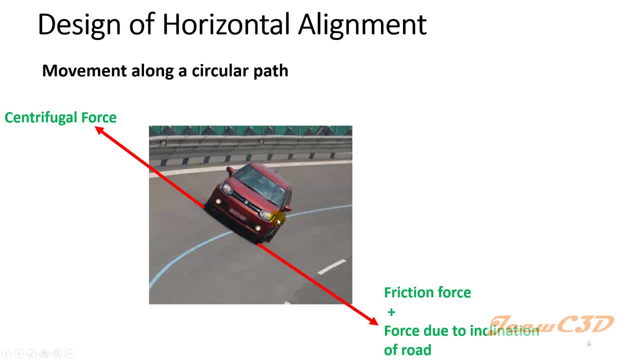 that means you don't need much superelevation. so when this radius is high, the curve radius is high. this friction force can single handedly tackle this centrifugal force. it does not need the force due to inclination of the road. so that means the curve does not need superelevation at this curve radius. 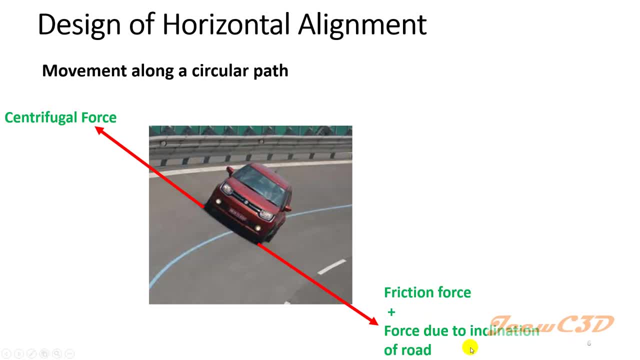 so at that radius, that means at a higher radius. this superelevation or the inclination of road will not be used to counteract the centrifugal force. the friction force itself counteract the centrifugal force. so that means you don't need to incline this road. 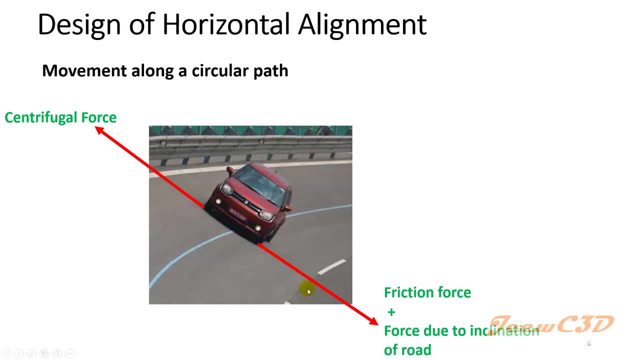 so you don't need to incline this road. instead you can use the normal cross pole at that section. so usually at a curve, in this curve your road is sloped like this, but at the at a higher radius. if this friction force single handedly counteract this centrifugal force, 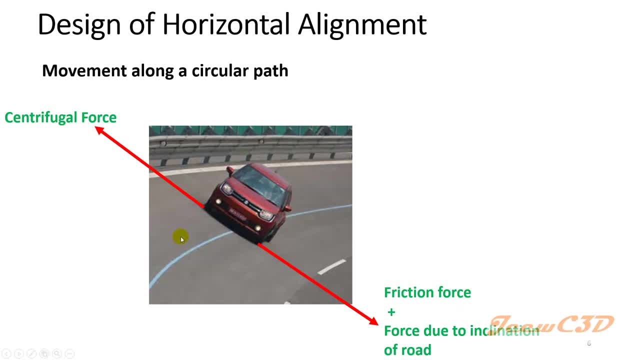 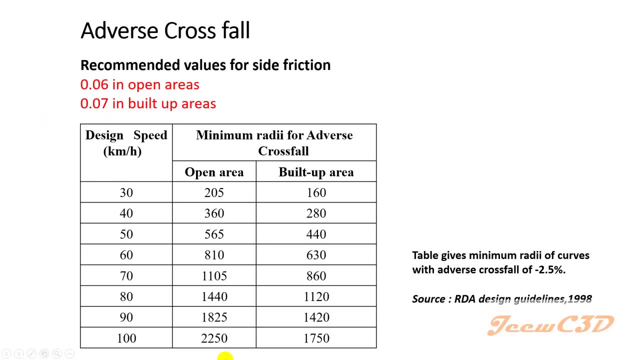 you can have this road, like this, sloped two ways. so you call that radius adverse cross pole. you call that radius adverse cross pole. this adverse cross pole means at that cross radius your road has the normal cross pole. you don't have a superelevation, it will only have a normal cross pole. 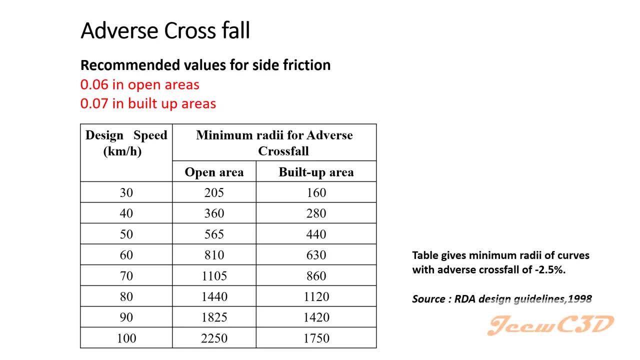 so to have the adverse cross pole, we select the side friction values as 0.06 and 0.07. for open areas, 0.06 that means Fmax, and for built up areas it is 0.07. so when you calculate the radius, 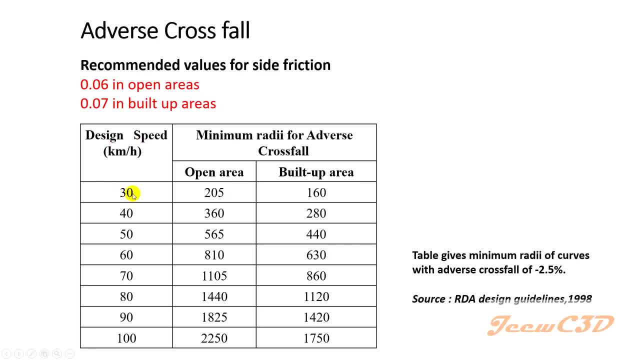 the radius would come. if the design speed is 30, the adverse cross pole for open area would be 205. for built up area it would be 160. so if your curve is 205 you don't need to have superelevation that so, if I 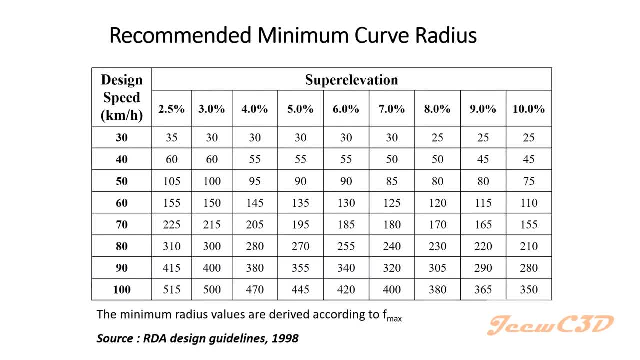 make it more clear: if you have a radius of 100 meters, you should have superelevation of 2.5, because if the design speed is 30 and your radius- your radius- is 100 meters, that means more than 35. you should have superelevation of. 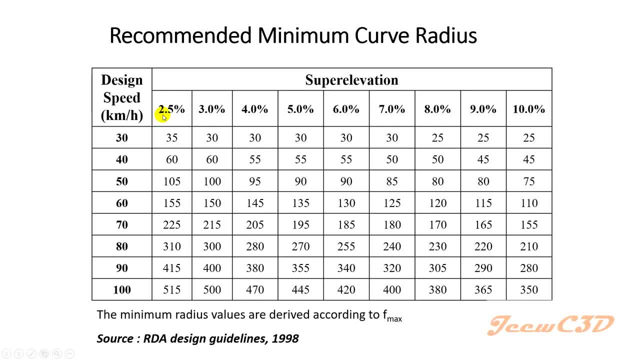 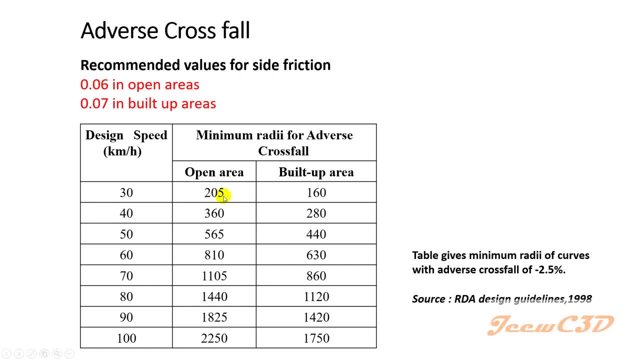 2.5. so when your radius is more than the adverse cross pole or equal to adverse cross pole, your superelevation will not be there. your superelevation would be the normal cross pole. so there won't be any superelevation. that superelevation would be replaced by the normal cross pole. 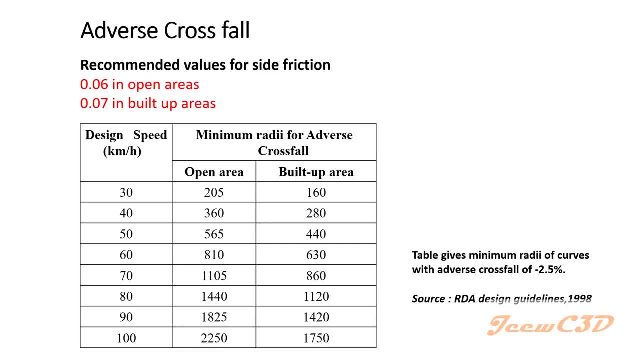 so we will be learning it more clearly in. we are learning about superelevation section, but for the moment you can. you have to understand: if your curve radius is greater than the adverse cross pole, you have to use normal cross pole for the row. that's about. 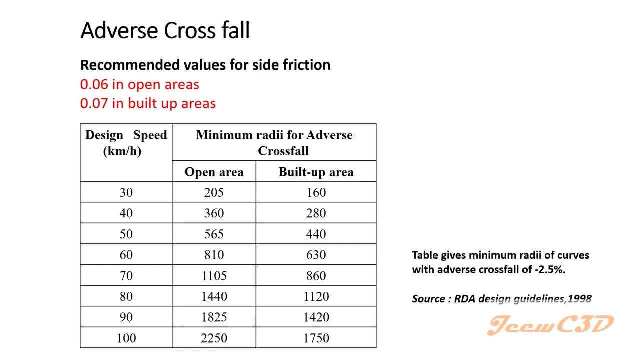 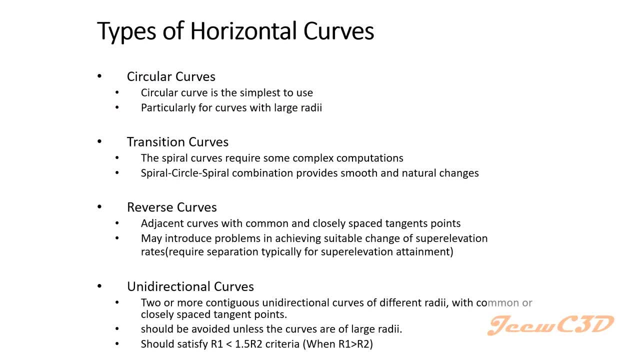 adverse cross pole. then we will learn about the types of horizontal curves. you have several types of curves: circular curves, transition curves, reverse curves and unidirectional curves. circular curves are simple curves, transition curves, i told you earlier they are the radius changing from infinity to some defining. 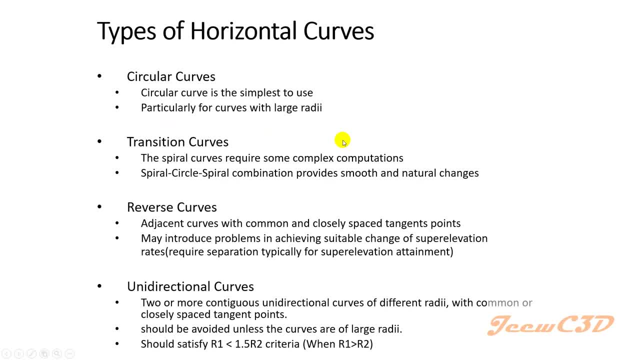 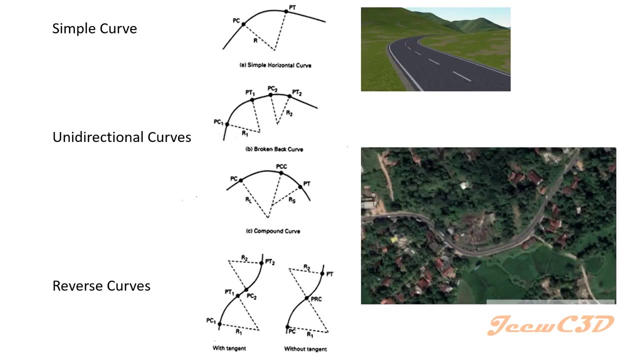 definite value. like in the first slide i told you about changing the radius from infinity to thousand, like that. reverse curves and unidirectional curves are type of curves where you have two curves in same direction or two curves in different direction. so we will be learning them here. 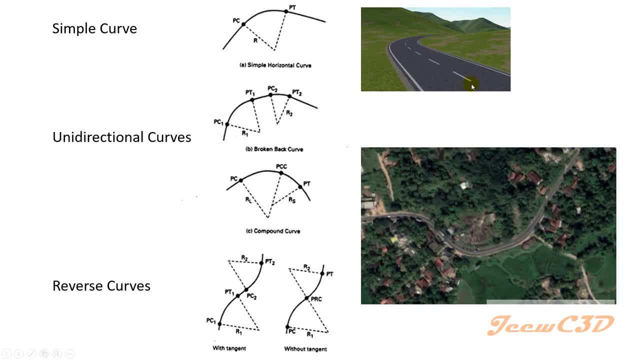 this is a simple curve. you have a curve on the top. we call it simple curve, then unidirectional curve means you have two curves in the same direction. sometimes there may be a small straight section in the middle. sometimes there won't be a straight section. you have. 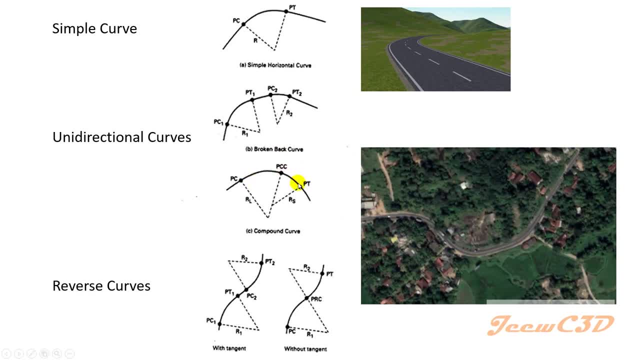 two curves, two radius of curves on the top. so if you have a small tangent section or a straight section, we call it a broken back curve. otherwise we call this a compound curve. so in reverse curves you have a curve coming from one direction and rotate, changing its direction. 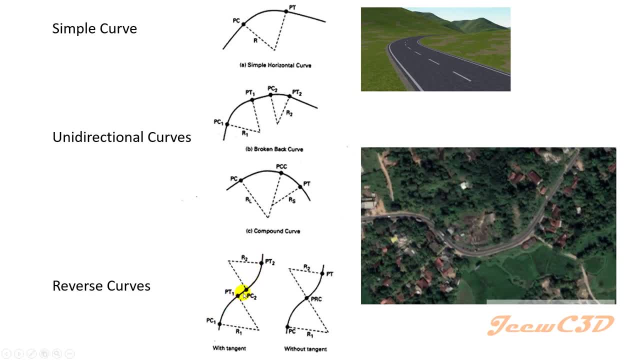 to the other side. there may be a small tangent in between. so this is a reverse curve with tangent and this is a reverse curve without tangent. so if i see this image you can see here i have a curve going this direction and i have another curve in the same direction. 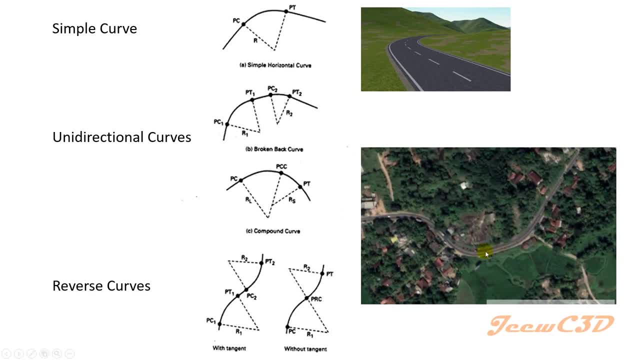 with a small straight section in the middle. so we call this a broken back curve. you have a curve in the same direction. you have another curve with a straight section in the middle. so if you don't have this straight section, only these two curves, you call it. 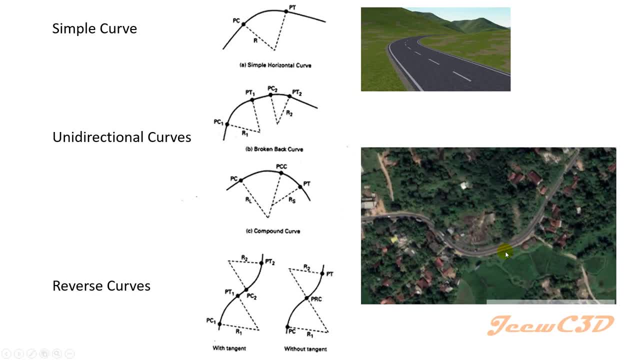 a unidirectional curve in here. you can see this is this curve is coming this direction and it is changing the direction to the other side. you call it a reverse curve: coming from this side and change the direction to the other side. so this section, you have a. 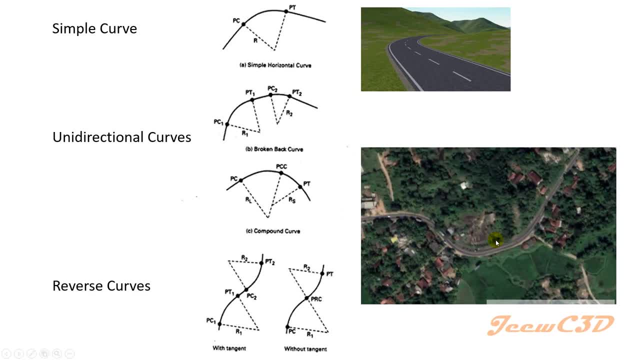 reverse curve. in this section you have a compound curve, so that is about horizontal alignment. we learned about coordinates, what are the transition sections? and we learned about superelevation. and we learned about the radius of curves. what are the minimum radius of curves we have to adopt? 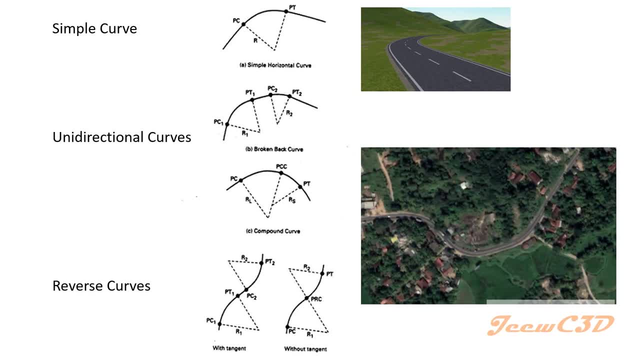 and then we learned about maximum superelevation. and minimum superelevation we have to use the cross pole and then the transition section. we have to have the horizontal curves and the horizontal curves. so in the next section we will be looking at the horizontal curves, we will be looking at the super elevation, one of the hardest and important criteria, important. 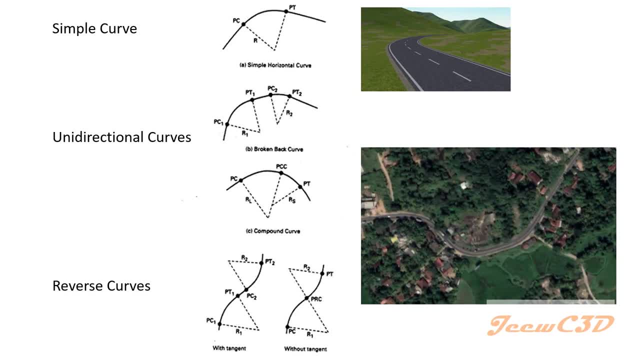 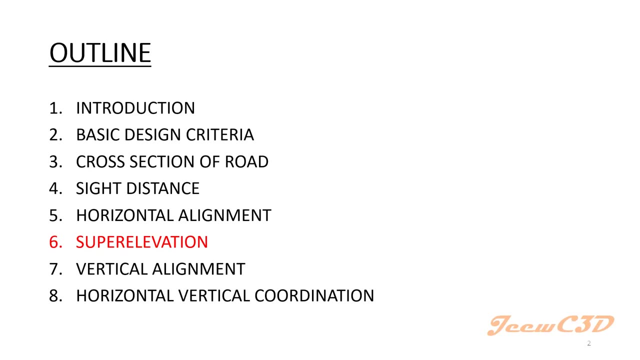 section in high ratio metric design. so we will be looking at that. in the next section in this lecture we are going to look at the super elevation of the road. super elevation is one of the most important thing in highway geometric design. so we have some kind of introduction about super elevation and the horizontal alignment section. 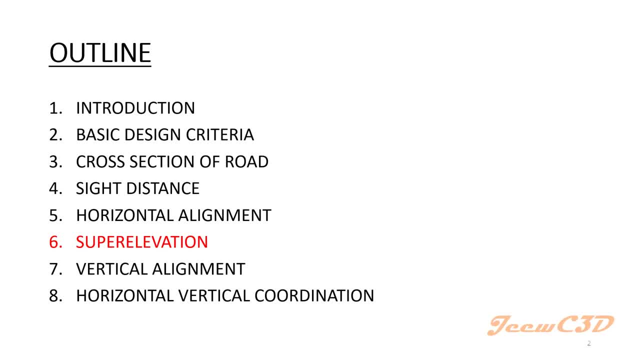 you know now what is the value of super elevation we need to consider depending on the radius of an alignment or the radius of a curve. in this section we are looking at how to apply super elevation to an alignment. so here in this section we are looking at the super 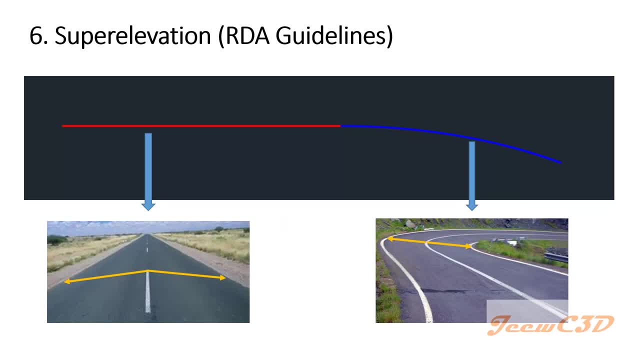 elevation according to rda design guidelines. if you think this is a plan of the road, this is an straight section. this red part and this blue section is a curved portion. in the straight section you have a crowd of this kind. you have slopes both sides of the road, from the center line. you call this the no. 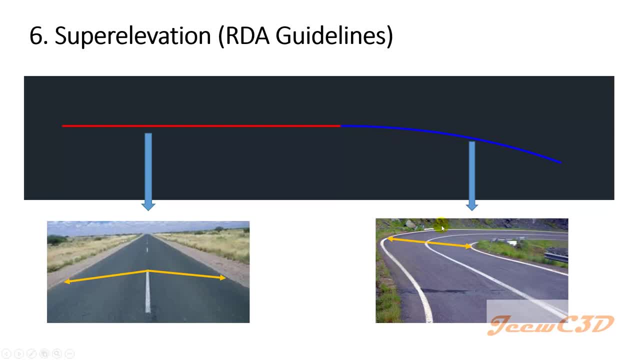 cross falls when you come into the curve, to provide proper centrifugal force, we have to rotate this pavement, or rotate this road in such a way that it provides the centrifugal acceleration, counteract the centrifugal force. so in that scenario your pavement will look like this: it will rotate. 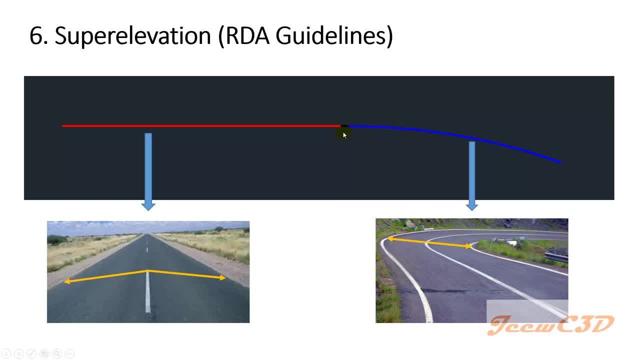 like this. so When the curve is rotating in this direction, we call it clockwise direction curve. So in this clockwise direction curve you can see your right side is turned upward and your left side is turned downward. So if you compare these two images, you can see your right side is at the bottom side and your left side is at the top side. 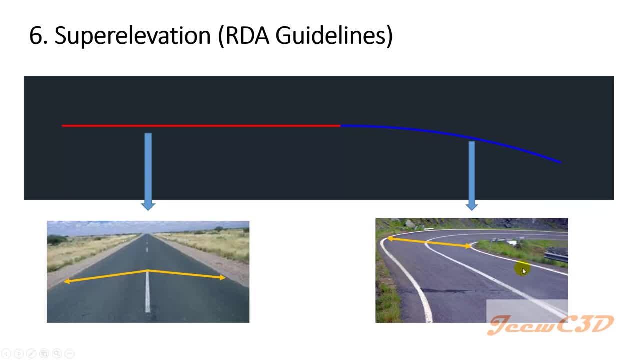 So if you compare these two images you can see the right side of both images have same slope or kind of same direction. It is sloping into the same direction. But when you consider the left side in the first image or in the straight section, the left side slope this way downward, but it has turned upward. 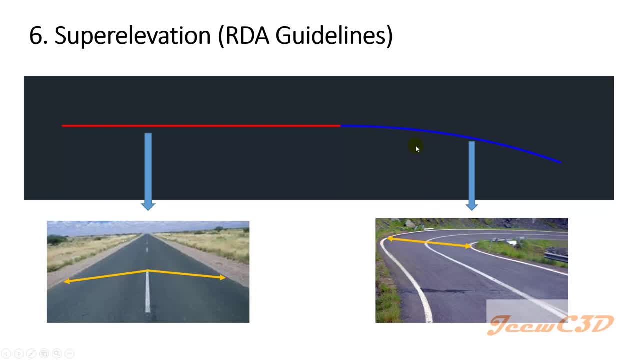 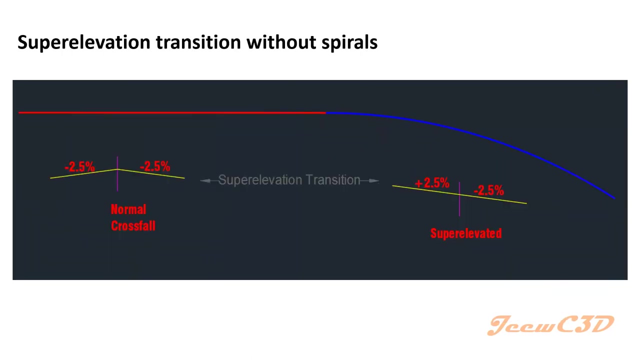 From the center line. it has turned upward in the curve. So you can see, the road has turned from this view to this view within this curve, along this road. So actually, what has happened is this: Let us say: in this straight section you have your road. 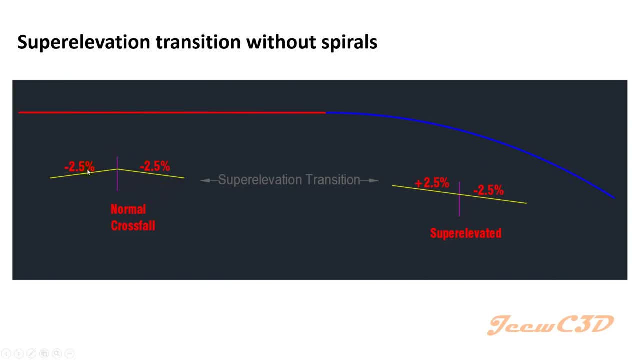 As minus 2.5 super elevation. we call it normal crosswalk and we know come inside the curve you have. for the left side you have plus 2.5 and to the right side you have minus 2.5.. 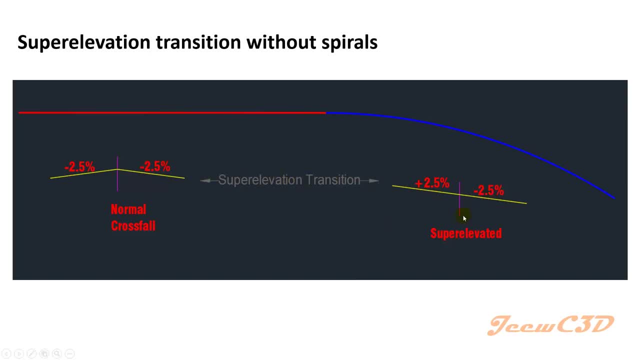 So, since this right side is same but your left side have different super elevation or different slopes, So if you consider the right side, this right side has to rotate upward and come Plus 2.5 somewhere in this road, So it will occur along some distance. 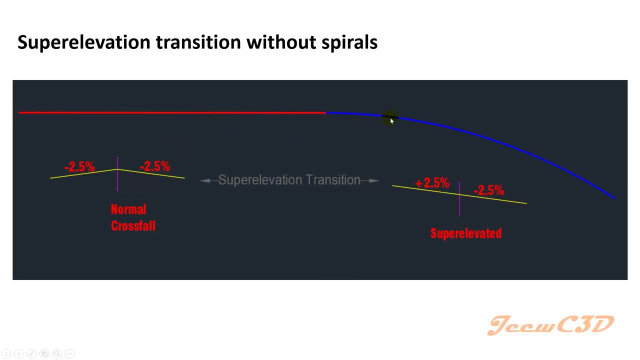 It will occur along some distance. we call it super elevation transition. This super elevation transition from minus 2.5 to plus 2.5, it occurs along some distance. We call it super elevation transition distance. so otherwise we call it super elevation development length. so i have named this section. 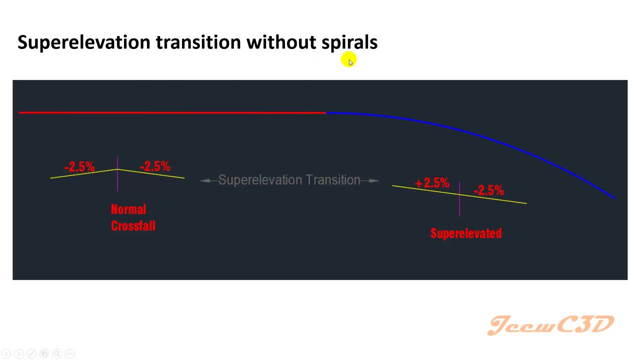 as super elevation transition without spirals. if you can remember, spirals are curves where you change the radius from infinite to a definite value. but without spiral means this straight and curve is smoothly joined. that means there is no spiral. the straight section is tangent to this curved section. this is this. this is kind of a smooth connection. but if you have a spiral curve, 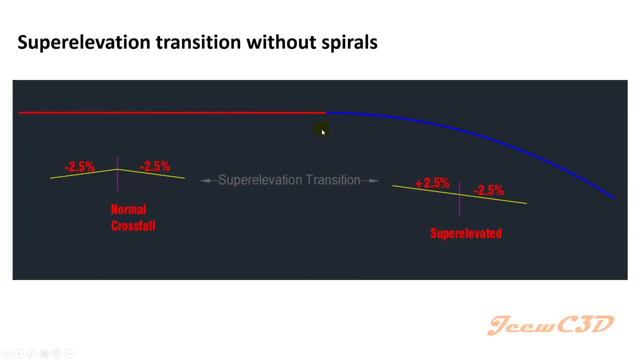 that is more desirable for drivers. that is more smooth connection than this one. but in this lecture series we will not be looking at the spirals, we will not be looking at only roads without spiders. so now we have some kind of idea. this super elevation transition is 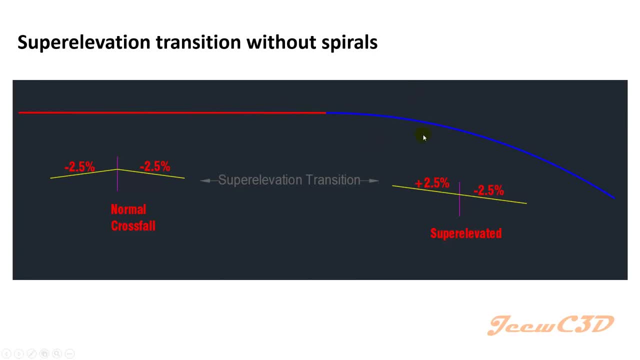 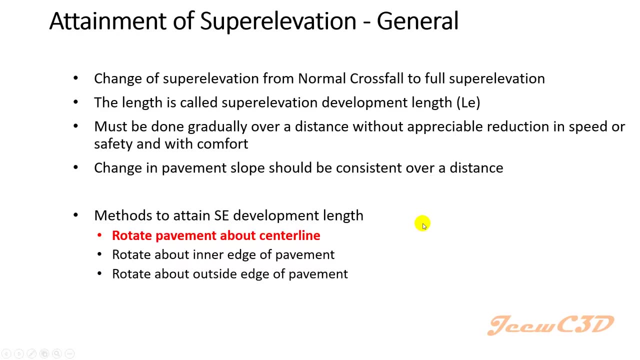 happening inside this road to rotate the pavement from minus 2.5 to plus 2.5. so we call this as attainment of super elevation. so the change of super from normal cross pole to full super elevation, that means from minus 2.5 to. 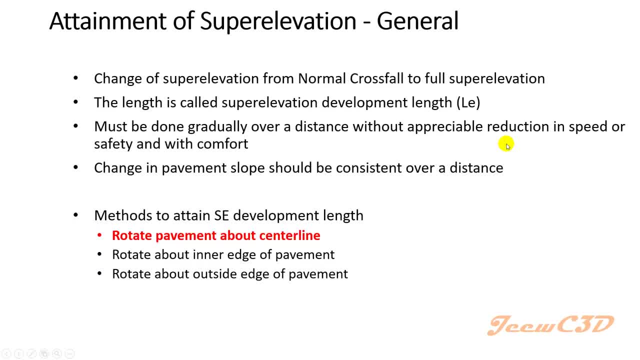 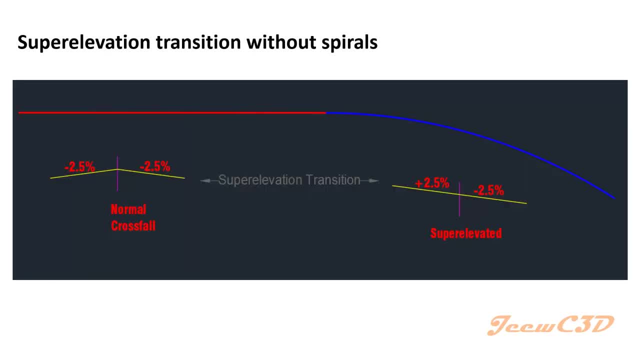 plus 2.5 is called super elevation development length. actually, even if I, when I say minus 2.5 to plus 2.5, it is only for this example. but if this is super elevation minus 5 and plus 5, that distance would be the super elevation. 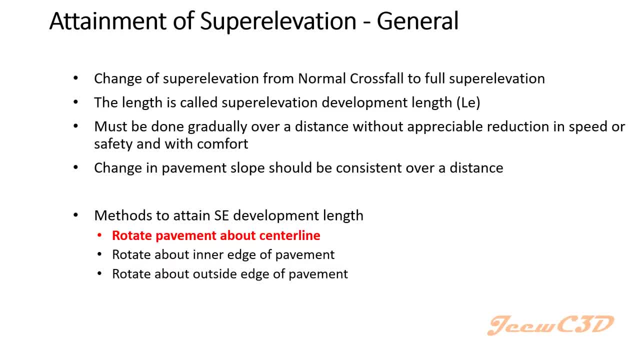 development length. so it should be gradually. it should be gradually over a distance without appreciable reduction in speed or safety or comfort. so when you are rotating the pavement you have to rotating the pavement along some distance of the road. so that should be a great variation of the pavement rotation so it might not feel to the driver that. 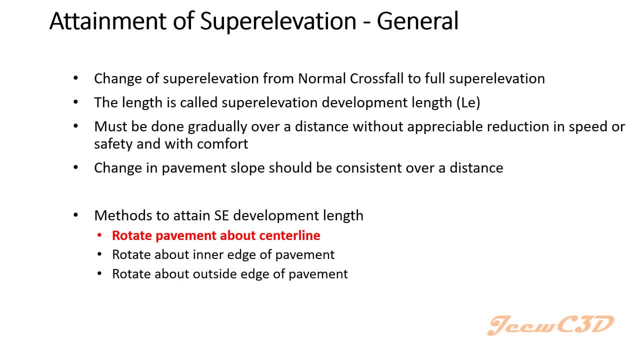 there is a change in the cross slope of the road, changing the slope of the road, so we call it the comfort effect of the road. so when we are rotating the road it should be rotating at the rate that is comfortable for the driver and the pavement. so there are three methods to attend to valuation. 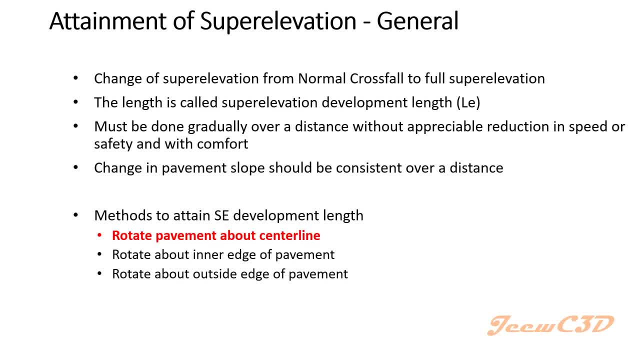 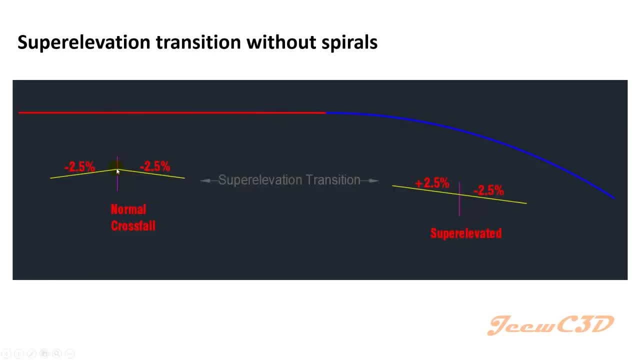 development length. but mainly what we are using is rotate the pavement above the centerline. if I go here, this pavement is rotated along this centerline. you can see this part is turned upward along this, so above this centerline. so most in most cases, we are rotating the pavement, with or without rotation. so this should be a better rotation than using the improvement along the road. 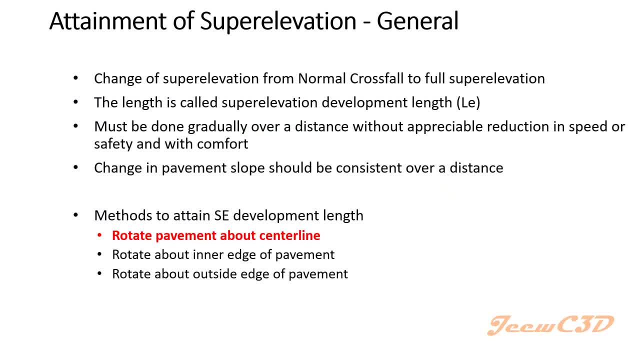 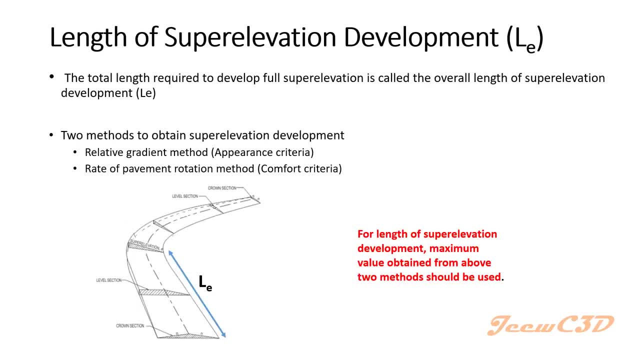 about the center line that is. here we consider superelevation, development length. so this is actually what happens in developing superelevation. you have a normal crown section or a normal straight section. your road will be like this: if it is normal crown, this is minus 2.5 then 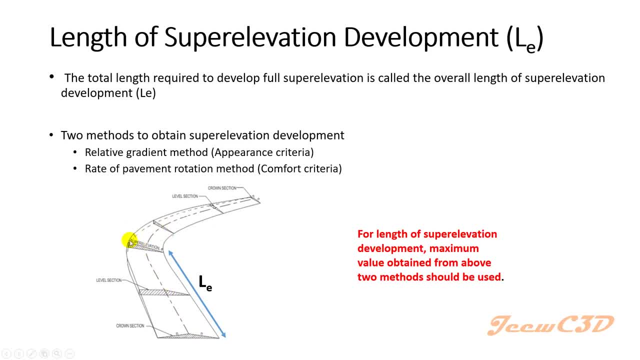 it is going into a curve. in the curve you have full superelevation. that is kind of superelevation value. if you say this value is 2.5, this side will be minus minus 2.5. this side will be plus 2.5 as. 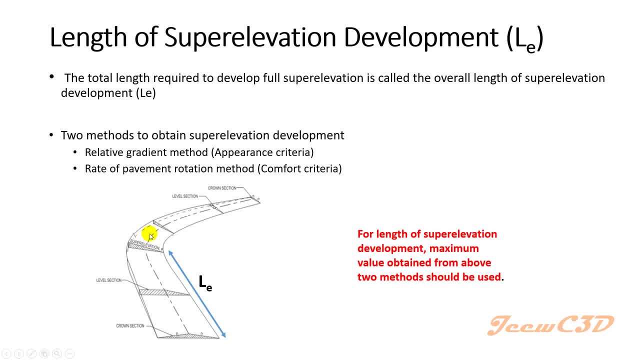 in the previous image. so if this is minus, if the superelevation is plus 4, this side should be minus 4, this side should be 4 plus flow plus 4. so in this example, this curve will. this curve will be super elevated like this: 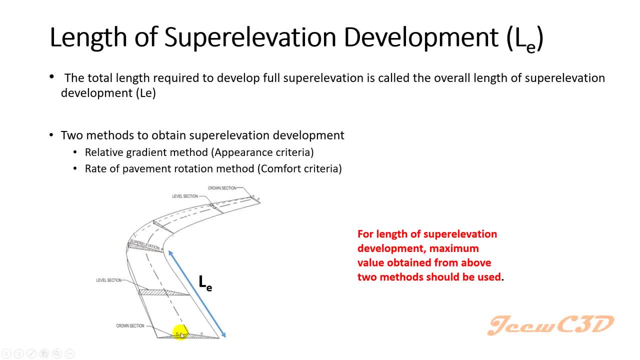 inside the curve. so you can see, along this length this left side is turned upward. along this length this left side is turned upward or rotate upward to get the required superelevation. so from the start of rotation to stop of the complete rotation, there is some distance. 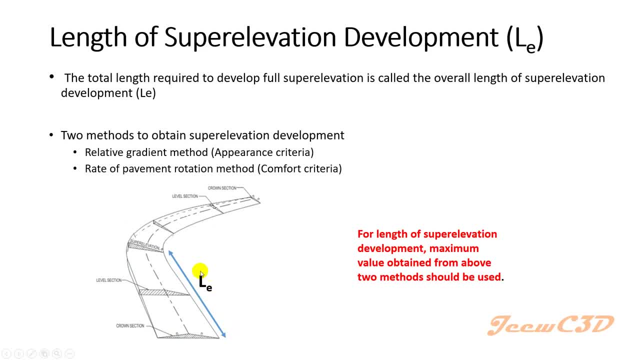 along the road. we call it the superelevation development length. this length can be calculated by two methods according to earlier design guidelines. they are relative gradient method and rate of payment rotation method. so this relative gradient method is depends or is designed or defined by considering the appearance criteria. 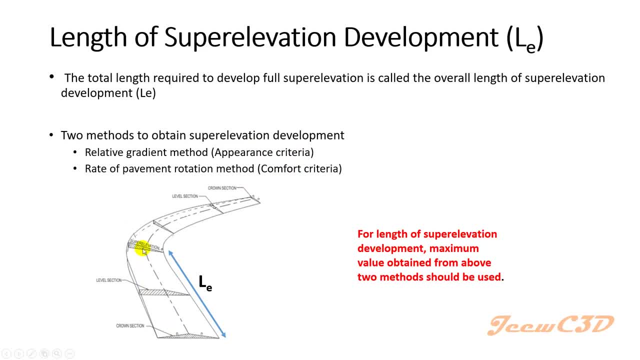 That means this rotation is taken place with some distance, If this distance is very low. so the driver see that within a short period or short length of road the pavement is rotated. the driver see, So in that case the appearance criteria is not good. 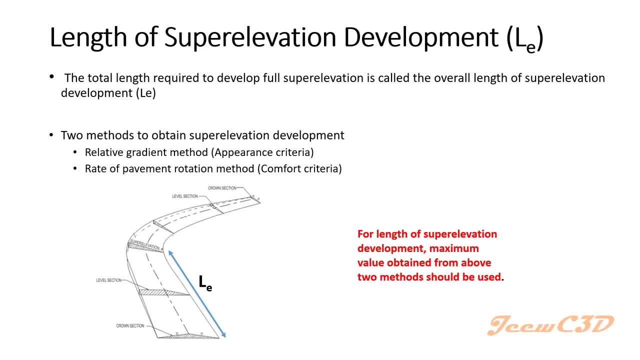 In other case about the comfort criteria. you have the rate of pavement rotation. If this pavement is rotated and come to full super elevation in a small length or a very lesser length, the driver feels that when he is driving in the curve, suddenly the pavement 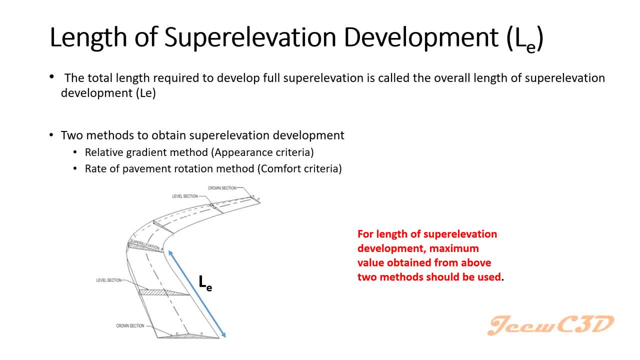 rotates Suddenly. the pavement rotates When the road slope changes. it feels to the drivers and the people inside the vehicle. So in that case your comfort criteria is not satisfied. So there are two methods to calculate the super elevation development length so that you can get the relative gradient method with appearance criteria and rate of pavement rotation. 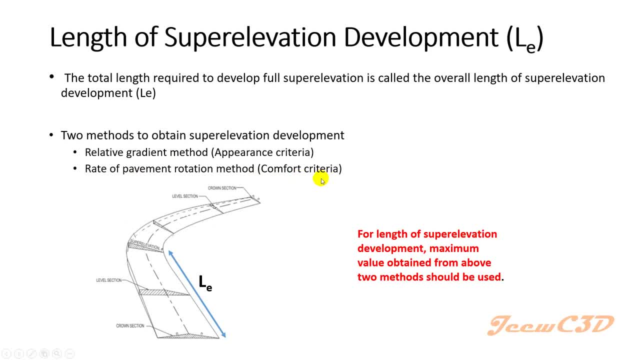 with comfort criteria. So when you are calculating the super elevation development length, you have to calculate the rate of pavement rotation, Then how to calculate super elevation development length. Finally, you will need to calculate for both of these methods and get the maximum value from these two methods. 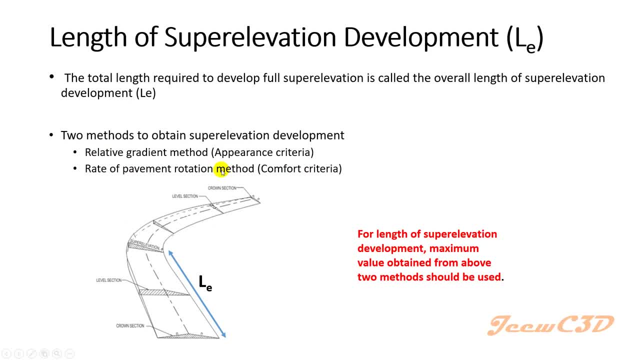 So when you get the maximum value, it will satisfy both these criteria. So that is how to get the super elevation development length, Actually how we calculate the super elevation development length. Now we are going to see the right way, see the equation to calculate this super elevation development length. so 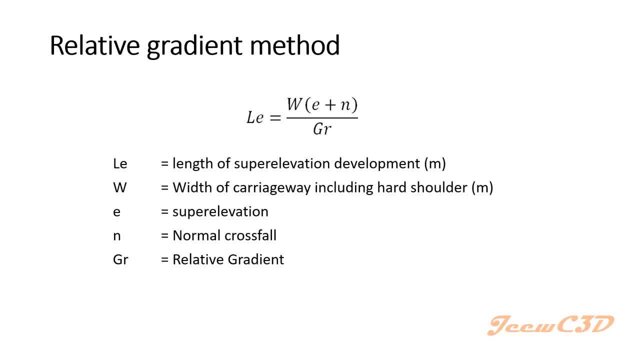 first we will look at the relative gradient method. so this is the equation for relative gradient method. it is given as L e, which is the super elevation development length, equals W into e plus n over gr. so L e means super elevation development length. as I told you earlier, W means width of the carriageway. 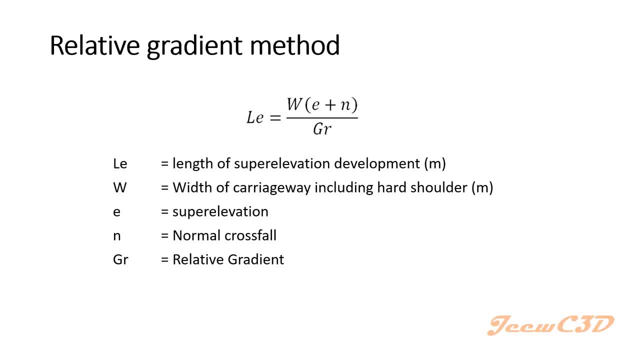 including hard shoulder. so if you can remember the lecture we told about the cross section of the roadway, I told you carriageway and what is carriageway and what is lane width and what is hard shoulder. so this W means lane width plus heart shoulder width. usually the correct way to get this would be the lane width. 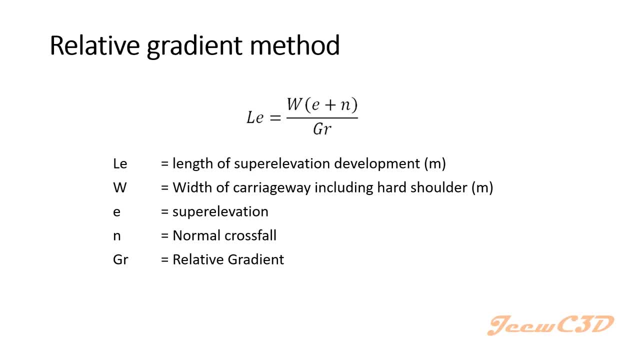 W is usually considered as lane width, but in Sri Lanka we use both lane width and heart shoulder width for W. so that means W equals addition of lane width and heart shoulder width. so E means the super elevation of the curve and N means the normal cross fall. so E plus N means, without considering this, E plus N part. 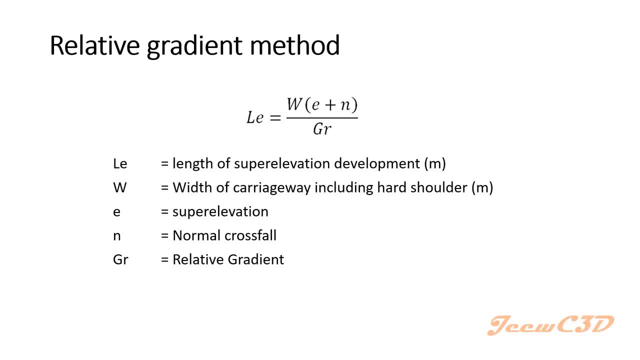 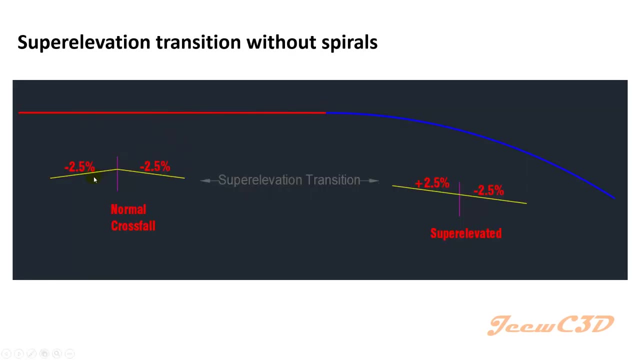 what actually happens is how much of a rotation has happened inside the curve. that means, if I go back to this previous slide, here actually the rotation is happening on the left side. right side is fixed, so what? how much? from how much a change is happening on the left side? that is meant. 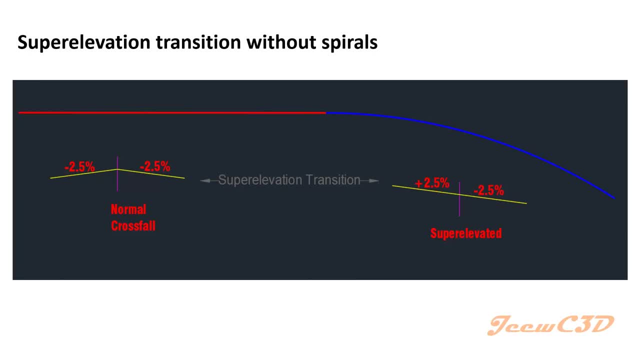 by the E plus N term. E plus N means minus 2.5 to plus 2.5. how much change from minus 2.5 to plus 2.5? that's what we are going to see in the next slide. that change is 5, so E plus N equals 5. that is how to get that easily without. 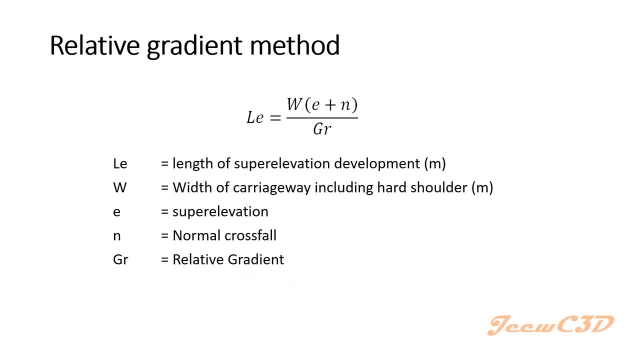 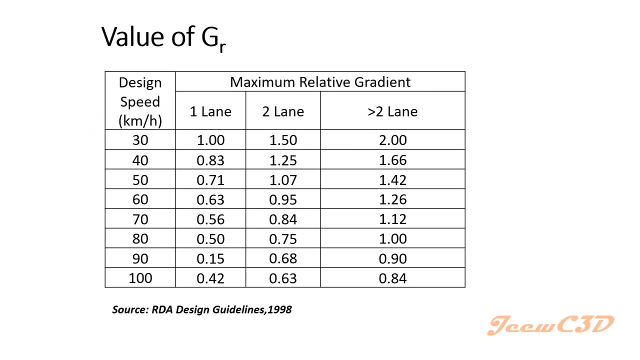 considering those, this E plus N term. you just think from how much the payment values change. that is the easiest way. then there is a factor called relative gradient, and it should be obtained using the relative gradient table. so if you have one lane which is rotating, that means 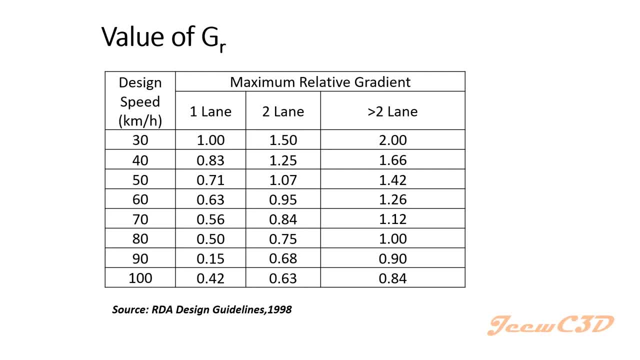 if there is. if there is a two-lane road, each lane would be rotated separately. so you have to use this equal, use this column to get the GR value. if you are designing for 50 kilometers per hour and if it is a two-lane road, you should take 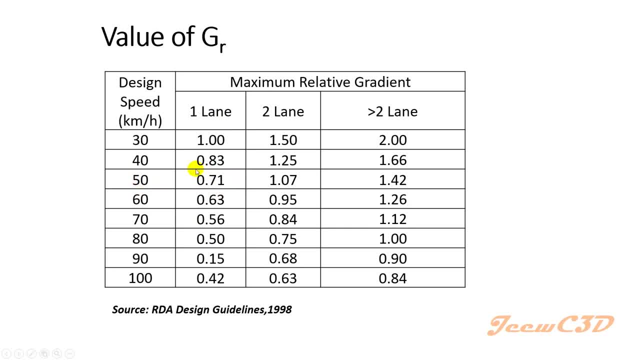 0.671 as GR. so if it is a four-lane road, two lanes would be rotated in one side. you have to learn use this two lane columns. if their lanes number of lanes are more than four lane, you have to use use this column actually. 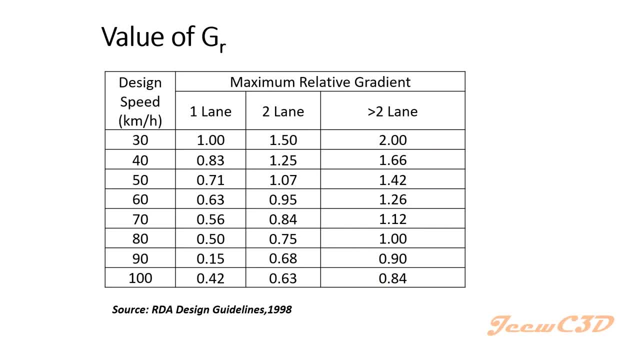 if the road is as single real or one-way road, that's the number of lanes greater than 2, you would have to reduce this column with the number of lanes. number of planes greater than one or equals to two, you have to use this column if it is the one-way rule. so it depends on the rotation lanes in the 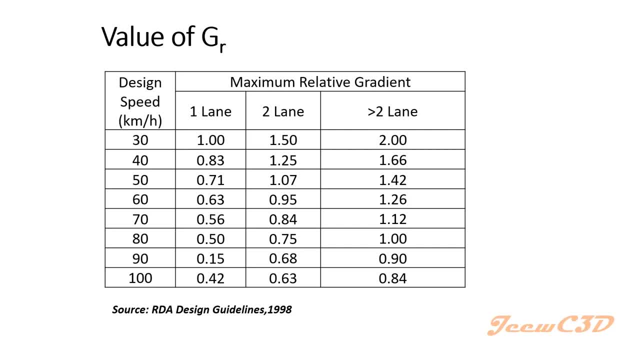 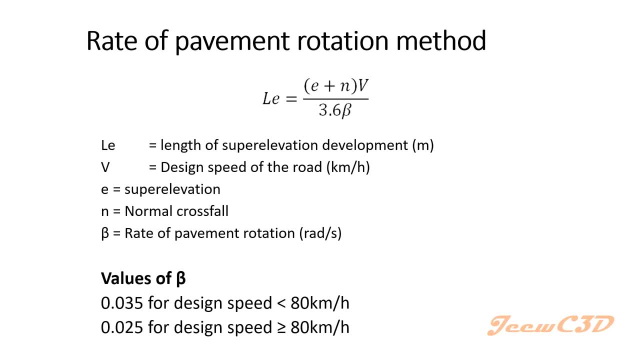 actual scenario. so that is how to get the GR value. now we are moving on to the other method, which is the rate of payment quotation method. in that method we are defining the super elevation development length as L? e equals e plus n into V over 3.6 beta. so L e is the length of super elevation development. 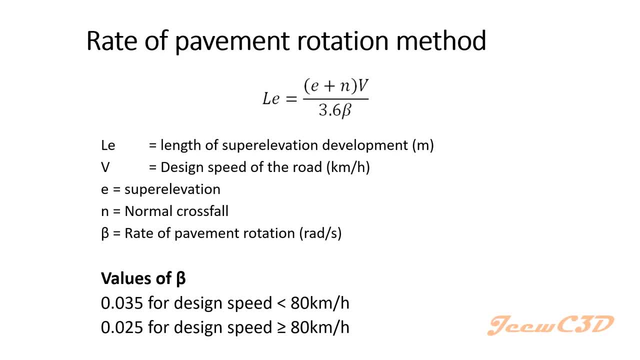 length e plus n term. as I told you earlier, it implies how much of change in the super elevation occurs in this transition or in this super elevation development length. so it is the same thing we learned in the relative gradient criteria. then V is the design speed of. 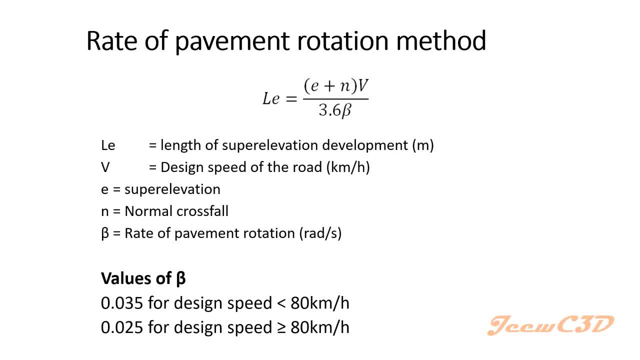 the road in kilometers per hour, then beta factor depends on the design speed of the road. so if your design speed is less than 80 kilometers per hour, your beta value should be 0.035. if your design speed is greater than 80 kilometers per hour, or equal to 80 kilometers per hour, you have to use 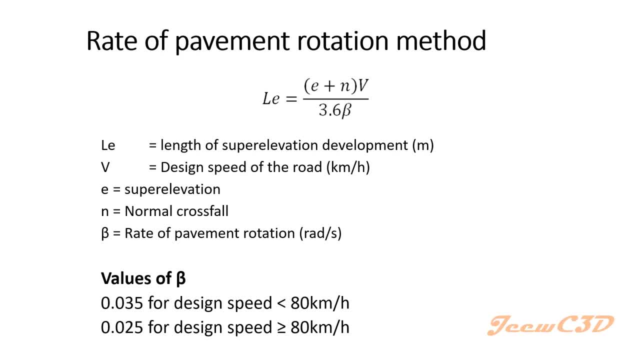 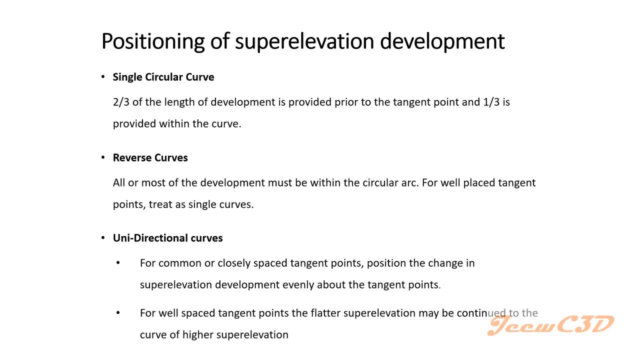 the beta value as 0.025, then we have something called positioning of super elevation development length. so up to this point we have learned what is the super elevation development length we need to get to rotate this payment or rotate the road to achieve the super elevation from normal cross fall to a. 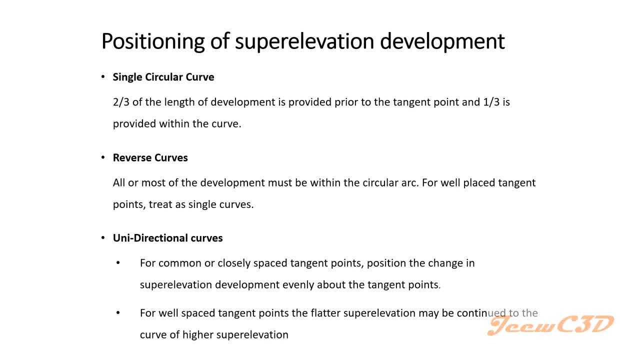 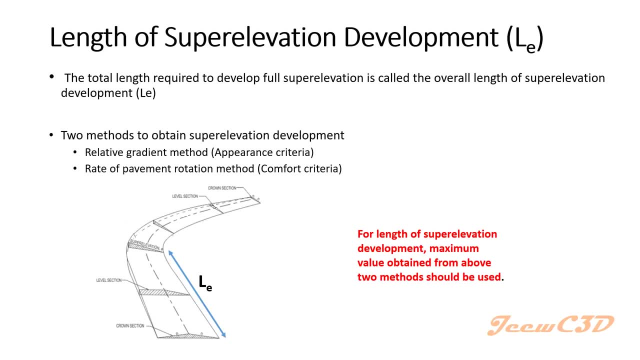 value of some kind of super elevation. so if I move back to this slide- you know this super elevation development length- then there is a thing we have to consider. that is where we need to place this length of super elevation development length, because there is a straight portion and there is a curved portion, so we need to 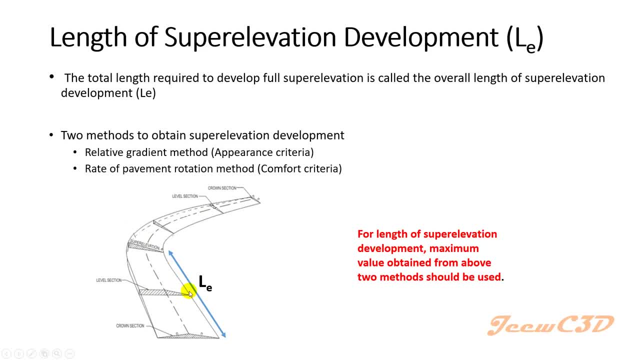 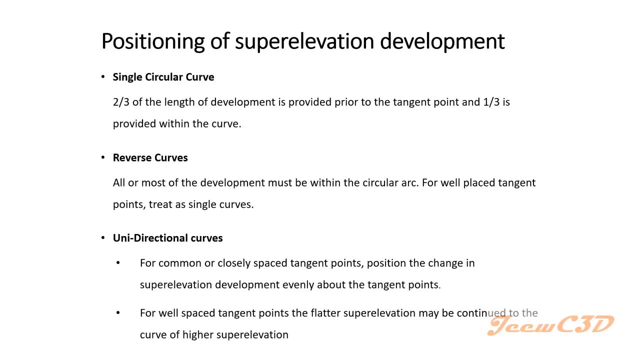 know whether we put this all LE length. that means whether we rotate this total payment within the straight section or within the curved section, or some part of in the straight section and some part in the curved section. so we have something called positioning of super elevation development length. 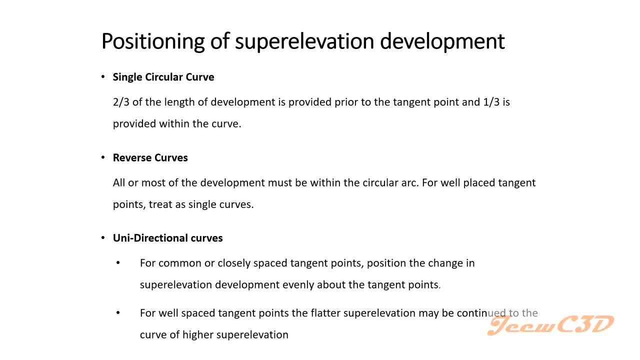 so positioning of super elevation development means on curve, how much we put the super elevation length on straight, how much we put the super elevation development length. so here we have three definitions how to distribute super elevation development length among each entity. so in this lesson we learned that 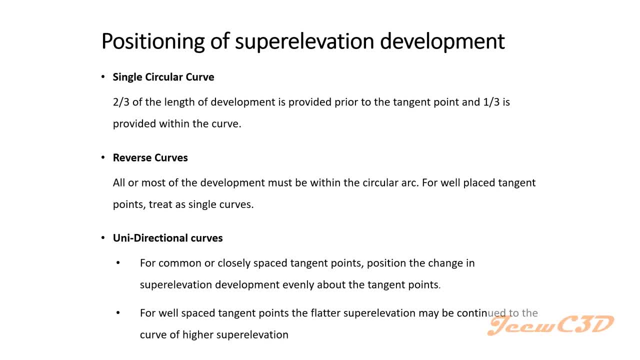 we have single circular curves, reverse curves and unidirectional curves. I have to mention that unidirectional curves we have to avoid as much as possible. that are, they are not desirable for alignment designers there. if any case, if you cannot avoid unidirectional curve, you can use 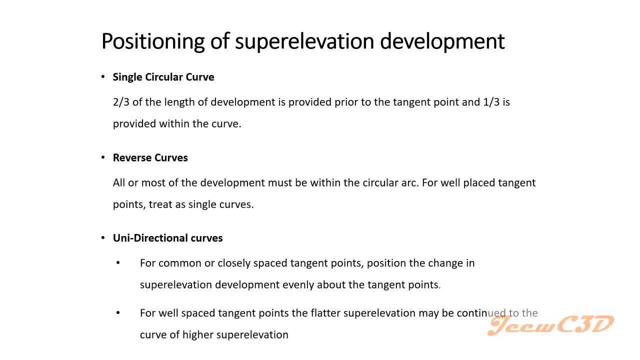 them, otherwise you have to avoid them as far as you could. so first we will look at how to distribute super elevation development lengths, or position of super elevation development length, along a single circular curve. so in a single circular curve it says two third of length of super elevation development lengths. it is to be provided prior to. 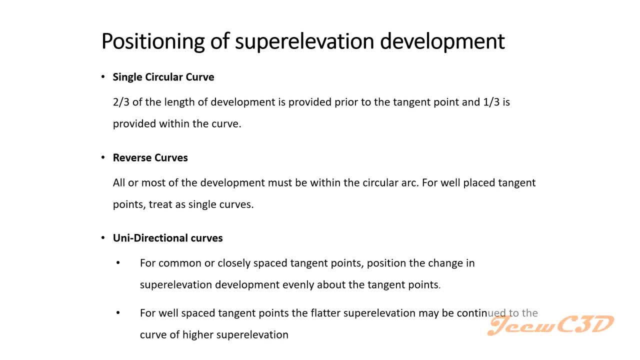 the tangent point and one-third of the super elevation development length should be position within the curve. so these are RDA guidelines. this is given in the RDA guidelines guidelines. so in other guidelines, such as as to show, they have some other definitions, but this one is related to our lead design guidelines. so it says: 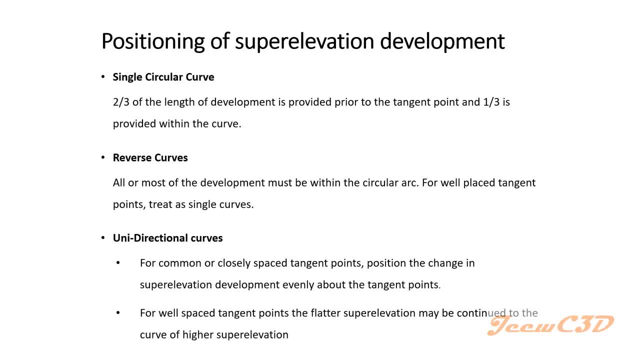 the development length should be to. third should be on the tangent and one third should be on the curve. so if your super elevation development length is 30, if it is a simple curve or a single circular curve, your 20 meter length would be on the tangent side and the 10 meter would be on the curve side. in this, 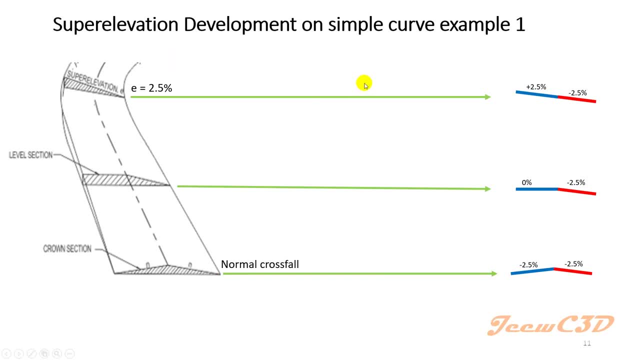 example, we assume this is a simple curve. so if I recall, what is a simple curve? simple curve means a curve where you have two sides connected to a large, larger straight section. that means before the curve you have a larger straight and after the curve also, you have a larger. 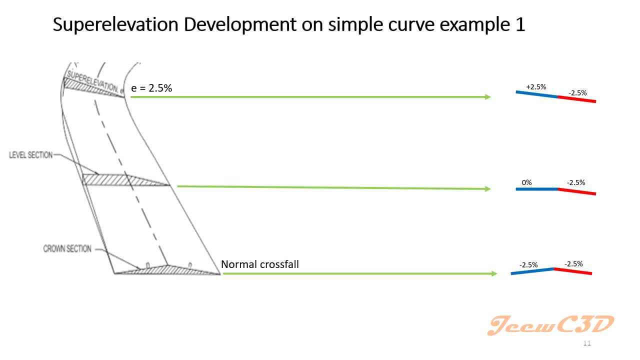 straight section or a lengthy straight section. sometimes, instead of a straight section you may have a very large radius curve, such as 2,000, 1,000 or something like that. it depends on the design speed. so whatever the curve radius which is greater than the adverse cross fall would be a larger radius curve. so we 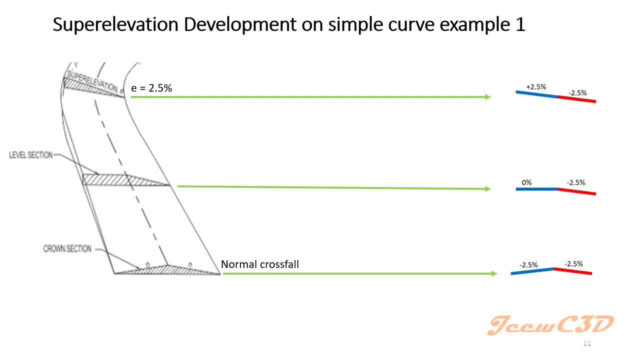 will be learning this in later super elevation lecture notes within civil 3d software section. so in this example now we have a simple curve, so assume this is a straight and you have a curve here. so in the straight section you have normal cross fall minus 2.5 both sides this blue. 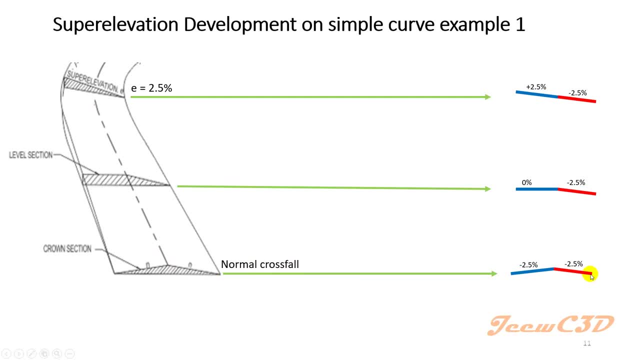 color represent the left side, red color represent the right side. so when the super elevation occurs at the, when you, when the super elevation or inclination of the road becomes 2.5 at the curve, your left side would be rotated up to plus 2.5. 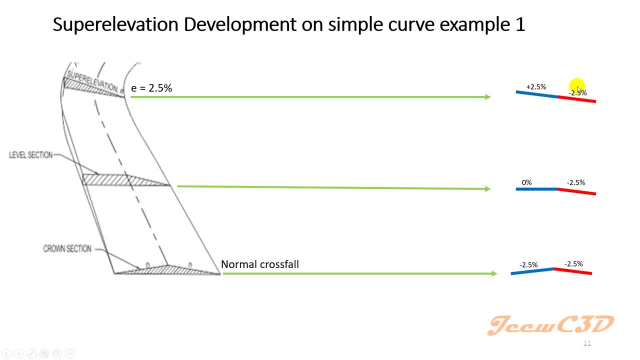 super elevation, but your right side would be remain as minus 2.5. so in this example you can see your left side is always minus 2.5, but your right side is. with the length it will be rotated up to plus 2 plus 2.5 from minus 2.5. so in this 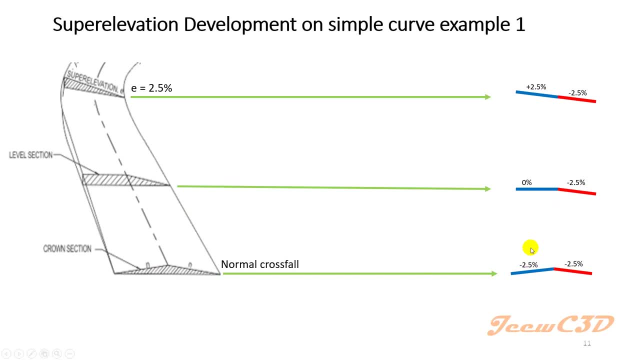 development. sometimes you will find a situation where you have a flat crown or a level section in this left side end. it like it is gradually increasing up to plus 2.5. so that is how this super elevation is developed, along this simple curve. so the positioning of super elevation would be from this length from: 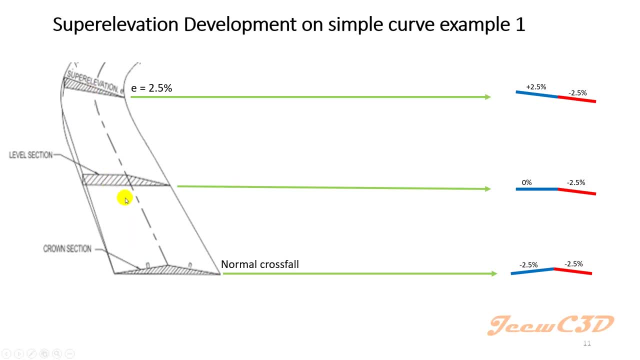 this super elevation development length. two-thirds of this length would be on the section and one-third would be on the straight section. that is the definition for simple curve. so we will look at another example related to simple curve. this time you have normal cross fall and once you get the super variation, your 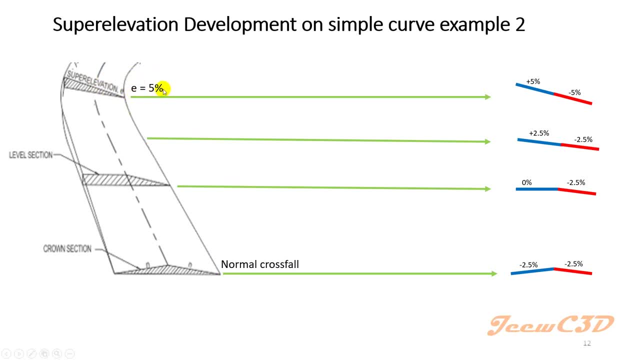 value would be plus 5. so that is kind of a sharper curve. so your left side would be minus 2.5 and it could be rotated up to plus 5 and your right side is going from minus 2.5 to minus 5. so if you think about the change here right left- 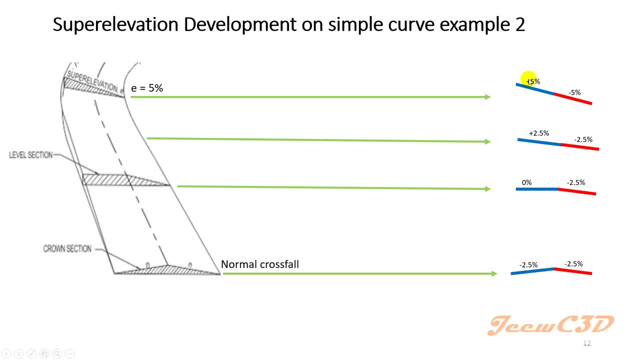 side would be changing from minus 2.5 to plus 5. so when you calculate in the superannuation development lane, always you have to select the largest change. so in this case you can see left side is from minus 2.5 to plus 5 and right side is minus 2.5 to. 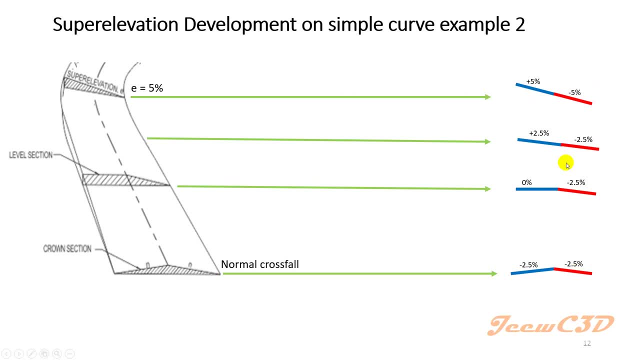 minus 5. this change is only minus 2.5, but this change is 7.5. so when you calculate the superannuation development lane, you have to take this e plus n term as 7.5 according to the superannuation development equations. so now 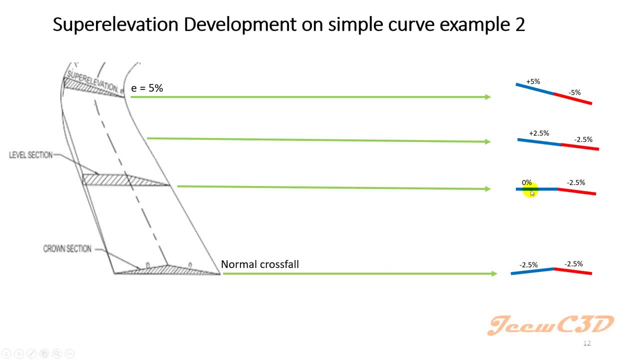 there is now. you can look at how this is developed. so in the normal cross fold you have minus 2.5 and minus 2.5 there will be then with the. with some distance this left side increases but the right sides remain as same and advanced instance. both the side become plus 2, minus 2.5. 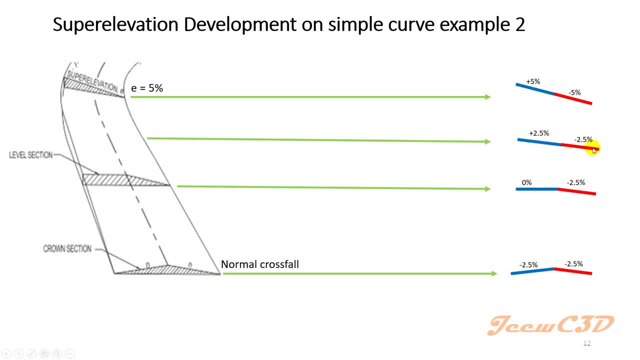 and plus 2.5. that means same super elevation but different values: minus 2.5 and plus 2.5. in this location we call this reverse crown. both super elevations are equal, but the sign is different. so after this point both sides of the road will be rotated up to the required. 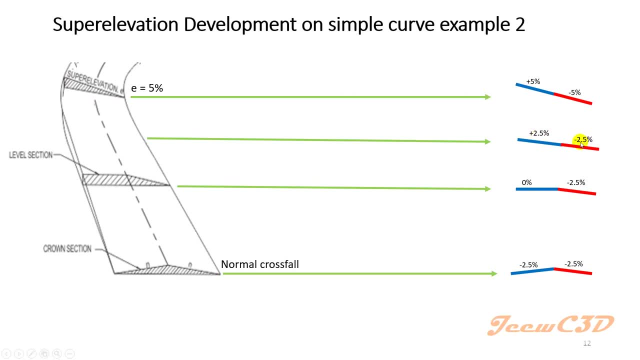 super elevation from this point. this one would be rotated to minus 5. this one would be rotated to plus 5. that is how we get it. so that is how the super elevation is developed, developed inside the curves, in in the same manner as i told you earlier. the super elevation 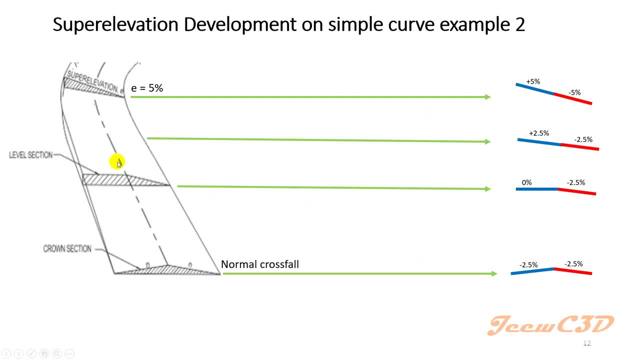 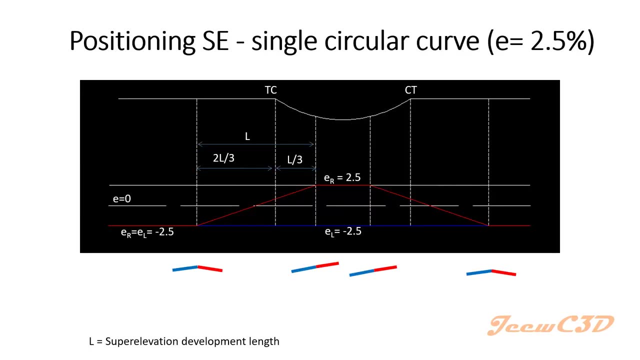 development plane would be placed two-thirds along the straight and one-third along the curve. so this is another way of representing the super elevation development. so this is your curve. this is a simple curve. they are: e equals 2.5. the super elevation is 2.5, as in example 1. 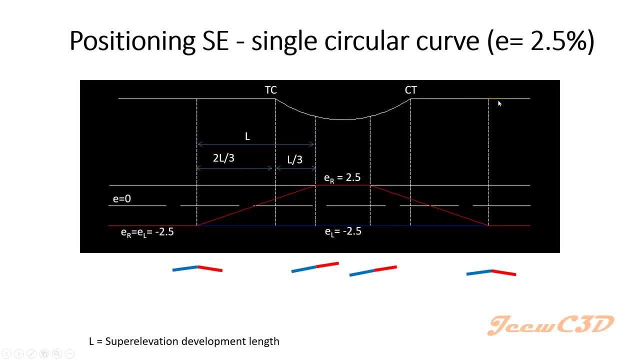 so this is a curve. this is a straight, this is a curve. this pc means tangent to curve point. this is tangent, this is curve. this is tangent to curve point. ct means curve to tangent point. this is the curve, this is the tangent. so inside curve you have super elevated section and from this super elevation development. 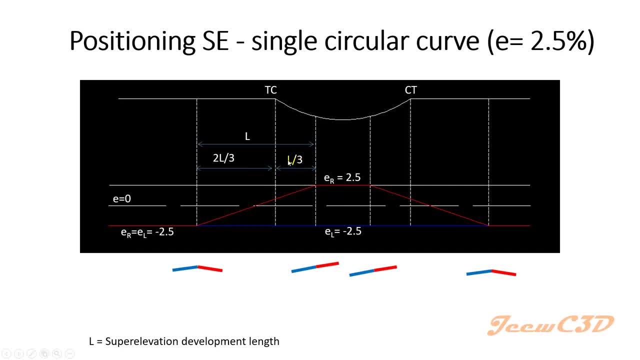 one-third. this l is the super elevation development length. so l over 2 will be inside the curve. 2, l over 3 will be outside the curve for the straight section. if you think about the super elevation at each section, at the start you have the normal crown. 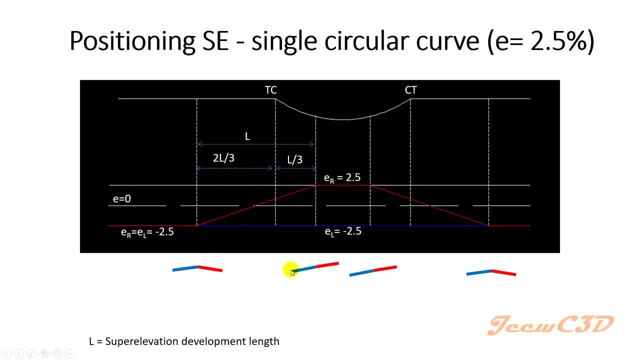 in this position you have the full super elevation. so if you consider the other side of the road, other side of the curve, it has the same thing: you have full super elevation up to this point. so in this red color means the right side, right side is going upward. so that is why. 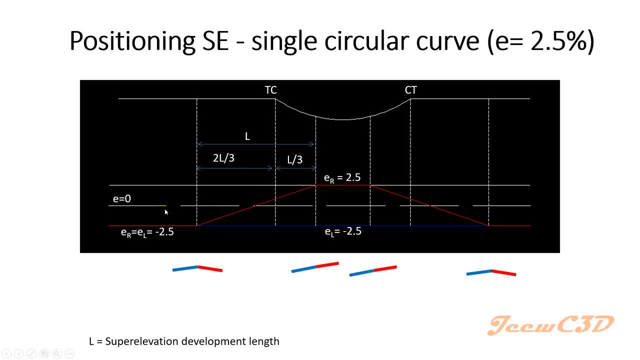 equal it. it is going upward. this is the e equals zero right. super elevation equals zero line. so this is super elevation equals plus two point five: this is super elevation equals minus 2.5. so after this point, within this curve plus 2.5 will be continued. so after: 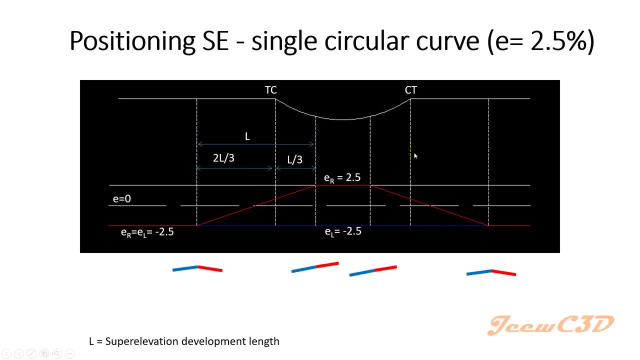 at the end of this curve you will have the same super elevation development as this one. if this is a simple curve, so we will position that super elevation development length l by l over 3 and 2 l over 3, as in the a start of the curve. so you will be having same super elevation develop content same. 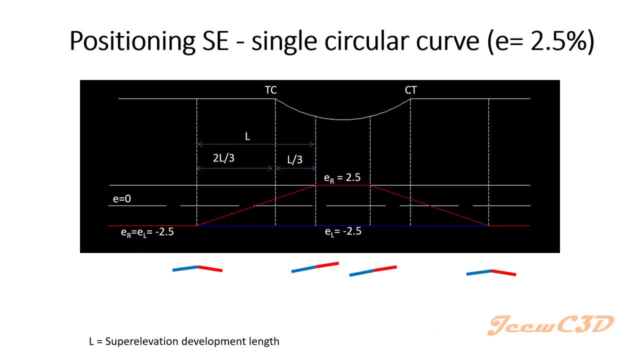 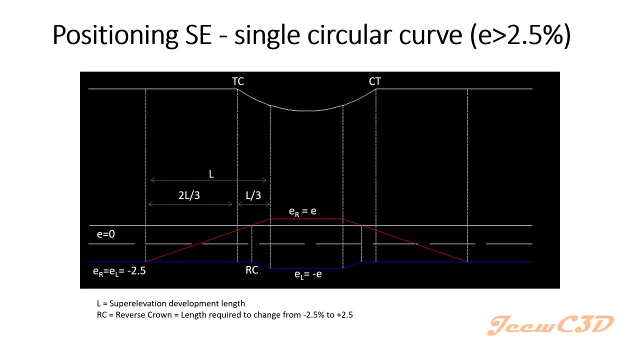 pavement rotation within that single circular curve. so that is how to position super elevation development length within a single circular curve. so in this, yeah, you have the super elevation development length greater than 2.5. in this case we call this point the reverse crown location. this 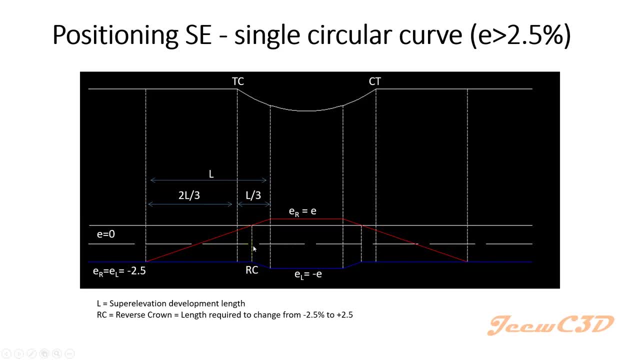 is the location where you have minus 2.5 and plus 2.5. so after this point, both side would be rotated. so from minus 2.5 to plus 2.5 your right side would be coming like this: but until this plus 2.5 point, left side would be always minus 2.5. 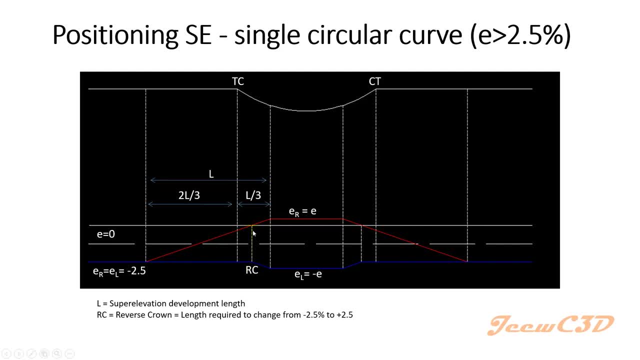 after that, both this pavement rotates, both sides rotates, and go to the required super elevation. you remember the last example. this value should be plus 5 and minus 5 according to that example. so your development length should be divided according to the single circular curve. so this is how to develop super elevation. 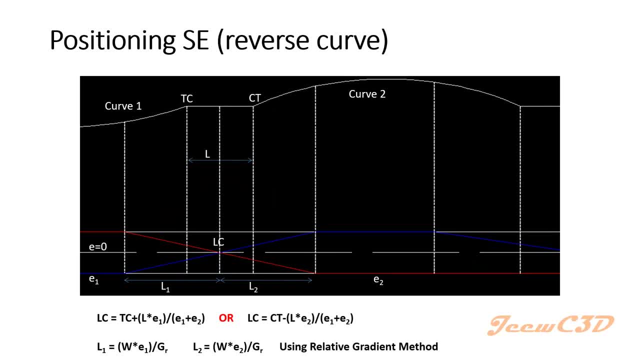 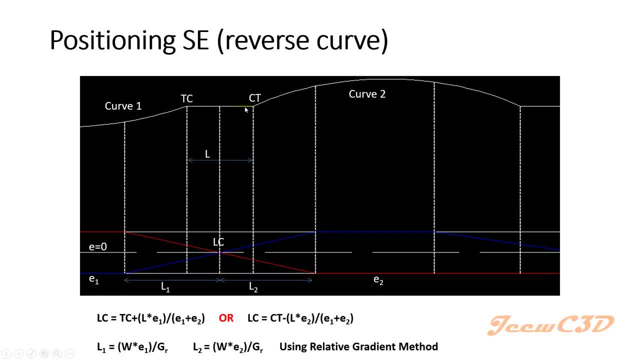 like this: and you have tangent to curve point, then you have a small straight point, then you have a small straight point, then you have a small straight, then you have a curve to tangent point, then you have a curve to tangent point, then you have a curve to tangent point and you have another curve. but that 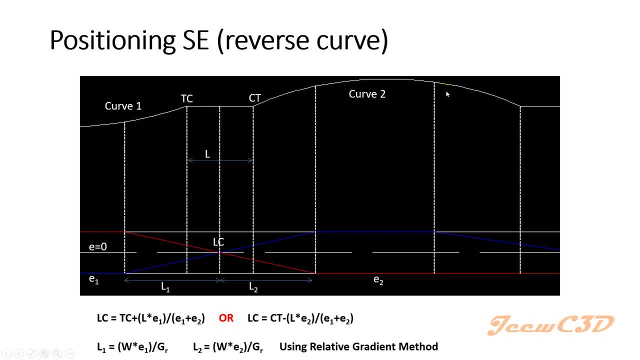 and you have another curve but that, and you have another curve, but that curve is in the other direction. so, since curve is in the other direction, so since curve is in the other direction, so since this is a curve, this has a super, this is a curve, this has a super. 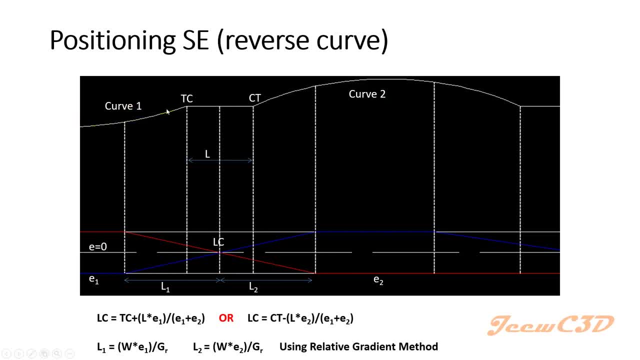 this is a curve. this has a super elevation. so this is going on the left elevation. so this is going on the left elevation. so this is going on the left side. is the anti-clockwise direction side. is the anti-clockwise direction side. is the anti-clockwise direction curve. you call it anti-clockwise direction. 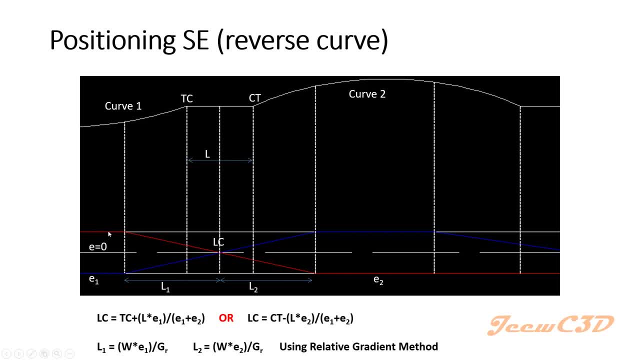 curve. you call it anti-clockwise direction. curve. you call it anti-clockwise direction. so your right side would be at a. so your right side would be at a. so your right side would be at a plus-super elevation. left side would be plus-super elevation. left side would be. 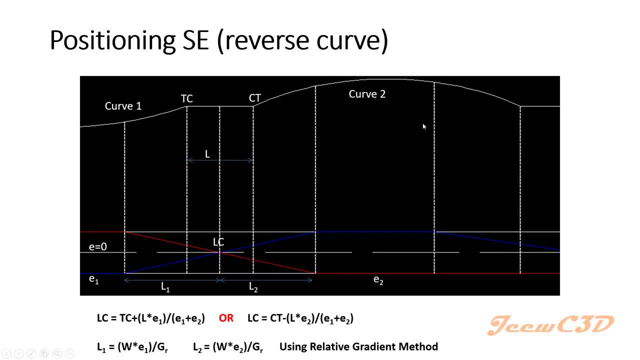 plus-super elevation. left side would be at a minus super elevation, then on the at a minus super elevation, then on the at a minus super elevation, then on the other curve, it is a clockwise curve. your other curve: it is a clockwise curve. your other curve it is a clockwise curve. your left side it is at a plus super. 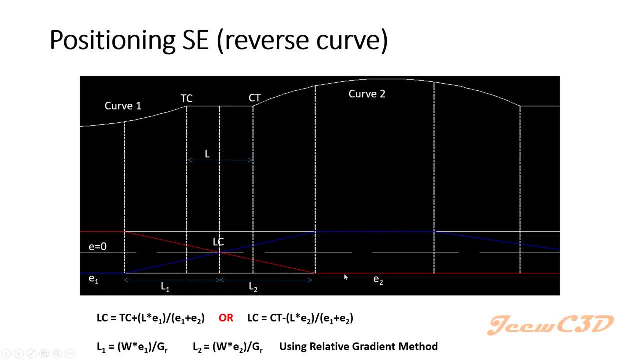 left side it is at a plus super left side it is at a plus super elevation and elevation and elevation and right side would be at a minus super right side would be at a minus super right side would be at a minus super elevation. so in that case you have to. 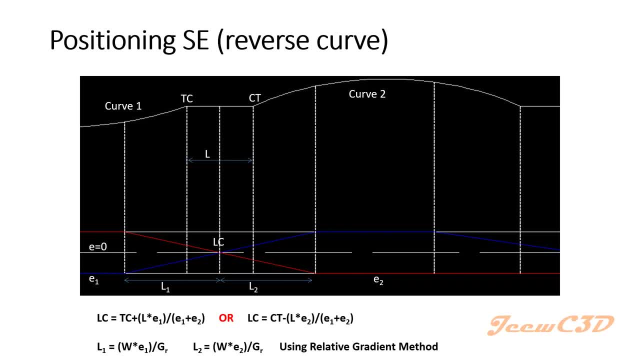 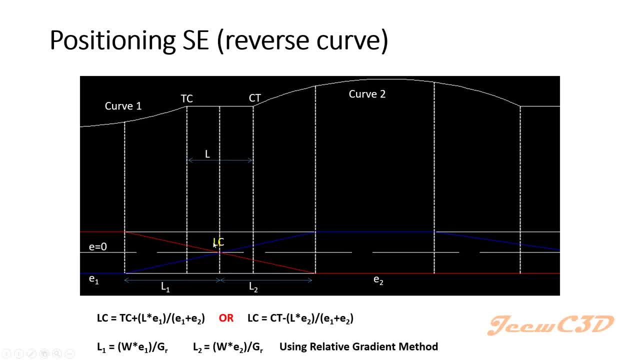 super elevation, zero point. we call it level crown. this point is called lc level crown. this point is called lc level crown. this point is called lc first. you need to find that one that is first. you need to find that one that is first. you need to find that one that is uh. 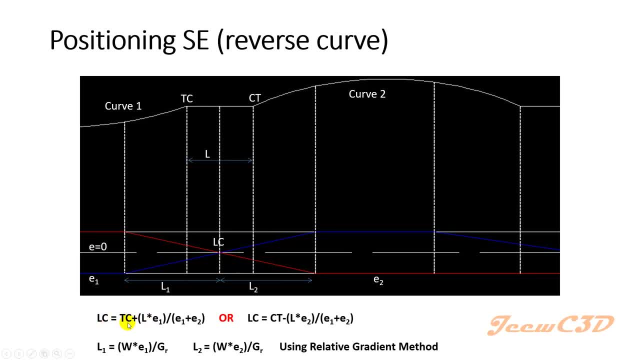 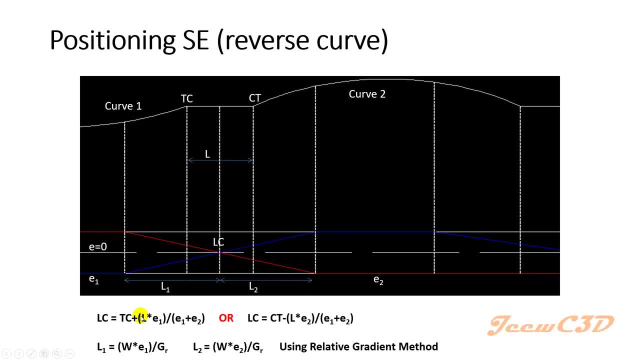 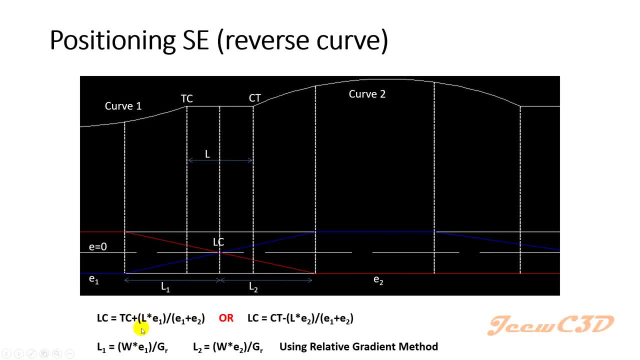 l e1 over e1 plus e2. this l is same as this. l is same as this, l is same as this. l uh this, l uh this, l uh this, uh this. l is same as this, uh this. l is same as this, uh this. l is same as this short, tangent length. so 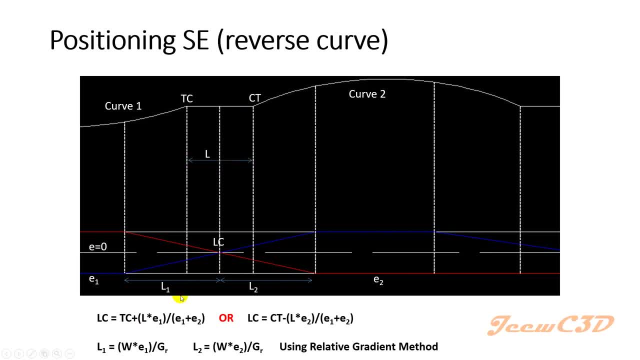 this short tangent length. so this short tangent length. so this short, short tangent length, this short, short tangent length, this short, short tangent length: l l. this short, short tangent length l. e1 means the super elevation of this. e1 means the super elevation of this. e1 means the super elevation of this curve. e2 means the super elevation of. 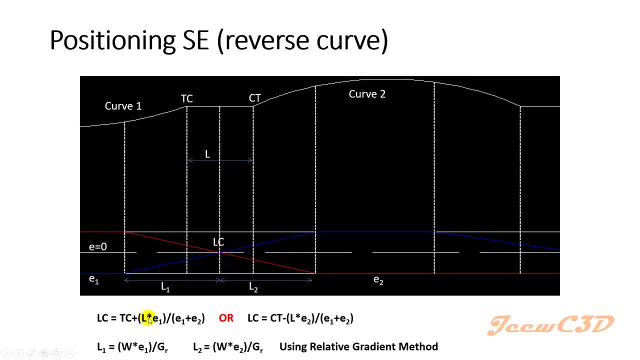 curve e2 means the super elevation of curve. e2 means the super elevation of this curve. so we will proportionately this curve, so we will proportionately this curve, so we will proportionately, uh uh uh, distribute the super elevation, distribute the super elevation, distribute the super elevation throughout this length. that is how to. 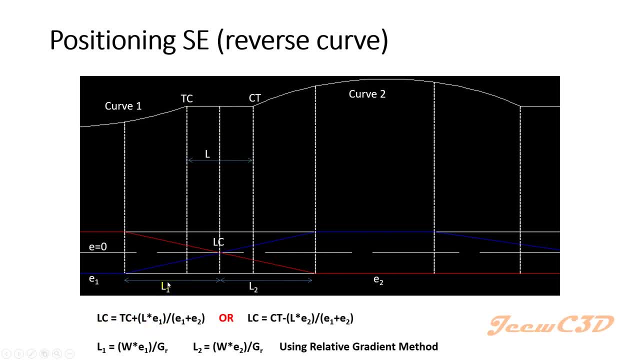 throughout this length. that is how to throughout this length. that is how to get this, get this, get this lc point, so lc point, so lc point. so, after getting a c point, you will be after getting a c point, you will be after getting a c point, you will be finding the. 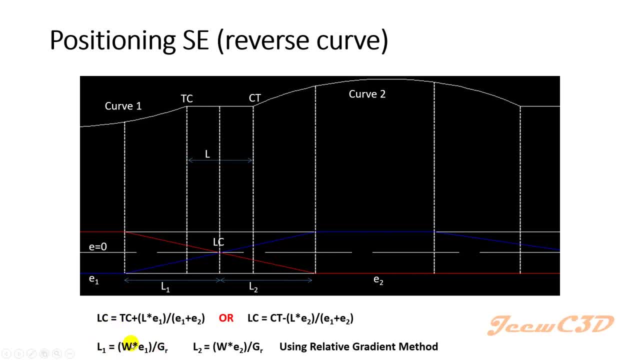 finding the finding the l1 and l2, but you need the l1. without finding this point, you can, without finding this point, you can, without finding this point, you can calculate l1 and l2. l1 means the super. calculate l1 and l2. l1 means the super. 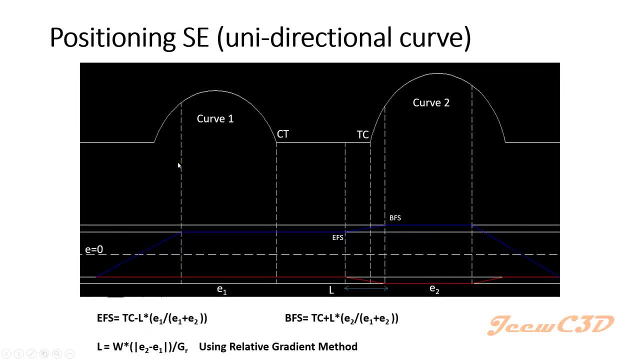 calculate l1 and l2: l1 means the super elevation of elevation of elevation of super elevation, development length of super elevation. development length of super elevation, development length of this curve and l2 is super elevation. this curve and l2 is super elevation. this curve and l2 is super elevation development length of. 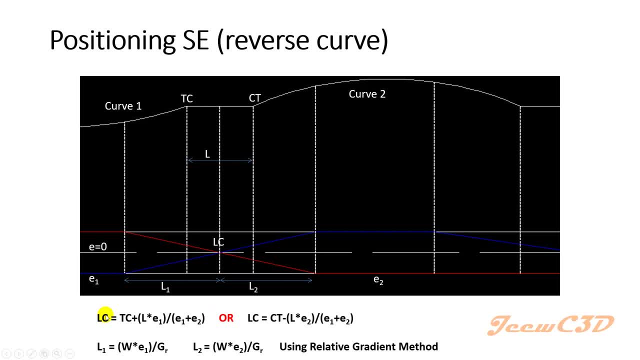 development. length of development, length of this curve, this lc point would be needed. this curve, this lc point would be needed. this curve, this lc point would be needed to distribute the super elevation, to distribute the super elevation, to distribute the super elevation. so we will, uh, we will. 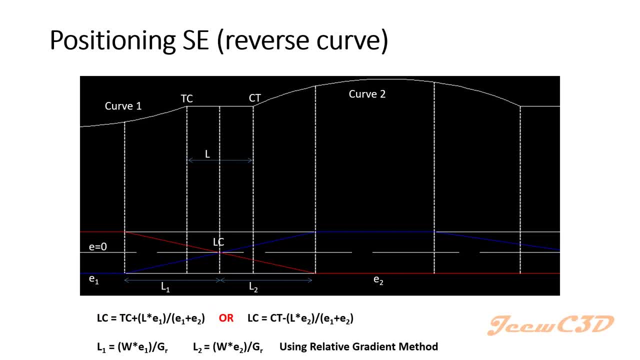 so we will, uh, we will, so we will, uh, we will look at this lc point uh, within the look at this lc point uh, within the look at this lc point uh, within the civil 3d section. how to distribute that civil 3d section. how to distribute that. 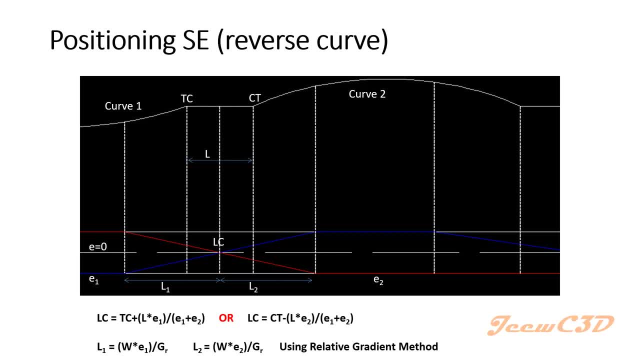 civil, 3d section, how to distribute that one, one one. so now in this, so now in this, so now in this session. we will find how to get this l1 session. we will find how to get this l1 session. we will find how to get this l1 length. l1 length is: 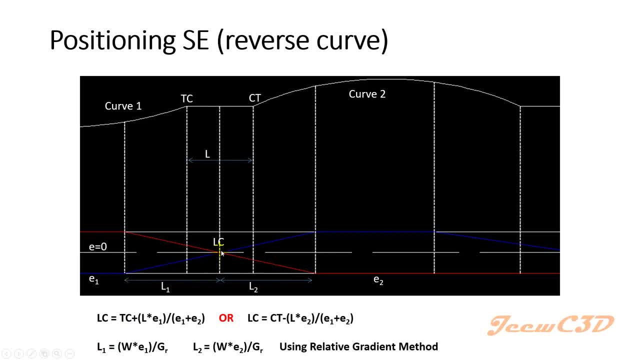 length. l1 length is length. l1 length is this one. after find this, this 11 crown, this one. after find this, this 11 crown, this one, after find this, this 11 crown. you have to, you have to, you have to. uh, get the next point. we'll find the point. 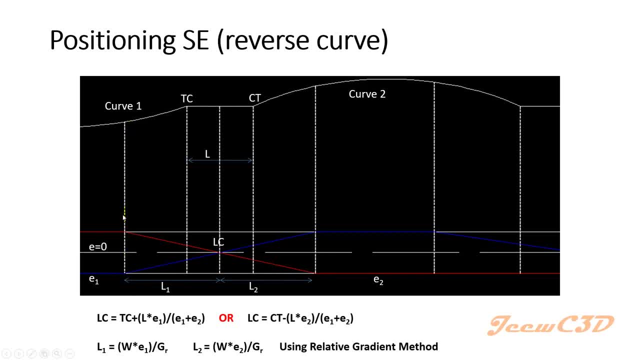 get the next point, we'll find the point. get the next point, we'll find the point. where super elevation change in the, where super elevation change in the, where super elevation change in the curve one from this point it is going. curve one: from this point it is going. 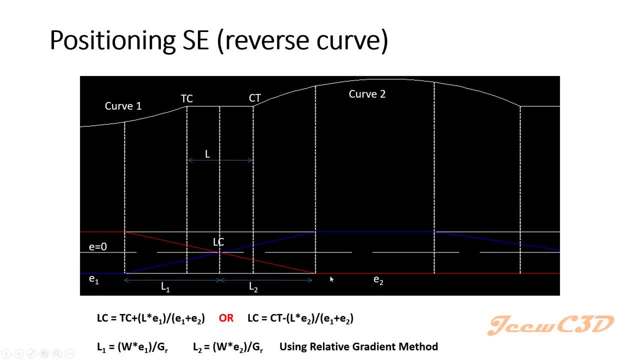 curve one from this point it is going downward, up to the super elevation of downward, up to the super elevation of downward, up to the super elevation of other side, because the right side, other side, because the right side, other side, because the right side super this, this right side super elevation. 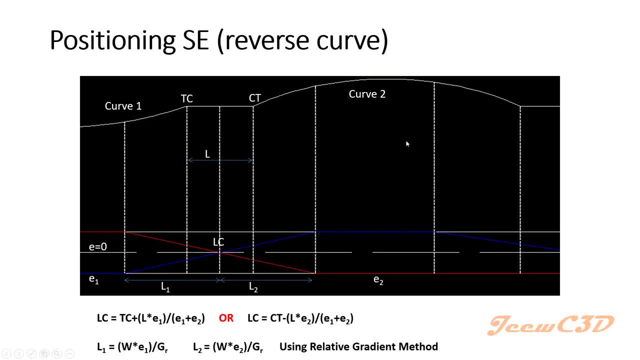 super this, this right side super elevation, super this, this right side super elevation, becomes, becomes, becomes minus on the other curve. so from this minus on the other curve, so from this minus on the other curve, so from this point it will change point, it will change point, it will change and come to this point. so this length, 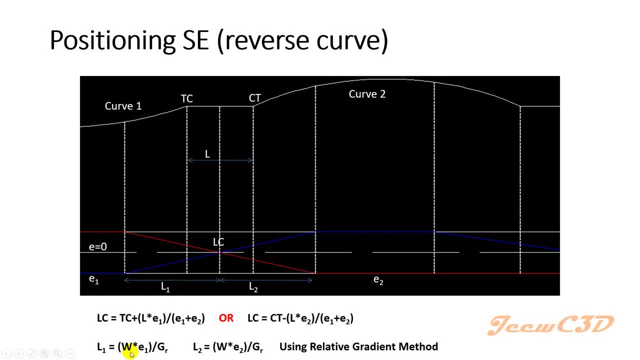 and come to this point, so this length, and come to this point, so this length would be, would be, would be: l1. l1 equals w means the l1. l1 equals w means the lane with just hard shoulder width, and e1 would be the super elevation of this curve and the gr. 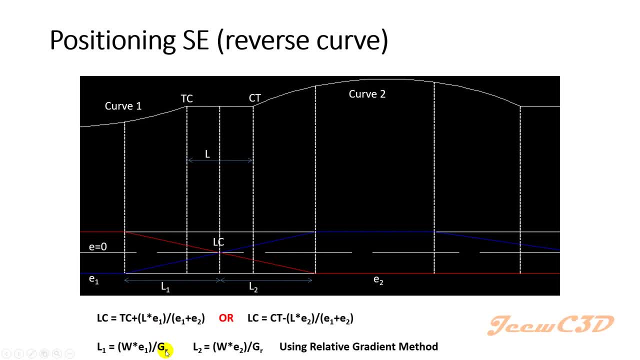 relative gradient and this is only for relative gradient but you have to calculate for rate of time and rotation as well and get the maximum value. so this l2 is for the other curve, so you can find the super elevation development length, this length for this curve, also for this: 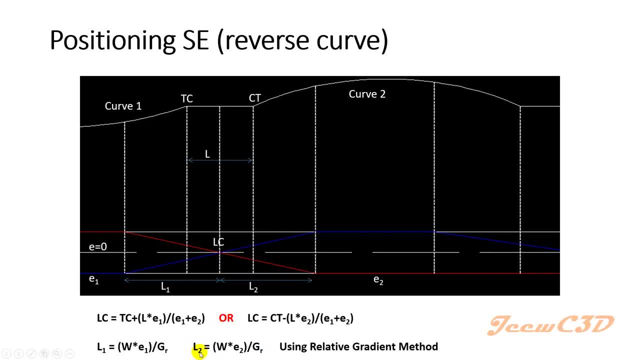 curve, also with l2, same equation, but your super elevation value should be used for the second curve. so that is, that is how to position super elevation in a reverse curve. mainly what we do is position reverse super elevation in between the short tangent. so if this short tangent is zero, 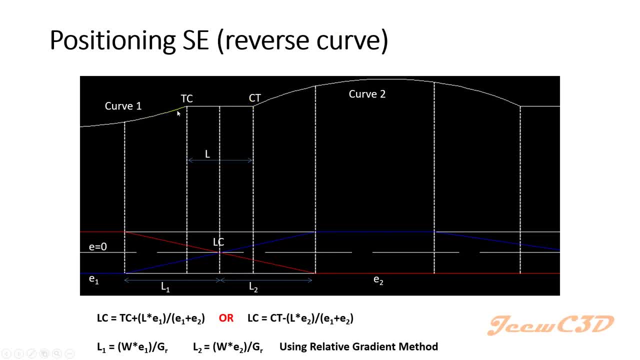 that means after this curve is right after this curve, you will start the other curve. no tangent there. so this pc and t ct point. this length, l becomes zero. so this, in that case, lc equal to tco ct. since this l is zero, lc will be equal to tco ct. so this is how to position, find the 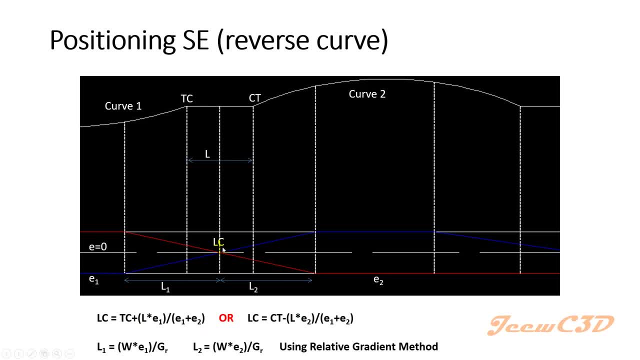 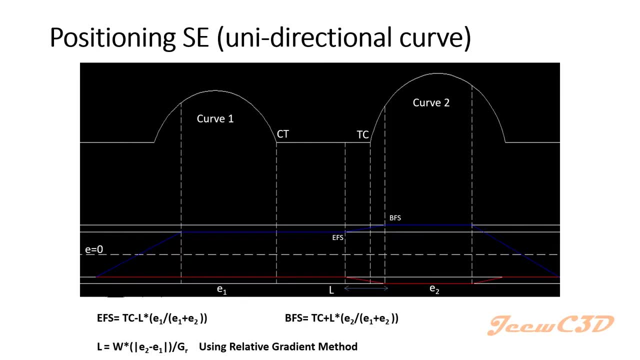 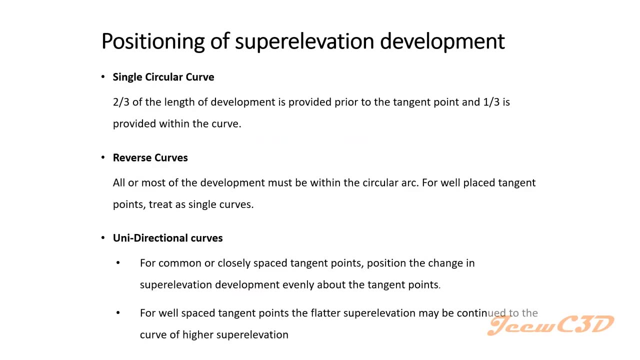 super elevation, zero point for reverse curves, then i have this: uh, unidirectional curves. so if i move back to the presentation here, unit direction, uh for reverse curves. all for more: super elevation: development length must be within circular arc for well-paced, tangent straight as single curves. so this: 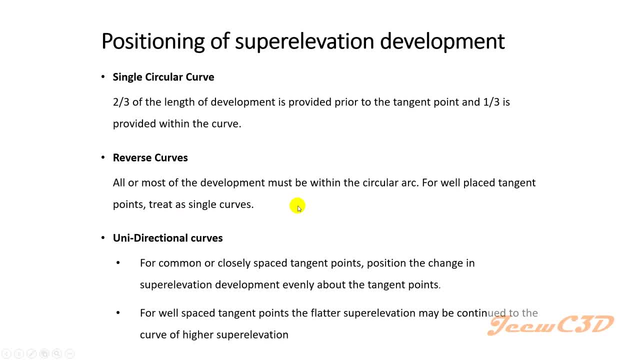 is the same thing i explained a little bit earlier. so this what we have done was this: one has a larger tangent in between two curves. they will be treated as single circular curves, like this case, so unidirectional curves. you have to to place the super elevation in such a way that that for closely spaced tangent points position. 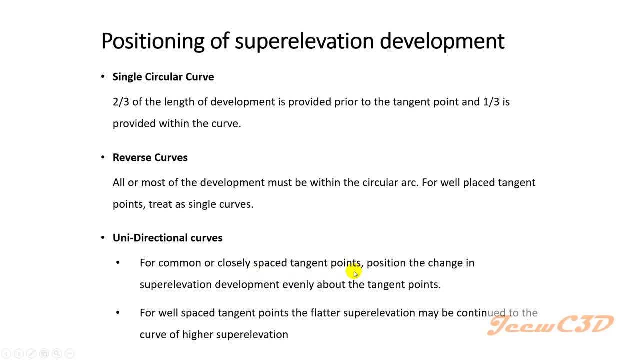 the super elevation plane in evenly above the tangent points, or for well-spaced tangent points, then you have to uh, use the flatter super elevation until the curve of higher super elevation. so i will be teaching this super elevation development in a much better way within the serial 3d class, so we will be looking in more detail inside that. 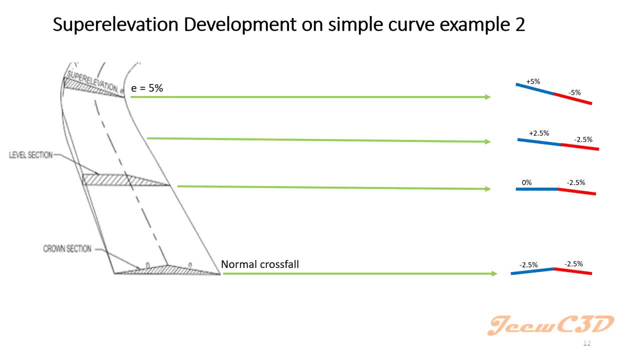 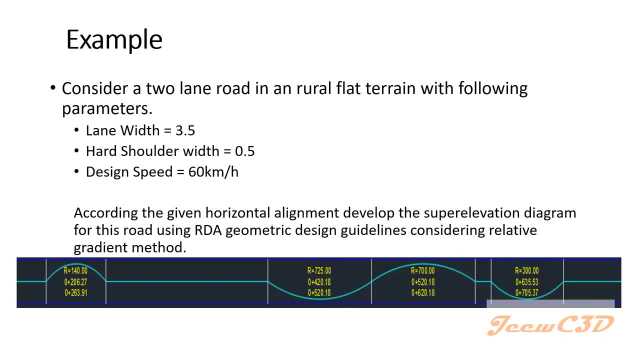 lecture. so after that we will look at an example, simple example, how to calculate the super elevation development length. so in this example we have considered of two lane road in a rural flat terrain with following parameters: equals 3.5 meters. arch holder is 0.5 meter. 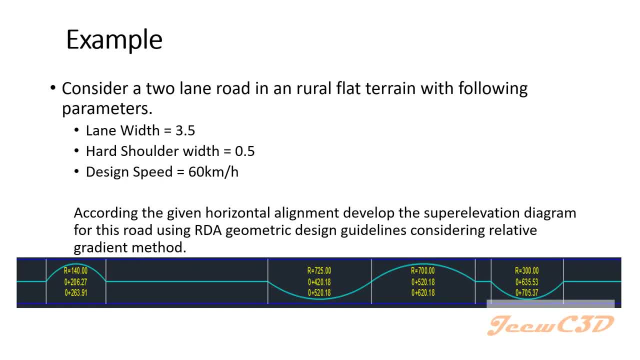 design speed is 60 kilometers per hour according to the given horizontal alignment. develop the super elevation diagram for this using RDA geometric design guidelines, considering the relative gradient method. so we are not going to develop the super elevation diagram, but this example we will be doing, calculating the super elevation development length. so this is. 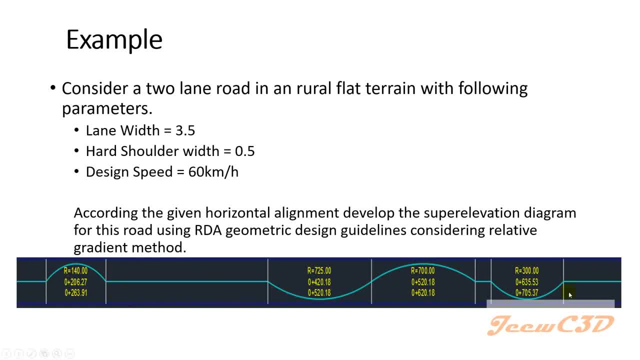 a typical alignment. so what this is saying is: this is a straight section. so this straight section start from 0 and it comes until 206.27. that is the length of this part, and after that point we have a curve, and that curve will be end at 263.91. since, again, you have a long straight section, it will go up to: 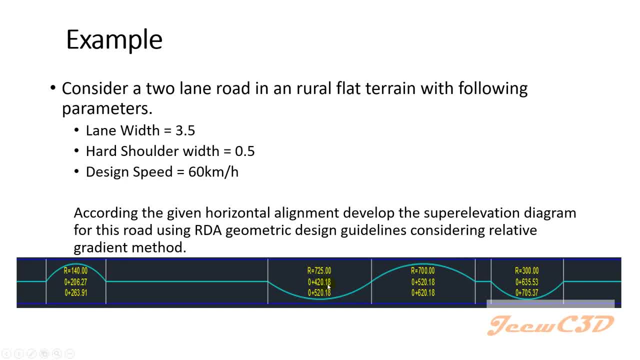 420.18. after that you have a curve of radius 725 that is going up to 520.18. so likewise you have this alignment. so it is us we are asking to develop the super elevation development length. it is saying this is a rural flat. 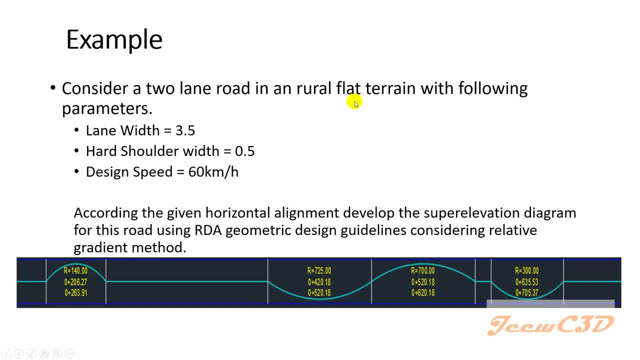 terrain. so since it is a Primal flat terrain, you have to memorize that you can let us see we are going to use. since it is a flat terrain, you can't go super elevation more than 6 percent, that is. that that is more normal is what the RDA guideline says. so since this is a rural area, also, we have larger 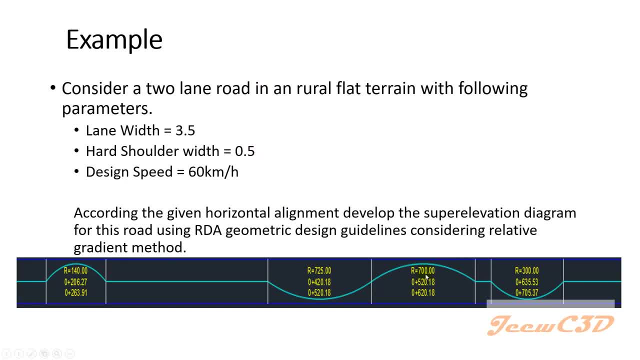 radius curves: 725,, 700 and 300. you need to look at the super elevation and adverse cross fall because of these larger radius curves with rural flat terrain. so first we will look at the radius. in here you have 140,, 725,, 700, 300, so this 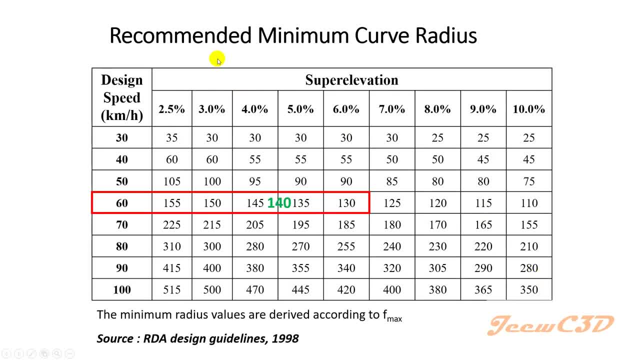 is the recommended minimum radius curves I gave you in the horizontal alignment lecture. so we have our design, speed is 60 and we have radius of 140. that is the lowest radius, so it is in between super elevation and adverse cross fall elevation 4 and 5, so you cannot interpolate and get the super elevation. 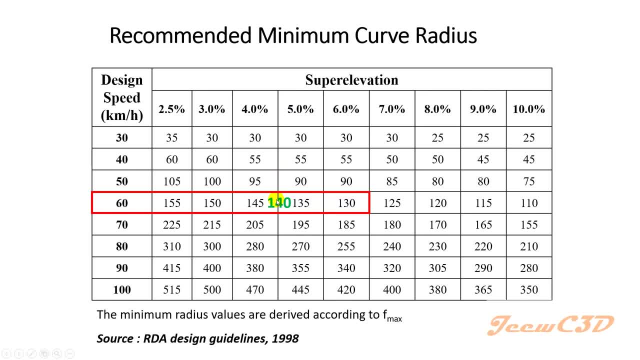 value. in this case you have to get the super elevation value, which is the closest one for and which is the closest one to this radius. it should you call this 140. this is less than 145, so you can't have super elevation 4, but it is. 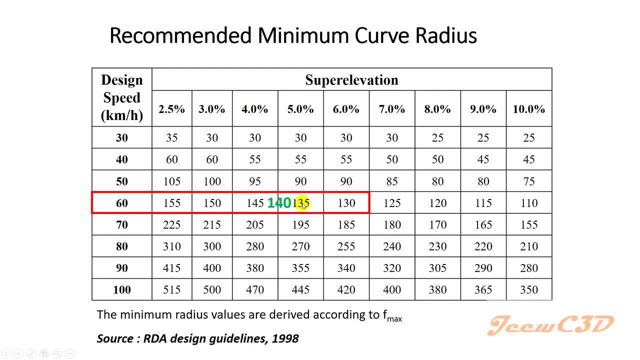 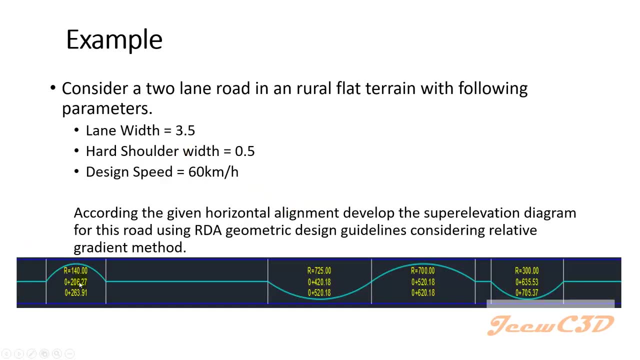 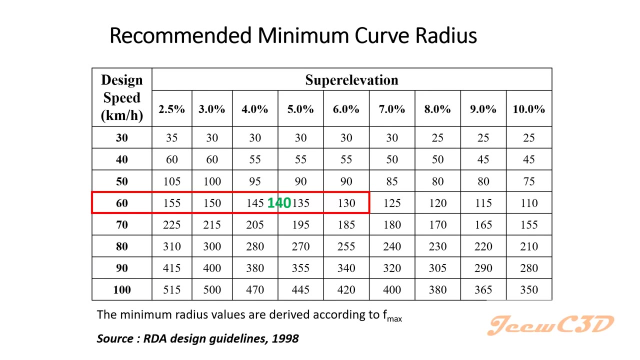 greater than 135. whatever the radius, greater than 135 and less than 145, you have to use super elevation 5. so 140 radius curve, that means this curve, you have to use super elevation 5. then you have radius 300, 725 and 700. the 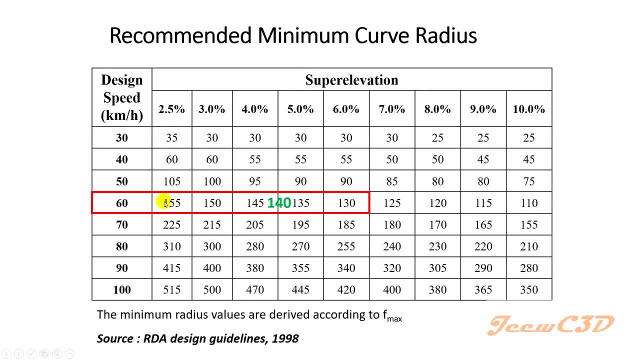 super elevation should be 2.5, because the curve greater than 155 radius will have super elevation of 2.5. but we have to check whether this the radius is beyond adverse cross-pole, because I told you, at the adverse cross-pole radius you don't need to apply super elevation. you 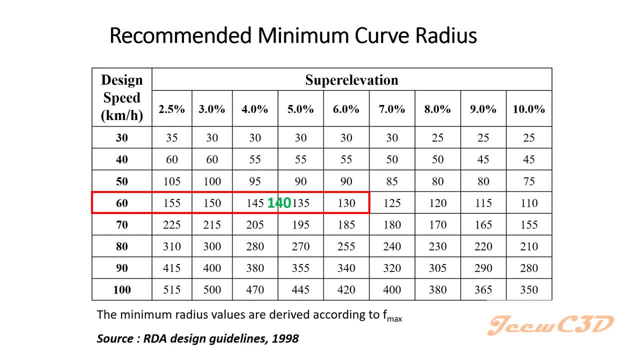 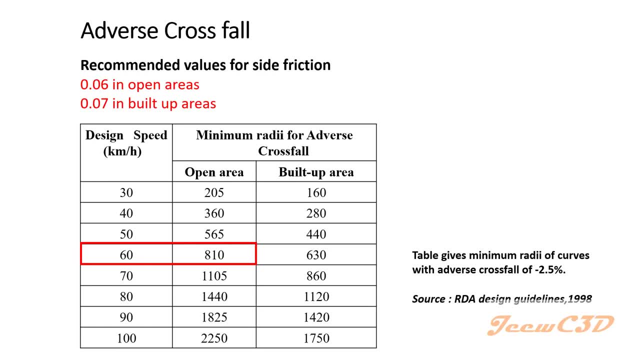 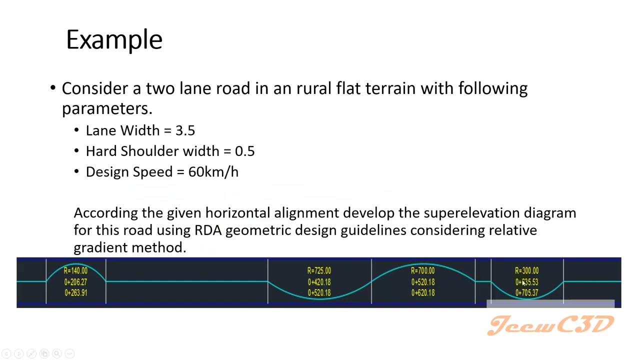 can go with the normal cross-pole, so this is the adverse cross-pole situation. so for the adverse cross-pole, this open area or otherwise we call it the rural area- adverse cross-pole radius would be 810. so in this example you have 725, 700, 300 radius. so you can, it is less than 810, so you. 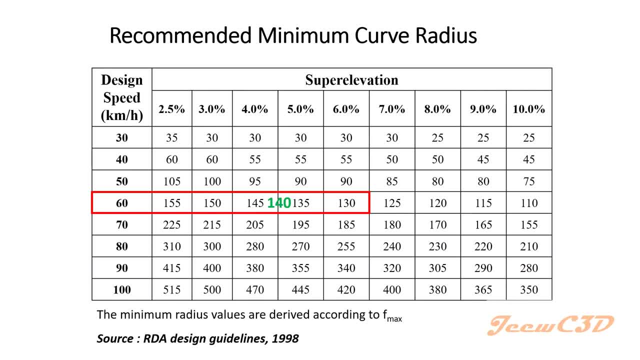 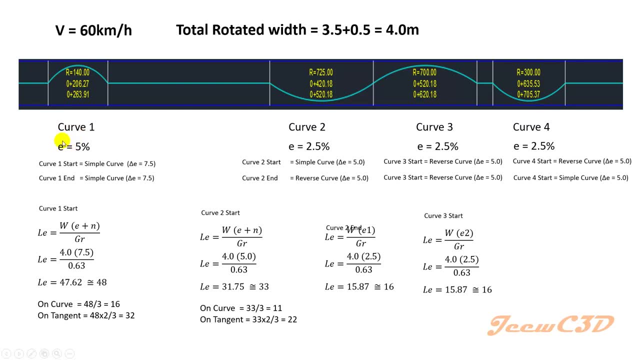 over. you have all of the curves. you should have super elevation of 2.5 because it is greater than 155 radius. so these are the super elevations you have. for curve 1, you have e equals 5. curve 2, you have equals 2.5. curve 3 also, you have e equals 2.5. and curve 4, you have e equals 2.5 as well. so if you 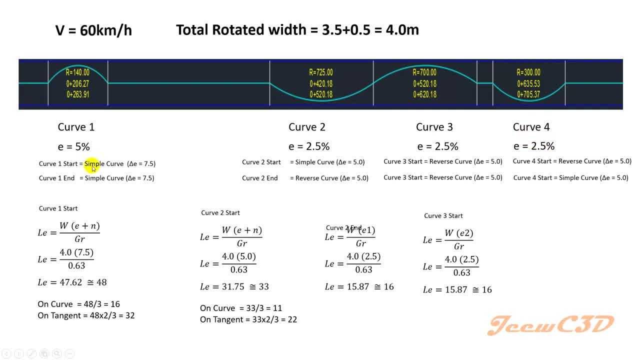 check up. think about the start section, this section of curve one. it is acting as a simple curve. that means you have a long straight and a curve. so long straight and curve. this is a. this is this. this part is acting as a simple curve. so in this section you have minus 2.5 super elevation. 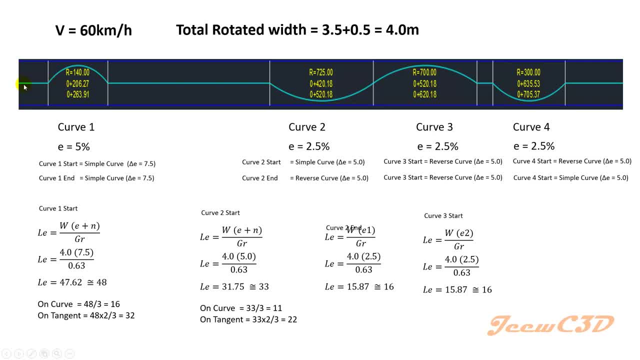 that is normal cross fall in this section. you have plus 5 super elevation. so minus 2.5 to plus 5 your delta e. otherwise e plus n would be 7.5. so if you consider the inside of this curve it has the same characteristics as the start side, so curve and long straight. so it has the 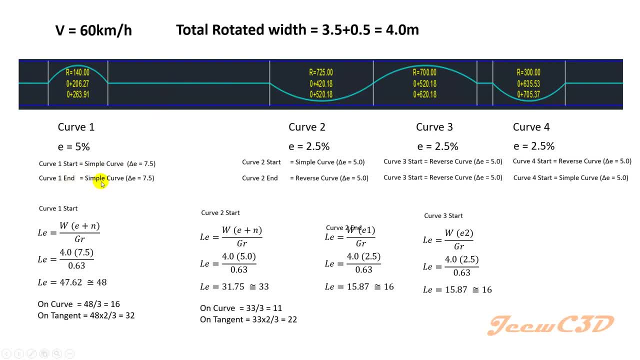 same characteristics. so curve in your e plus n is 7.5 as well. so we put the equation relative gradient method, equation lv equals w into e plus n, 4 gr. so your w is total rotated width, that is r shoulder, with plus plane width, that is 3.5 into 0.5, that is 4 meters. so this is 4 meters and this 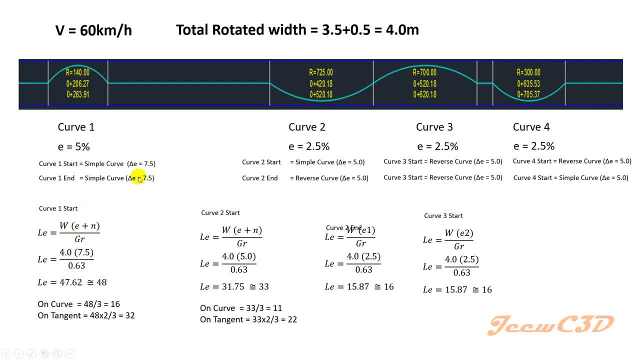 change is 7.5 and gr for uh 60 kilometers per hour is 0.63. if you can look at that value of 4 gr in the in start of the presentation, we will find this time is 0.63. so when you calculate this you will get 47.62. so if you can remember, 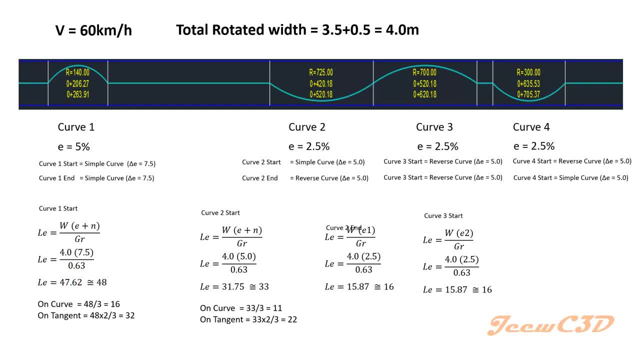 four simple curves. when you are distributing the super elevation development length, we say two-thirds of the length would be uh at the tangent and one-third of the length would be uh at the tangent and 1.3 the length should be at 0.2. and so for the first question by the蓮 Goshan, when we calculate L for a certain function and L for sending length, and plane length is now 0.73 and this 2, 3 third of the length would be uh at the tangent, and 1.3 because the deliberately l upper side of the・・. 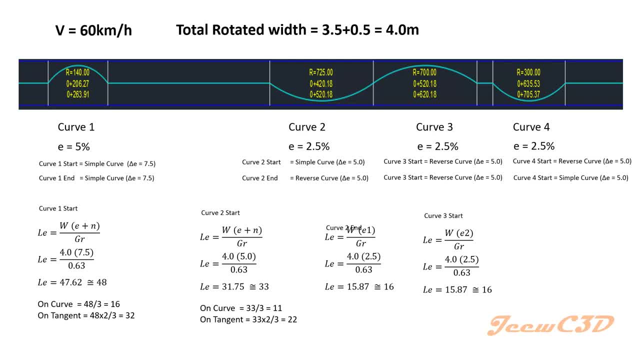 At the tangent and one third would be on the curve. So in this case we are selecting a length which is divisible by 3. so because you have to put that and you have to third and one third, so forty seven point six to be. 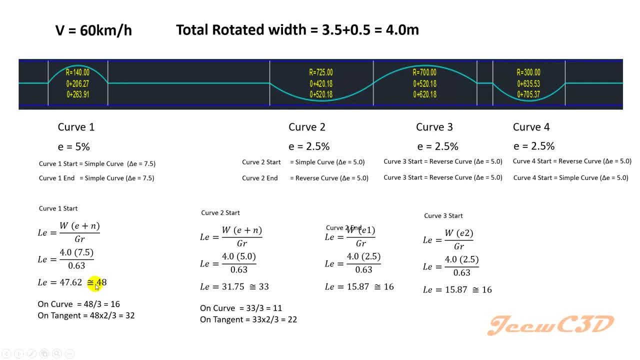 To sit or select 48. so one-third would be 16 and two-thirds would be 32. so on tangent we will have a length of 32 and on curve we will have a length of 16. so This is for the Start of the curve. your curve n also like a simple curve. 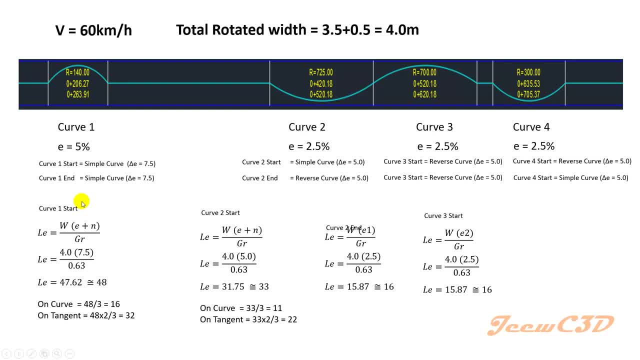 So you have the same calculation for the curve n as well and you will get these same values. So if you go to the start of curve 2, this curve 2 has a long straight section and a curve, So this is acting as a simple curve, so you can do the same calculation as 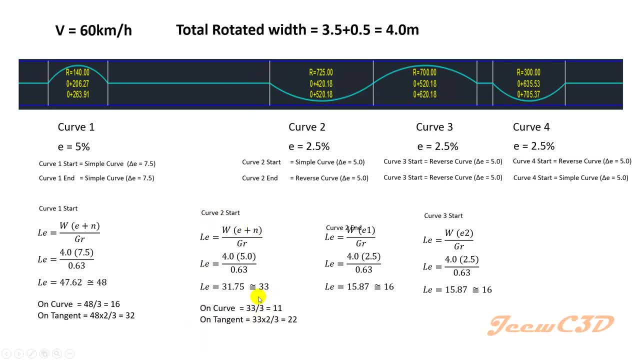 Before to get this value for this part, e plus n equals 5, because this is minus 2.5, This is plus 2.5.. So variation minus 2.5 to plus 2.5, that the change is 5. so that is how we get this. so that length become you select as 33 to this to be divisible by: 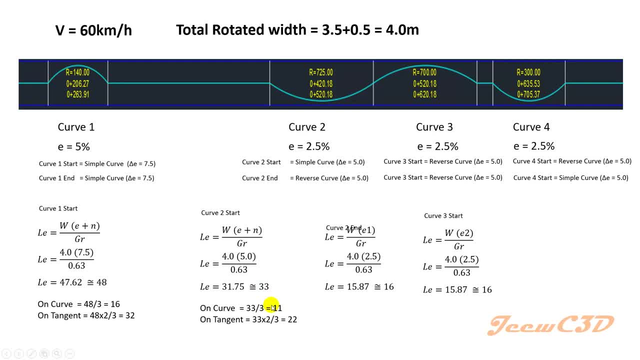 3. so one curve to start act as a simple curve, Then curve to end we use. Consider about the curve to end. This is a Reverse curve. this curve is turning this side, The other curve is turning other side. This is a reverse curve with a common tangent point. That means that 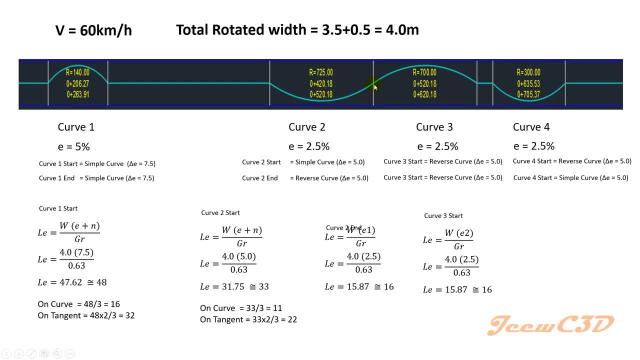 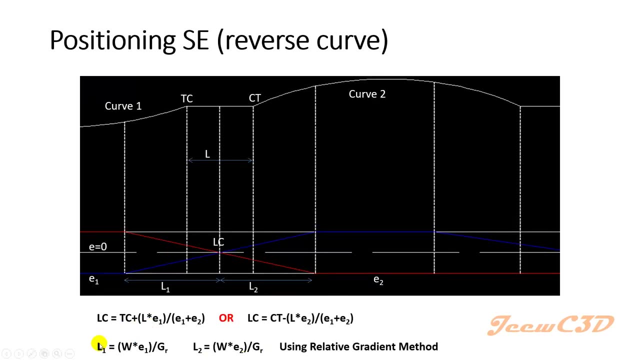 Tangent point. length is zero. There is no tangent at all Tangent point, so that length would be: if you can recall Here That length would be l. for this side l1 w, e1 over gr. for this side, l2 equals w e2 over gr. 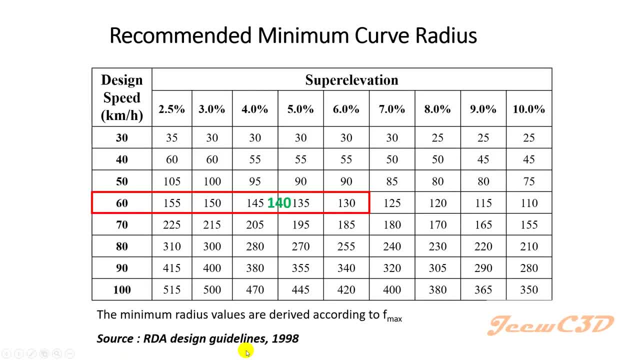 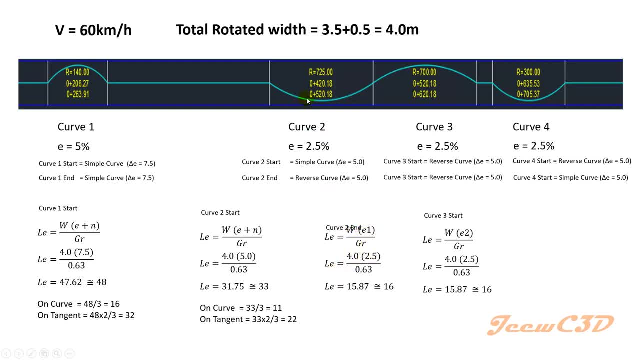 so here w e1 over gr 4 into e1 means this super elevation 2.5 gr is 0.63. in this case we are just rounding up to a full value or 0 decimal place, and we are not rounding up To a value which is divisible by 3, because we are not. 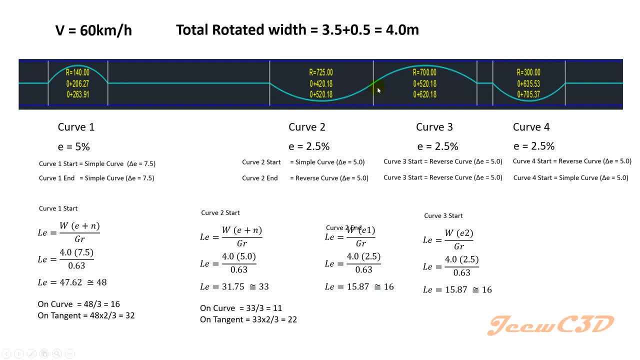 positioning, super elevation development, one third or two-thirds here, just putting this value. So on the other side, curve 3 start, that means this one. it is also part of that reverse curve. So it is W, e2 over gr. so this is e and this e is equal. so you have the same length here. so again you have. 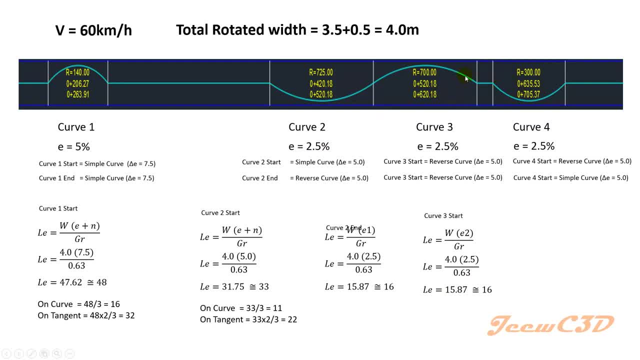 another reverse curve here, so curve 3 end and curve 4 start, so you can calculate this in your own and see what is happening you, what are the values you get. and this curve 3 end would be a reverse curve with a short tangent and curve 4 start will also be a 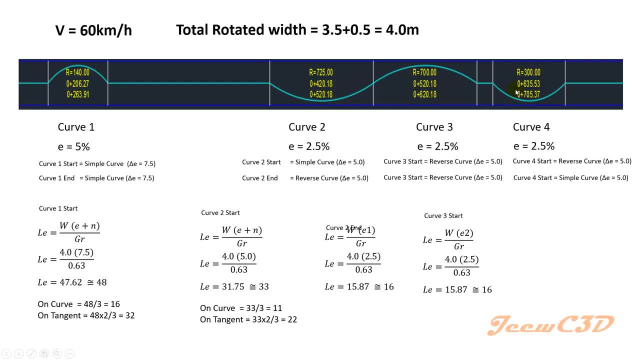 reverse curve with a short tangent and curve 4 end. this side would be another simple curve because you have the curve and you have a long straight so you can by yourself calculate this length and see what is coming here. so i will be discussing this things in a later day with the complete exercise. so that is about super elevation development length. 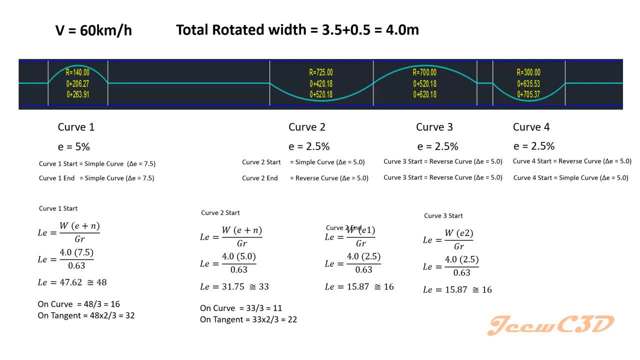 according to rda design guidelines. so in the next, next lecture we will be looking at another way of calculating super elevation development length, that is according to post road guidelines. that is different from the rda guidelines. we will be looking at that one also to have an idea. 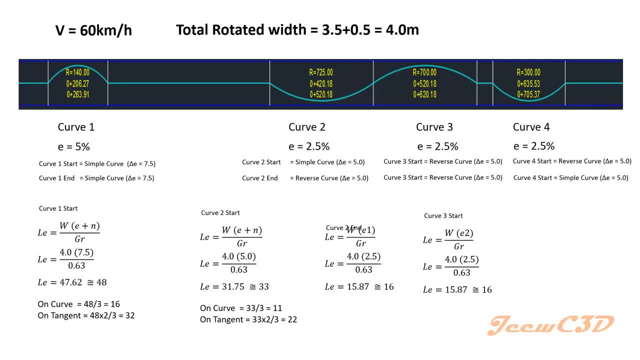 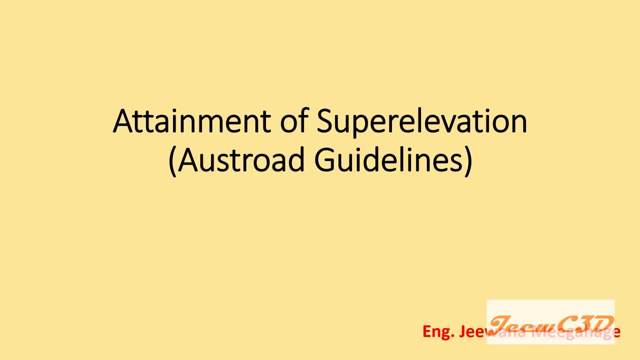 about how the super elevation development lengths are calculated in other parts of the world. in the previous video, we learned about how to attain super elevation through rda guidelines. in this, what we are doing is applying super elevation through post road guidelines, basically, the selection of radius for each curve related to design, speed and vertical alignment guidelines. 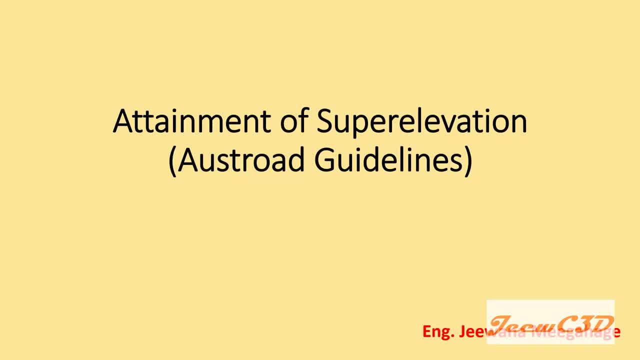 so those things are more or less similar in all the guidelines, with only small differences. but the attainment of super elevation through post road guidelines is not the same as the full range of the super elevation development length, length, the attainment of super elevation. there are some differences. that is why i am especially 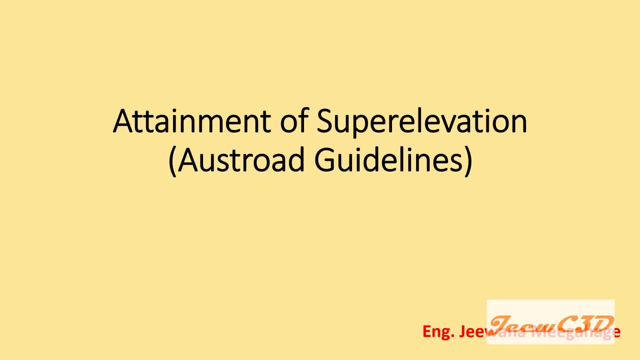 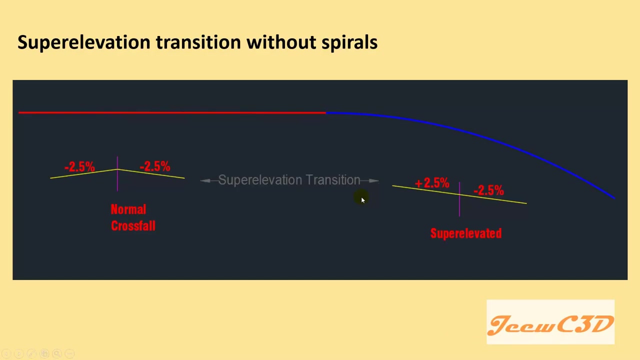 teaching you this short method and the rda method, and also there is a store guidelines so you can have a look about that. in this session, what we are doing is attainment of super elevation. in terms of post road guidelines, it is same as the Later 1.. here we talked about two rda guidelines, but there are small. 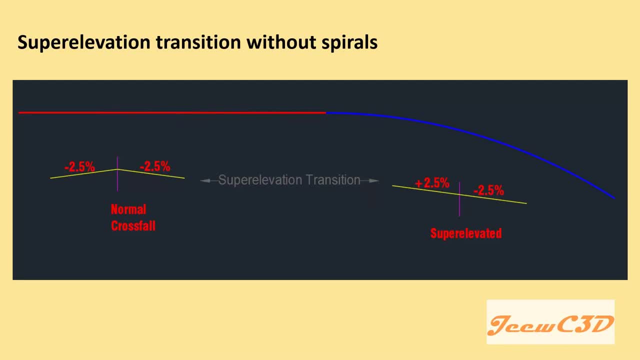 differences in between where you get the super elevation development length. so in this example, what we are doing is the super elevation transitions without spirals. so, as i explained this in my previous video, so you have the normal stress fall and you have the food upgraded section inside the curve and is defined in sports grids. I explain this in my previous video. so you have the normal stress fall and you have the full super elevation builder section inside the curve. in between, But see you in the next video. Thank you for watching. See you soon. Bye. 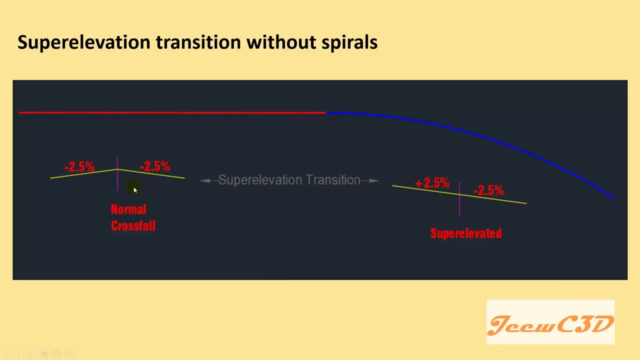 we have a superannuation transition. Even though I have used 2.5 values as normal first poles, especially in Australian guidelines, they use minus 3 as the normal first pole in Australia. Here I have used the old image I used in RDA. 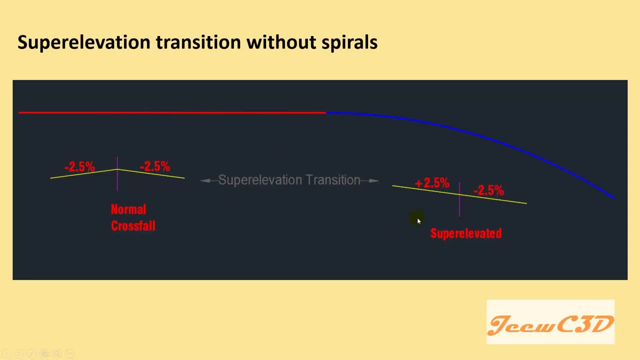 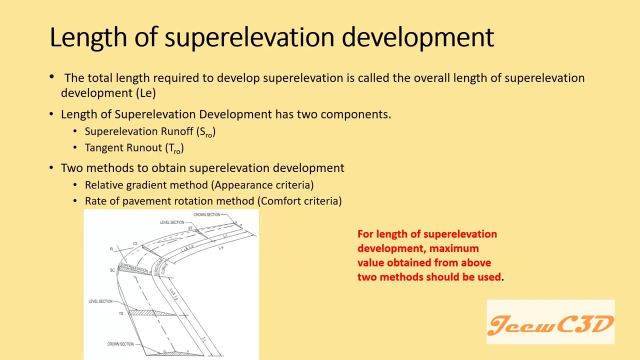 guidelines. That is why I am using minus 2.5.. Then we have two methods to get the superannuation development length. But there are new things to discover here, because we have two components in superannuation development length, That is, superannuation runoff and tangent runoff. 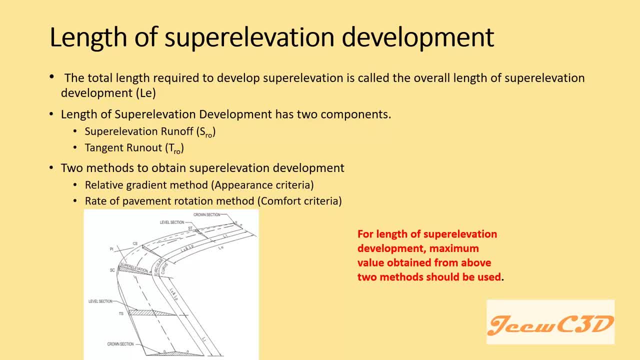 If you can remember what RDA guidelines taught you. that is, you get the superannuation development by either relative gradient or method for rate of payment rotation method only. what you get is the length of payment rotation length of the super elevation development. then you divided. 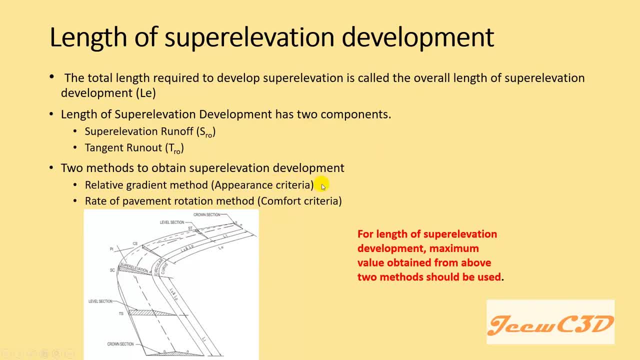 it into the curve and the straight according to the criteria, or if it is in a reverse curve, you have some way of doing that, but instead we have two things called super elevation runoff, SRO and tangent runoff. super elevation runoff means the length you required to change your cross pole from. 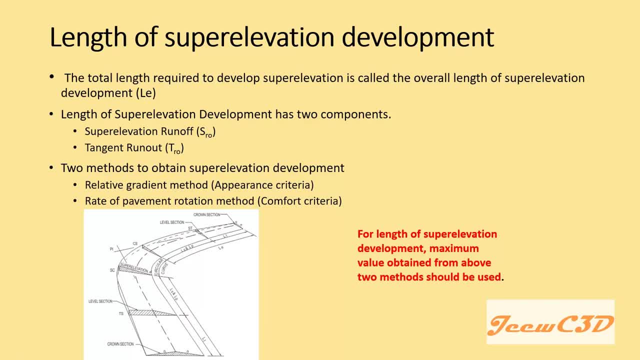 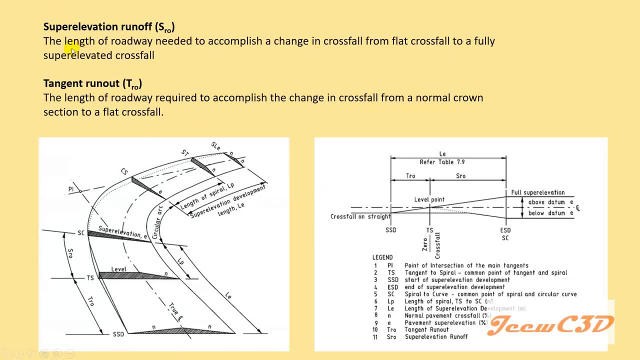 flat super elevation to the super elevated section. so here I have described the length for raw day needed to accomplish the change in first pole. from That means, if you consider this section, this left side will be super-elevating, so super-elevation manner. 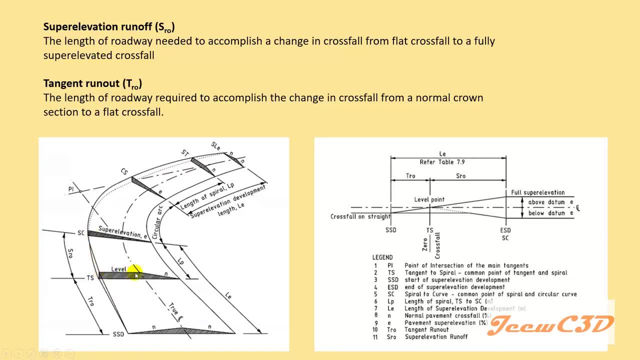 This means where your pavement cross-lock is from zero super-elevation. that means level relief, which is specified by the super-elevation. so this distance is called the super-elevation run-out and this distance is called the tangent run-out, where you change from normal cross-fall. 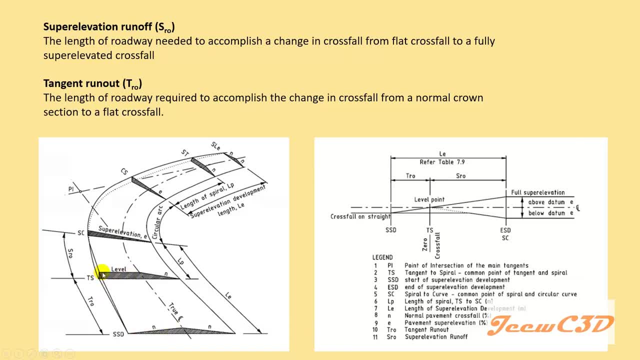 to level ground, or level is equal to zero location. this distance is called the tangent run-out. If you get the super-elevation diagram you can see this is normal cross-fall point. where this is level ground up to this point, the length is tangent run-out. 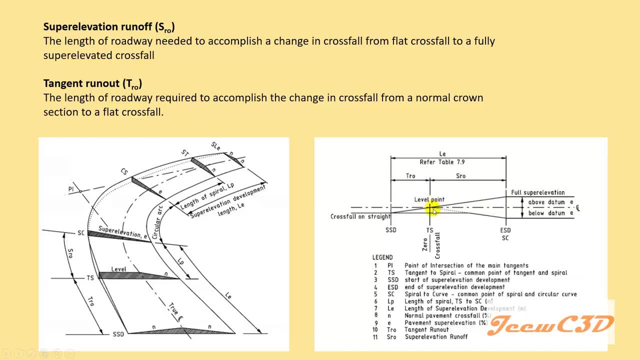 Then from level ground point or the super-elevation zero point to the full super-elevation point, you have super-elevation run-out. So that is the two criteria you have to remember when you are doing super-elevation. development length with short guidelines. 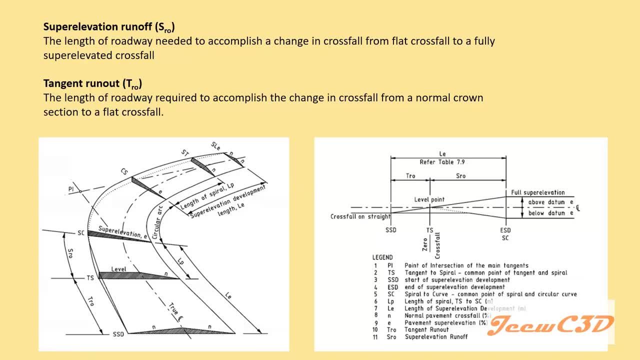 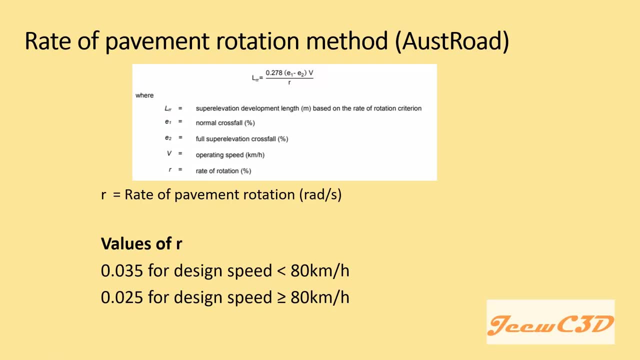 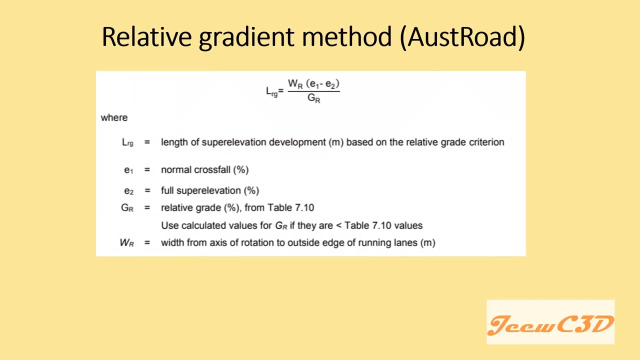 This thing is not there in RDA guideline. So there are two methods, as I told you earlier, to get the super-elevation development length, that is, pavement type of pavement rotation method, in a short and relative gradient method. So both of these were in RDA guidelines also, but there are some little differences actually. 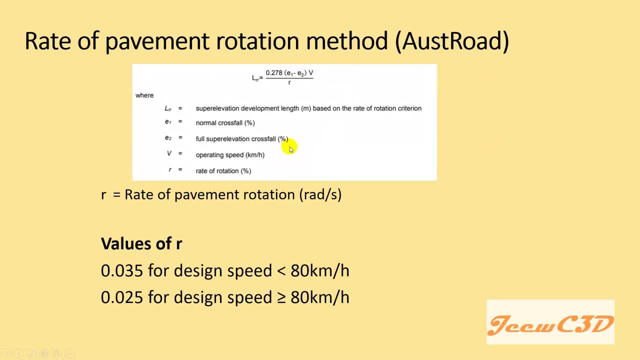 this thing is more or less the same one, But the relative gradient method is different. The gradient method is a little more different than the RDA one, So this rate of pavement rotation length of super-elevation development length is given by this equation. 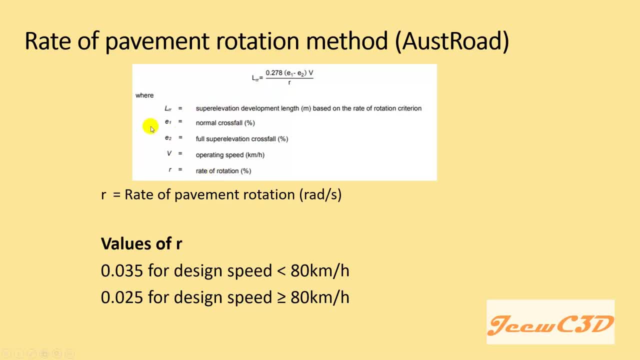 So you can substitute the values to this equation and get the super-elevation development length. So this ARRO length of super-elevation development related to rate of pavement rotation is from the change of pavement length, That is, the change of pavement from normal cross-college to full super-elevation. 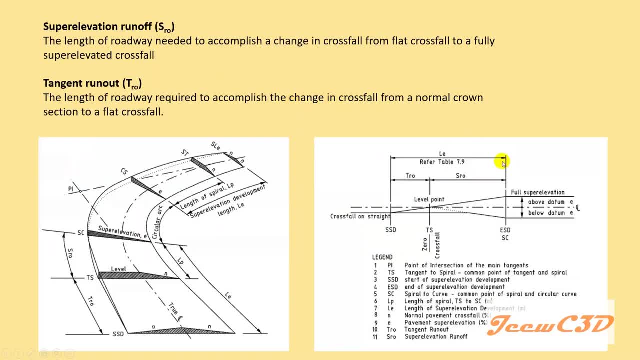 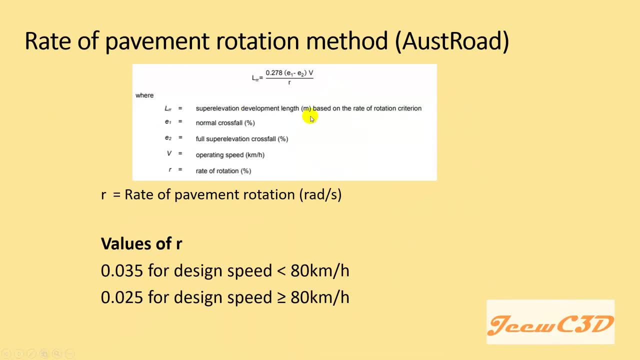 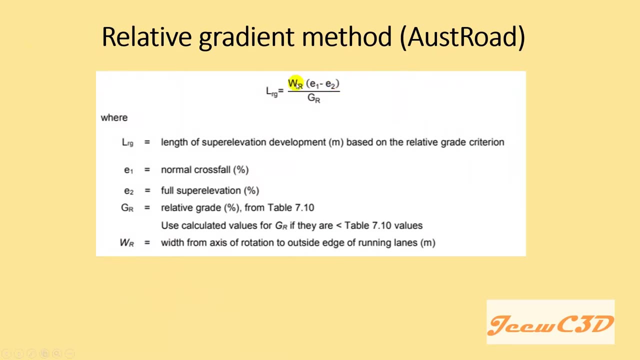 That means this LE normal cross-college to full super-elevation. That is the value given by this equation. Then we move onto the next method, that is relative gradient method. So you have this kind of equation. So this is same as the super-elevation development length we talked earlier. 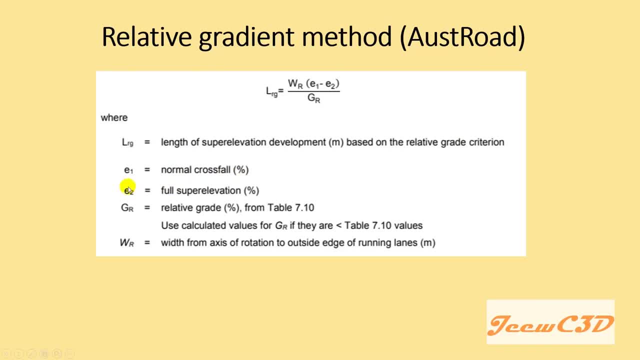 Which is equal to this LEs. So E1 would be the normal force pole, E2 would be the pulse of elevation value. This GR is the important value we have to consider in this location. I will give you more detail on this in the next slide. 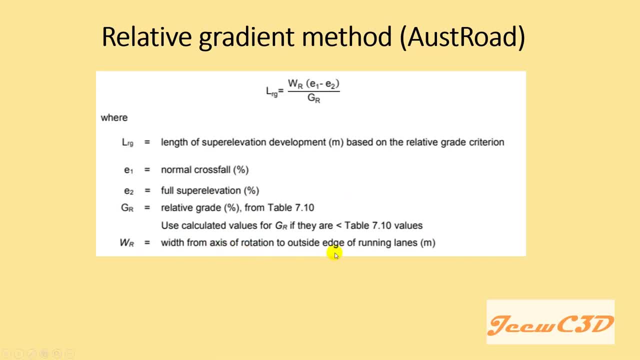 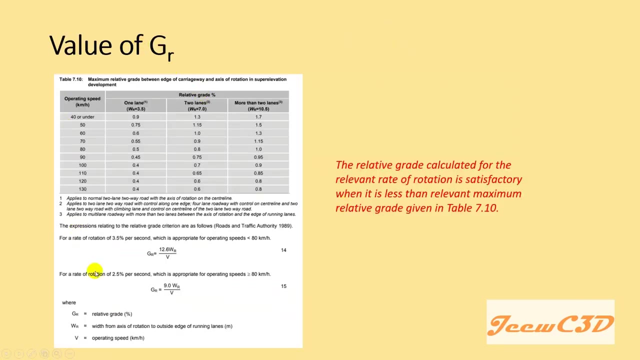 And WR is the width from axis of rotation to the outside digest running lanes. That means the lane width actually. In other words, this is the lane width. So here you have values for GR for lane one lane, the lane width is 3.5,. you have the GR values. 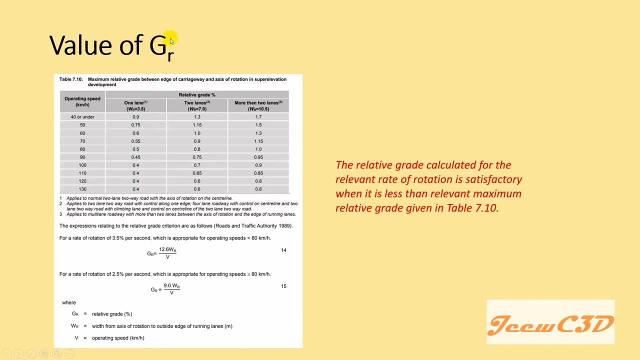 You can remember, we have this GR, which means the maximum relative gradient. So we had this in RDA design guidelines too. But in OSTRO there is a little more difference, Because you can calculate GR from this equation Either for this one or this one, depending on your speed. 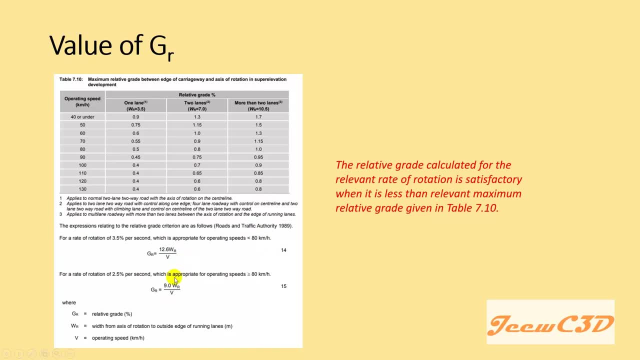 If your speed is less than 80 kmph, you have to use this one. If it is equal or greater than 80 kmph, you have to use this equation. So you have to use your lane width here. So let us say you calculate GR for 50 kmph. 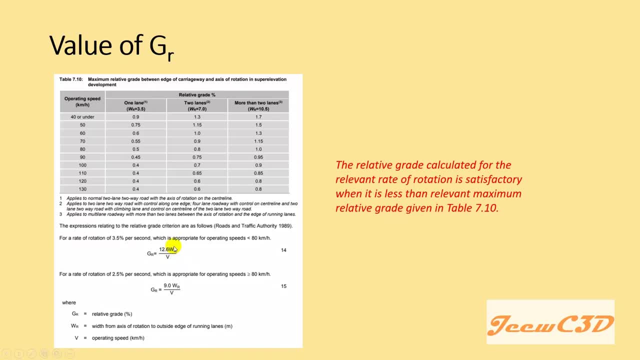 You put 50 here. If your lane width is, let us say, 3.6 meters, you put it here. Then you calculate the value. So if this value is less than this value, that means 0.75.. 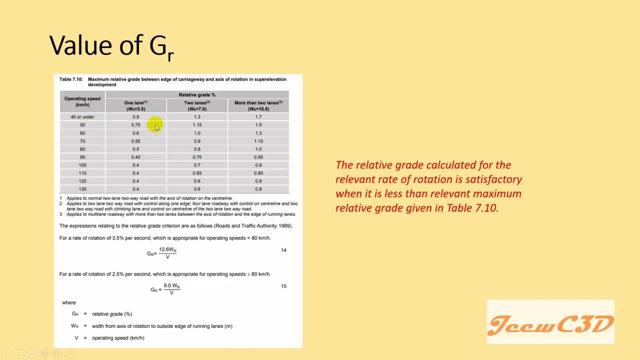 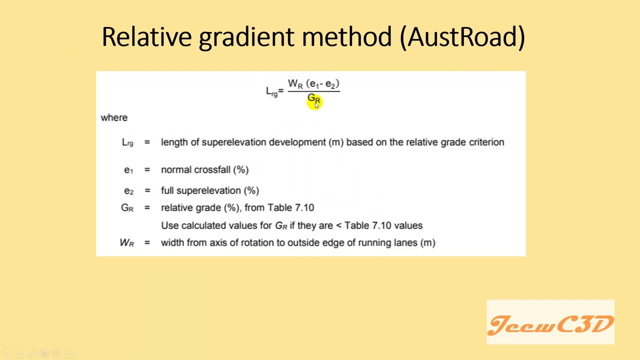 So for 50 design speed for one lane, your maximum relative gradient is 0.75.. Once you calculate it here, if the value is less than 0.75, you have to use this equation. If it is greater than 0.75, you can use that lower value to this equation. 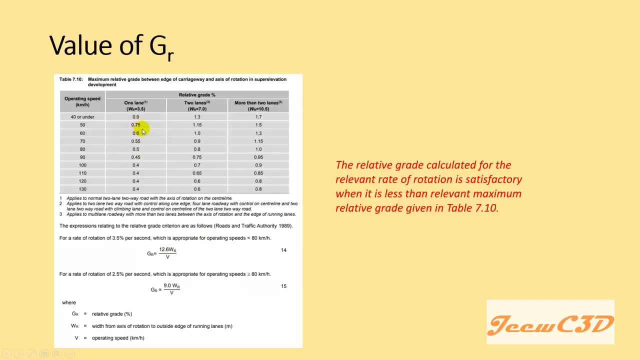 If it is greater than this value, that means if it is greater than 0.75, you have to use 0.75 in this equation. That is the importance of GR in this relative gradient method. So 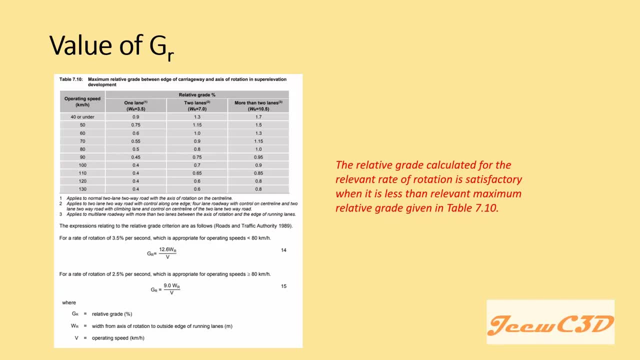 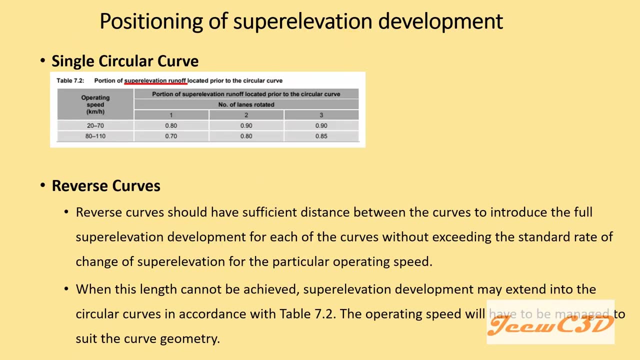 For post showed method. if it is a single circular curve, that means you don't have any spirals. So your portion of super elevation, nanop, will be located like this. So your operating speed is 20 to 70. So you will be putting 80% on the straight section. 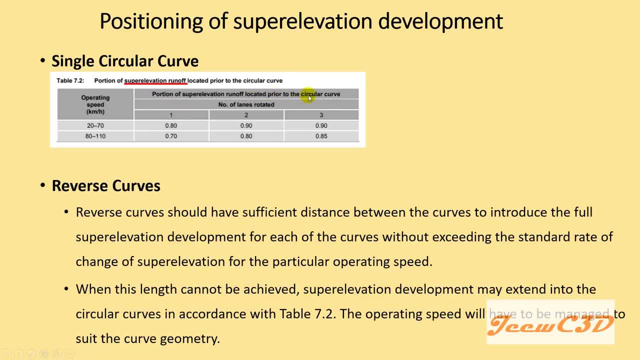 This means portion of super elevation, nanop, located higher to the circular curve. That means higher to the circular curve means on the straight. So this is 80% In RDA guideline of course 66% or 67% that means 2 third. But here you have 80% of the super elevation in the tangent section and only 20% on the straight. 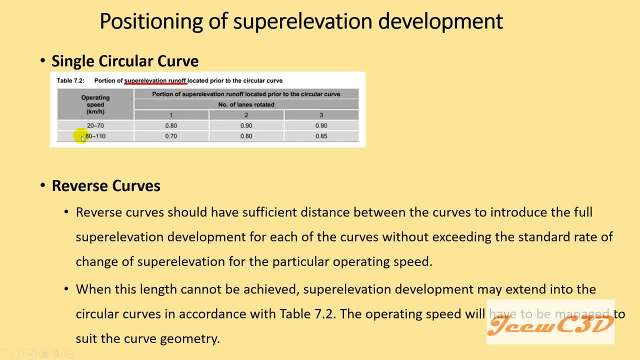 On the curve section. So if the speed is greater than 80 you have to use 70%. Then, in terms of reverse curves, it is saying that reverse curve should have sufficient distance between the curves to introduce full super elevation development for each curves without exceeding the standard rate of changing super elevation for the particular operating speed. 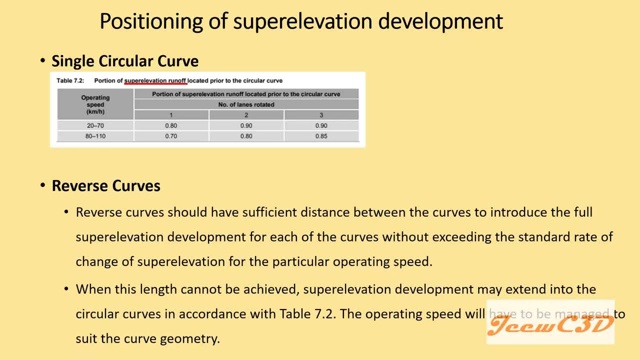 This means it is assuming that you have a small tangent in between the reverse curve so that you can apply super elevation development length. So if you consider about a reverse curve, in a reverse curve you don't have a tangent run out section Because in reverse curve you don't have a normal cross force. It is going one super elevation to the other. 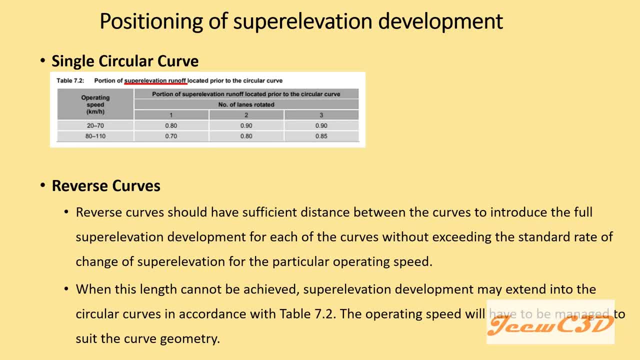 So there is nothing something called normal round in that section. So you don't have a tangent run out section. So you have only super elevation run out for one curve and super elevation run out for the other curve. In this what is assuming is both these run out lengths are in the tangent in between the reverse curve. 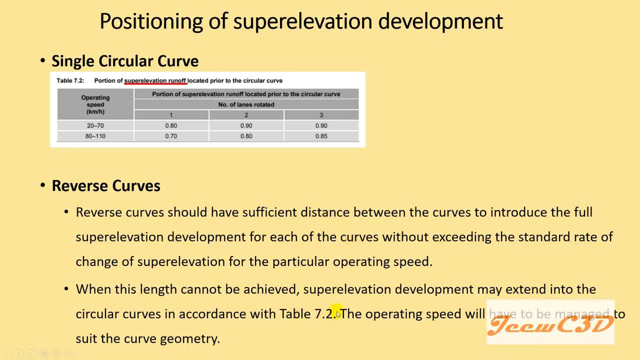 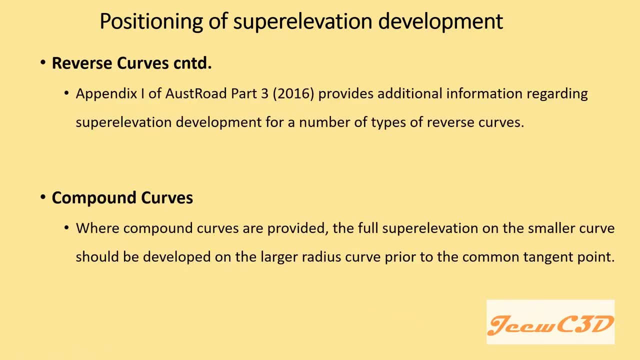 So if that cannot be placed, you have to use this table 7.2, which is this one to divide the super elevation development length inside the curve. But not only that. there are so many things about reverse curves in Ostrot, So there is something called appendix I of Ostrot, part 3 in 2016 version. 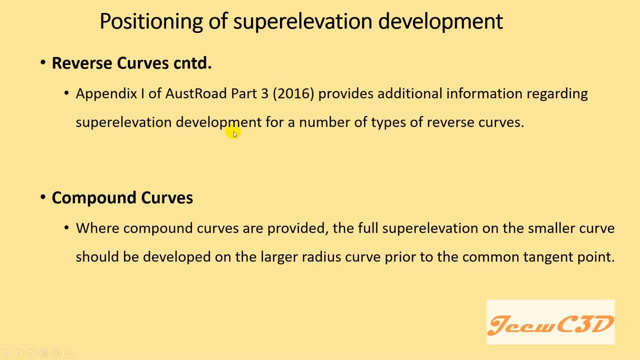 Provides additional information Regarding super elevation development for a number of types of reverse curve. If you got a chance, you can view this and see. there are lot of occasions you can apply super elevation development length inside reverse curves, Not only the one we talked about. 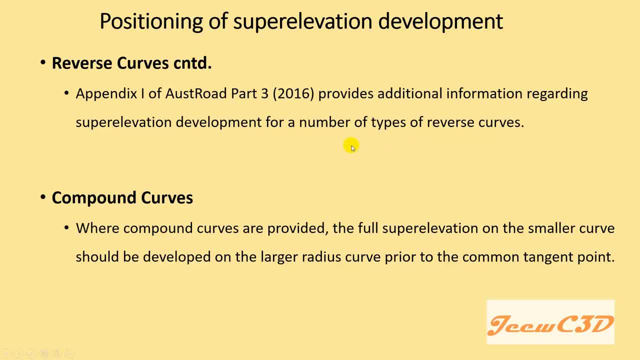 So I hope I better you. if you have some time, you can repair this. You should Repair this appendix I of Ostrot, part 3, 2016.. Then, about compound curve. that means the curve which is rotating in the same direction with different curve radius. 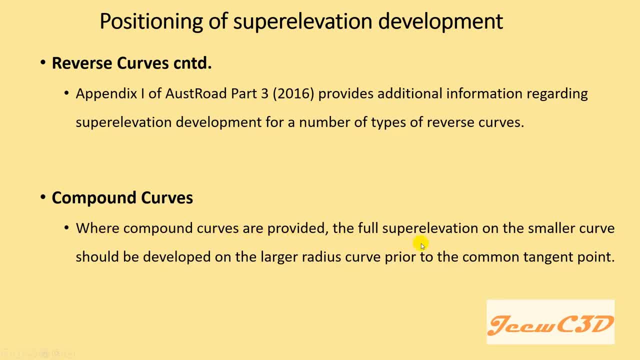 So where compound curves are provided, the super elevation on the smaller curve should be developed on the large curve radius prior to the common tangent point. So At a compound curve your super elevation in the smaller curve or smaller curve super elevation will be higher. So that should be developed on the larger radius curve prior to the common tangent point. 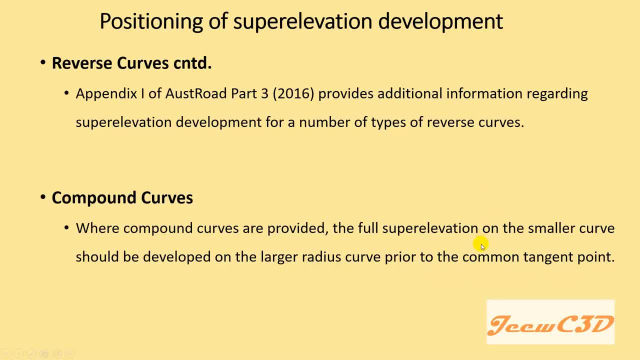 That means, as there is a common tangent point, super elevation development should be occurred before the smaller radius curve. So that means it should be within the, it should be fully within the large radius curve. So that is what is saying here. So that's about super elevation development within the Ostrot guidelines. 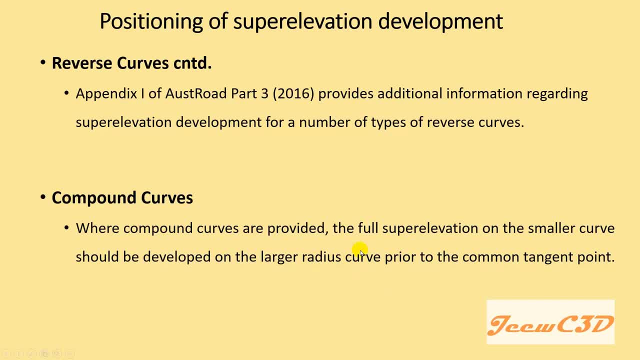 So this is a small summary of the Ostrot guidelines. There are so many things to know on this guideline, But I think this is Some summary of the guidelines so that you can follow if you Need to learn about Ostrot. so you can get an idea from this and you can follow the Ostrot guidelines later. 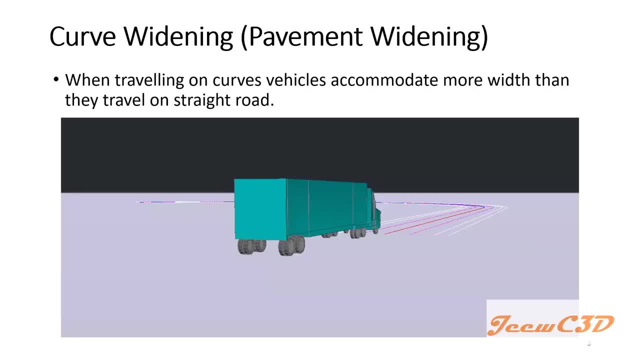 How do how the things happen in Ostrot guidelines? In this section we are going to Learn some Something called curve widening or otherwise. we are calling it pavement widening. So when traveling on curves, vehicles accommodate more width than they travel on straight road. 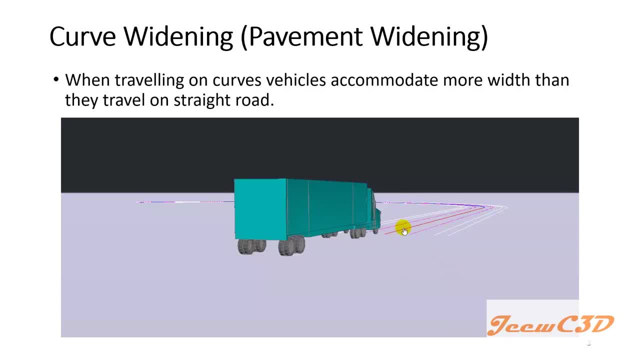 So if you look at this image, This is the centerline of the road. This magenta color lines are the centerline of the Travel Vehicle. So this vehicle is traveled along a centerline in this lane. So this white line and this red line, for the centerline is a lane and this is the center of that lane. 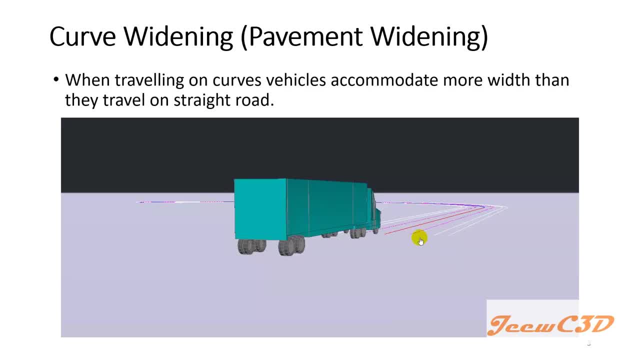 And after that we have the hard shoulder. So usually the vehicles are expected to run inside the lane. So, but we will look at how It is Going to happen When the vehicle is traveling on a curve, especially a heavy vehicle. So here this vehicle is traveling. 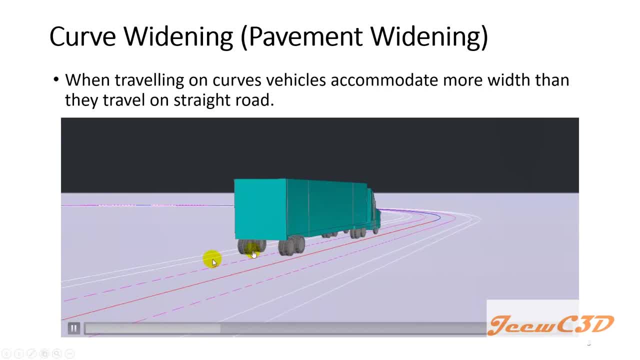 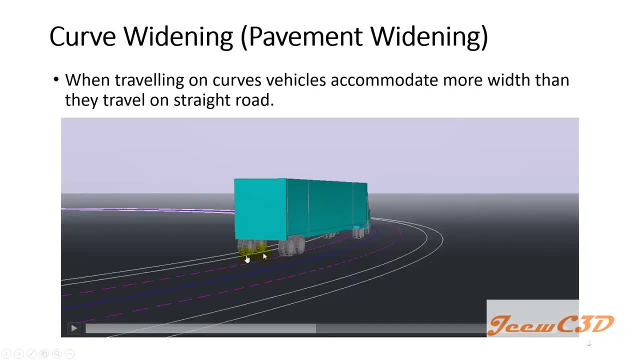 Now these Tracks tires are inside the lane, So you will see what happens when it comes inside the curve. So this outside tires are going outside the lane. So this is the lane, This area is the lane, But The outside tires are going out of the lane. 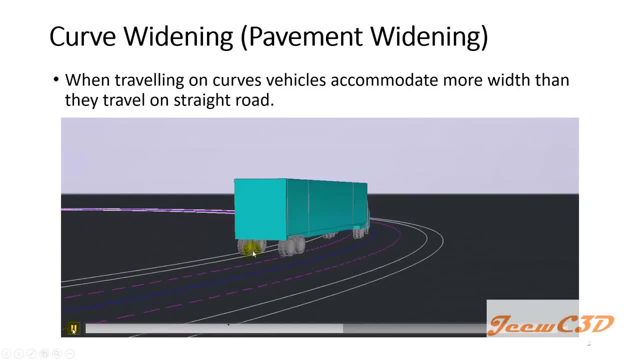 It is inside the hard shoulder. Sometimes it may go outside the hard shoulder also, So in that case, what we need is we need to increase the width of the lane So that the full width of the vehicle will be accommodated Inside the lane of the road. 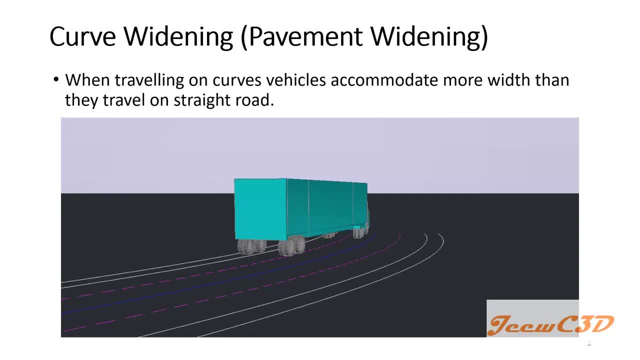 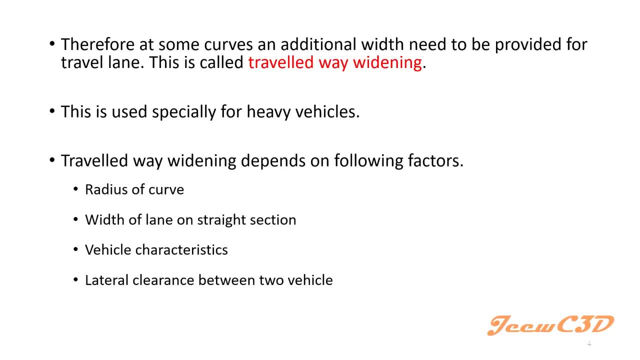 So this is called this increased width. inside these curves are called curve widening or else the pavement widening. So this is also called travel way widening, because we are widening the travel way. There is some other widening called side distance widening. It will be used when. 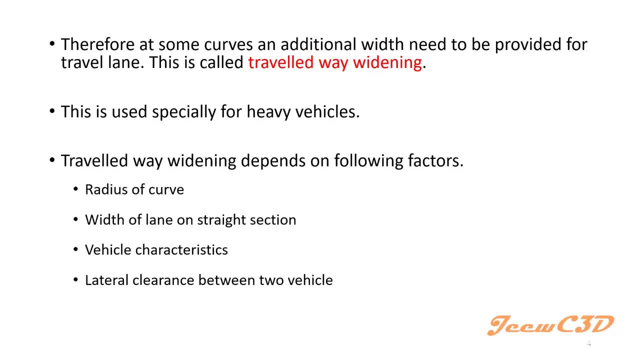 The side distance obstruct by a object in the road. so we widen the widening the road. we call it side distance widening, But in this case what we do is travel way widening, which is increasing the width of the road inside curves. So this is specially used for heavy vehicles, as you saw in that example, light vehicles such as car or vans. 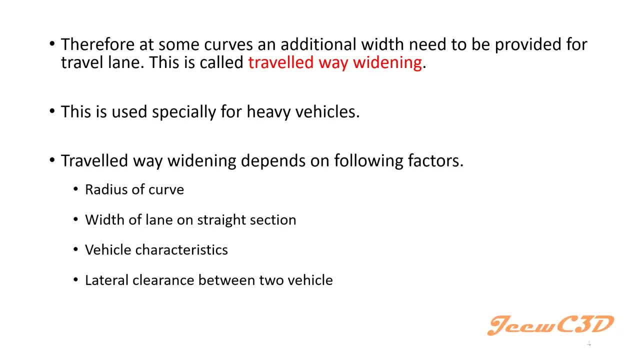 This will not be affected by the curve radius, But for large vehicles like trucks or buses they might go outside the lane when they are getting the curves, when you are traveling on the curves, especially for sharper curves. So this travel way widening depends on four factors. 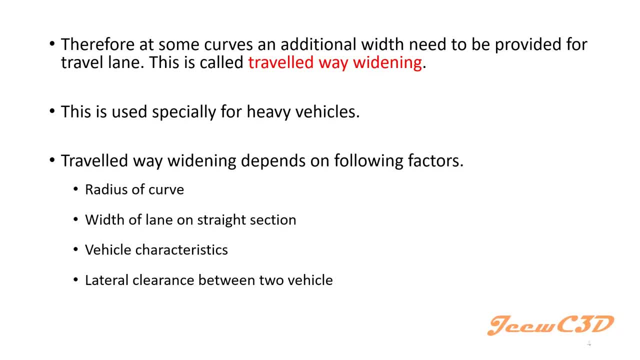 They are radius of curve and width of the lane in straight section. Straight section section means that straight sections. we don't have any widening. so we consider that normal plane width of a straight section in the vehicle characteristics, such as design, vehicle or what kind of vehicle they are and the parts uh connected to that vehicle. so if you consider about a truck, 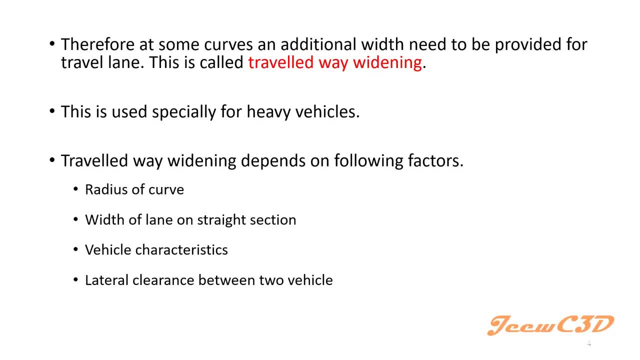 you have a front part and rear part so depending on the vehicle characteristics, that widening may be different. so we need to define the widening for the design vehicle. we learn what is design vehicle in the earlier lectures. so we have to design or we have to think about, think about. 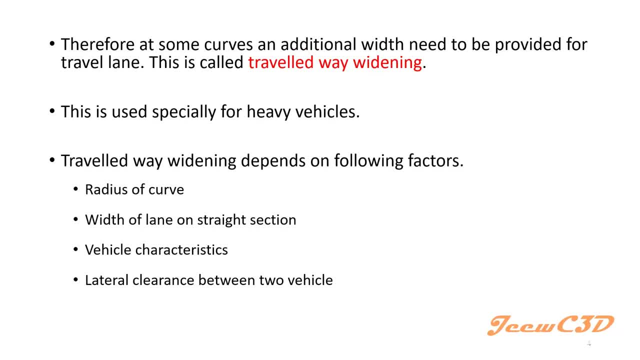 or we have to assign widening on curves according to the design vehicle. then the last one is lateral clearance between two vehicles, because when a vehicle is traveling on a curve and another vehicle coming on inside other side of the curve or otherwise, if this vehicle is overtaking another, 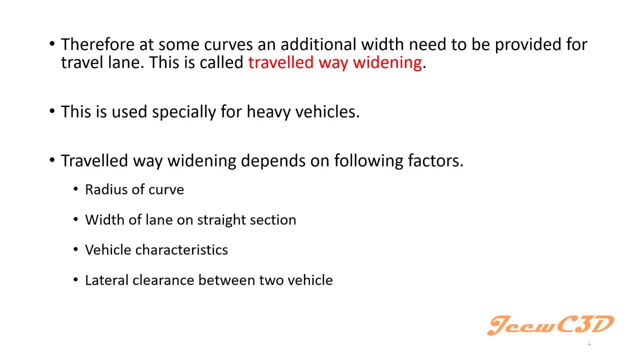 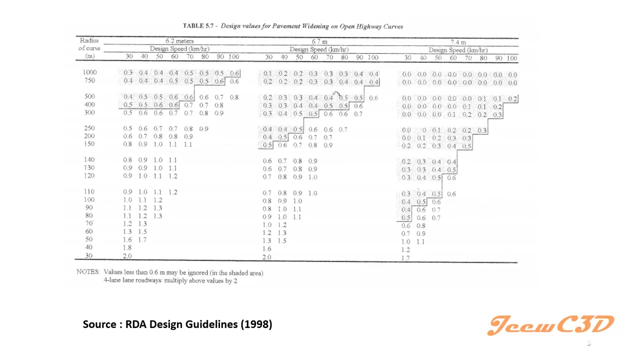 vehicle, there may be a small gap between two vehicles when the overtaking is taken place. usually in straight sections this gap is a little bit low, but in curved section the drivers maintain more gap to have more safer overtaking or traversing movement inside the curve. so this is the table, or this is the values defined in rda guidelines for curve widening. 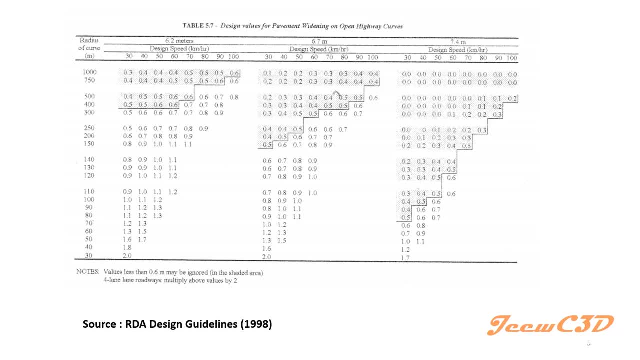 usually curve. widening is a very expensive thing. you because you have to widen the pavement or the widening the lanes to accommodate this vehicle parts. so usually if this widening with this less than 0.6 meter, we ignore that widening so we don't widen, in that if the widening is greater than 0.6 meters we will be widening the. 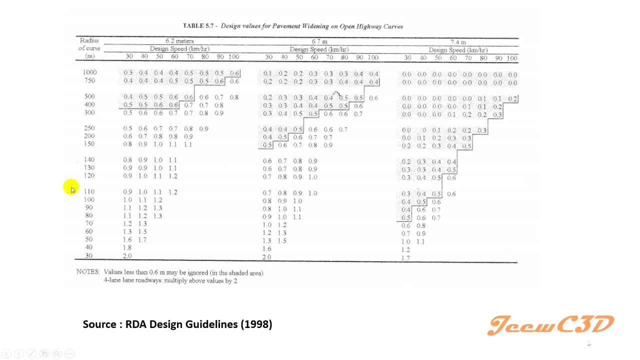 road. so in this table you have the amount of widening according to the radius of the curve and according to the width of the lane. we actually width of the total lane with i mean this 6.2 meter means 3 point into one direction and 3 point into other direction likewise. so, depending on that data, these widening values are. 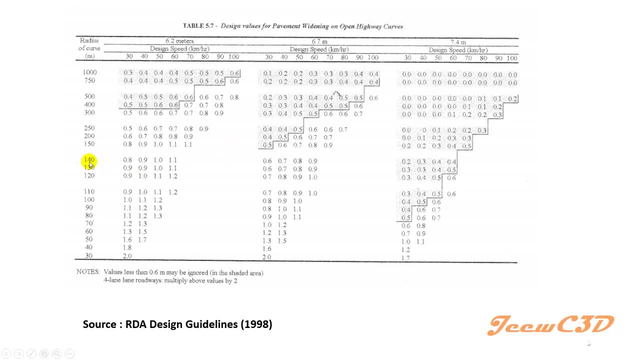 defined. for example, if your radius is 140 and if your design speed is 30 and your lane width is 3.1 meter, so you will be having a 0.8 meter widening width. so that is how to get the widening values. so if you have 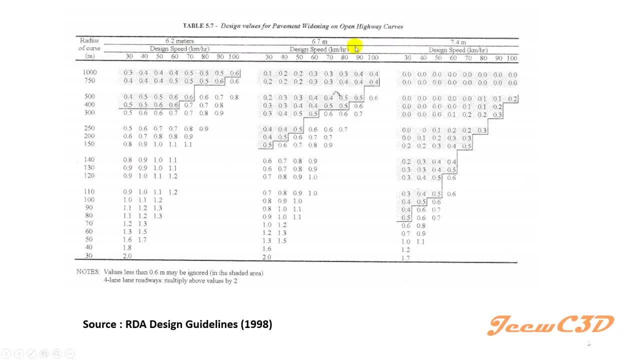 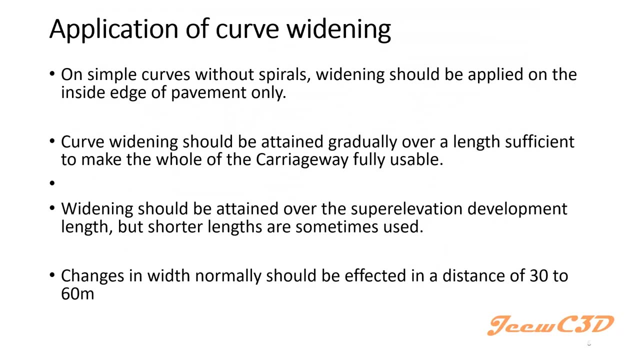 lane widths in between these values. you can use interpolation. then about the application of curve widening, how the curve widening is placed, because on straight sections you have one lane width. if you have a curve widening inside the curves, you have another lane width. so this lane width have to be positioned inside the curves as well as in the. 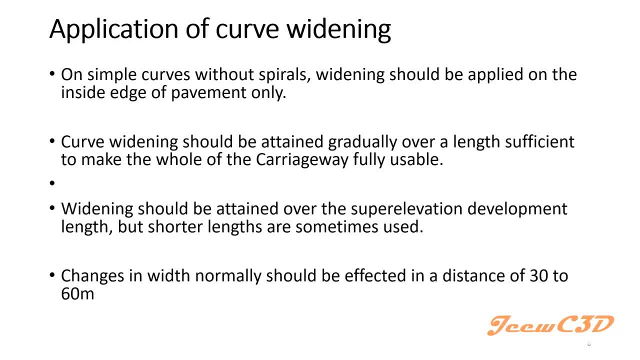 straight section. so how to get the widening of the curve widening, you have to use interpolation. now this white minis application is described here. on simple curves without spirals, widening should be placed on the inside, the edge of the payment. usually we are placing the widening in the inside edge of the payment because that is the side where are the vehicles going outside the 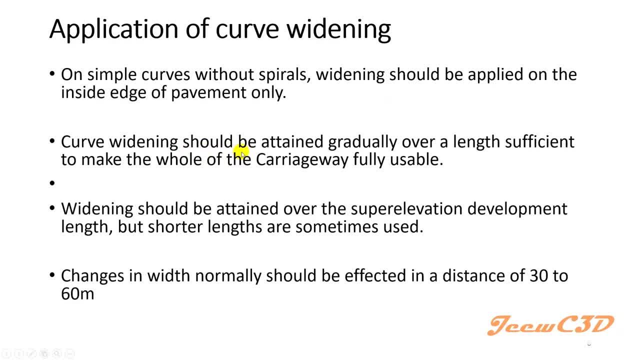 curve. so in curve widening will be attained gradually over a length two, sufficient to make the whole carriageway fully usable. so this curve widening will be obtained. so if the straight section lane, which is 3.5, and inside the curve, with curve widening if the lane which is 4. 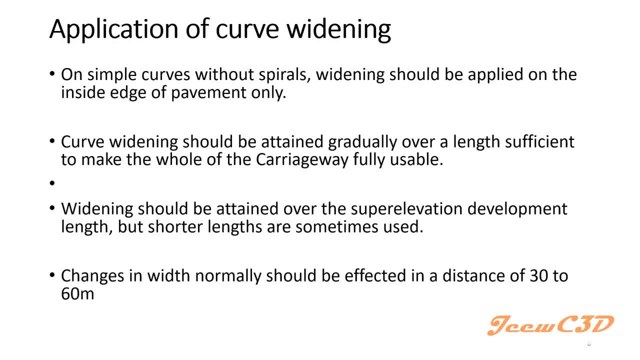 meter, so 3.5 to 4 meter, which will be gradually attained inside the travel way. otherwise the carriageway won't be fully usable if you suddenly increase the width of the lane if the other part would not be is usable. so instead of that, what we do is we are gradually increasing the width. 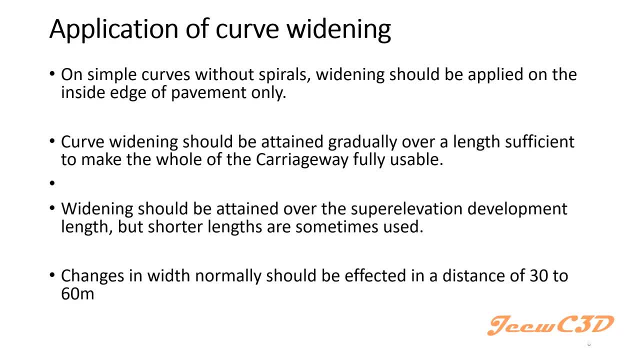 of the road from one width to the other width. so this widening will be attained usually over the super elevation development lane. but if you can use shorter lanes it can also be used. so usually these widths are changed. widths are changed in fitting the distance of 60, 30 meter to 60 meter. so that is about widening of horizontal curves. then we will. 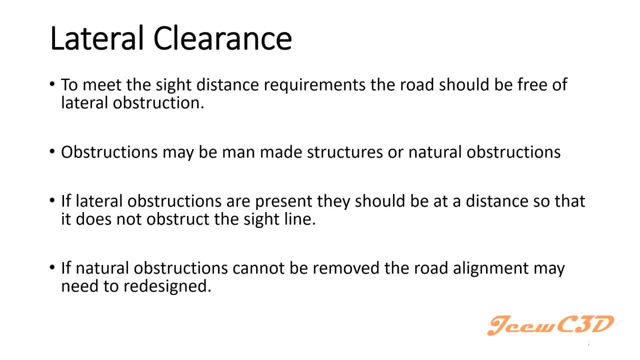 be looking at something called lateral clearance- clearance, so this thing is used to have the proper side distance requirement on the road. so to meet the side distance requirement of a road, that road should be free of lateral obstructions. lateral obstructions means the obstruction at the outside edge of the curve, where it will be, where that object will be. 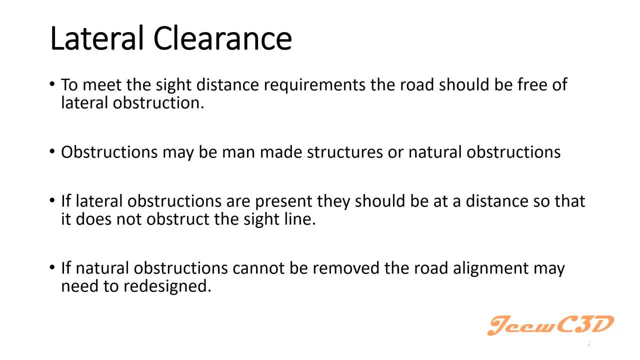 disturbing the side distance of the vehicles. so these obstructions are man-made structures, so natural obstructions. so when you are traveling on a curve, if you have a house inside edge of the closer to the inside edge of the road, you cannot see the other part of the curve because of the house, so it obstructs the side distance. on the other hand, if there is a 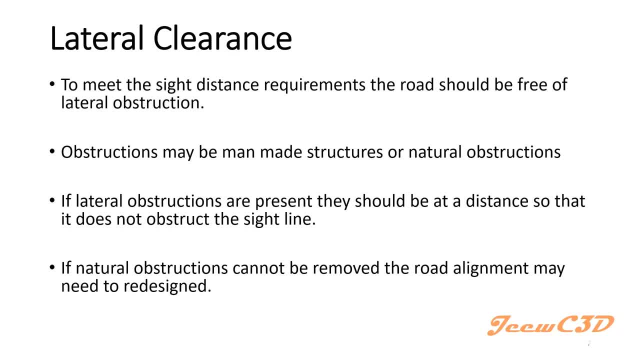 larger rope closer to the inside edge of the road. still that will be disturbing your side distance. so these are obstructions would be placed in a distance. they are this: the side distance is not obstructed. so if, if they cannot be uh moved, or if there's a natural obstruction, sometimes we may not able to. 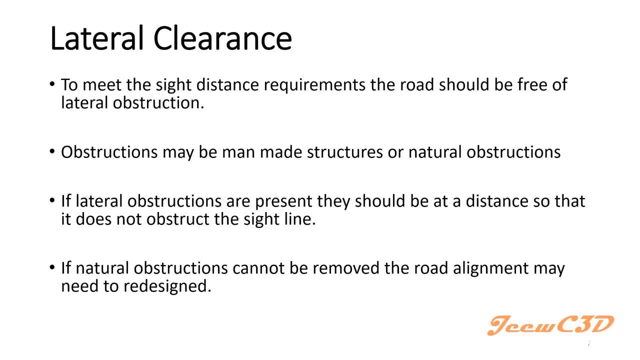 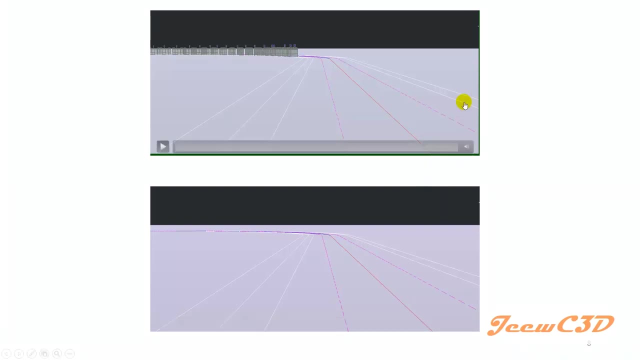 move that obstruction, so in that case we have to redesign or move our horizontal alignment so that to side. so we have to think about that, uh, when you are designing. if the lateral clearance are not there, so in here we will be looking at a situation: we obstruct the side distance. so in this top one, 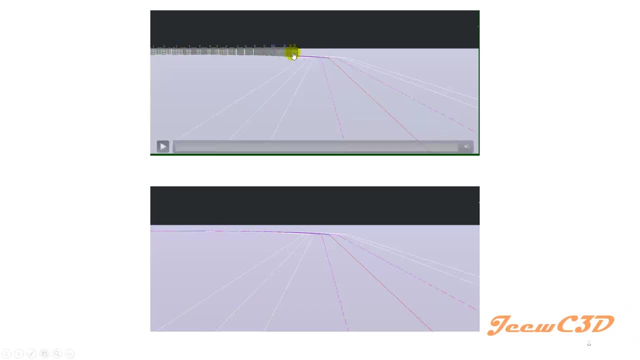 you have set of shops or uh uh merchant area where the side distance will be obstruct inside the curve here this is a straight section. then you are getting a curve- here this is a straight section, same section without these obstructions. we will see how the things happening in both these scenarios. 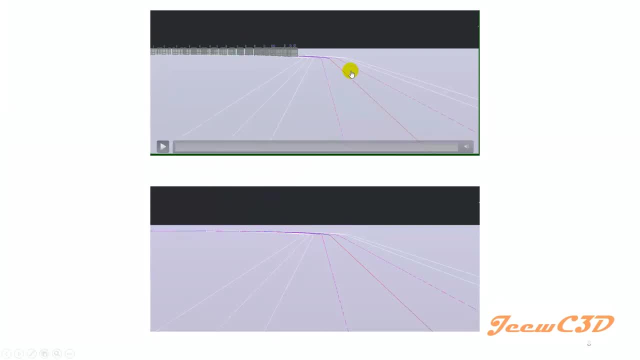 you have the center line of the road here. this is the center line of the lane, this will be the lane and this is the center line of the lane and this will be the hard shoulder. this is somewhere outside the hard shoulder so you can see, in both cases the vehicle is running. so this is seen as a driver eye height view. so you 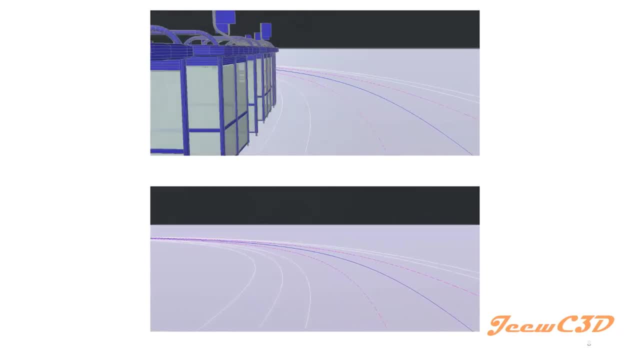 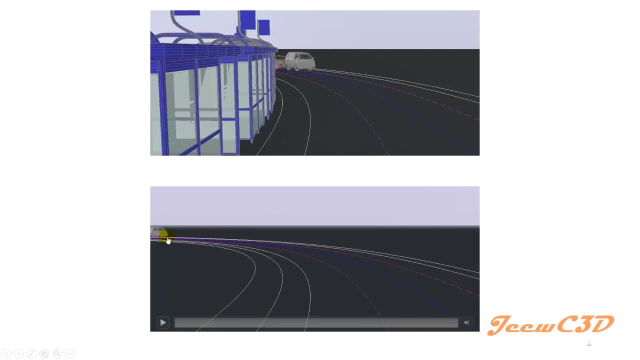 can see what is happening here at the bottom image you can see: once the obstructed obstruction is seen, the vehicle is stopped. if you can remember, this stopped first and this stopped second. that means this vehicle was seen later than this one. so that means this is obstructed by these uh objects, so the site view is obstructed. 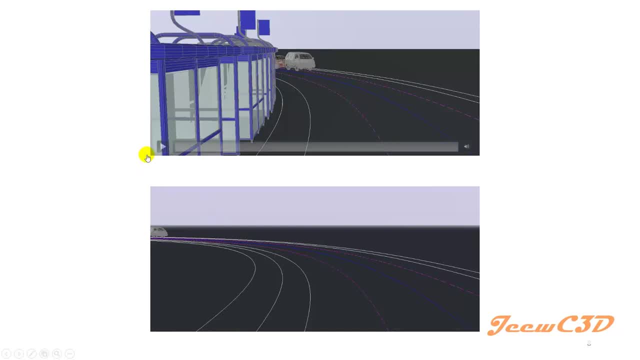 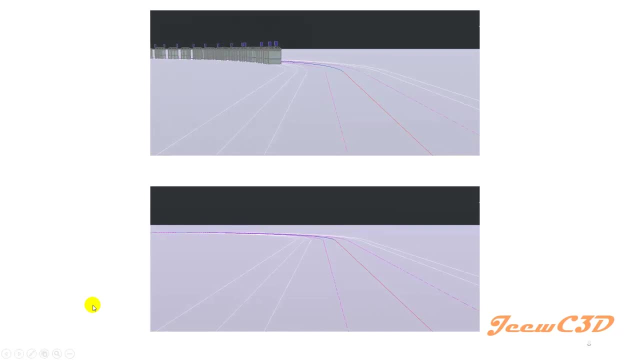 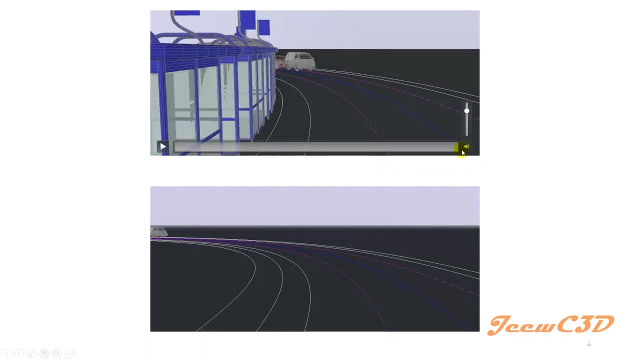 by this object objects. so if you view that again, you will see it, baby, they are started at same time. this when the obstruct when the vehicle coming from the other side is seen. this vehicle has traveled 17 seconds- you can see it here- and this vehicle has only 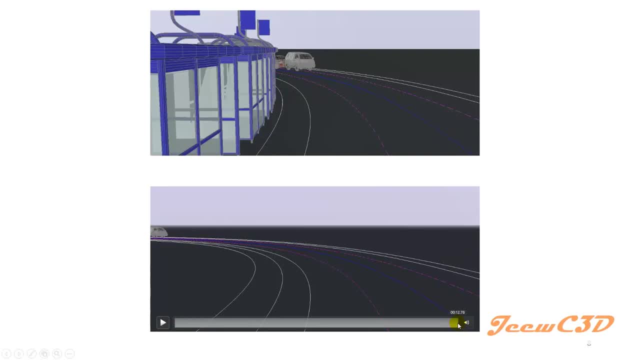 traveled 13 seconds, So that vehicle sees the object 4 seconds earlier than the first one. That is because of these obstructions. In this case you don't have any obstruction, So you will see the objects closer to the inside of the road will be disturbing the. 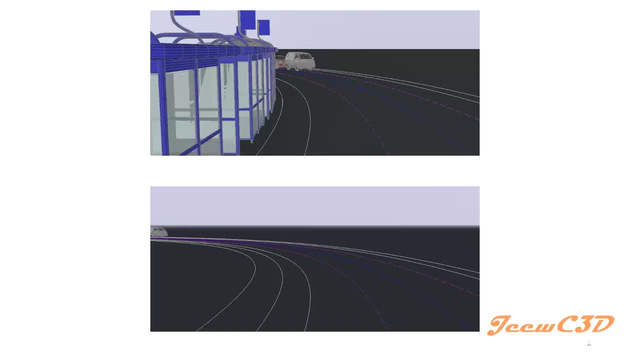 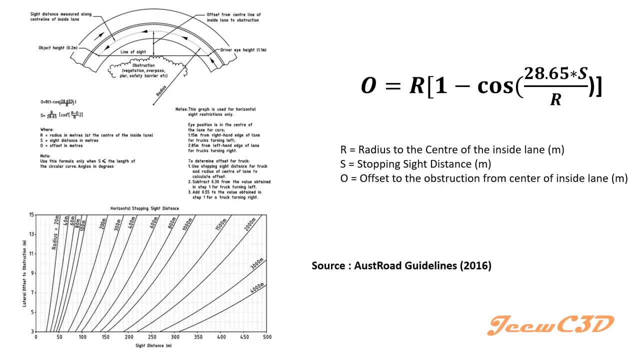 sight distance. So these objects have to be placed outside the lane edge or the outside edge of the road, but it could be at some distance where it will not be disturbing the sight distance. In this equation we will be looking at how to check the lateral offset for road crossings. 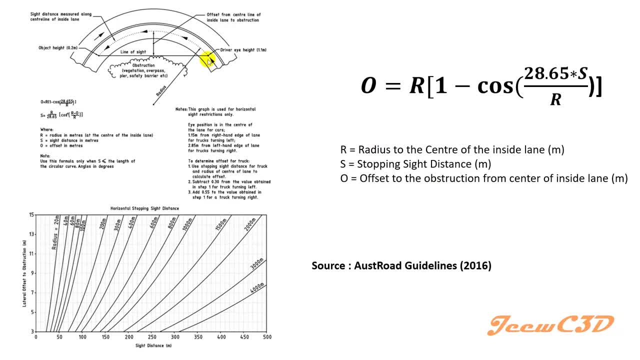 So these objects have to be placed outside the lane edge or the outside edge of the road. So you will be looking at how to check the lateral offset for road crossings. Here you have the travelling vehicle. This is the centre of the travelling path of that vehicle. 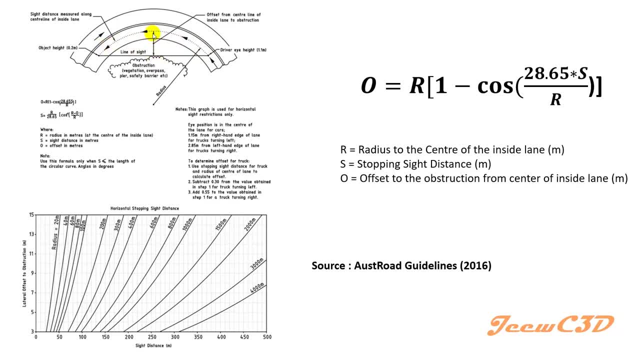 This is the obstruction, This would be the line of sight offset, So that one is given as O this length. So this O equals R into 1 minus cos 28.65 s over R. They are s' be the stopping side distance and stopping side distance or side distance. 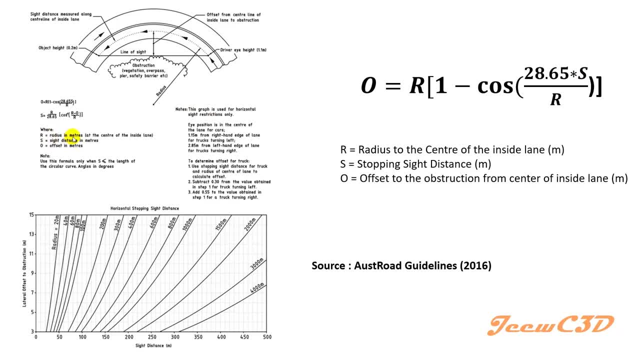 and R will be the radius of the curve in the inside plane, so that R is not the radius of the road curve but it will be the radius in meters at the center of the inside lane. so this cost value 28.65 into S over R. so this cost value. 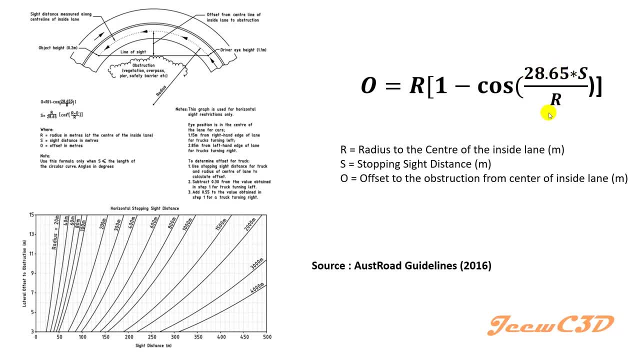 should be calculated in decrease. when you are applying the equation, then this equation is developed only for the situation where side distance is greater than or less. side distance is less than or equal to R and the less than or equal to length of the curve, so your side distance would be: 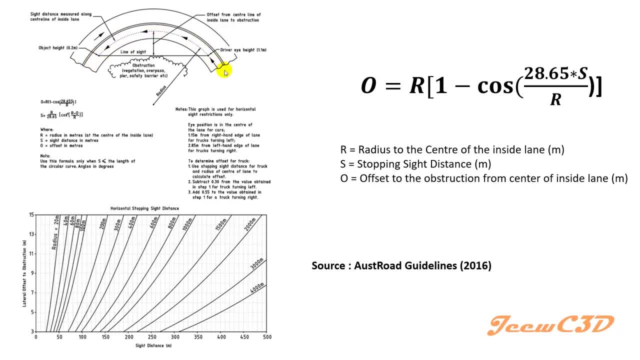 something like this: your curve length would be greater than this side distance. so if it is at the other case, or the side distance is greater than the length of the curve, you have to graphically analyze this situation to find out. the lateral offset need to be considered in the road. 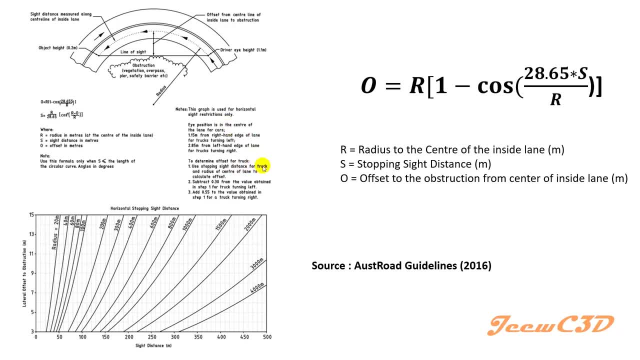 curve. so one more thing: this equation is developed using a short guidelines, but in RDA guidelines also we have a similar equation but kind of difference than this one, but it gives the same values, but the equations is equation is different slightly, since this one is a more easy equation. 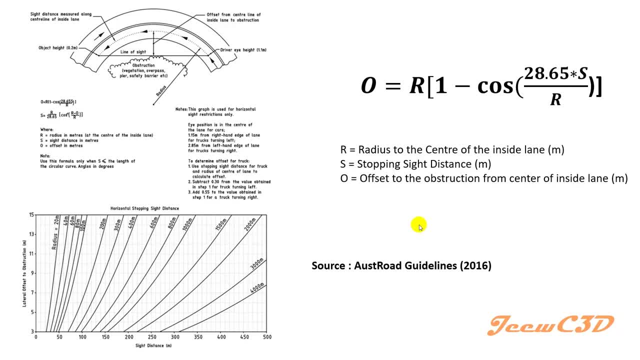 than the RDA guideline. I have shown it here, so you can directly calculate the lateral offset needed for a vehicle traveling inside of the curve, so that the obstructions will not be a problem to the side distance of that vehicle. same thing can be obtained from this curve. 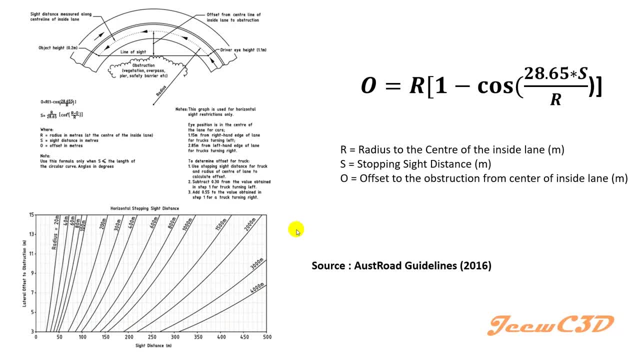 also. so that is about the lateral offset with this curve also. so that is about the lateral offset with required for the horizontal curves inside the roads. So in this session we have looked at curve widening of roads and lateral offset of the curves. In the next session we will 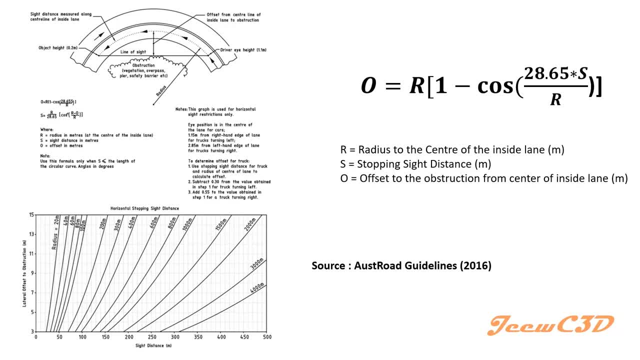 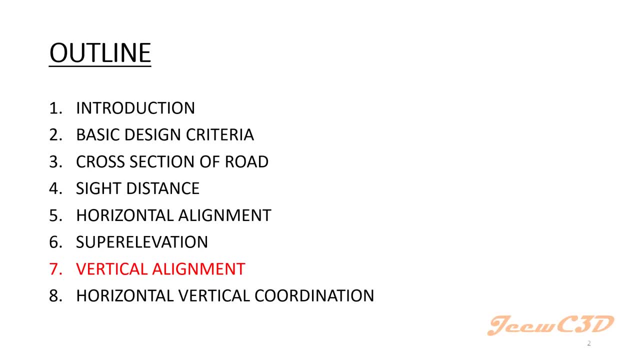 be looking at vertical alignment of the road. In this video we are going to look at vertical alignment. Vertical alignment is the elevation component of a road, where you study about the elevation or otherwise the gradient and vertical curves of a road. So in vertical alignment we have two elements: the straight, 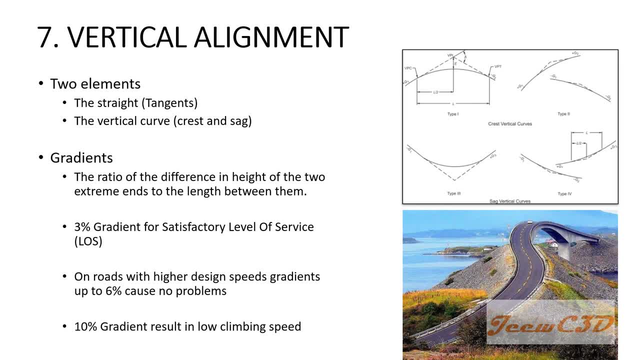 section. that means the tangent section. Straight means the grade region of the road, So the gradient section and the vertical curve. We have crest curves and sag curves, So a curve like this would be called as a crest curve. So all these are crest curves and this kind. 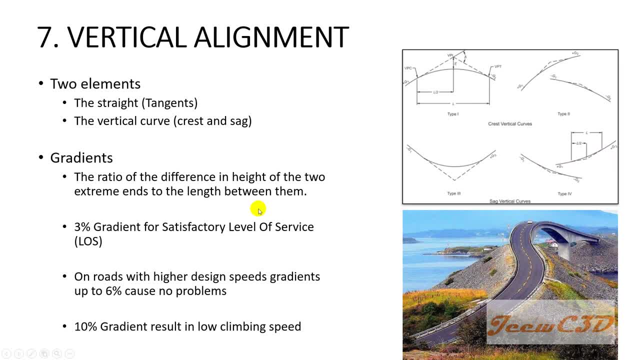 of curves are called sag curves. So in terms of the gradient of the vertical alignment, so up to three percent of gradient, you will be traveling without general similarities to the. lets say You will be traveling without cyber medicine. então, country of sickness. 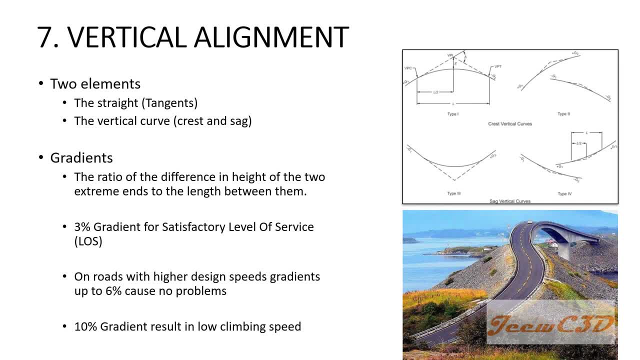 much problem when traveling. without much problem we specially mean the design vehicle that should be. usually it is a heavy vehicle such as a truck. so in vertical alignment we call it about 3% gradient. the heavy vehicles are not suffering when it is traveling. so when the gradients up to 6% there may be not. 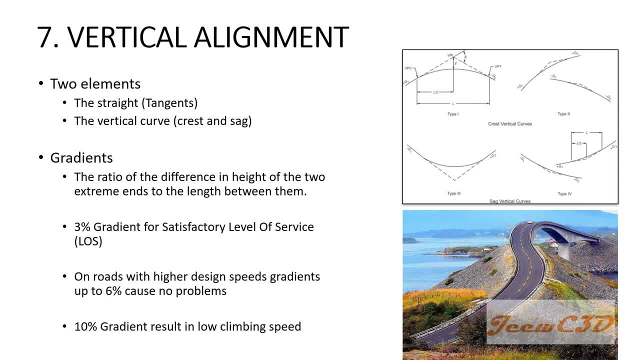 much of a problem, but when you have gradients higher than 10% there may be, they may be finding hard to travel on those roads. so, if you can remember, we travel from Kurunagal to Kandy around Galagajara. we have a two-way road. 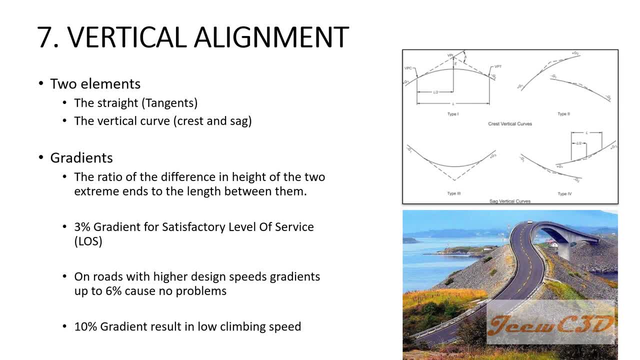 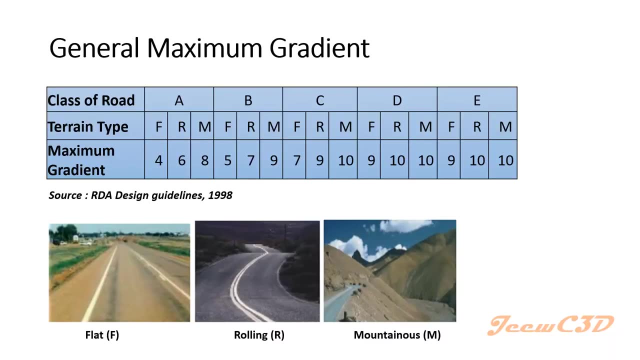 very sharp gradient area so the steep slope in the roads are present, so you can usually see these heavy vehicles. trucks are traveling slow in this area. so that is what happens when you have high gradients in roads. so the general maximum gradients according to RDA design guidelines are given in this. 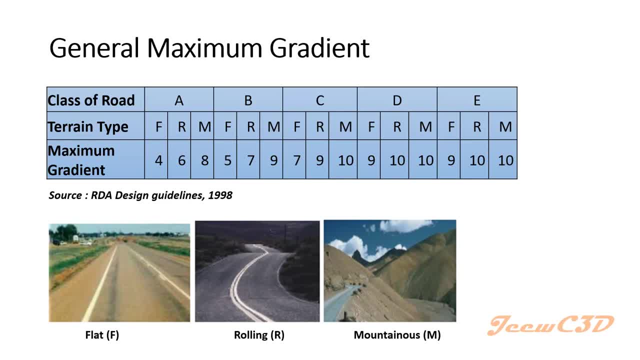 table. so they are given in terms of the class of the road. so you have A class B, class C and D, C, D and E. so this F means the flat terrain. a flat terrain means a terrain kind of level area. the topography of the area is a level. so R means the rolling terrain. in that 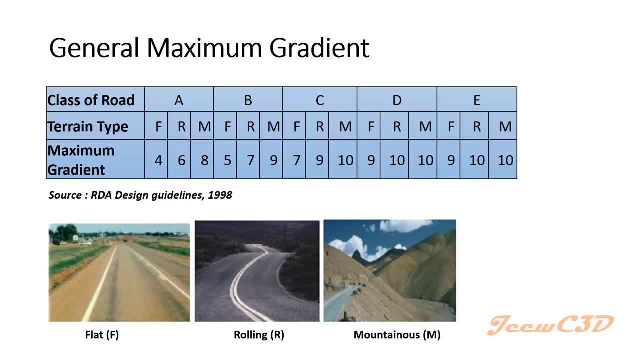 terrain you have the level condition as well as some gradient, so some mountainous conditions and if you call it when we come to a mountainous terrain for M, you have a mountain road, so you have high gradients at frequent intervals. so for a A class приход, if it is a flood rate, flat terrain- you can use up to 4% of. 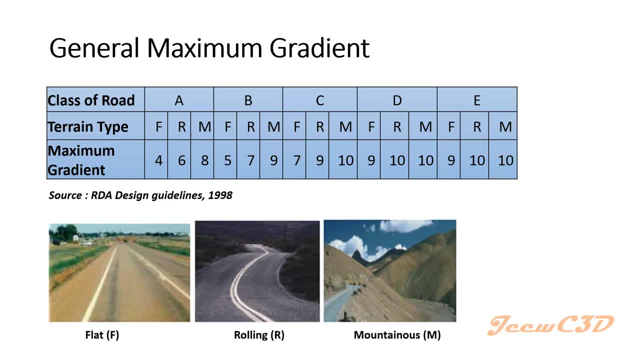 gradient for vertical alignment design. for rolling terrain you can go up to 63% C, for this жить水 gänd Daha six percent, and for mountainous terrain you can go up to eight percent. so when the level of the road coming low, lower, like b, c, d and e, you can go up to a higher gradient of the road. so then, 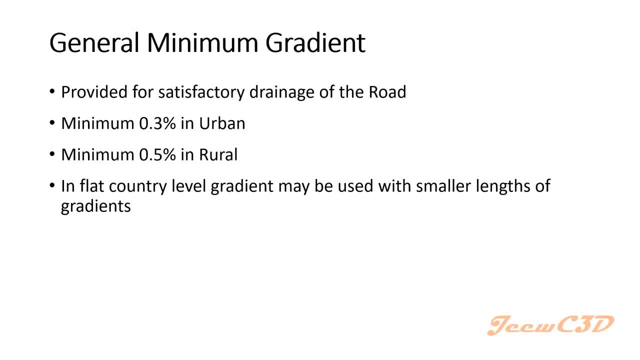 we talked about the minimum gradient. because you have a maximum gradient, so the you cannot have a level ground without zero to zero percent gradient. so you cannot have a flat road, because it is not good for drainage so water coming onto the road it will not pass through. on the longitudinal section. 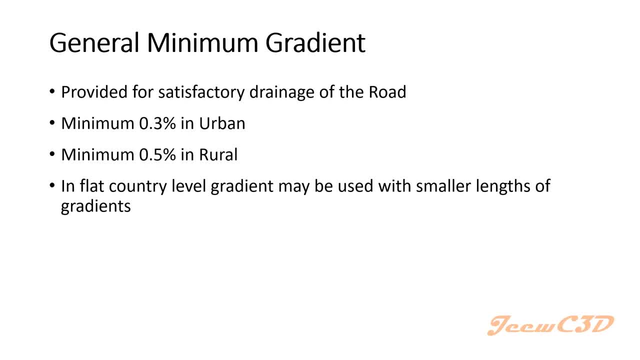 of the road on the cross section side of the road, if the water on the road would be passed through the super elevation. but if you consider about the longitudinal distance, it moves and it won't be draining off because if you have a level ground or as the road, so in that case we 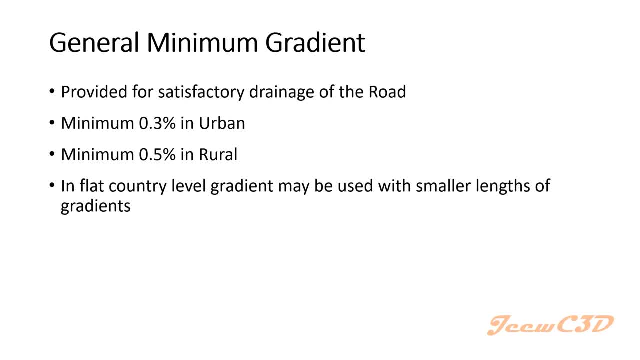 are using 0.3 percent gradient in urban areas and 0.5 percent gradient in rural areas, but in some flat areas you can use flat roads of smaller lengths without adhering to this 0.3 percent. you can use a small lens of flat gradient. that means, uh, zero percent gradient. so then we will. 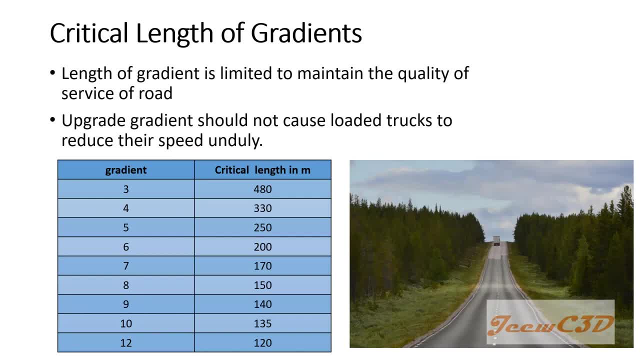 be looking at something called critical length of gradient. so when you have a gradient road, so like here, you have a gradient road. so if this gradient is too much, that means the length of this gradient is too much. heavy vehicles experiencing very hard travel, so it will hard for the vehicles to heavy vehicles to travel in this. 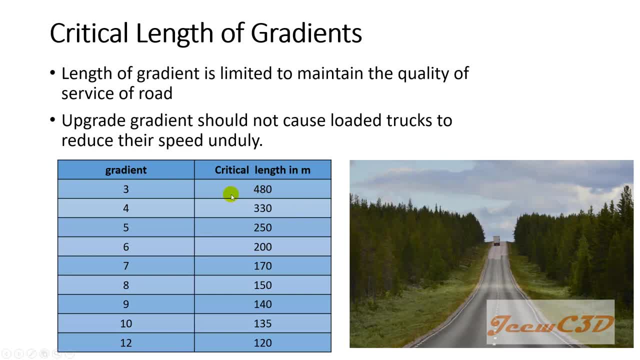 area. so because of that we are specifying maximum critic, maximum length where you have to go with certain gradient. so for 30 plus 3 percent gradient we have to go for a maximum length of 480. so this tangent length would be less than 480. this gradient length should be less than 480. 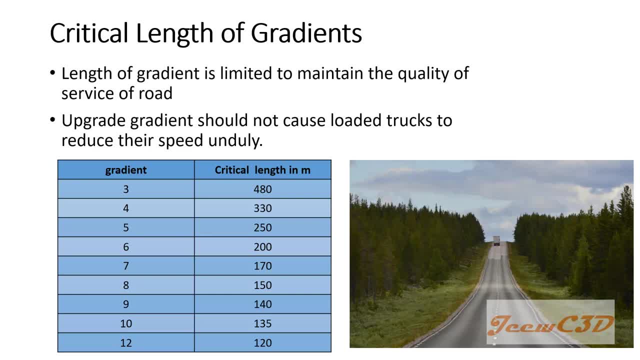 when you are designing. so when it comes to 480, you have to have a vertical curve and is the gradient and you again you can increase the gradient if you want- after the vertical curve. that means when you have a vertical curve you will be having a lesser gradient than the. 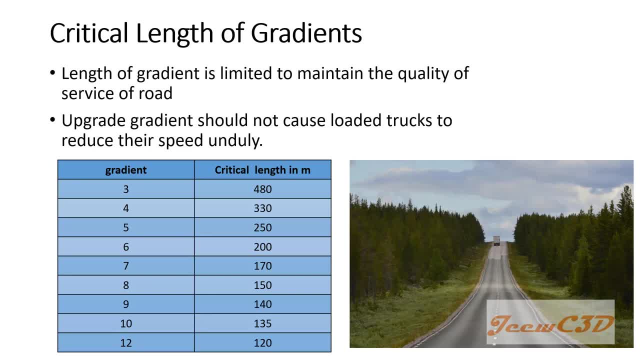 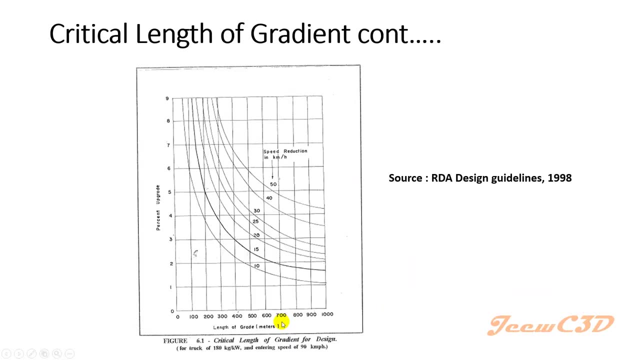 first gradient so will make the travel of the vehicle more easier. so according to the gradient you have certain critical lengths. you can see when the gradient is too high this critical lengths become very low. so this chart also gives a way to calculate. the can obtain the critical length according to the gradient of the road and also it. 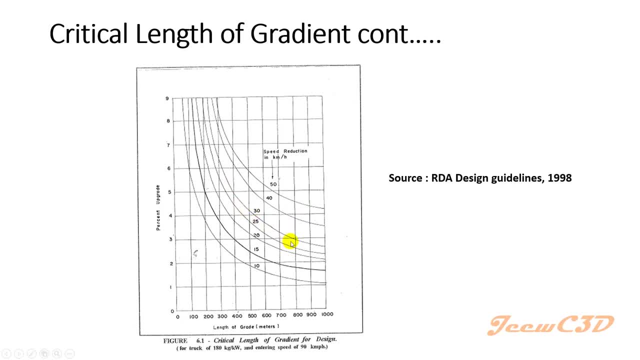 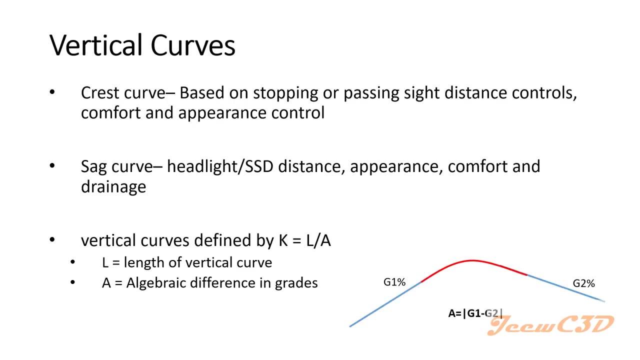 has the speed of the vehicle also. that means the speed reduction, how much speed reduction the vehicle will occur when it is traveling on a gradient section. then you have the vertical curve. so to know about the gradient, this thing, so to connect the gradients, these two gradients, we have vertical curves. they are called vertical curves, so you. 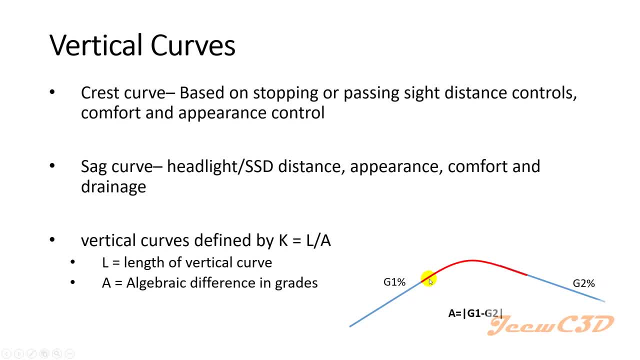 can have this type of crest curve. otherwise you can have this type of sag curves. so in these crest curves we are dealing with the stopping or passing side distance and comfort and appearance control. we will be talking that in a later slide. so in the sag curves, if you can remember, under side distance lesson we learned about headlight. 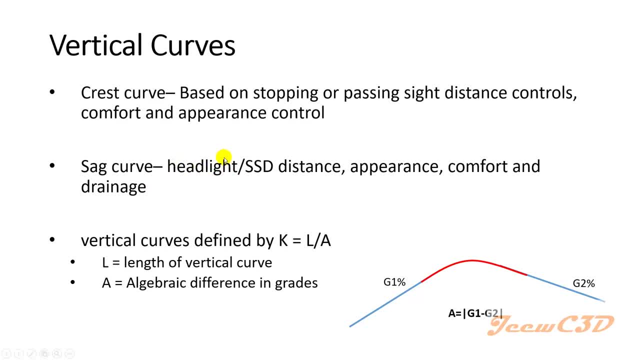 side distance. so in sag curves mainly we are looking at headline side distance and stopping side distance, apart from the appearance, comfort and especially the drainage criteria, because at a sag curve like this you have a sag curve, so in the center sag curve the water will be collected because of the shape. so we have to have more attention. 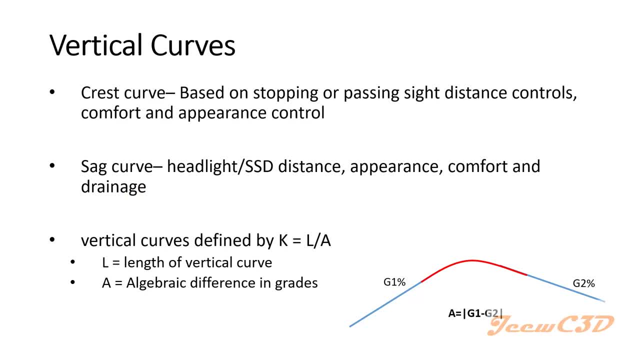 about the drainage part in that sag curves. so when you are talking about vertical curves there is a term called k where the curvature is defined. the term k, or the coefficient of vertical curves, equals to length of vertical curve over a, a means length of vertical curve. 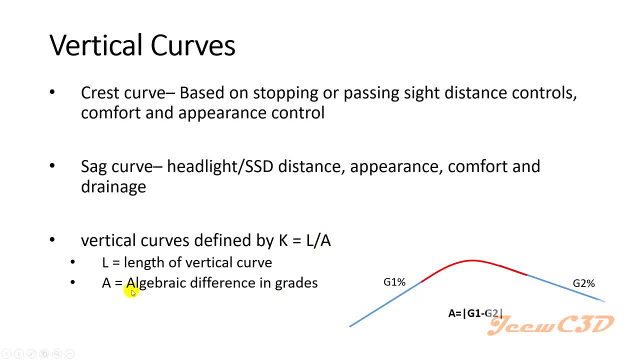 over a, the algebraic difference between the grades. So this a means g1 minus g2, and you have to get the mod of that value without the plus or minus sign. So this k value equals l over a. So the curvature is given by length over a value. So if you define, if you 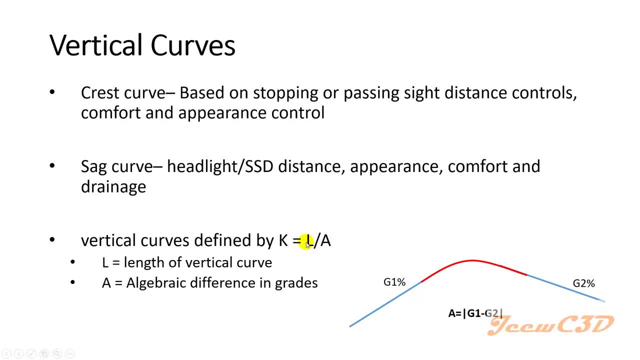 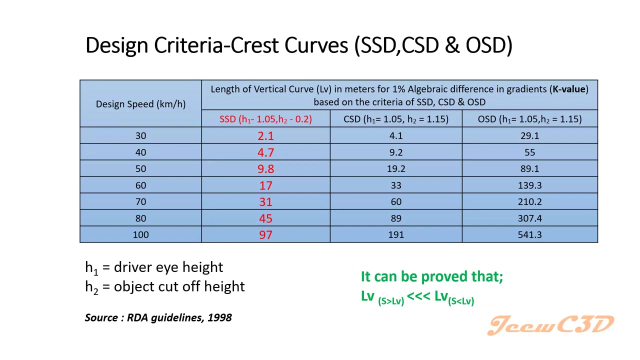 take this equation closely, you can see this. k means the length of vertical curve to have 1 percent gradient chain. That is the definition of k. So then we will be looking at what are the k values for designing each type of horizontal curves. So sorry, vertical curves. So first we 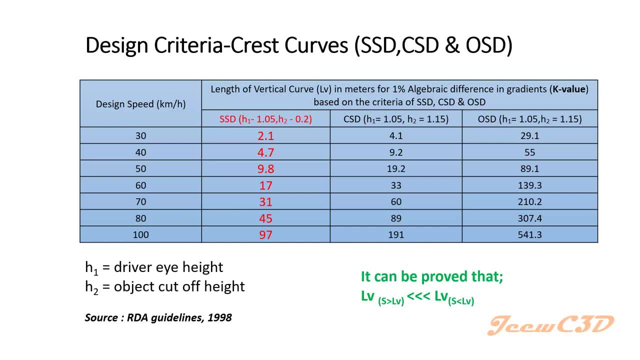 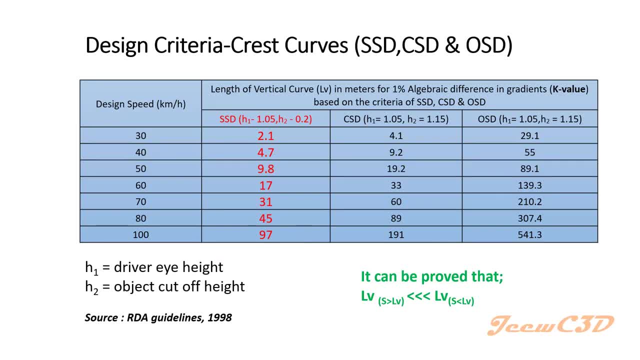 So everything will be defined in terms of k in vertical curves. Sometimes we define the things with length of the curve, but most of the time we define the vertical curves in terms of k value. So in this table you have the stopping side distance. continuation. 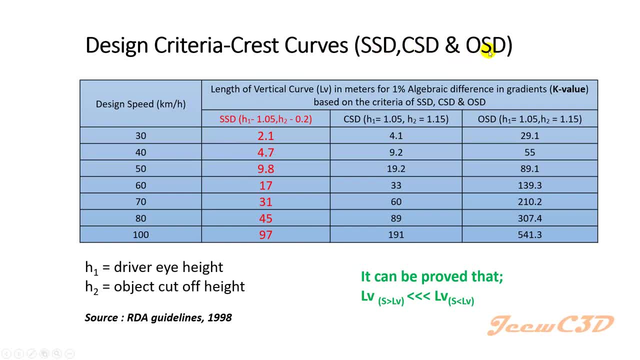 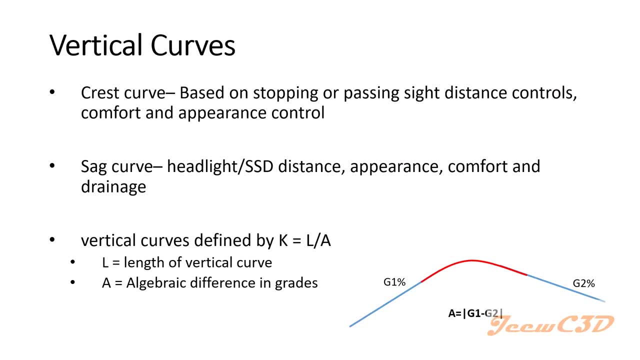 continuation sight distance and overtaking sight distance. they are at the crest curve. how much of k value you need for a vertical curve? so if you can remember, in the sight distance lesson there a vehicle is coming on this side and there is an object on this side. so we are calculating the sight distance so that sight distance should be seen along. 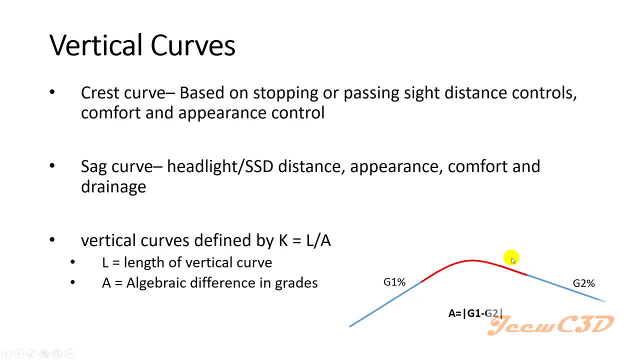 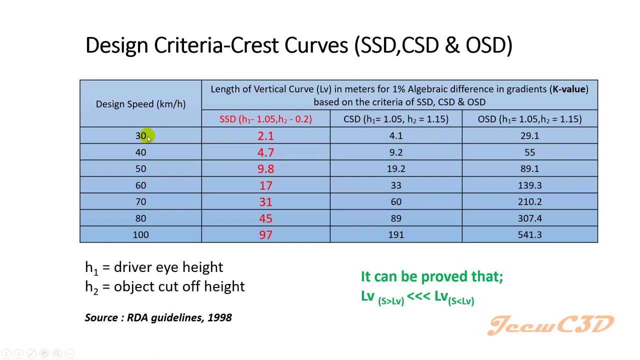 this vertical curve so that it should be provided by this curvature, otherwise it could be blocked by curvature. so what we are doing is we are providing that curvature to the road to have that satisfactory sight distance. so here, for design speed of 30 you have to have 2.1. 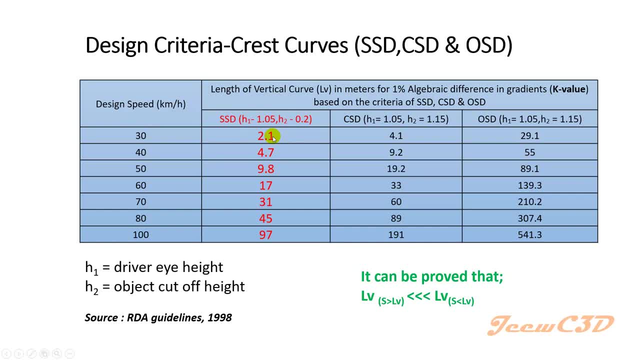 k value of your vertical curve should have 32 k. so now we should have calculated the of the vertical curve in this manner. so we are starting have a k value. this crest vertical curve should have a k value of 2.5- 2.1 to have satisfactory. 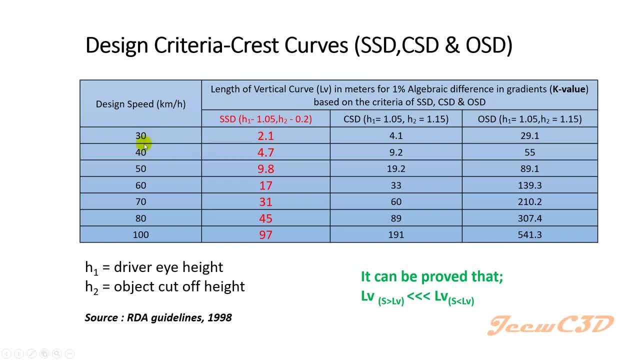 stopping side distance. so when the speed is increasing, you can see the k value is also increasing. so in this calculations, when you are getting this length, we are considering h1 as the driver height, which is 1.05, and h2 as the object cutoff height, which is 1.2. 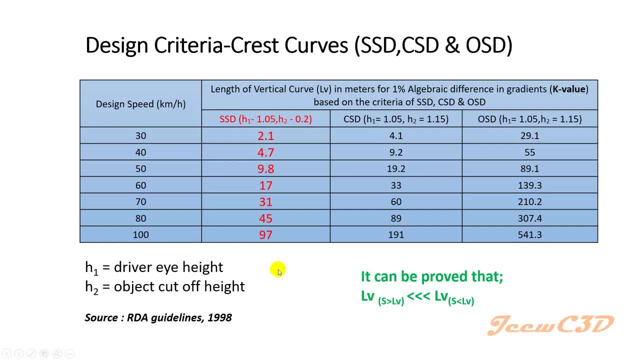 so there are two locations where side distance can be considered along with the vertical curve length. that is, length of vertical curve where side distance is greater than length of vertical curve, and the other one is length of vertical curve where side distance is less than the length of vertical curve. but when you have, when we do the calculations, 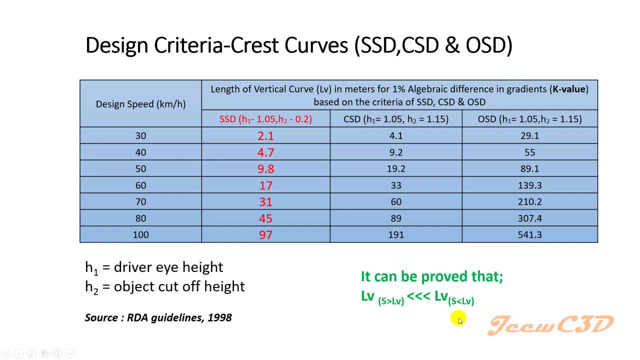 we can prove that this length of vertical curve where side distance is less than the length of vertical curve. that means if the side distance is 30 and length of vertical curve would be 35 or 40. so in these situations we are only calculating these things. that means where your side distance is greater than length of 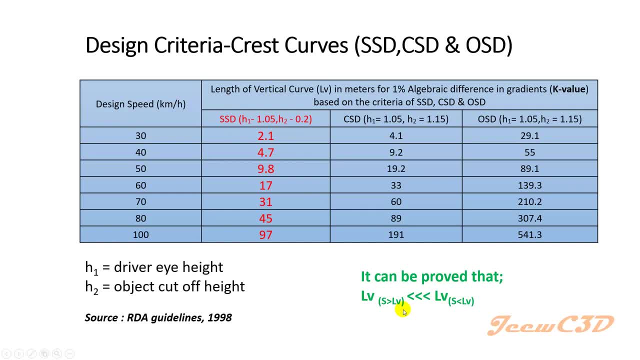 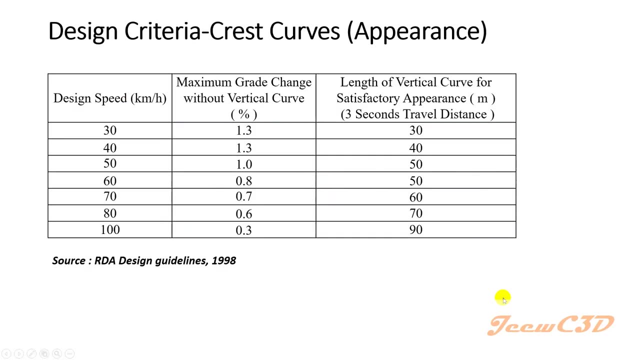 vertical curve. we are not considering this because this LV is greater than this LV. so we always consider in calculations our length of vertical curve is greater than the side distance when you have the rest curve criteria for appearance. so appearance criteria we are considering the curve length instead of 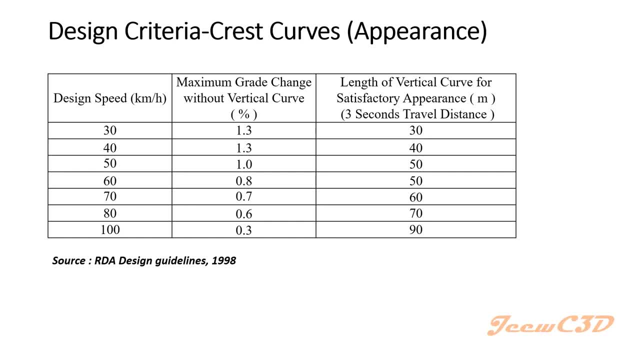 a K value. so if you have have a very shorter vertical curve it is not. it is not giving good appearance. very shorter vertical curves will not be giving good appearance. so to give good appearance you should have kind of 3 seconds travel time for the vertical curve. so if the design speed is 30, your vertical 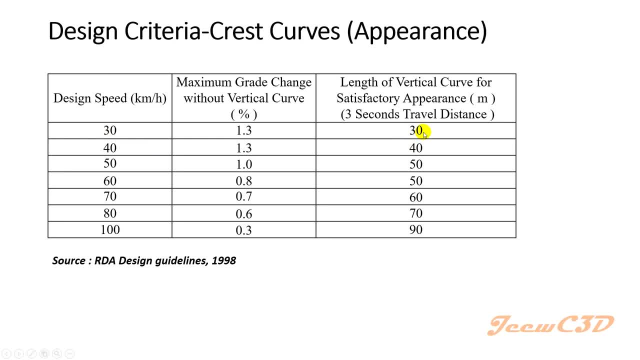 curve length. for crest curves it should be at least 30. so gain for 40 it should be 40.. for appearance criteria: this can be used in sag curves also otherwise, because this appearance criteria would be catering crest and sag both, but it is defined for crest curves. 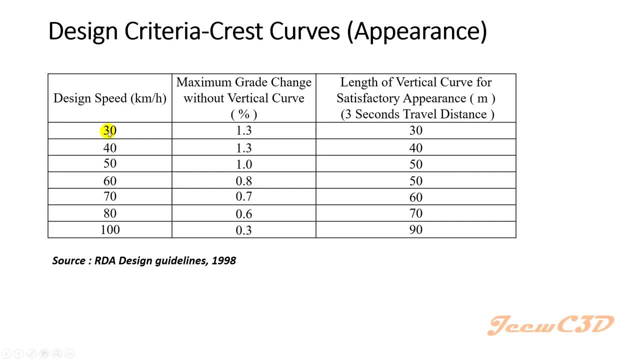 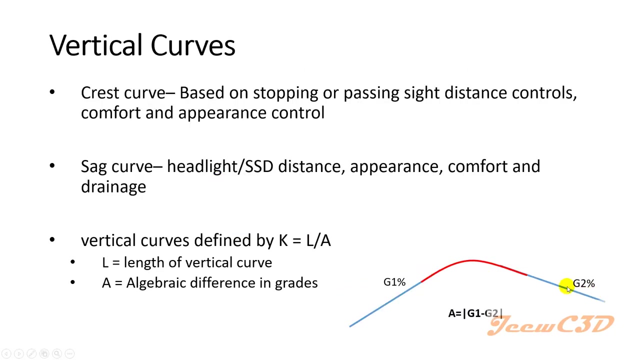 this 30, you have 30 meter length of vertical curve. or if it is the design speed of 60, for design speed of 60, you can have to have 50 meter length. so sometimes if the gradient change, so this gradient change is very low. if this gradient change is very low, you can avoid a vertical curve. 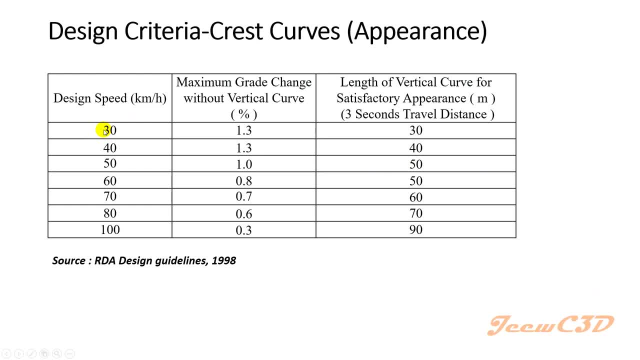 so for design speed of 30, if the gradient change is less than 1.3, you can avoid a vertical curve and only retain the two tangent section. so if you can, if you can consider a situation where you have one percent upgrade and again it is upgrading at a nine percent gradient. so the percentage 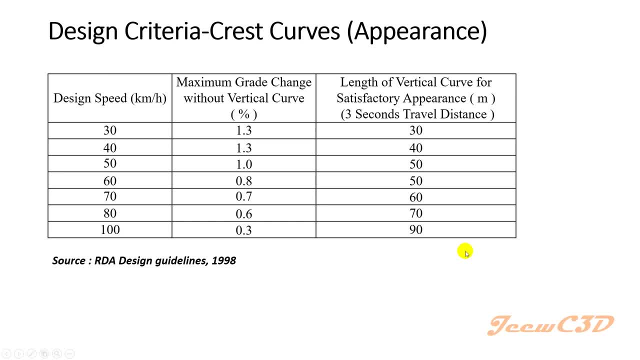 change is point one percent. so that case, for a design speed of 30, you can have 1.3, uh or less. sorry. so if, since this gradient changes 0.1, it is less than 1.3 if the design speed is 30 or 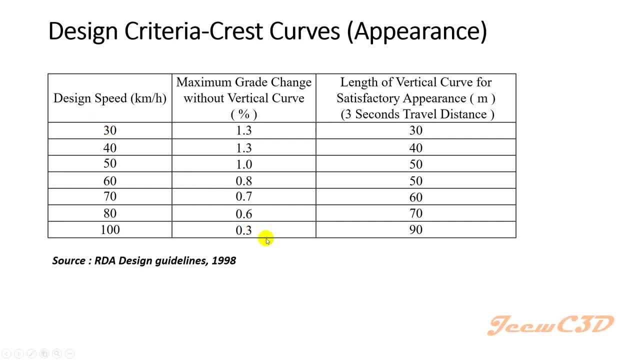 even up to 100 meter gradient, 100 meter design speed, you can have that section without a vertical curve. So sometimes you may encounter this kind of situations where the gradient change is less than these values. So you can design the road without a vertical curve. 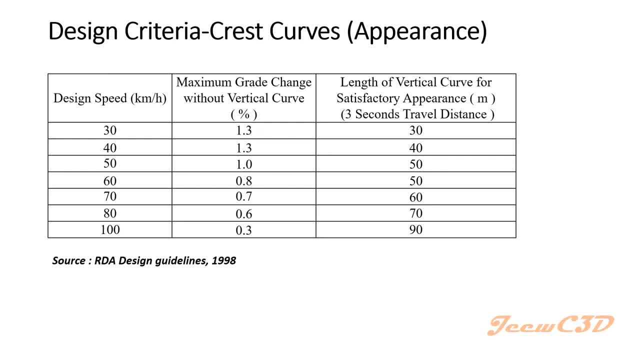 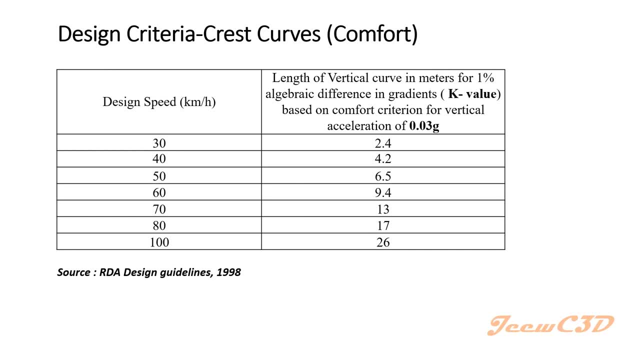 So then we are considering about something called the crest curves, with comfort criteria. Sometimes, when you are traveling on a road, you might feel that you are at some vertical curves, you might feel that you are going like over the top of the road, or you are feeling like very hard to travel in that road due to the speed. 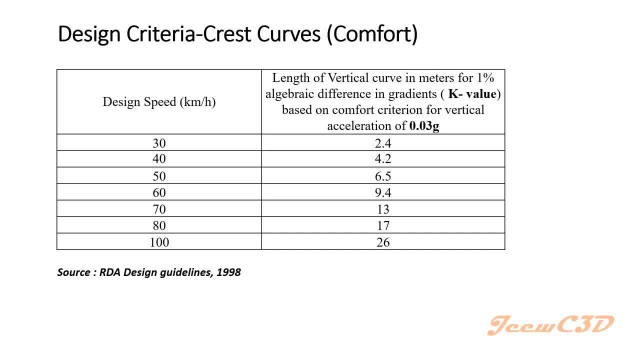 So that means the comfort criteria of that vertical curves are not there, So we have to have the vertical curves to satisfy the comfort criteria also. So in that case the K value should be 2.44 design speed of 30 kilometers per hour and 4.24 design speed of 40 kilometers per hour. 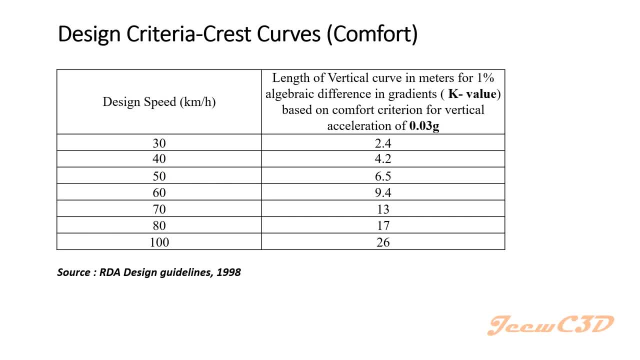 So if you consider that, So let us consider about example, If this gradient change is in a vertical curve, if the gradient change is 3%, if the gradient change is 3%, so then this value should be multiplied by 3, because this is the value for 1% gradient change. 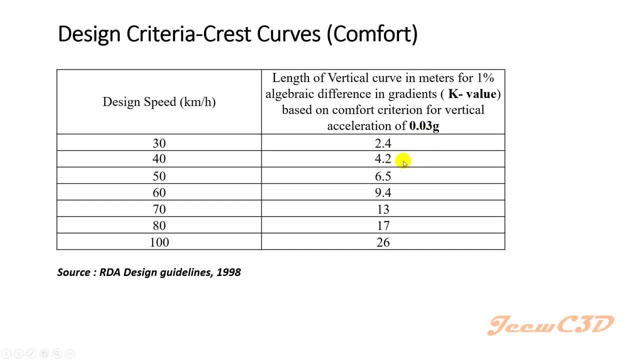 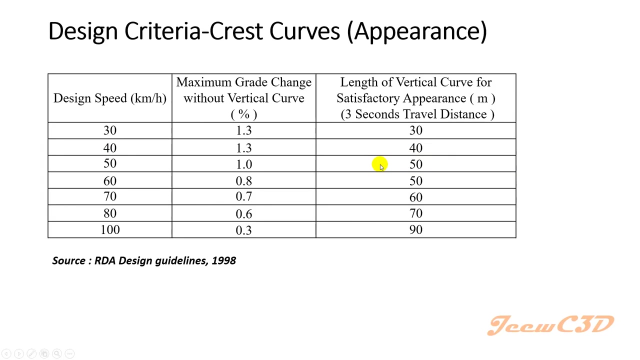 If it is 3% gradient change, you have to multiply it by this. multiply this 4.2 by 3%, 3, that means about 12.6.. So you have to use the vertical curve of curve length of 12.64 higher. But if you consider about 40 and if this is 12.6, but for the appearance criteria you have to use vertical curve length of 12.64 higher. 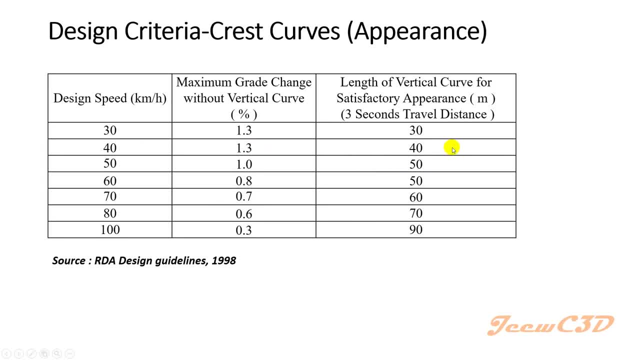 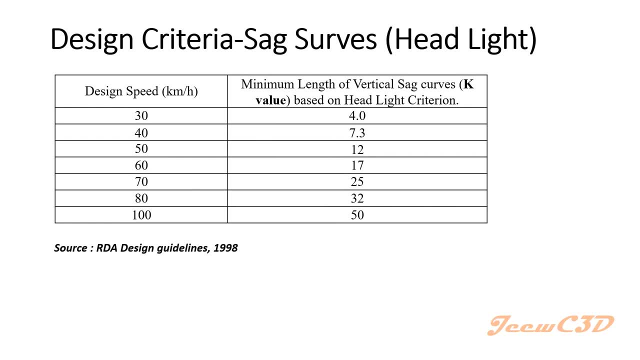 So this value is a drift of 50. So you have to consider all these facts when selecting the vertical curve length. Then we are going to the sag curves. In sag curves we are especially dealing with the headlight sight distance. 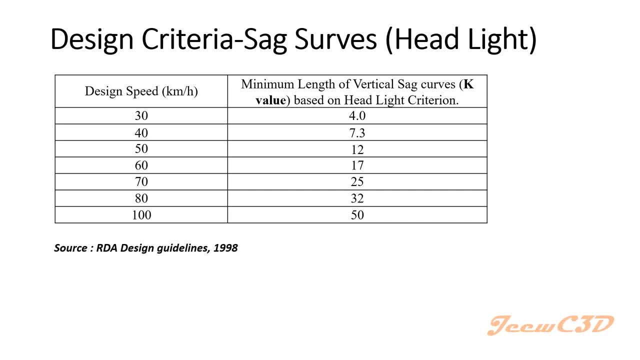 So in terms of the headlight criteria, the K values of the sag curves would be: for 30 kilometers per hour, it should be 4, and 40 kilometers per hour, it should be 7.3.. Like that that. so then you have something called design criteria for sag curves, for. 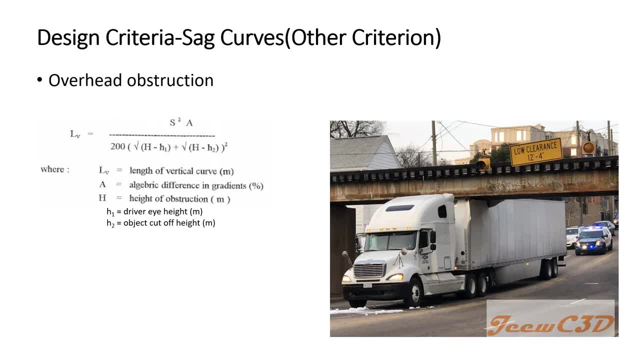 overhead obstructions. so under sight distance criteria we learn about the overhead obstructions, especially for sag curves when we have underneath road and we have overhead obstruction, so we have to check the vertical clearance properly and actually when you have overhead obstruction you have to make sure this obstruction will not obstruct the sight line when the 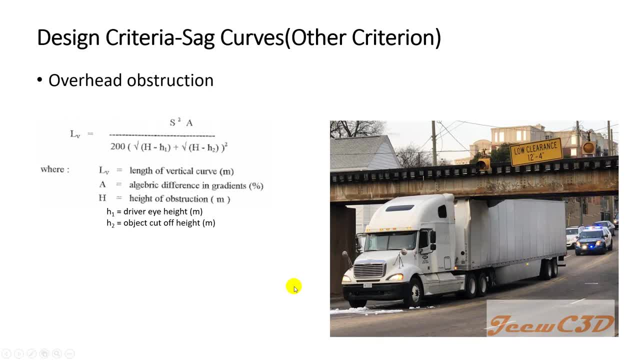 vehicles are coming at the top of the road, so this can be calculated using this equation: this length of vertical curve to satisfy this criteria, so that this vehicle is this sight distance is not blocked by the head obstruction. this is given by this equation where you have the 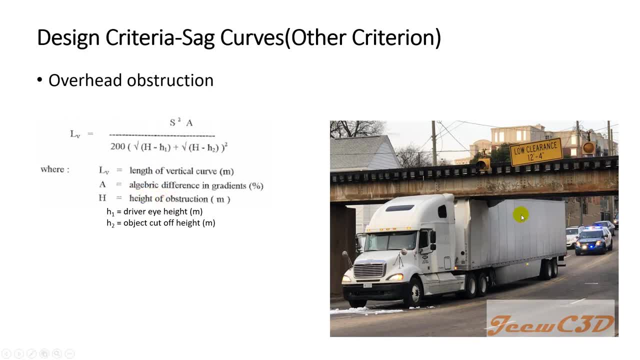 height of obstruction from this pavement surface and h1 will be the drive-in height and h2 would be the object cutoff height. so this is about the vertical alignment designing, uh, road, highway design. so when you are designing vertical curves and gradients, you have to think of these factors. so in actual terms, these are derived. with so many equations i haven't 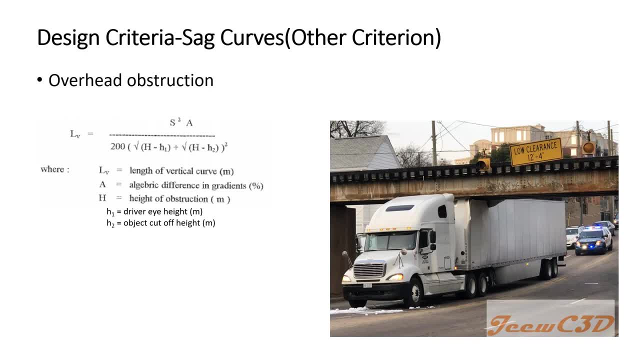 put these equations in here because of the time constraints, but when you are going to a job or when you are reading more about these things, you will come across- come across so many equation derivations, so you will be seeing how these equations are derived from basic principles. but 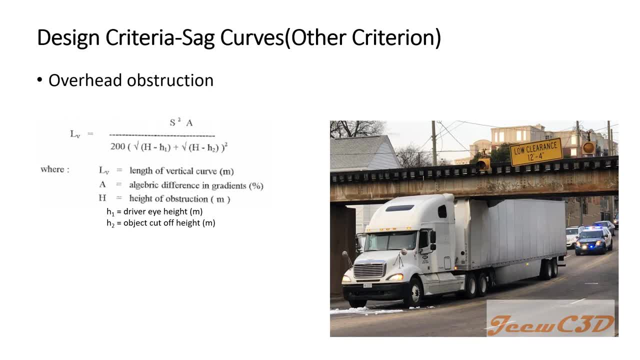 at the moment i am giving you the equations- how to calculate these things and how to apply these things into a real design world. so at the civil 3d class we will be looking at how to apply these things in real world alignment design. in the next class we will be looking at the horizontal and vertical alignment coordination. we 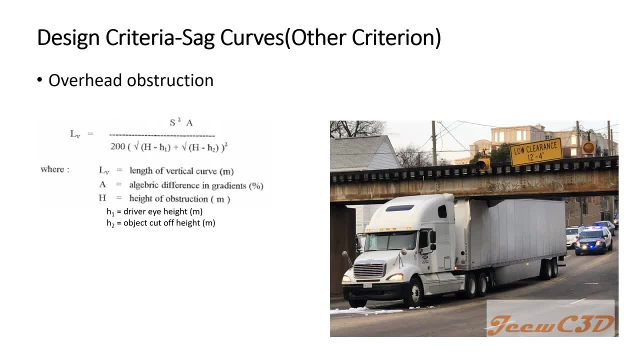 are, we have we are. when designing codes: yeah, we need to consider the horizontal alignment and vertical climb alignment- uh, both together to get a very much desirable code for much safety and efficient driving. so in that section we will be learning how to combine horizontal alignment and vertical alignment together to have a better road. 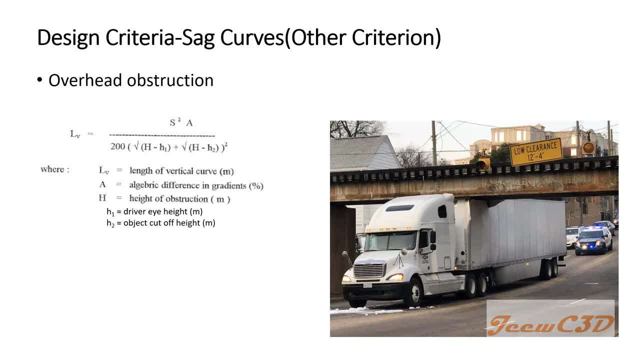 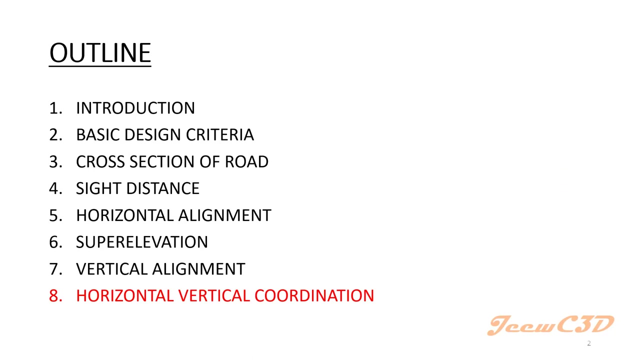 so after that we will be looking at the civil 3d class, where you can design your own roads with horizontal and vertical alignments. in this video we are going to learn about horizontal and vertical coordination of geometric design. uh, so far we have learned up to seven. 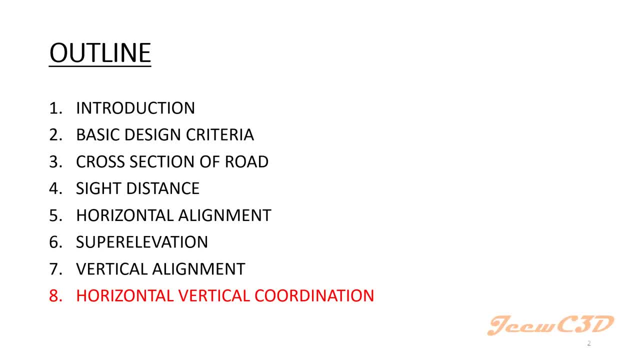 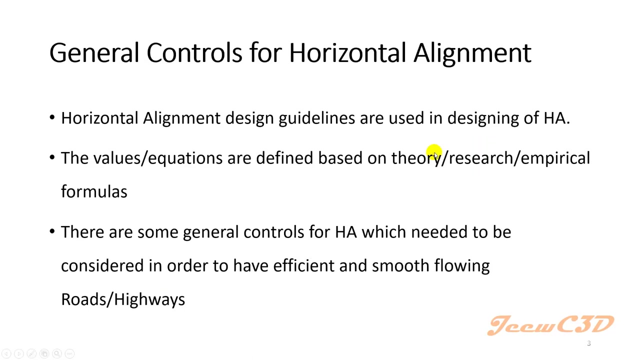 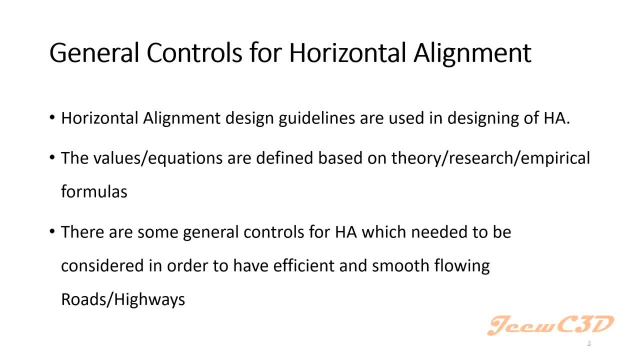 formulas and by engineering theories, but when you are applying this to an actual roadway, you have to think beyond the theory and research to empirical formulas and apply what is suitable for the scenario, so otherwise you won't be having efficient or smooth flowing roads or highways. to do that, we have general 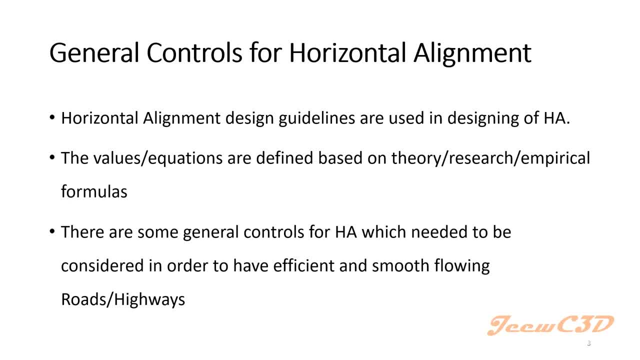 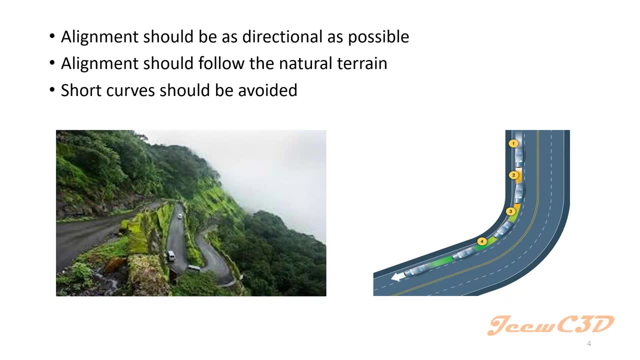 controls for horizontal alignment, vertical alignment, as well as both horizontal and vertical alignment. in this section we are looking at the general controls for horizontal alignment. one thing we have to consider is your alignment, or the road should follow the natural terrain as far as possible. in this left side image you can see this is a hilly road, but the road 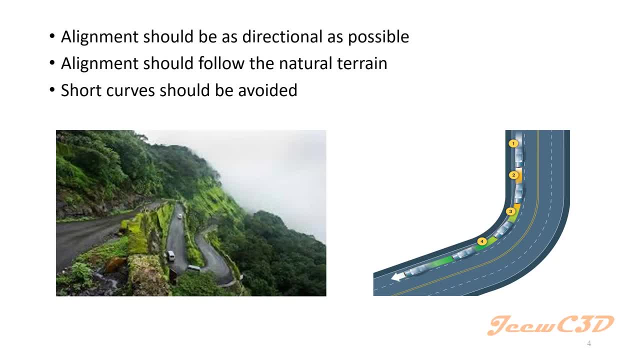 road is coming on the contours, so it is following the natural terrain, then we have to avoid as much as shorter curves. you know we should not use shorter curves in designing the horizontal alignment. shorter curves make driving uncomfortable. here in this right side image you can see there is a very short curve, a sharp short curve, so the driver's would not be, would not feel. 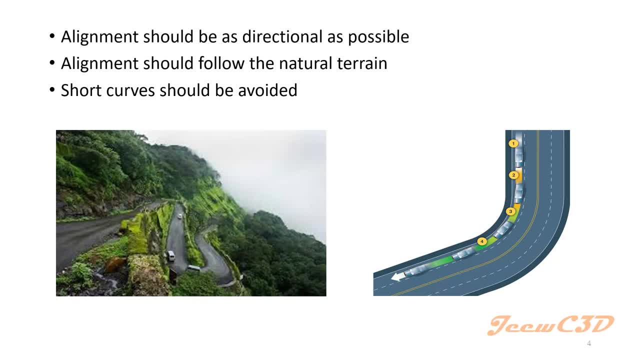 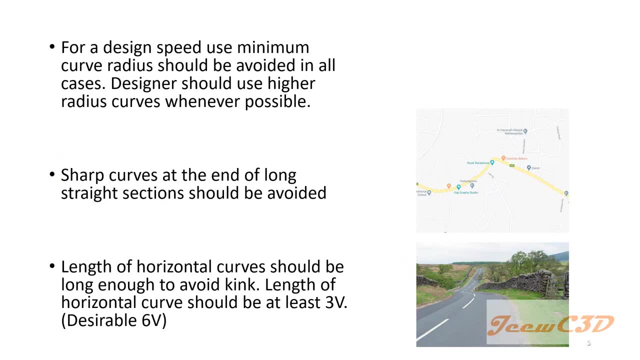 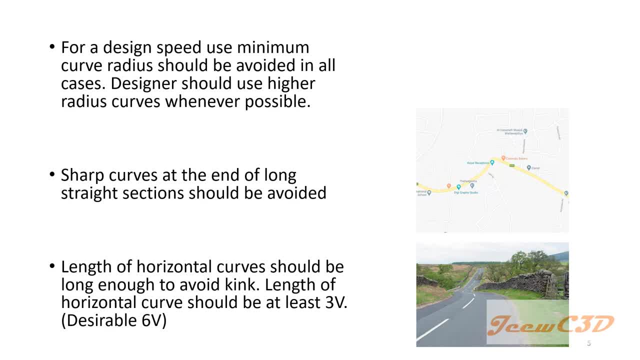 tables according to various design speed: how much of radius we have to use according to super elevation. for example, if you are designing a curve to 30 meter design 30 kilometers per hour design speed, so to have super elevation of 2.5, you should have a minimum radius of 35. that does not mean you should always use 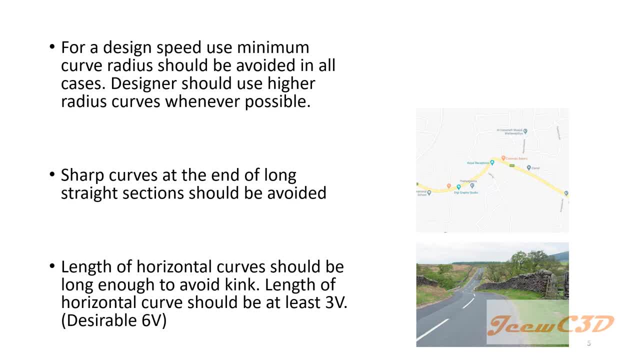 35 meter. you have to use higher, super higher radius as much as possible. if there is room or space there, if there is space for design, so in that location, installation of a 35 meter radius curve. if you can have 50 meter radius curve, you have to put that radius. 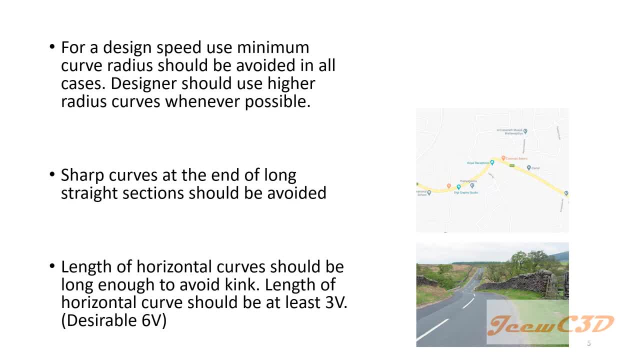 because that may be that makes the driver more comfortable in driving in that section. so you have to use a desirable radius instead of the minimum radius, the absolute minimum radius. you have to use a desirable radius which is larger than the minimum radius. then you have to avoid. 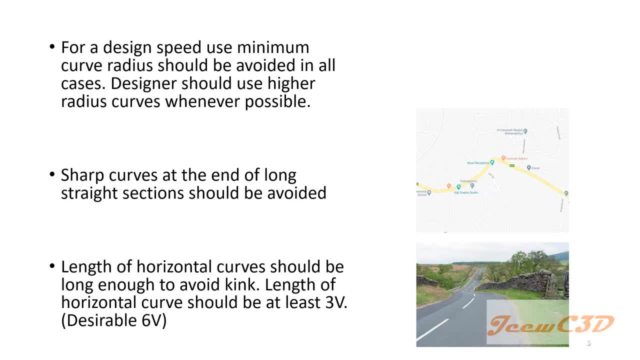 sharp curves at the end of long straight section. in this top image you may see this is a long straight section. all of a sudden you will be coming on a sharp curve. so this kind of curves might be very dangerous in the night time because when the vehicle comes from this side. 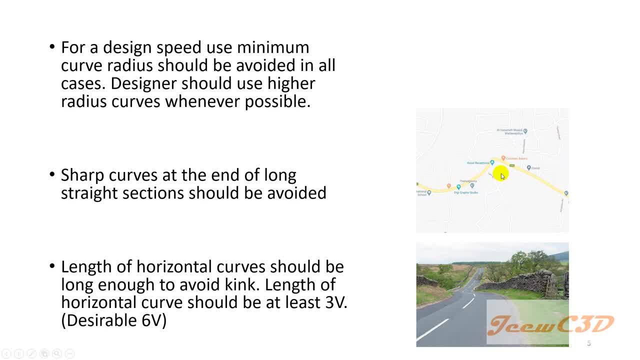 he may not see the curve at once. so accidents may be very frequent at at this type of location, so you have to avoid them as much as possible. then you have to use the user sufficient horizontal curve length to avoid the v of a kinks. so it says you have to at least use 3v for your horizontal. 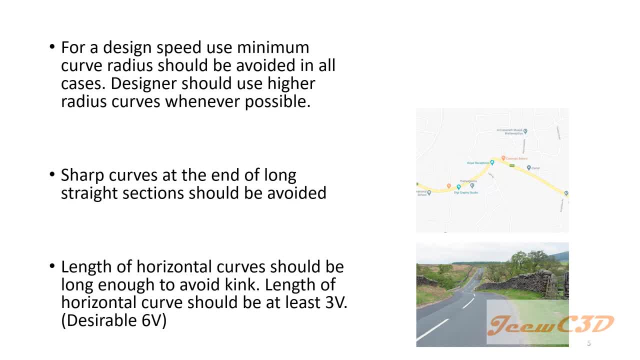 curve length means if your design speed is 100 kilometers per hour, so your curve length should be at least 300 meters, like that. so that is how to use the curve length, but that should be the least value. the desirable value would be 6V. so if 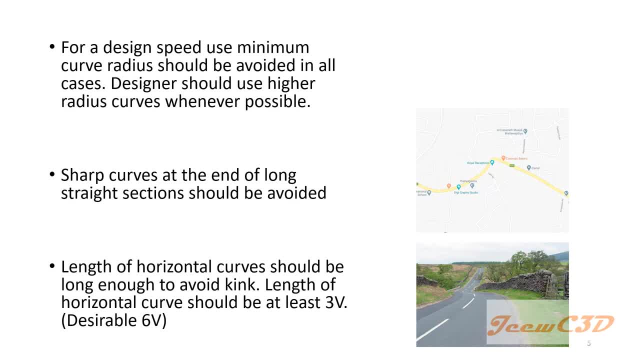 your of your design speed is 100 kilometers per hour, your desirable curve length would be 6V. that should be 600 meters. so if you have shorter curve lengths, you may can see this is a very unpleasant view of the road. we call it kink, so to avoid the shorter horizontal curves we have to use 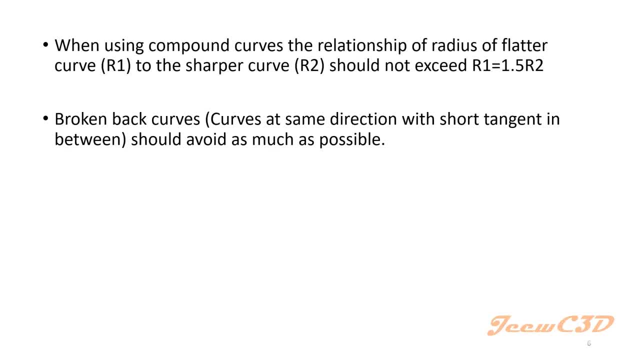 sufficient length of curve. then when using compound curves, that means curves which going on the same direction without a tangent. so when you are using that kind of curve the radius ratio should be: r1 equals 1.5. r2, that means the larger radius curve should be. 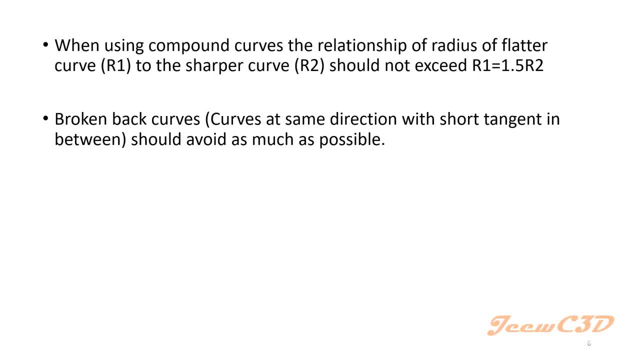 equal or less than 1.5 times the sharper radius curve, then you have to avoid broken back curves as much as possible. broken back curves means two curves rotating in the same direction with a small short tangent or small straight section in between. so we have to avoid that. 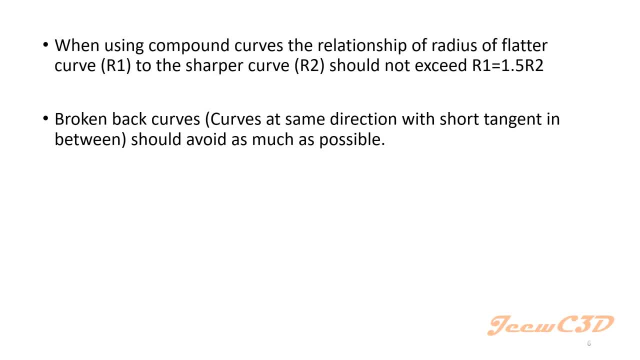 broken back curves as much as possible, because when there's a straight section after the curve, driver feels that there's a straight portion, so in that straight portion he might increase the speed. but all of the sudden he will come across another curve, so that might be undesirable for the driver or he might 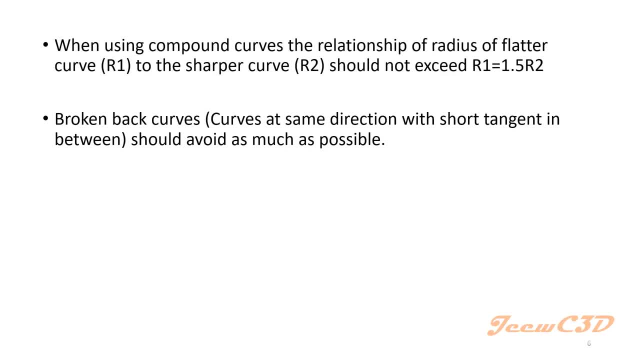 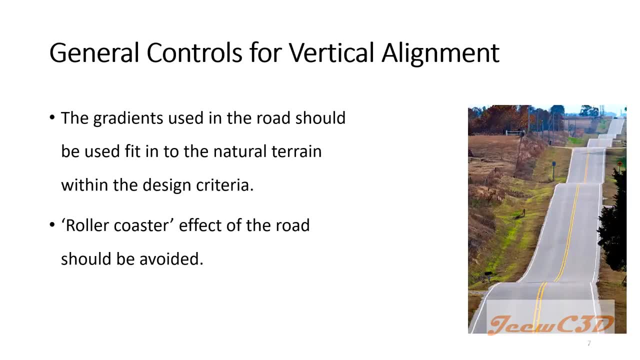 face unexpected conditions due to this curve behavior, then we will be looking at the general controls for horizontal vertical curves, vertical alignment. so, as I said earlier, the gradients and the vertical curve should be used to fit the natural terrain, but in doing so you should not make the road with the roller coaster effect. 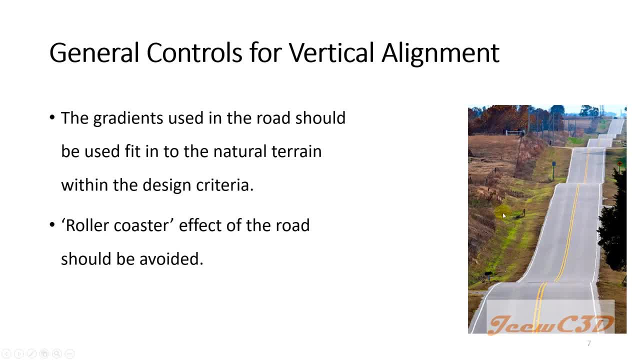 so in this case you can see this road is looking like following the natural terrain. but this is kind of a roller coaster road so you can, if you are here, you might see, might see you may not see the vehicle coming in this sag curve, so this is called the roller coaster effect. so you have to avoid that effect when. 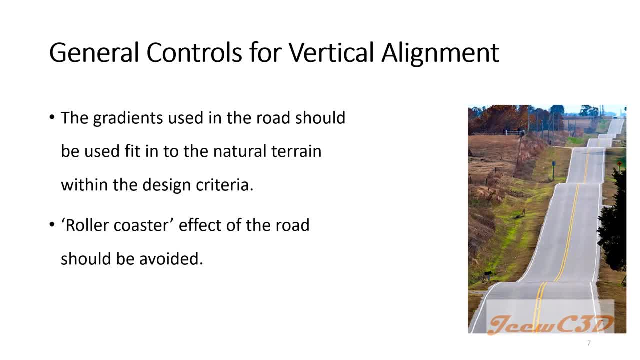 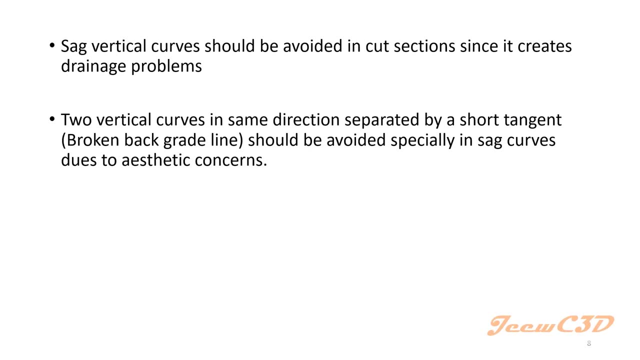 designing the road when you are following the natural terrain. so instead of that, you have to use suitable method to avoid that effect and follow the natural terrain. then sag vertical curves should be avoid in cut sections. if you can remember a sag vertical curve, which is a curve like this, so in sag vertical, 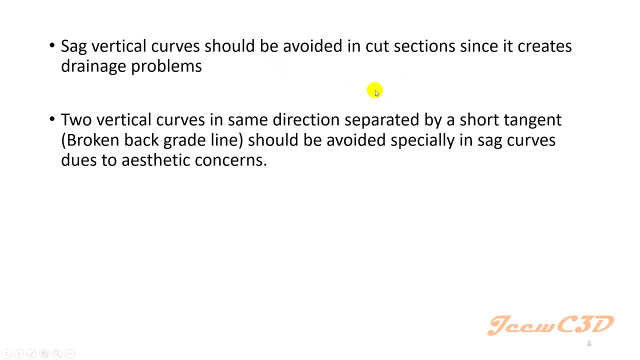 curves, the water is collected at the center. so if you have a cut section, that means the road is going through a mountain, you have to cut the road to, you have to cut the existing road ground to create the new road. so in that sense, there will be a section where the 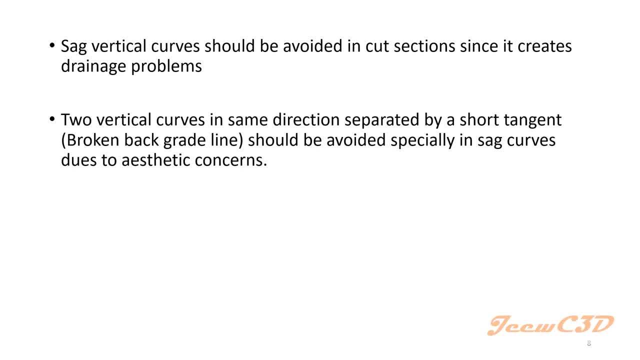 water is collecting at the center of the curve, since there is a cut section. you you have to put more effort to remove the water out of the cut section, because if there is a fill section, water will automatically drain out through the fill section because road is at a higher level and the natural ground is at a 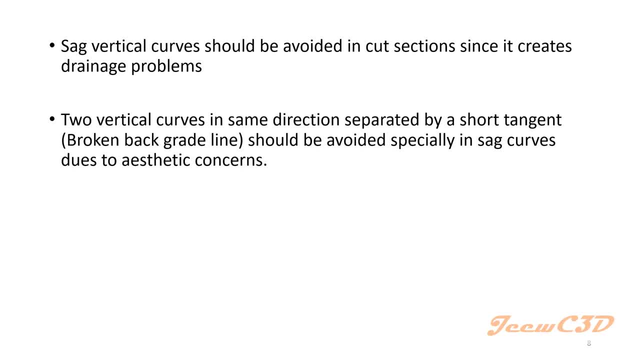 lower level, but in a cut section what would happen is the road is at a lower level, then the natural ground is at a higher level, so it is hard to drain out the water. so you have to avoid sag vertical curves in cut sections, then two vertical curves in same direction, separated by a short tangent which is 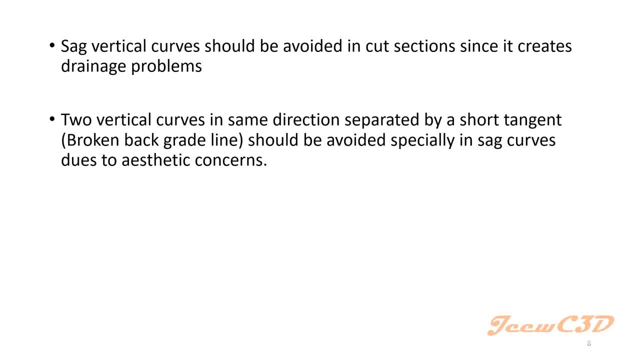 called broken curve. broken back grade line should be avoided, specially in sag curves due to static conditions. I think you could understand this thing. so two vertical curves separated by a short tangent. so I explained the behavior in the horizontal alignment which is meant by the broken back horizontal curve. so same thing happens here: broken back. 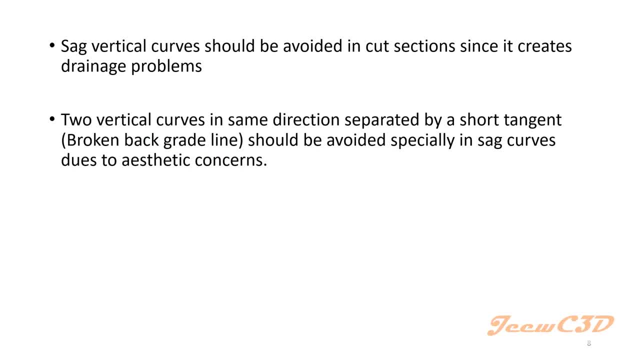 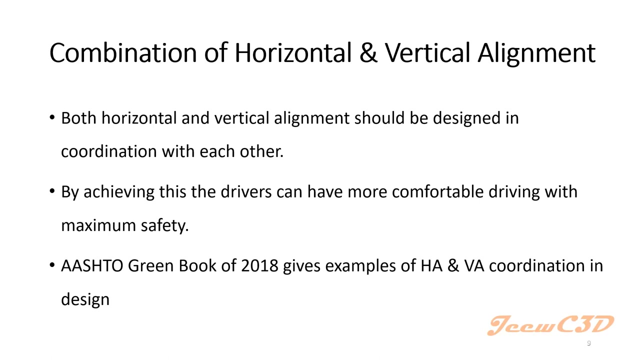 grade lines should have two vertical curves with a short tangent in between, especially in sag sections. it will be very hard or it will be very unpleasant view due to this broken back grade line effect. then we will be looking at the combination of this horizontal and vertical alignment. I will explain in the 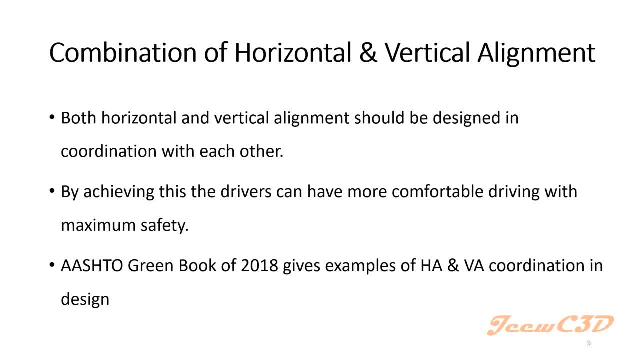 initial part of this lecture thought we looked about the horizontal and vertical control by individual sense- horizontal only and vertical only- but in this now we are looking at both of them together. so how can we use both horizontal and vertical alignment together to have a better driving, comfortable and better safety and better? 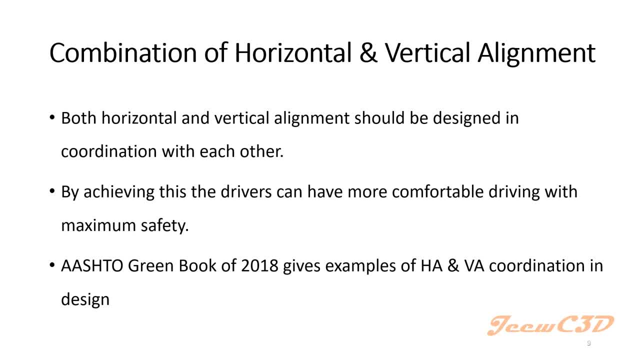 code in our design perspective. so Astro Green Book 2018 gives some examples of horizontal and vertical. this HA and GA means horizontal alignment and vertical alignment, coordination in design. Astro Green Book means that is a design guideline used or developed in USA. so this is this 2018 version is the. 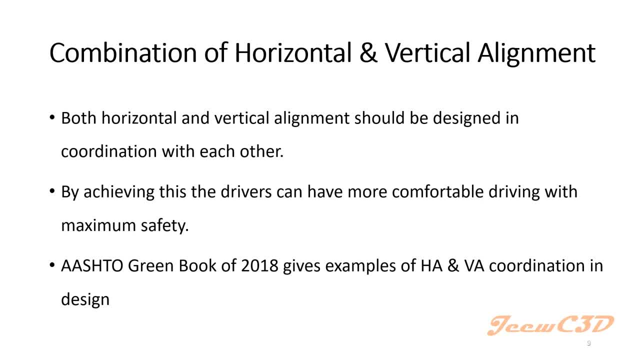 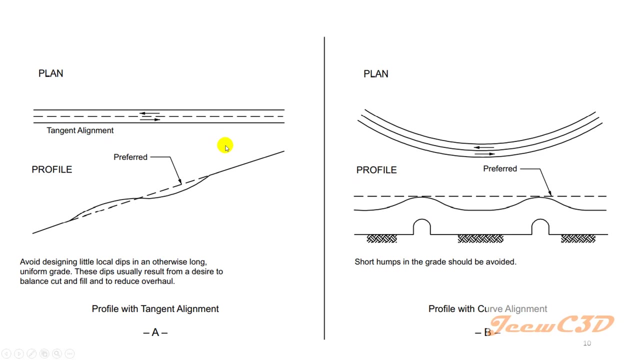 most recent version it gives some examples of horizontal and vertical alignment coordination. so you have other versions of this book also. it and those this at those books also we have the same examples. so these are some of the examples you have to follow in horizontal and vertical alignment to have a better 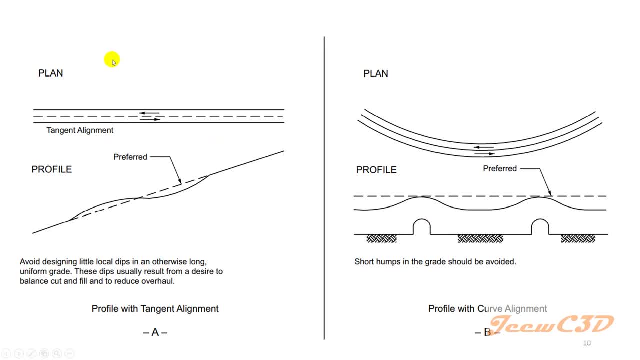 coordination. so in this you have to note that in America the driving direction is eles applying dynamic action lighting very opposite from ours. so they are driving this day on the left side of the road, in blood road, and this day on the right side of the road. 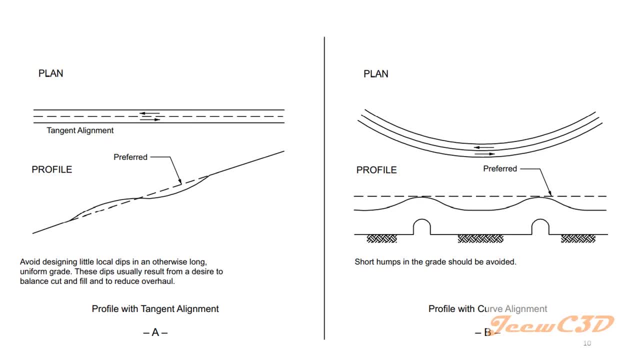 so in Sri Lanka we are going the other way. apart from that, we have all those things have to be followed as it is when you are designing. so if you have a straight section here, but it described is, you should not have a crest curve and a sag curve like this when you are designing. instead, you can have a straight, tangent section. 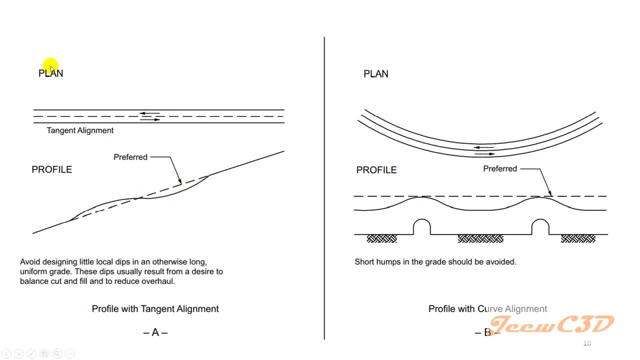 in the profile, also in your plan or in the horizontal alignment. if you have a tangent section, you can have a tangent section in vertical profile also. here it says: if you have a curve, you should not have bumps in your profile like crest, sag crest. so you should not use this kind. 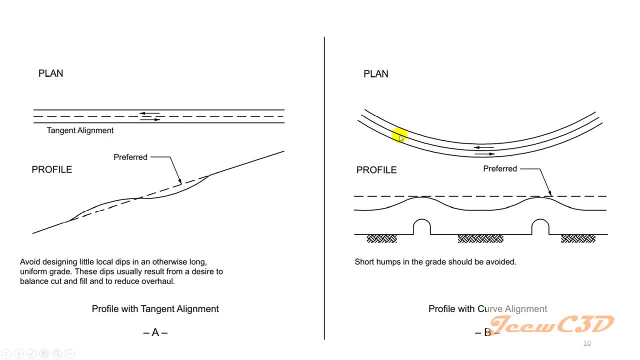 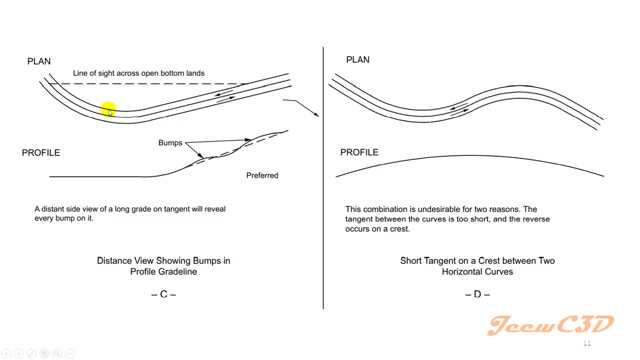 of behavior on your profile if you have a plan curve on your horizontal alignment. so if your horizontal alignment is a curve, your vertical alignment should not be like this. instead you can have the vertical profile, some kind of a grid. then you have this thing: you have a curve here and you have a straight here in your horizontal alignment. 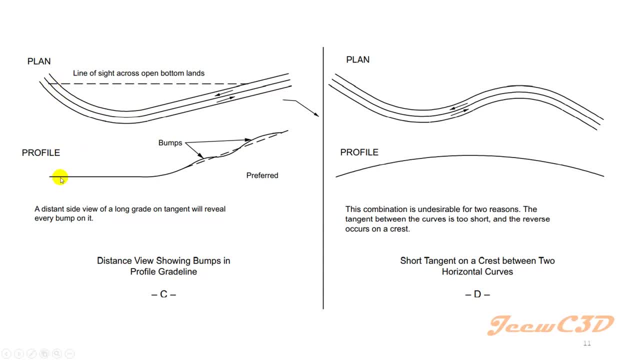 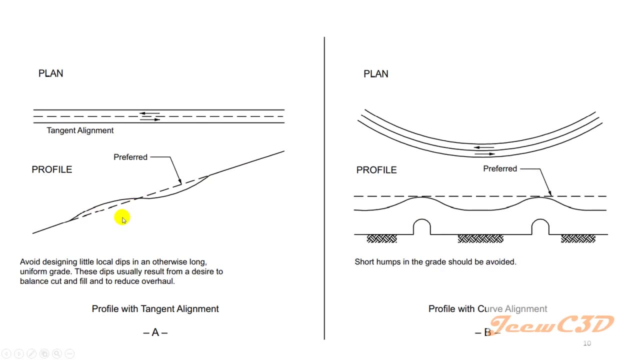 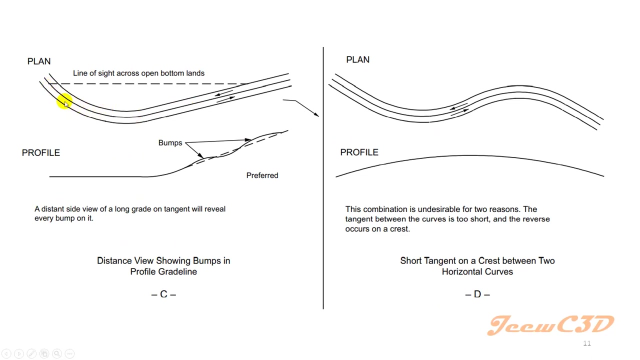 here you have in the profile, you have a lower ground here and a high ground here. so if you have vertical curves like this in, as this in the initial example, like this, so the vehicles coming from this side, according to this image, the vehicles are coming from this side, so it will make an unpleasant. 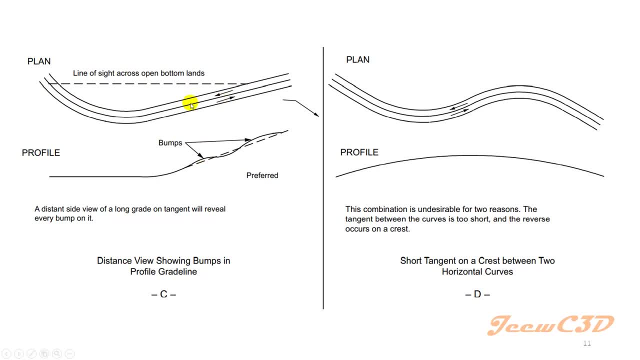 on the road. if you design the profile like this, so instead you can have single grade, here you have a short tangent in between the horizontal curves. this is a reverse curve separate by a short tangent, so this is called. this is not desirable for two reasons, that is, this tangent is not desirable. 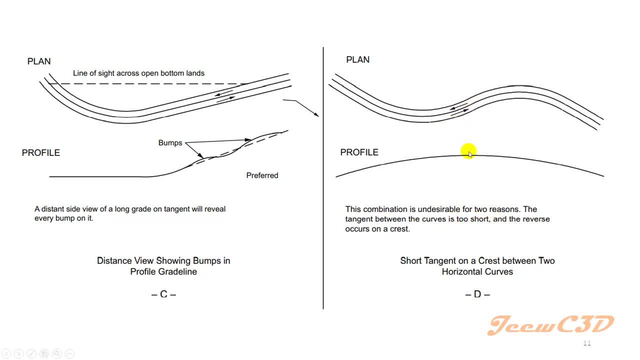 it is too short, and this reverse curve occurs on a crest. so this crest, the crest, is the top point. so at this top point the gradient is very low. it is close to 0. here the gradient is somewhat higher. which side also somewhat higher, here the gradient is very low. so it is a tendency to collect water at. this point. and if you see here it is straight on the right side, so you can't have an opposite them. and if you see here, if it is straight on here, then this will be also a point, a attachment, and if you have, and if you have any similar type in between two points, then increases the gradient also, it doesn't matter. 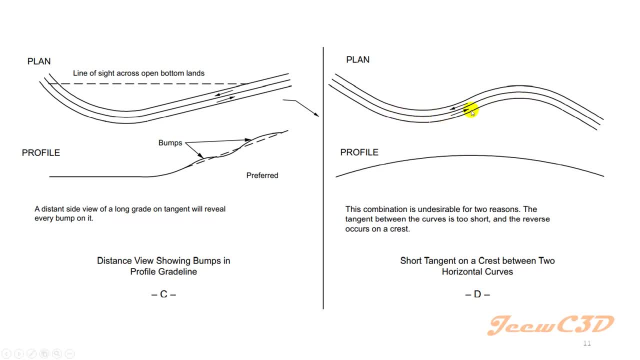 have a reverse curve. there will be a level crown area, you call it. there will be a level road because super elevation occurs, for the water flows this side. according to this super elevation, according to this curve, water flows this side. so the road is turning this side here and turning this side here. 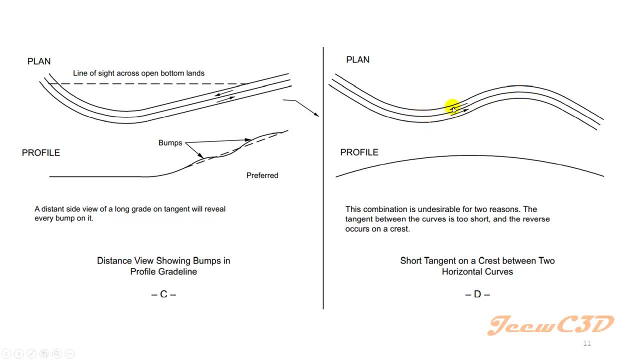 so this road have to rotate to the other side in this area. so in this area you may have a lower gradient road or lower super elevation road, especially you will have a zero super elevation here. so here you have the zero super elevation, you have the zero gradient, so there is a very 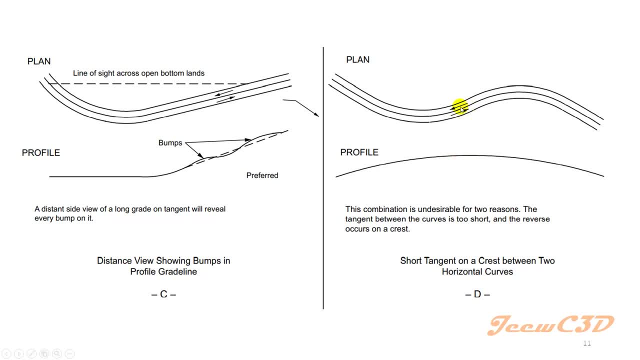 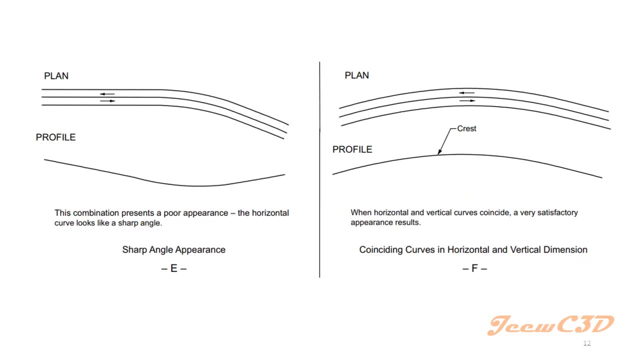 high tendency to collect water in this area, so accident may be very frequent in this areas. if you design the horizontal alignment and vertical alignment like this, then also we have another scenario where you have a shorter sag curve, smaller sag curve, with a sharp horizontal curve. so this arrangement, make this the make this horizontal curve more sharper. 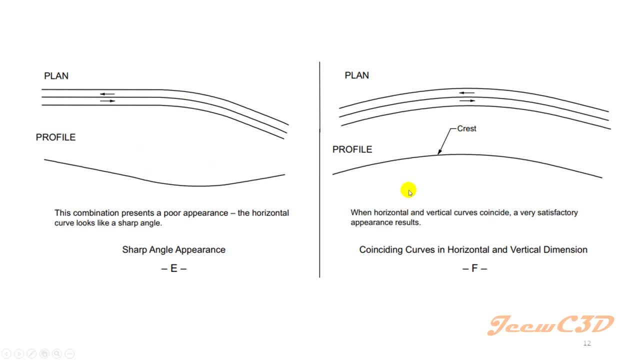 so instead you can have a first curve with a long curve, with a long first curve. also, you can have long sag curve as well. both these are okay without this one, which is has a sharper curve and a smaller, very, uh, shorter sag curve. the length of the curve is very low. so there are some other scenarios. 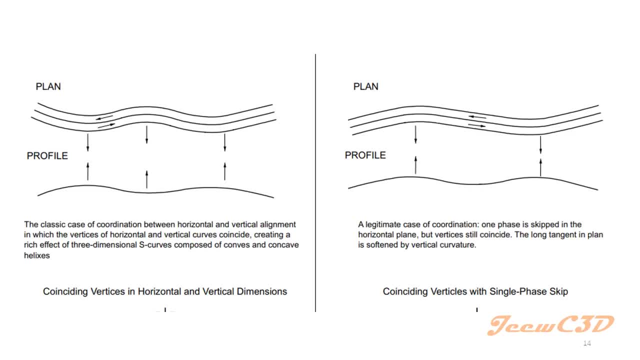 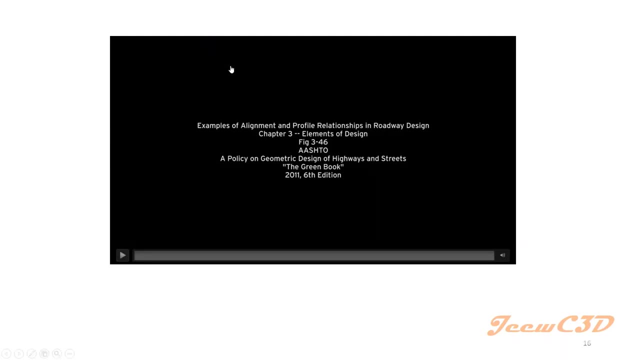 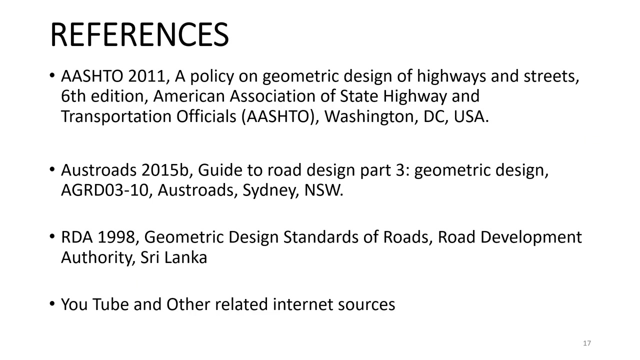 so you can uh watch them, you can see them and learn them uh, by yourself. uh, if uh, then i will be showing you a small video of what we have discussed so far. that's about horizontal and vertical coordination in geometric design of highways. with that we will be concluding the theory part of 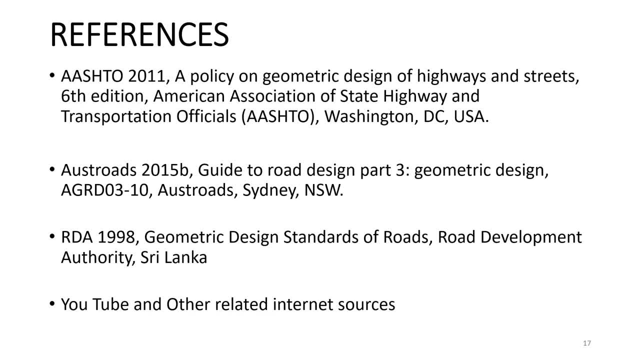 geometric design in highway engineering. These are the references I have used in throughout my lecture series. So far, we have learned a lot of things and there are a lot more to be studied by yourself because, depending on the time schedule, I cannot teach everything related to geometric design, but I have. 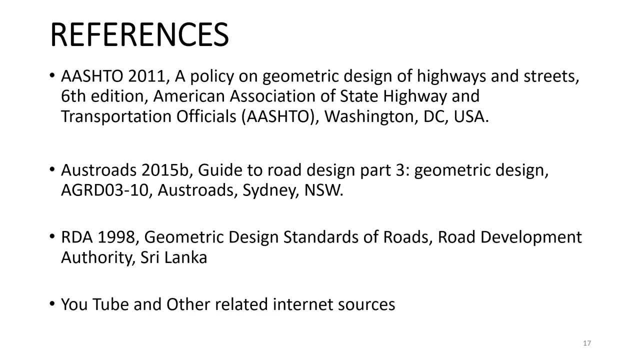 given one of the most important components in geometric design so that you can follow geometric designs after you go to the industry. So I hope you will. you have a good, good knowledge using this lecture series and I wish you will ask questions and ask for clarification through the forum I have. 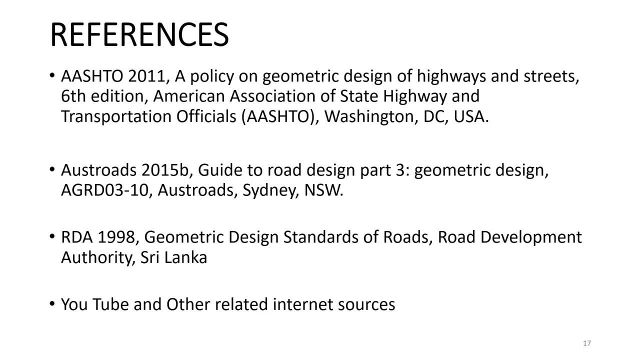 created in fields. Again, if you have problems, I will be conducting a zoom lecture session or zoom discussion session in the coming weeks so you can ask your questions for clarification, So I can explain them more to you, so that you can understand them very clearly. and then in the coming weeks we will be starting the civil 3d design. 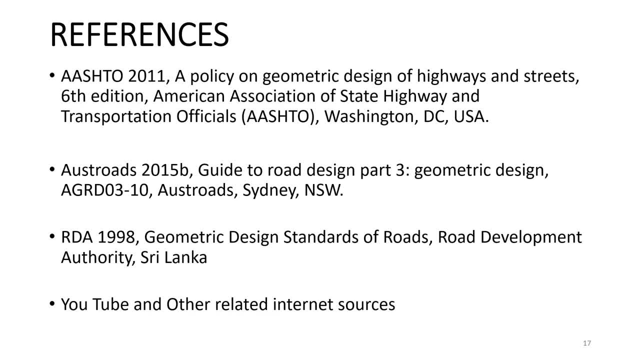 software. So with civil 3d you can learn more and you can practice these learned theories and learned geometric design components using real-world examples. So thank you very much for watching this video. I hope you have enjoyed this video That will be in the coming weeks, So before starting civil 3d, I hope you can. 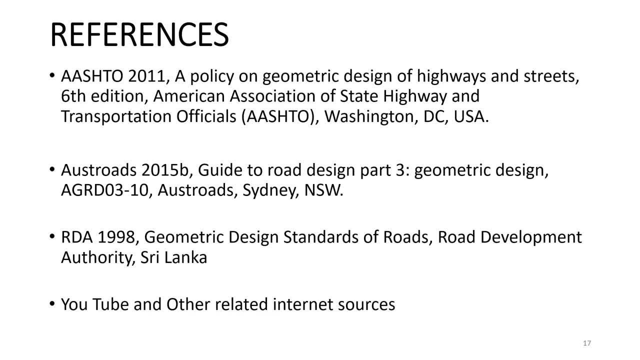 ask me any questions for clarification or anything you need to know about this geometric design through the forum I have created for you or otherwise, in the zoom discussion session, which I will be informed you later day. what is the exact date and time? So until then, thank you for all I.